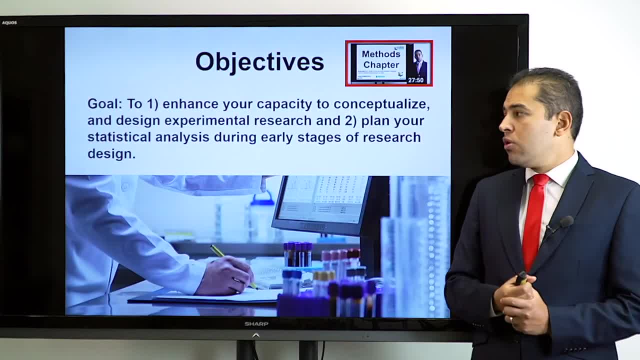 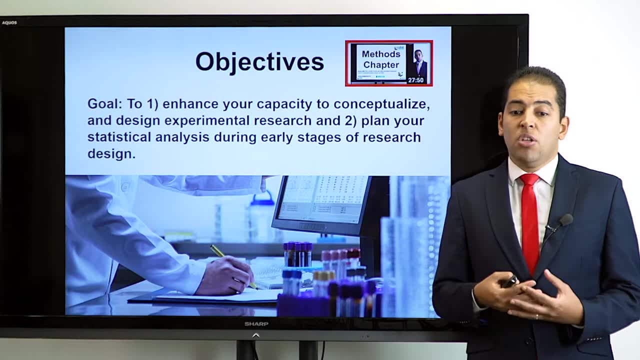 experimental research methodology. Now let's move talking about the objective of this presentation. Well, the goal number one of this presentation is to enhance your capacity to conceptualize and design experimental research. number one and number two is to plan your statistical planning during early stages. 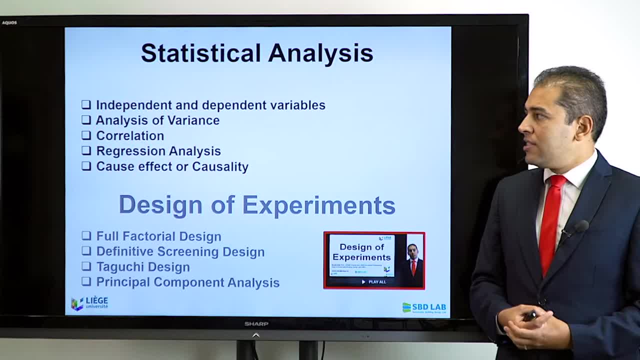 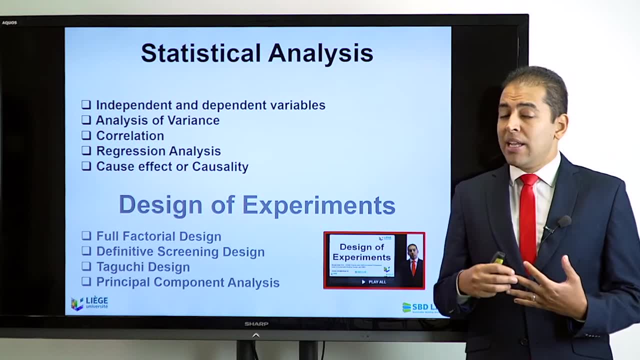 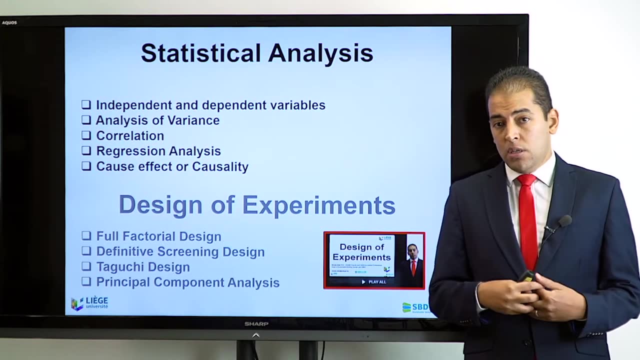 of research. When we talk about statistical analysis, we are talking here about different variables, but mainly, I'm talking here about defining your independent and dependent variables: analysis of variance, the regression analysis and the cause effect or the causality effect. In this sense, this is the basic, or this is the foundation that will take you to the 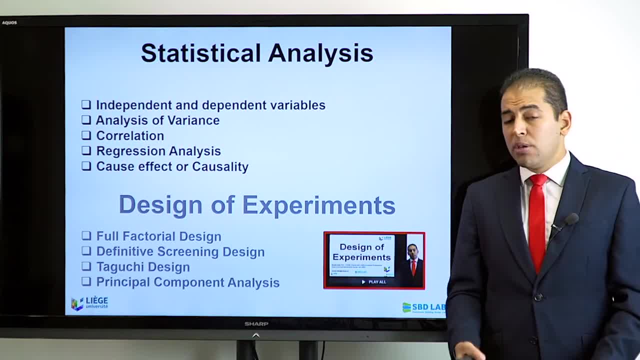 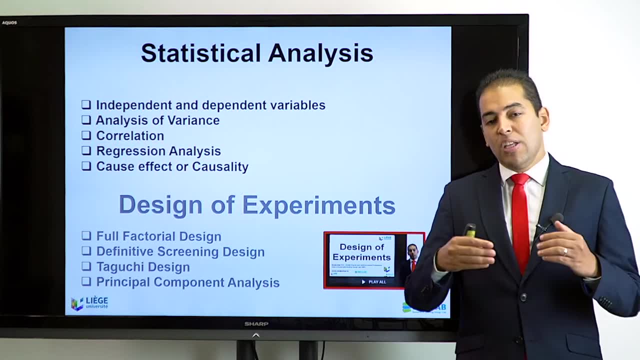 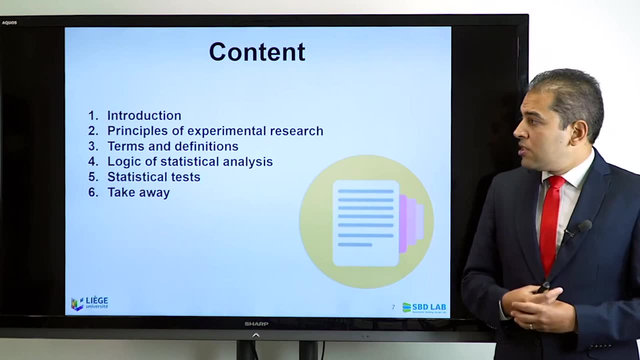 next step of conducting design of experiment, and in the following presentation I will talk in detail about how conducting the design of experiments. but let us focus now on statistics, so that we are able to go later on on designing our experimental statistics. The content of today's presentation is mainly an introduction, talking about the 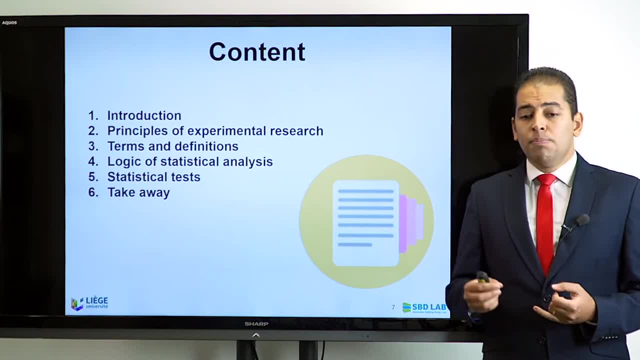 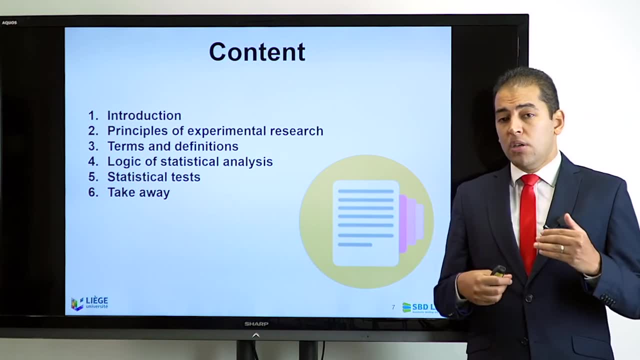 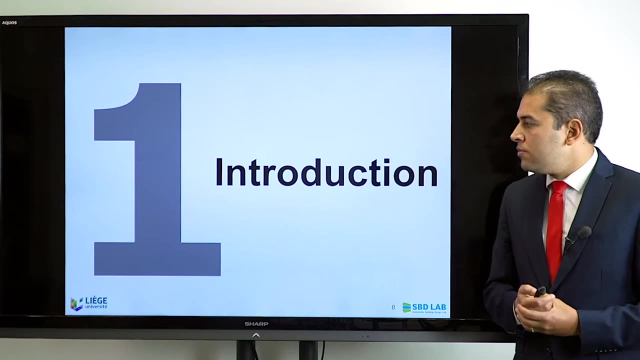 principle of experimental research, reminding you about them, terms and definitions, logic of statistical analysis, statistical tests that are commonly used and how to go in order to conduct them, and, finally, some takeaway message. So let's start with the introduction. What is the nature of? 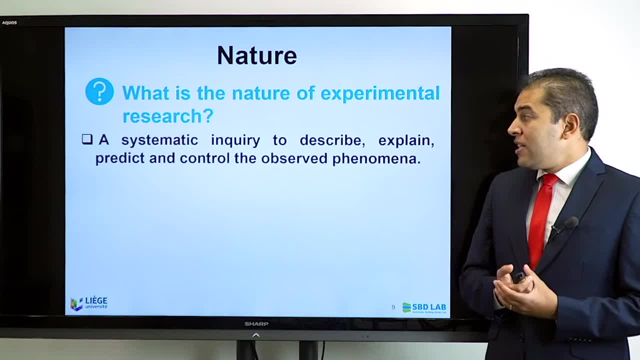 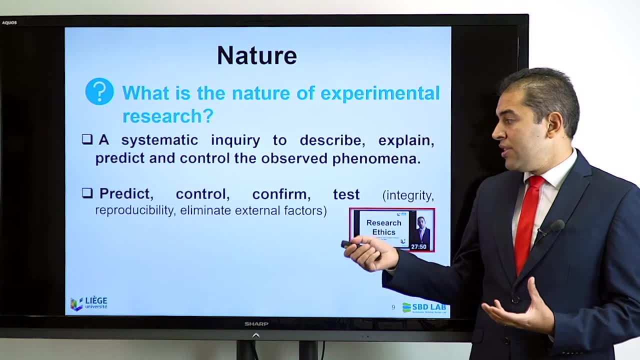 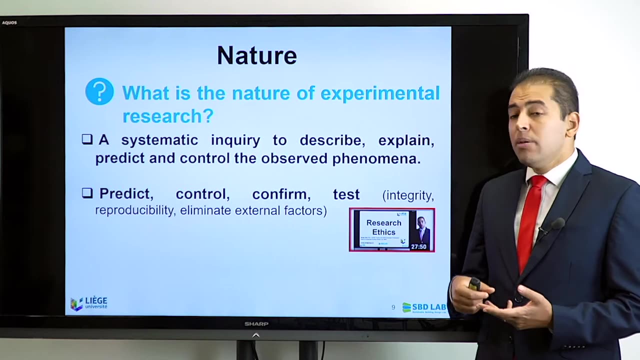 experimental research. Well, it is a systematic inquiry to describe, explain, predict and control the observed phenomena. and in this sense, we seek to predict, control, confirm the tests and test while taking into account integrity, reproductibility and eliminate external factors. and in 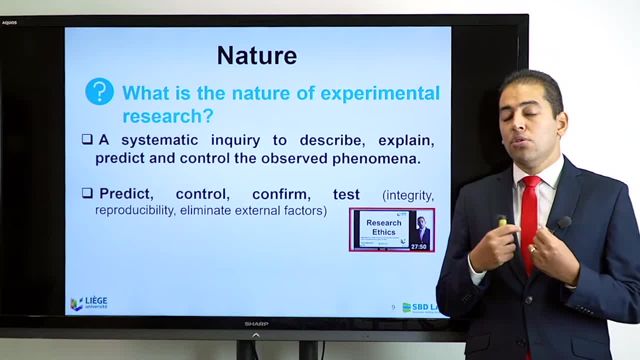 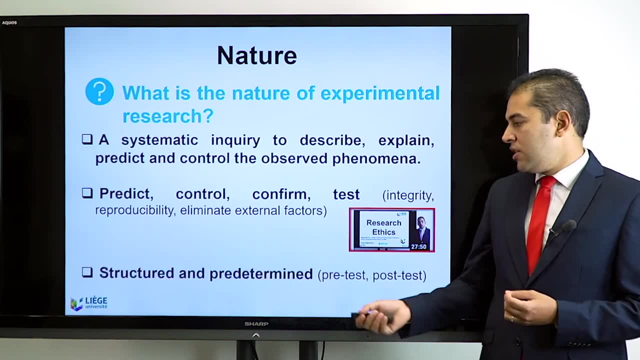 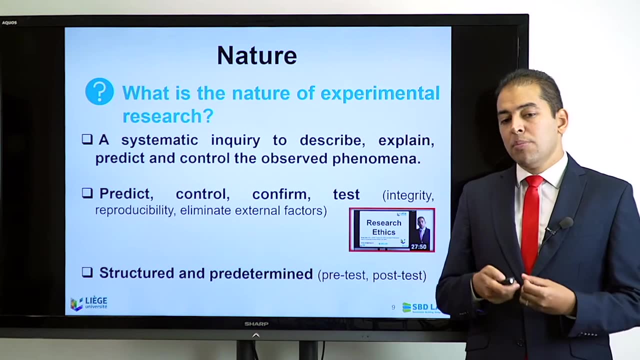 previous presentation on control, we talked how to make sure that we try to reduce noise or external neutralize all external factors. So in this sense it is structured and pre-determined. Experimental research is structured and pre-determined and you must have a pre-test and a post-test. 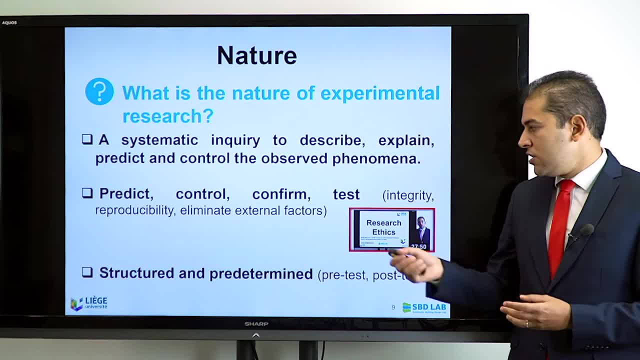 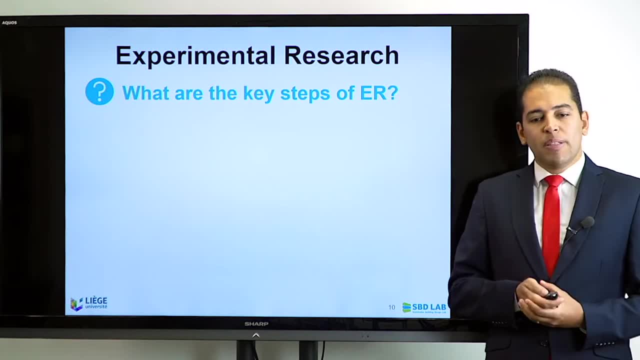 Have a look at my previous research on research ethics if you are interested to know more about integrity. Well further with experimental research. what are the key steps for experimental research? First of all, we have to have knowledge and experience about statistics, and this makes the importance of this. 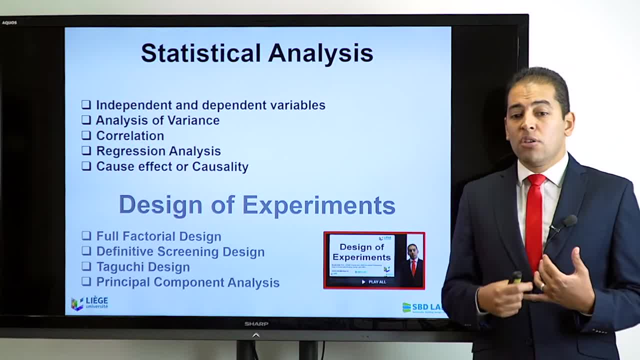 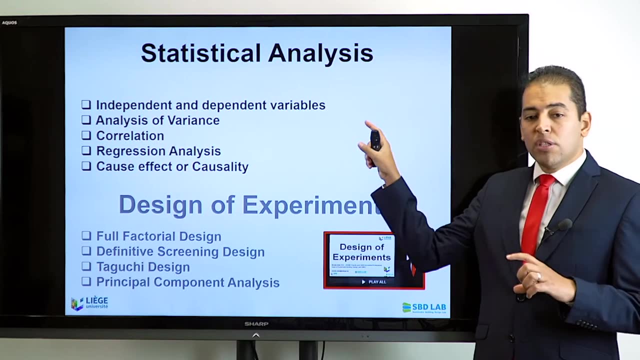 talking here about different variables, but mainly I'm talking here about defining your independent and dependent variables: analysis of variants, the regression analysis and the cause effect or the causality effect. In this sense, this is the basic, or this is the foundation that will take you to the 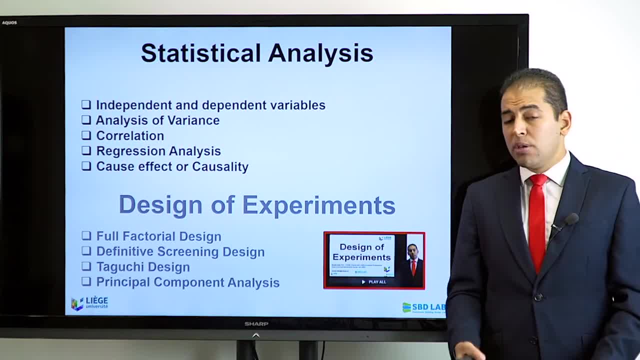 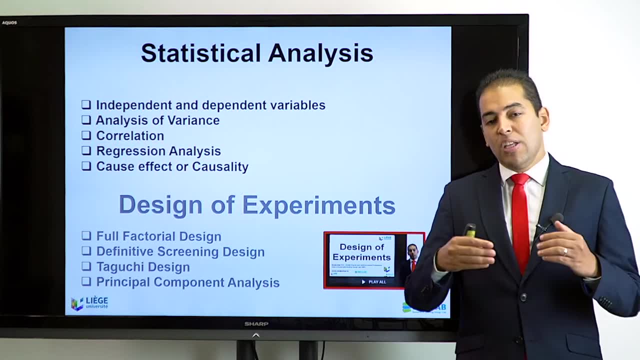 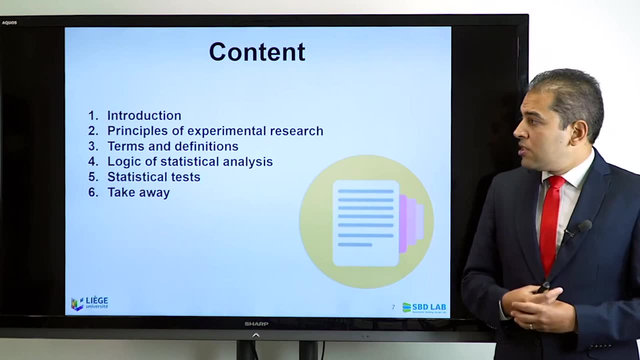 next step of conducting design of experiment, and in the following presentation I will talk in detail about how conducting the design of experiments. but let us focus now on statistics, so that we are able to go later on on designing our experimental statistics. The content of today's presentation is mainly an introduction, talking about the 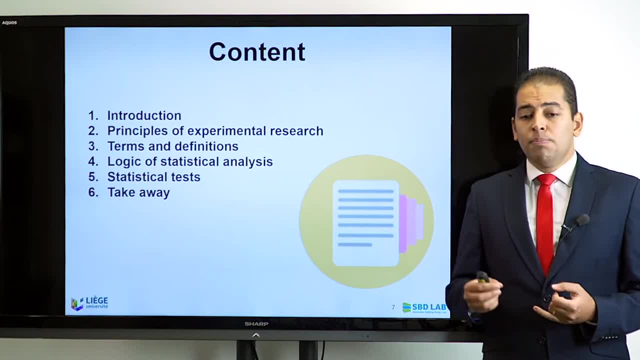 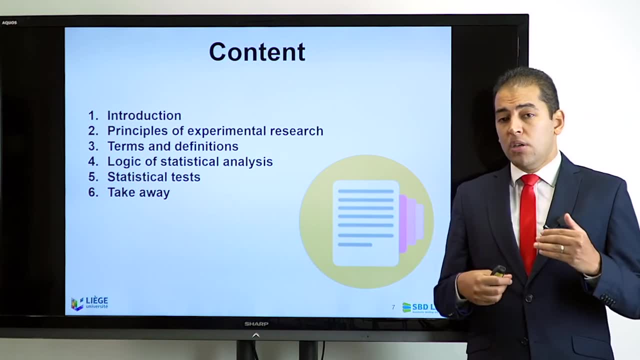 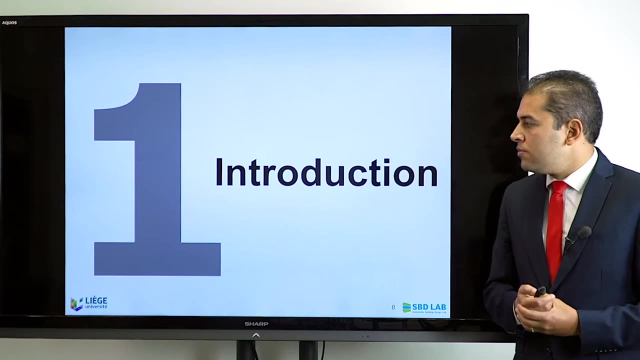 principle of experimental research, reminding you about them, terms and definitions, logic of statistical analysis, statistical tests that are commonly used and how to go in order to conduct them, and, finally, some takeaway message. So let's start with the introduction. What is the nature of? 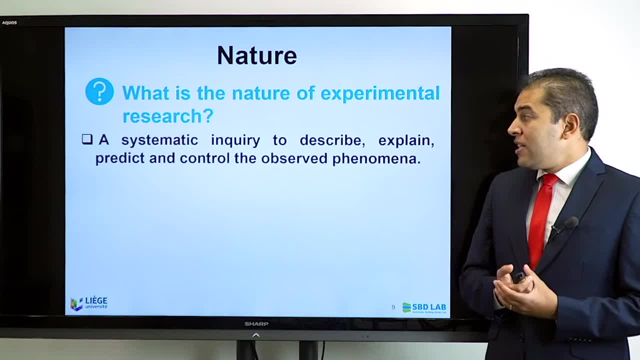 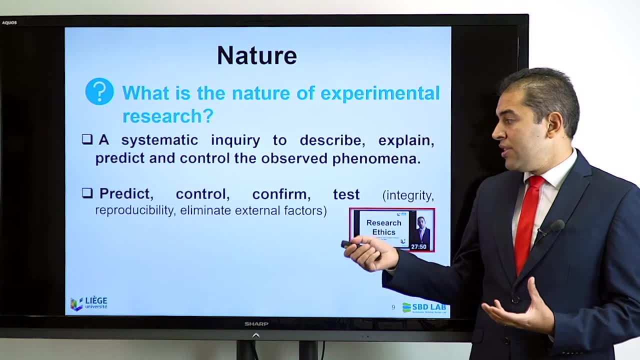 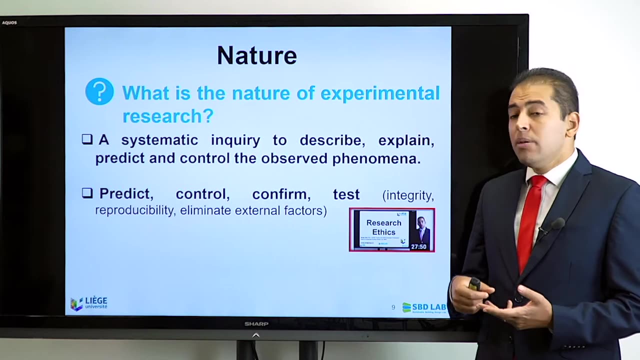 experimental research. Well, it is a systematic inquiry to describe, explain, predict and control the observed phenomena. and in this sense, we seek to predict, control, confirm the tests and test while taking into account integrity, reproductibility and eliminate external factors. and in 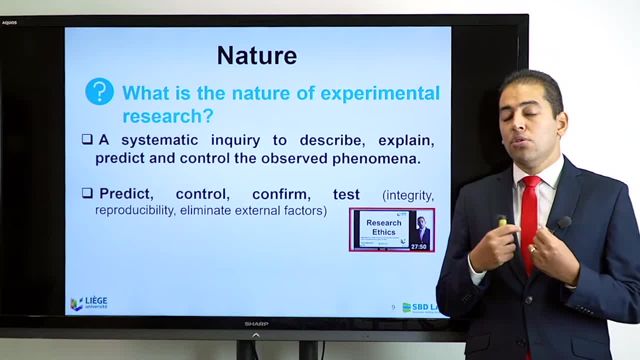 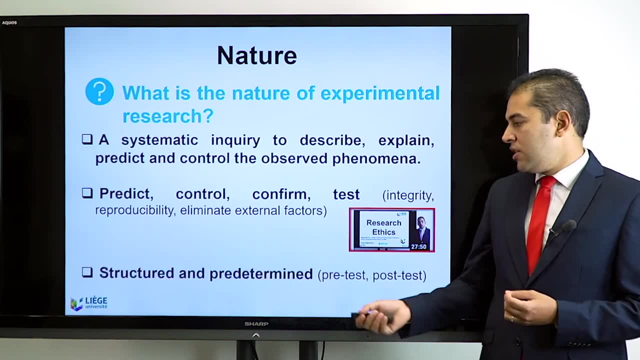 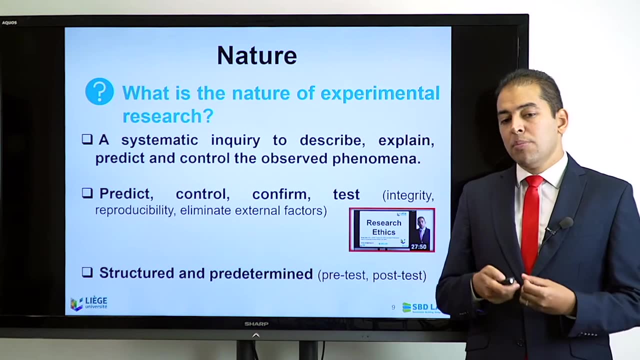 previous presentation on control, we talked how to make sure that we try to reduce noise or external neutralize all external factors. So in this sense it is structured and pre-determined. Experimental research is structured and pre-determined and you must have a pre-test and a post-test. 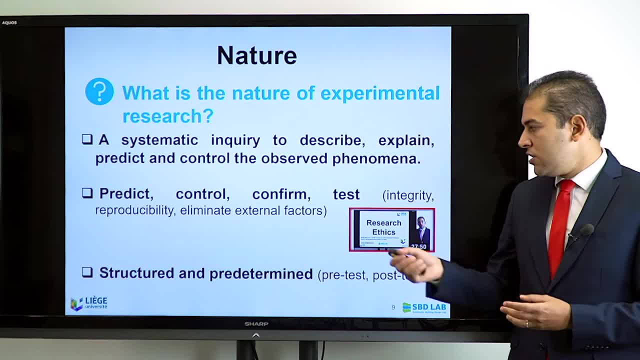 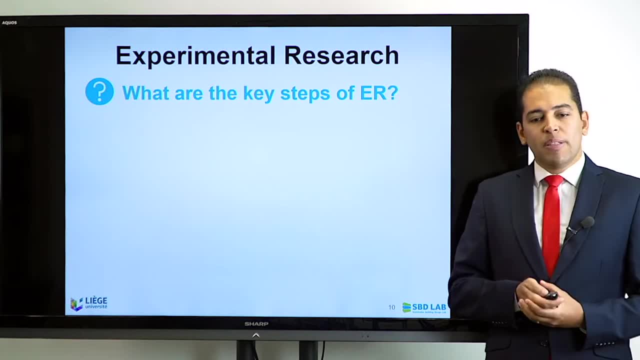 Have a look at my previous research on research ethics if you are interested to know more about integrity. Well further with experimental research. what are the key steps for experimental research? First of all, we have to have knowledge and experience about statistics, and this makes the importance of this. 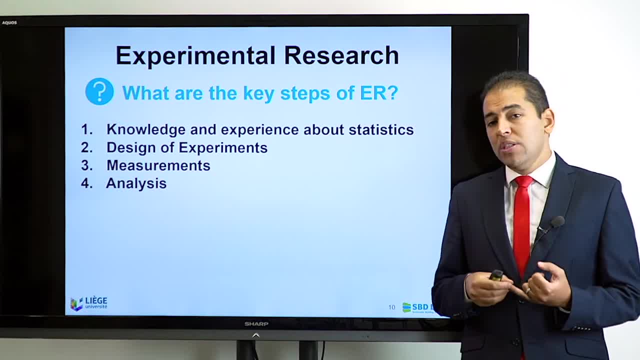 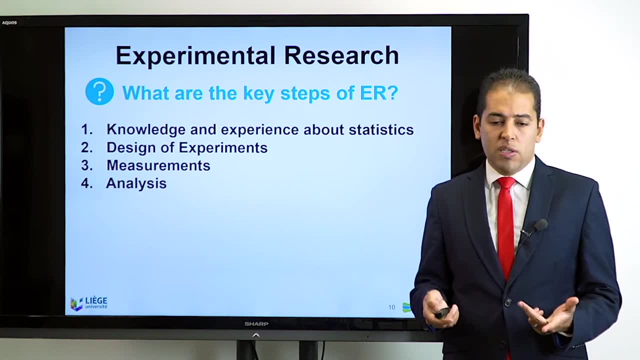 presentation. Then we will design our experiment. Once we design it, we can conduct our measurement and perform our measurements, and then comes the analysis, the post-processing of result and the data visualization. So statistical analysis is not the last part of your research. that will be performed after. 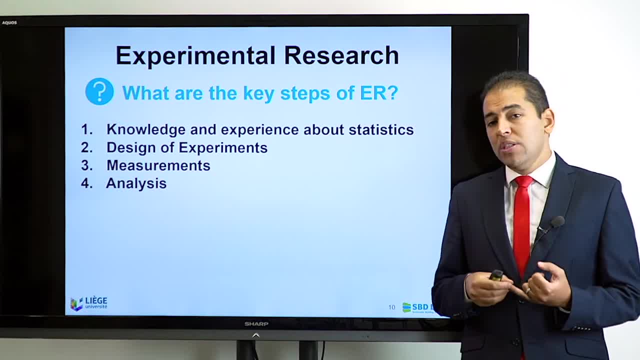 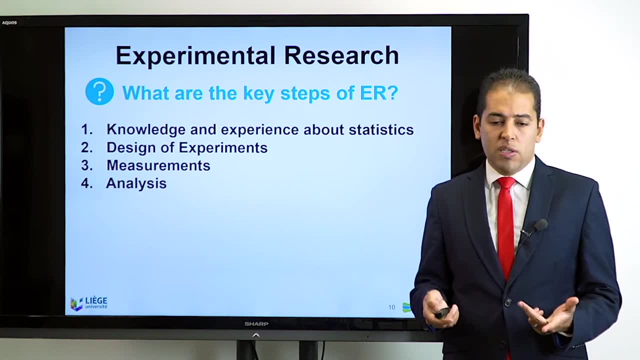 presentation. Then we will design our experiment. Once we design it, we can conduct our measurement and perform our measurements, and then comes the analysis, the post-processing of result and the data visualization. So statistical analysis is not the last part of your research. that will be performed after. 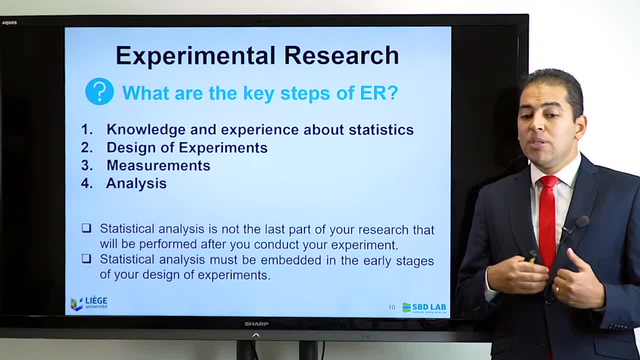 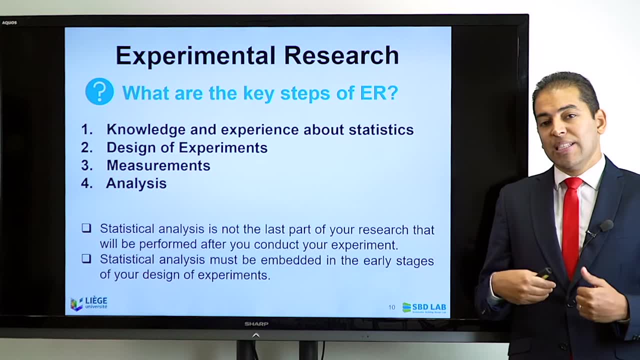 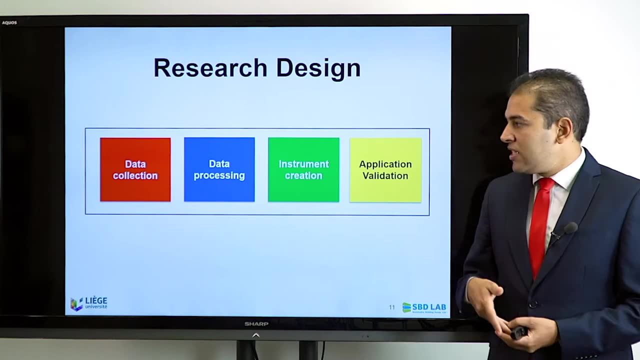 you conduct your experiment. Statistical analysis must be embedded in the early stage of your design of experiment. Therefore, it's very important to know and learn about statistics before designing your experiment and keep into account that many scholars or researchers or scientists they start collecting data and after that they start to think how to process them and 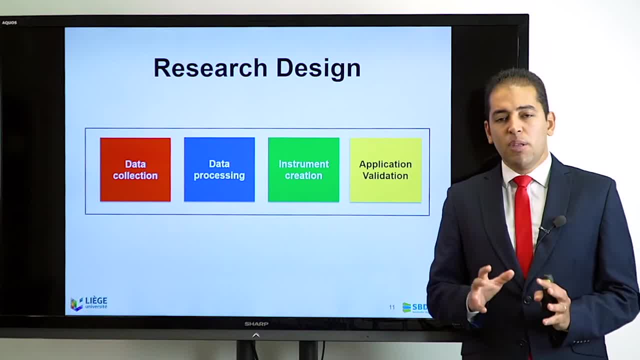 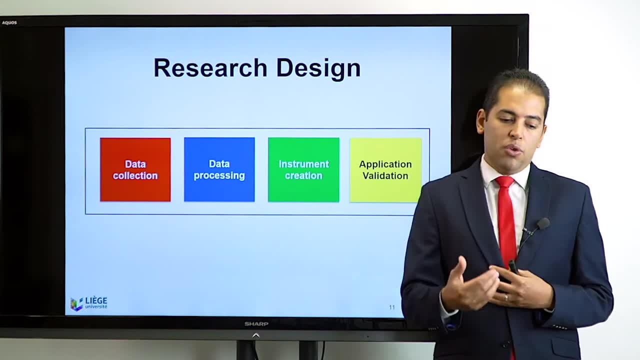 how to make sense of them, and this is totally wrong. Actually, from the beginning, you have to consider your design of experiment, take into account what kind of statistical test you are looking to conduct, what kind of data you conduct, and then you start collecting data, not the other way. 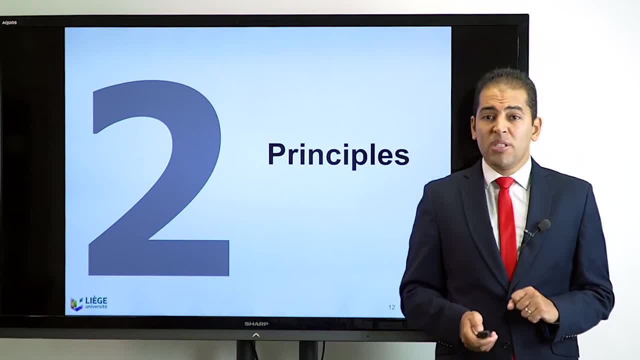 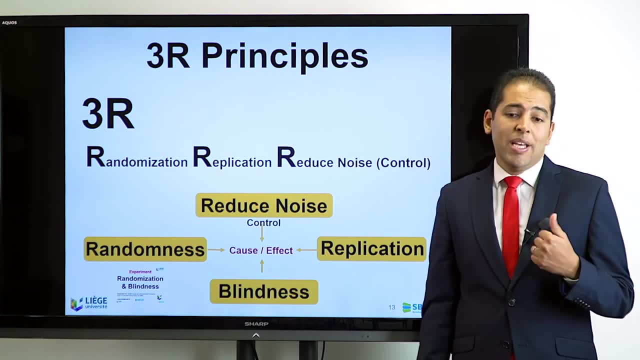 around Now just a very fast reminder on the principle of experimental research. As we mentioned before, the three R's are the principle of experimental research, Randomization, replication and reduction of noise or control, and the advantage of experimental research that it allows you to do that. 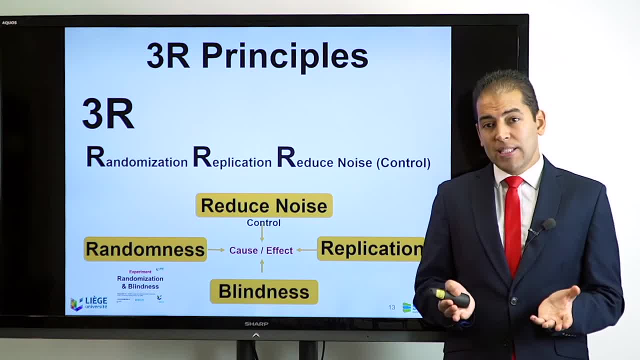 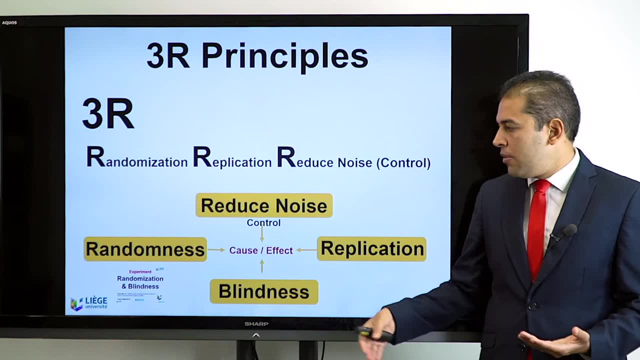 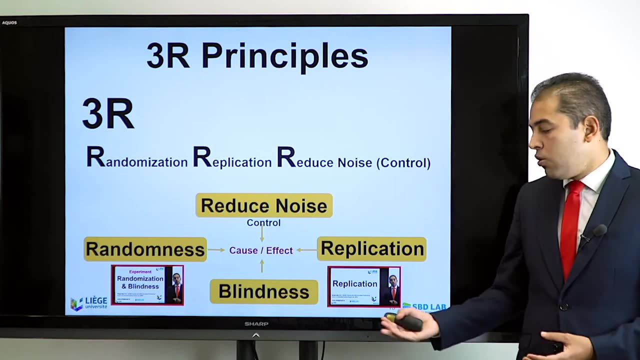 So, in a controlled environment for testing, you have to be able to conduct those three elements. and don't forget that blindness is considered most of the time as part of the randomization. If you want to know more about randomization, or blindness, or replication, you can watch the. 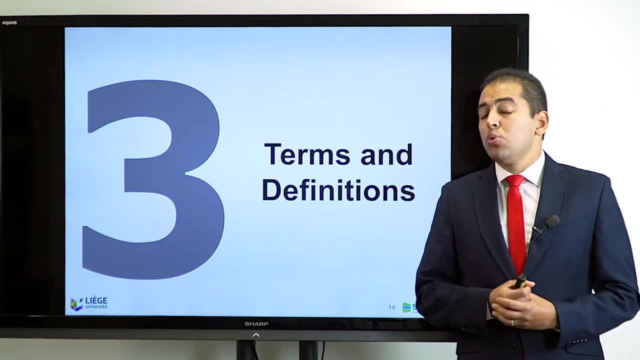 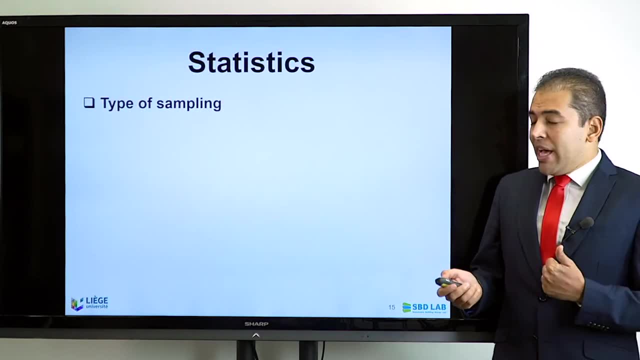 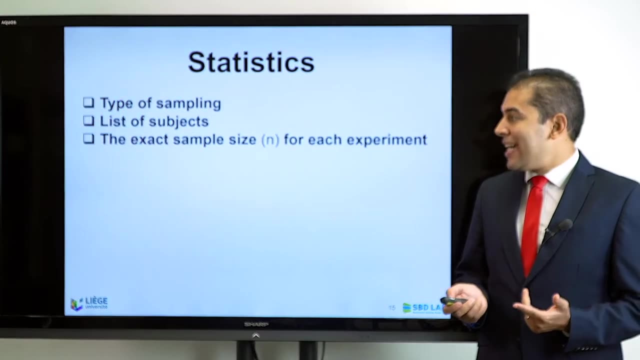 videos here below in the link. Now let's talk to the terms and definitions of experimental research. First of all, statistics. We have to look at the type of sampling that we are using. We have to look at the list of subjects that we are working with. We have to look at the exact sample. 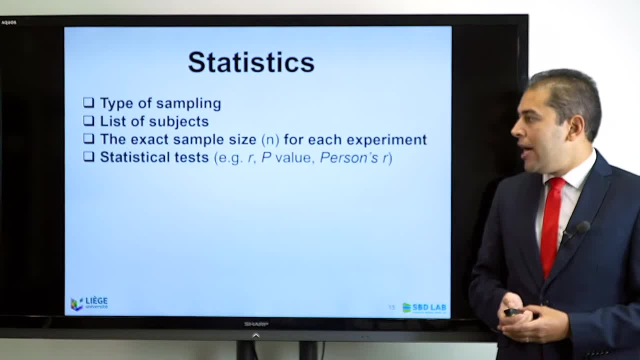 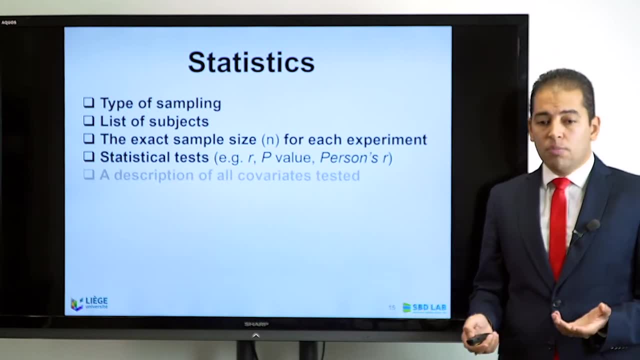 size which is indicated always in the end for each experiment, and you must look at a statistical test that you are looking out for, For example, the R value, the P value, the Pearson's R and so on. So it's very important to look at that and 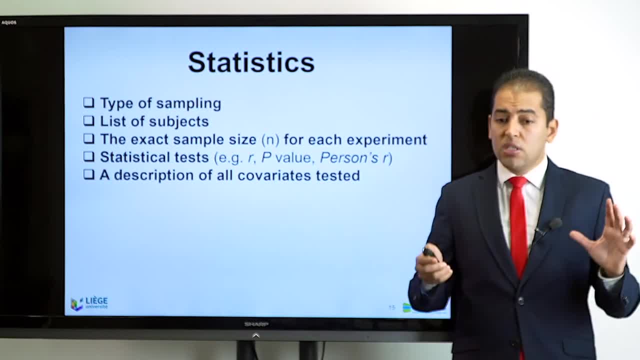 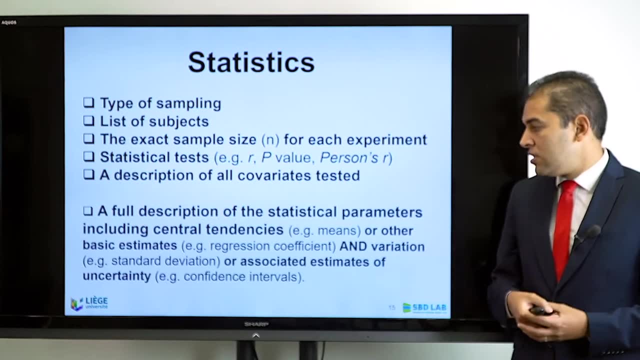 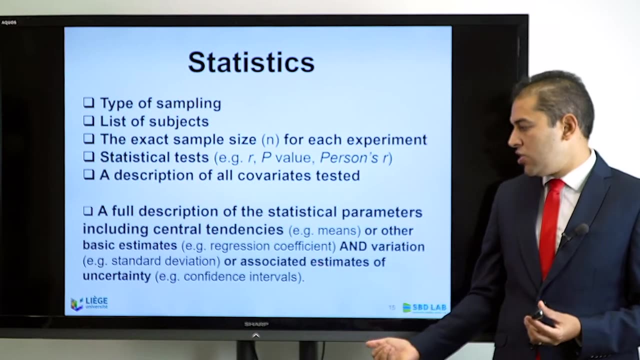 you have to describe your covariates, that you will be tested. This is the first part when I'm talking about statistics. So a full description of the statistic parameters, including central tendencies like the means, or other basic estimates like the regression coefficient or the variation, for example, the standard deviation or 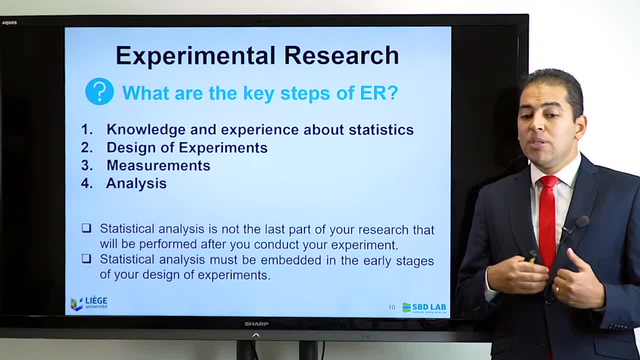 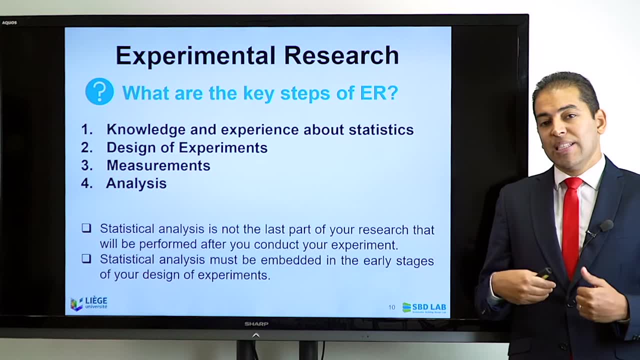 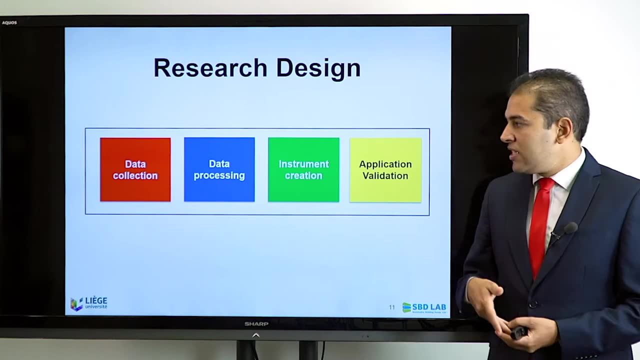 you conduct your experiment. Statistical analysis must be embedded in the early stage of your design of experiment. Therefore, it's very important to know and learn about statistics before designing your experiment and keep into account that many scholars or researchers or scientists they start collecting data and after that they start to think how to process them and 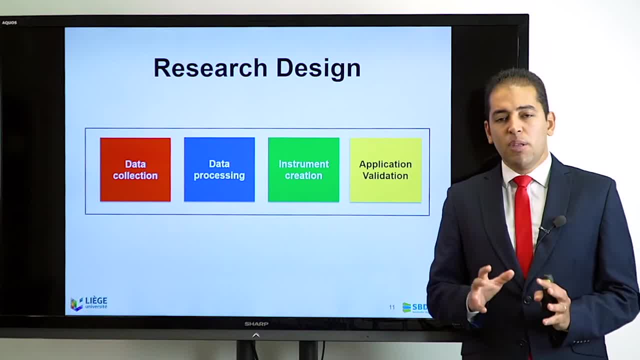 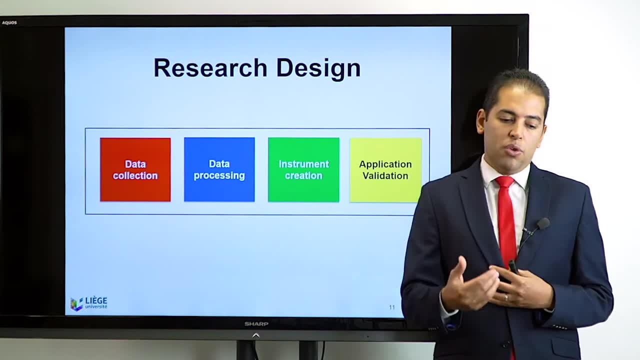 how to make sense of them, and this is totally wrong. Actually, from the beginning, you have to consider your design of experiment, take into account what kind of statistical test you are looking to conduct, what kind of data you conduct, and then you start collecting data, not the other way. 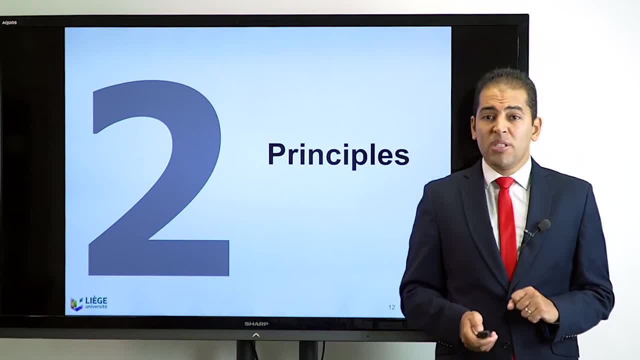 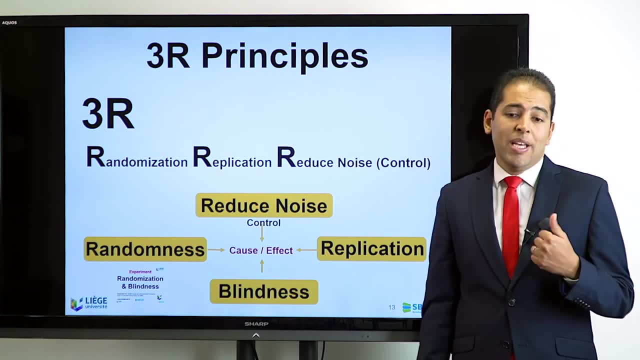 around Now just a very fast reminder on the principle of experimental research. As we mentioned before, the three R's are the principle of experimental research, Randomization, replication and reduction of noise or control, and the advantage of experimental research that it allows you to do that. 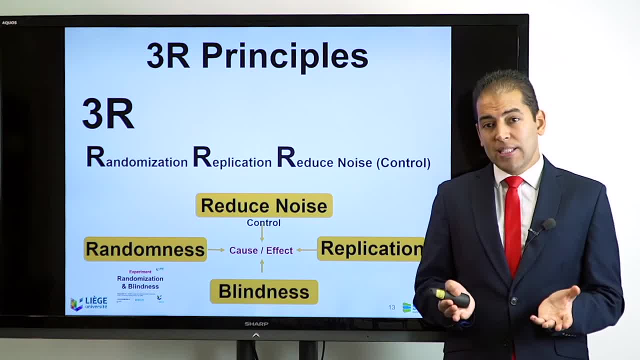 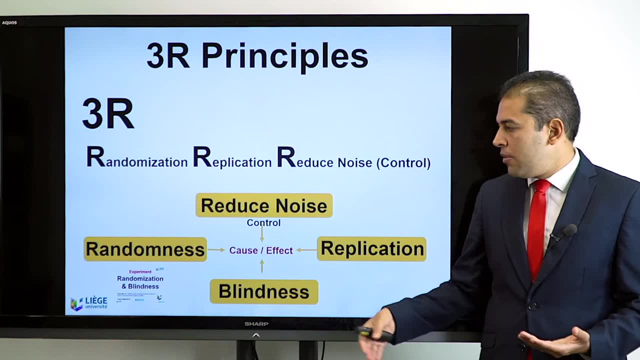 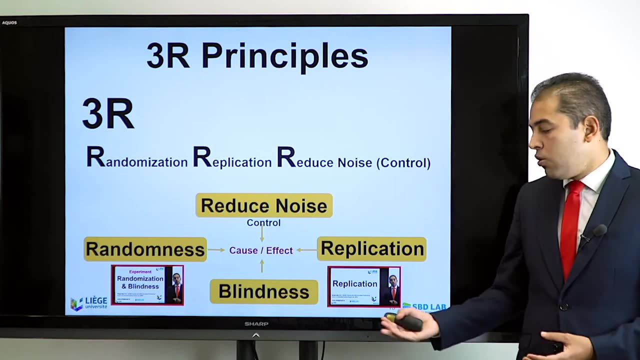 So, in a controlled environment for testing, you have to be able to conduct those three elements. and don't forget that blindness is considered most of the time as part of the randomization. If you want to know more about randomization, or blindness, or replication, you can watch the. 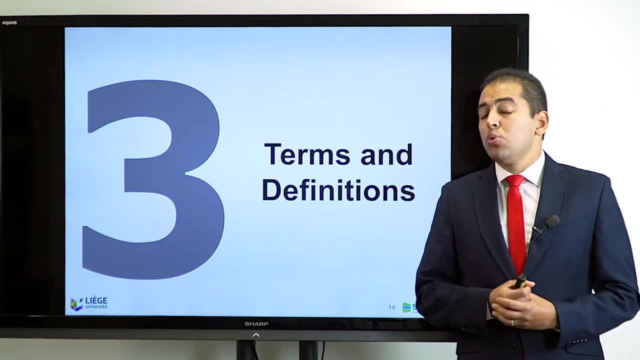 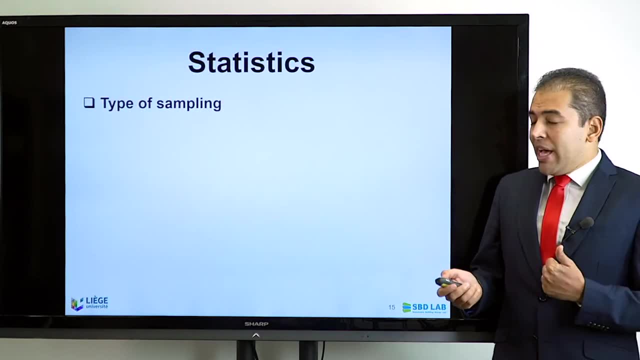 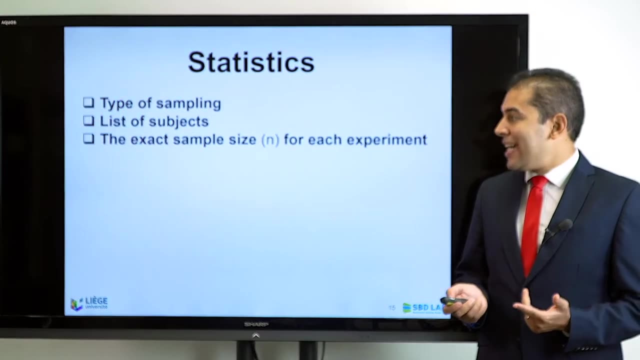 videos here below in the link. Now let's talk to the terms and definitions of experimental research. First of all, statistics. We have to look at the type of sampling that we are using. We have to look at the list of subjects that we are working with. We have to look at the exact sample. 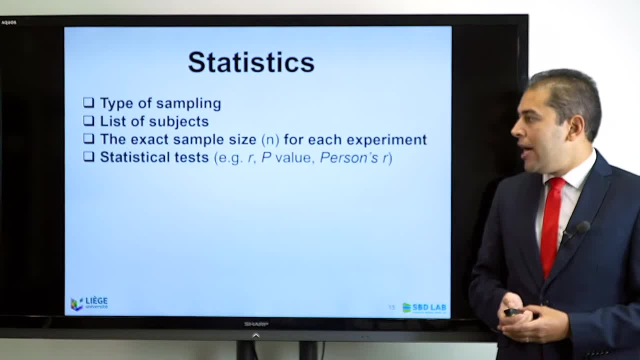 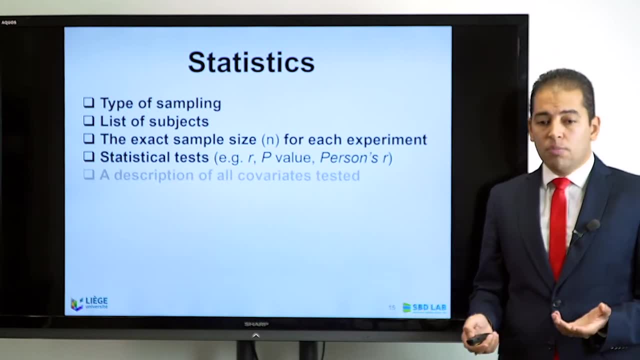 size which is indicated always in the end for each experiment, and you must look at a statistical test that you are looking out for, For example, the R value, the P value, the Pearson's R and so on. So it's very important to look at that and 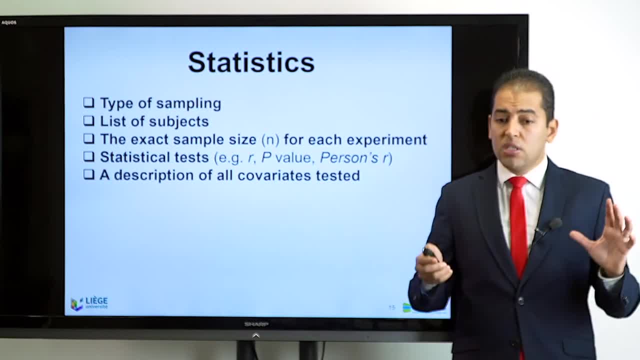 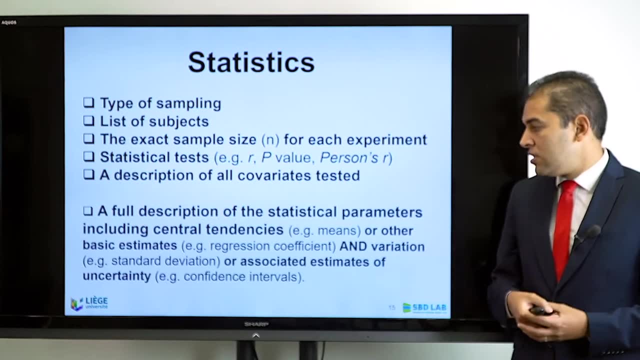 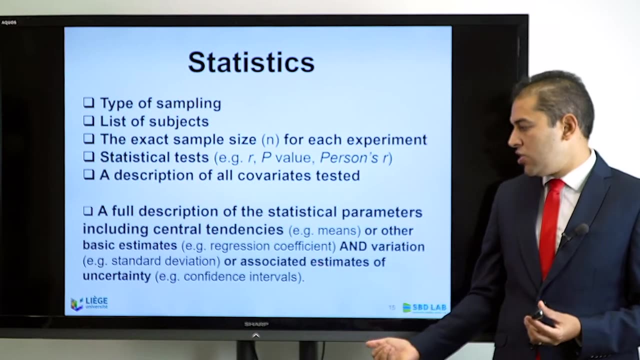 you have to describe your covariates, that you will be tested. This is the first part when I'm talking about statistics. So a full description of the statistic parameters, including central tendencies like the means, or other basic estimates like the regression coefficient or the variation, for example, the standard deviation or 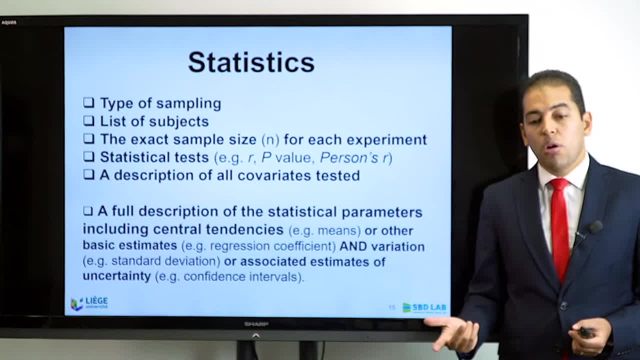 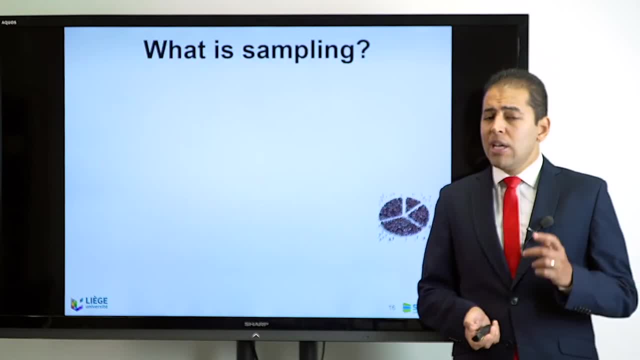 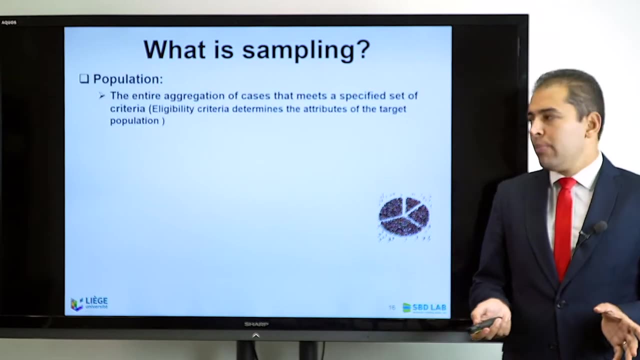 the associated estimates of uncertainty, which is represented through the confidence of interval. They all make part of the process of statistical analysis for your work. Now let's go further in detail and ask some questions here. What is sampling? Well, to understand what sampling, you have to make sure that. 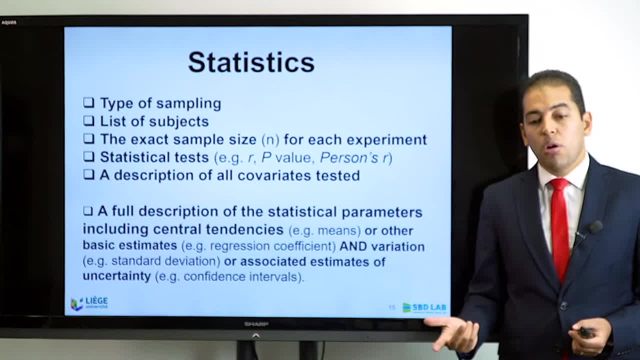 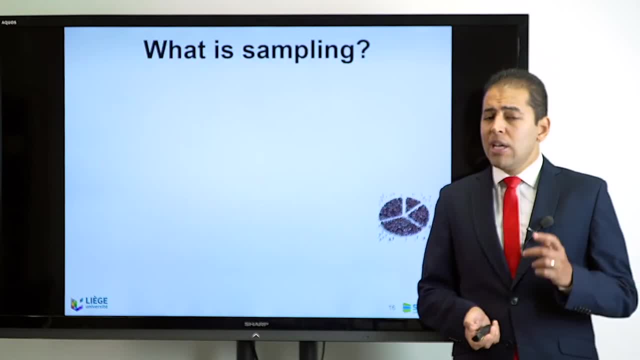 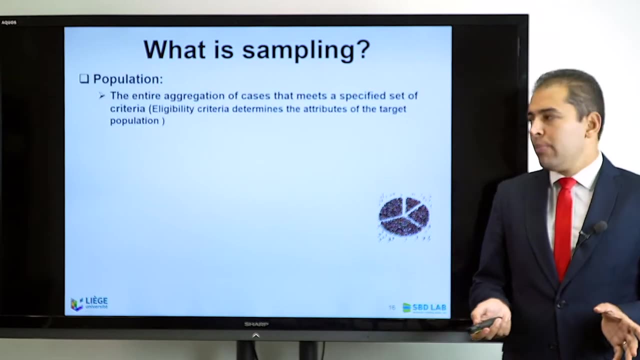 the associated estimates of uncertainty, which is represented through the confidence of interval. They all make part of the process of statistical analysis for your work. Now let's go further in detail and ask some questions here. What is sampling? Well, to understand what sampling, you have to make sure that. 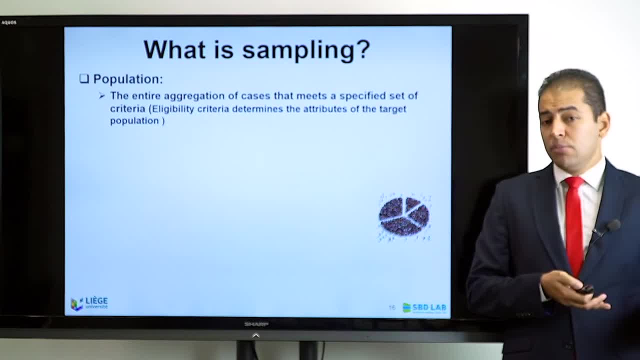 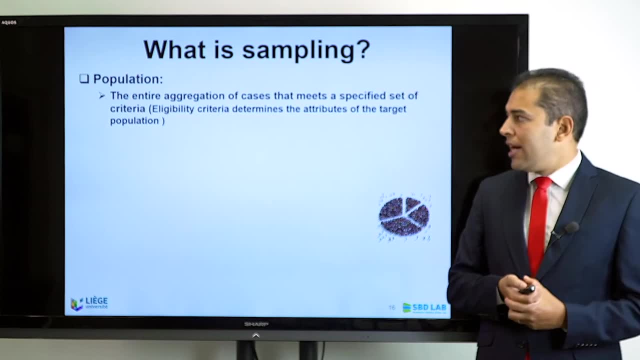 your subject. there is a population of your subject, Whether we mentioned before in the presentation on subjects, they can be human, they can be object, they can be a car, whatever kind of testing subject you are looking at in your experimental setting. But when we look at about 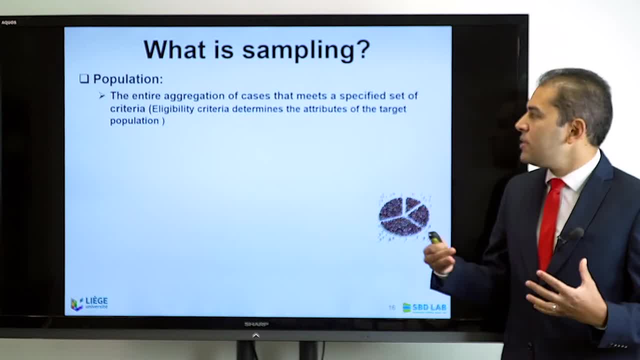 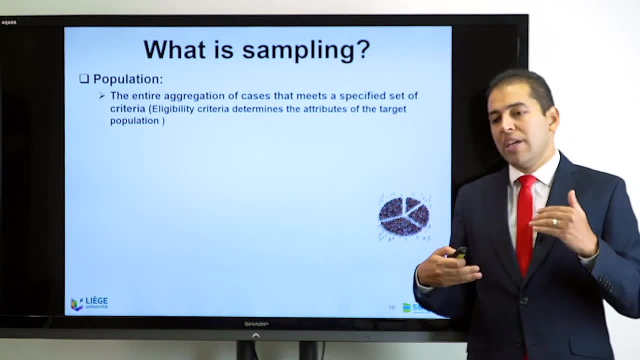 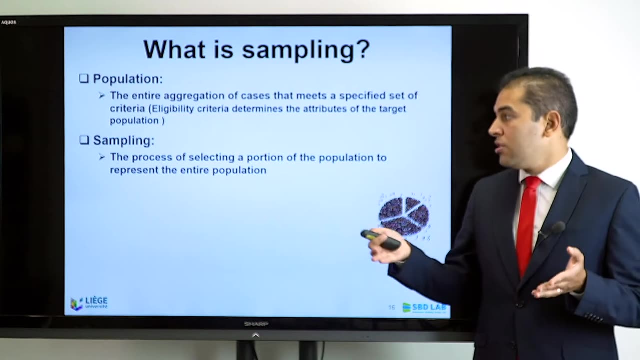 population, it is the entire aggregation of cases that meets a specified set of criteria and in this sense, you must have eligibility criteria and you have to set an inclusion and exclusion criteria to make sure that you are defining your population. Then, from this population, you start the sampling, which is the process. 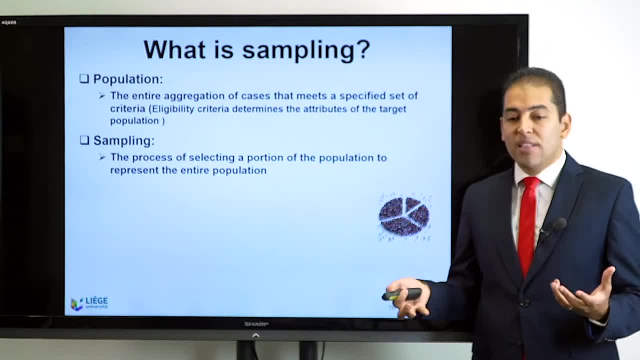 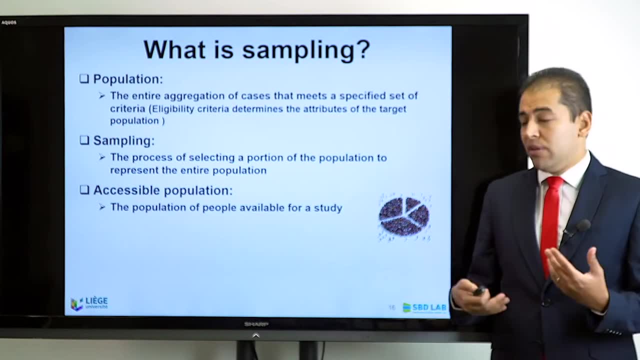 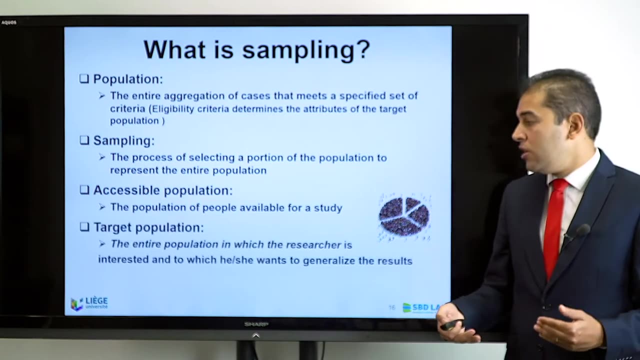 of selecting a population. So you have a portion of the population to represent the entire population, and then you have your accessible population, which is the population of people or subjects, whatever they are. even they are specimens or samples that will be available for your study, for your experiment. and, finally, you must focus on 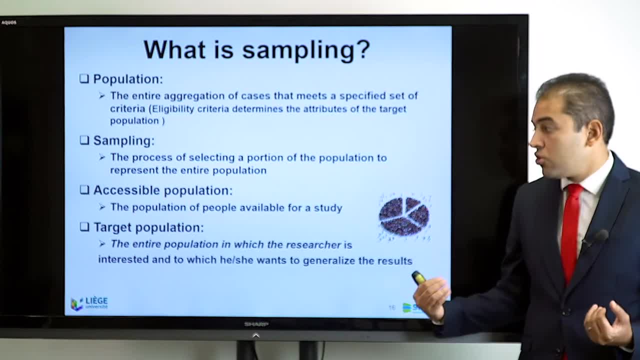 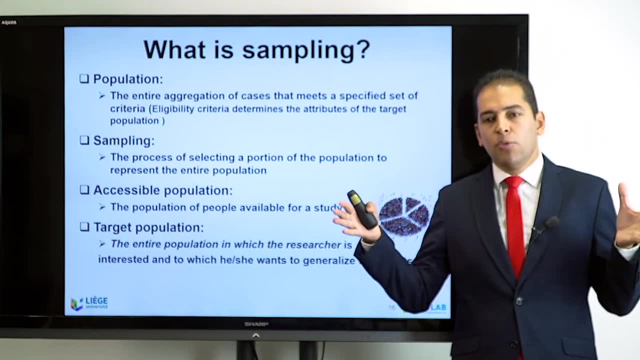 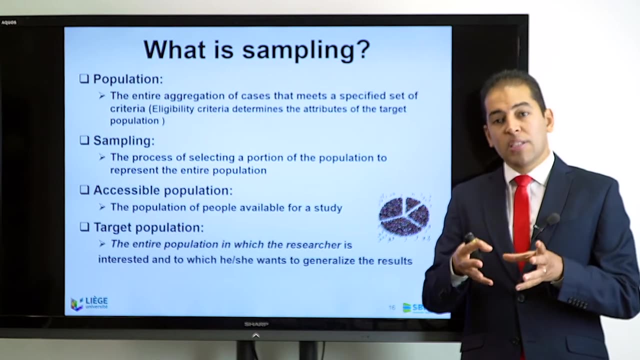 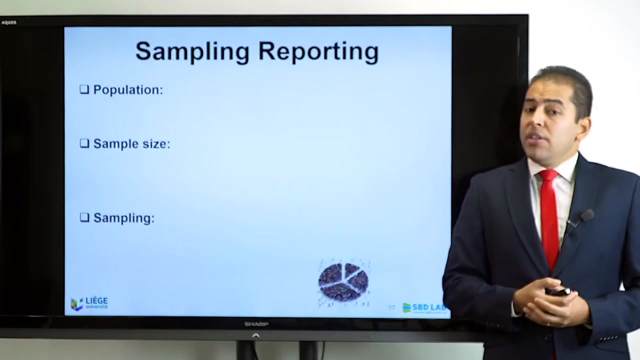 your target population, which is the entire population in which the researchers is interested and to which he or she wants to generalize the results. So, in fact, with sampling, we are reducing the investigated subjects to a number of limited subjects that will allow us to extract or learn from about the overall population, Now very important when we do. 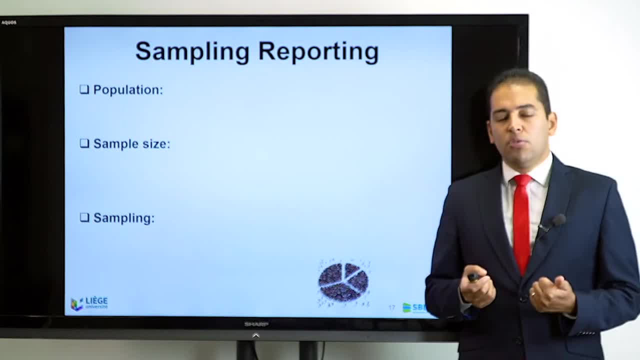 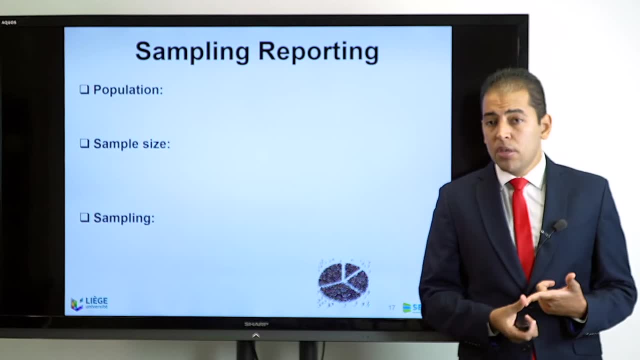 sampling reporting to take into account the following: if you are looking to publish your reports, that you are doing your public, if you will publish your experimental protocol or if you are going to publish your results in a paper at the end of the day, you must be very conscious about reporting. So when we 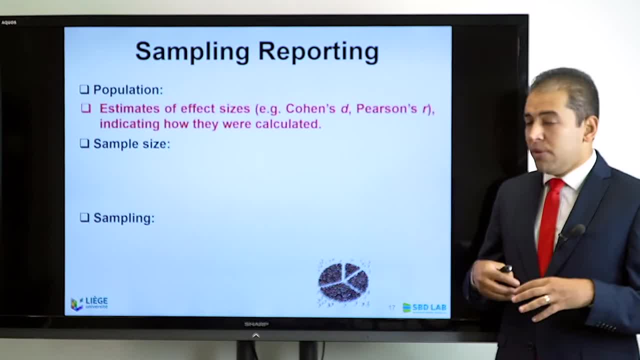 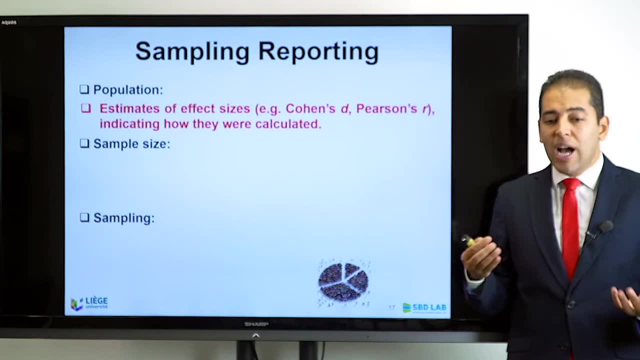 talk about reporting regarding population, you must be very conscious about reporting. So when we talk about reporting regarding population, it is the estimate of effect, of size of your population. For example, you have the Cohen's D, you have the Pearson's R and they are indicating. 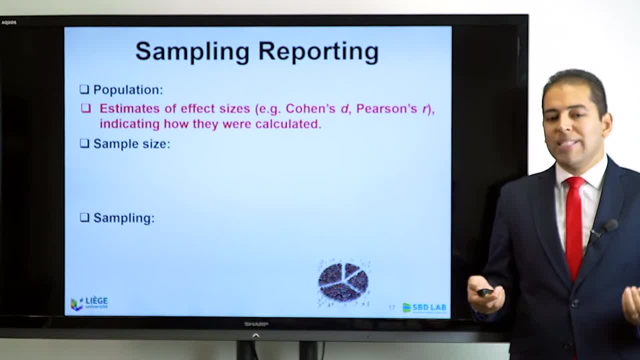 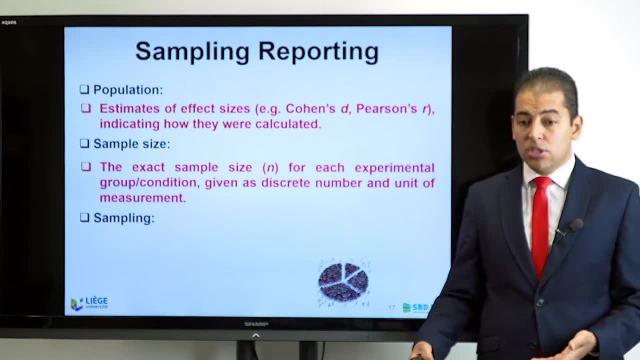 how they were. you must indicate how they were used. When we talk about samples, sampling size, how to report that, you have to have the exact sample size n number for each experimental group and condition given as a discrete number and unit of measurement. and when you are reporting about sampling you have to 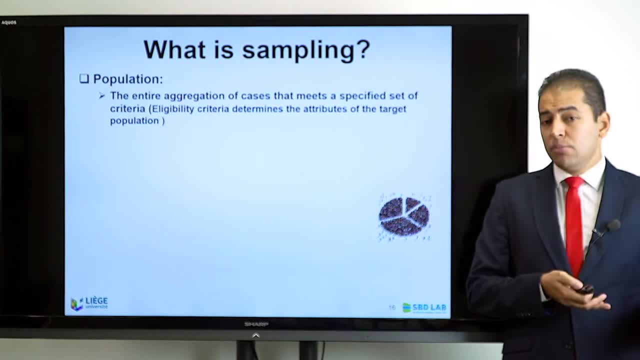 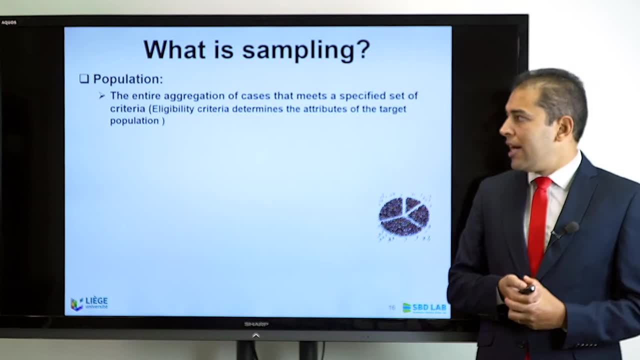 your subject. there is a population of your subject, Whether we mentioned before in a presentation on subjects, they can be human, they can be object, they can be a car, whatever kind of testing subject you are looking at in your experiment setting. But when you 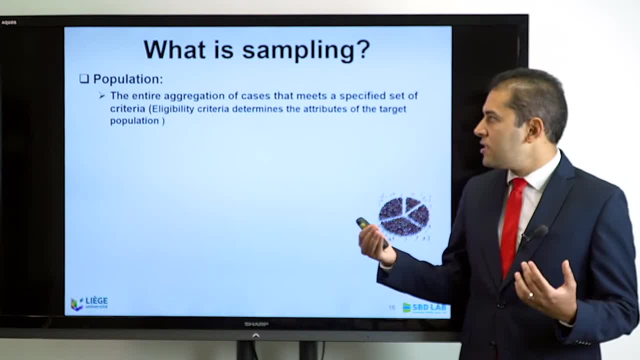 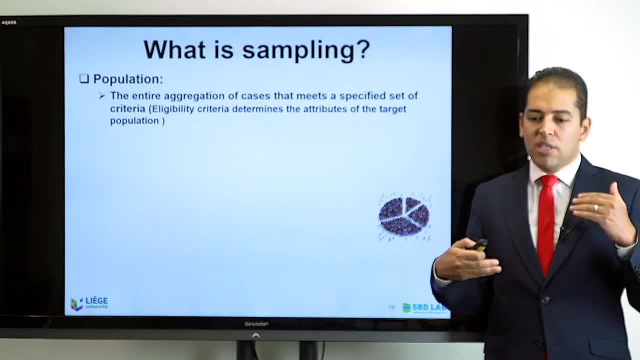 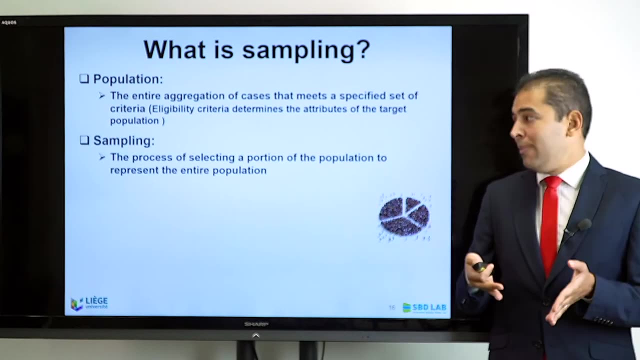 look out about population. it is the entire aggregation of cases that meets a specified set of criteria And in this sense you must have tremendously criteria and you have to set an inclusion and exclusion criteria to make sure that you are defining your population. Then from this population you start a sampling. 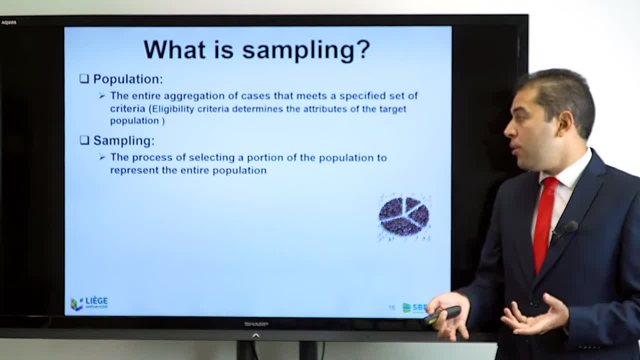 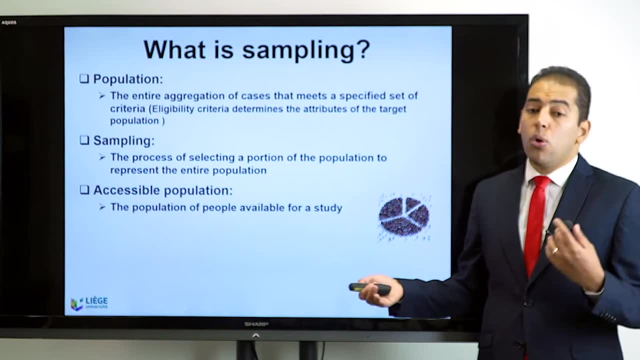 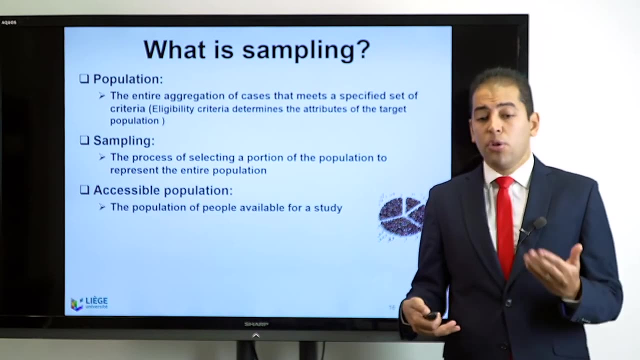 which is the process of selecting a population portion of the population to represent the entire population. and then you have your accessible population, which is the population of people or subjects, whatever they are. even they are specimens or samples that will be available for your study, for your experiment. and, finally, you must focus on your target population. 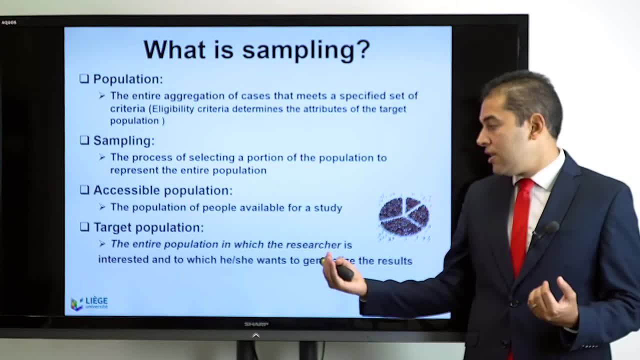 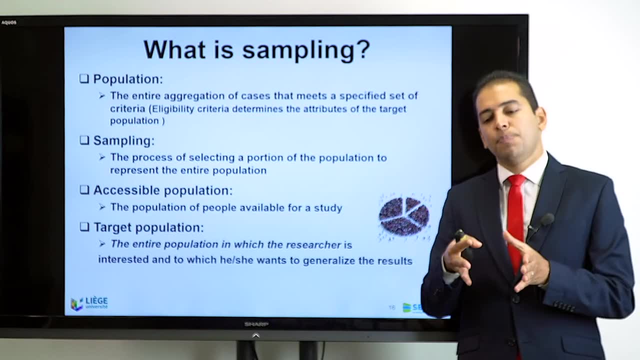 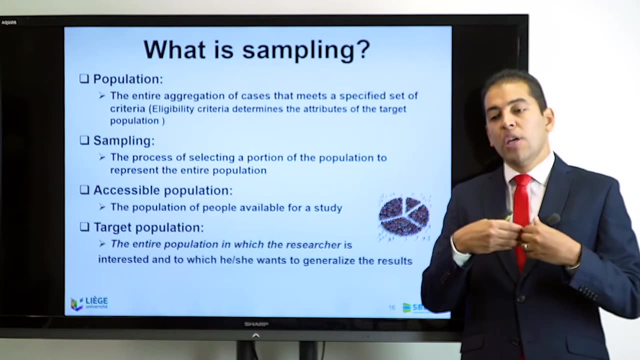 which is the entire population in which the researcher is interested and to which he or she wants to generalize the results. So, in fact, with sampling, we are reducing the investigated subjects to a number of limited subjects that will allow us to extract or learn from about the overall population. 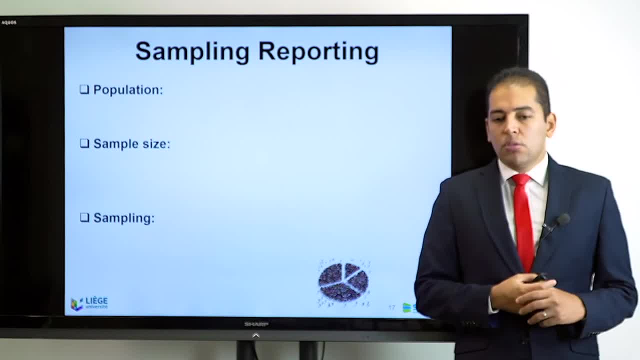 Now very important, when we do sampling, reporting, to take into account the following: If you are looking to publish your reports, if you will publish your experimental protocol, or if you are going to publish your results in a paper at the end of the day, you must be very, very careful. 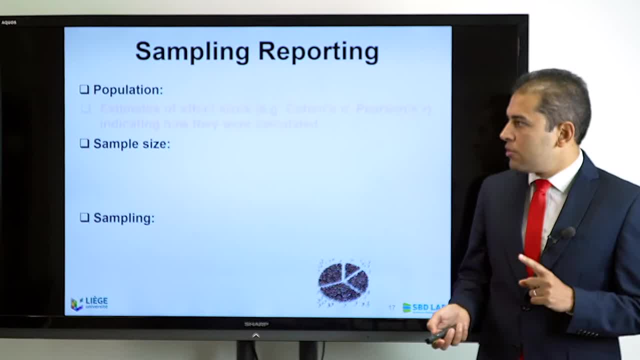 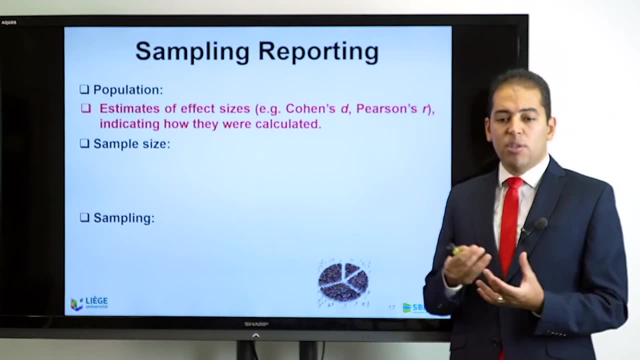 It is very important to be very conscious about reporting. So when we talk about reporting regarding population, it is the estimate of effect, of size of your population. For example, you have the Cohens D, you have the Pearsons R and you must indicate how they were used. 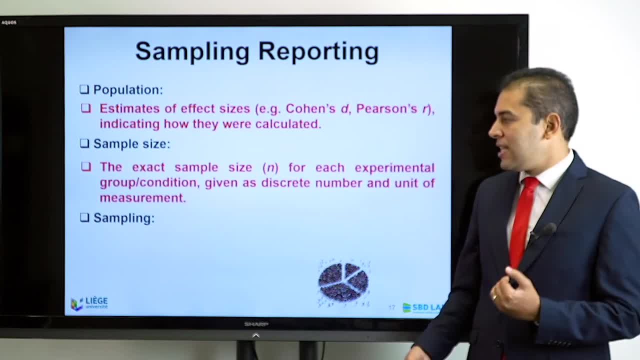 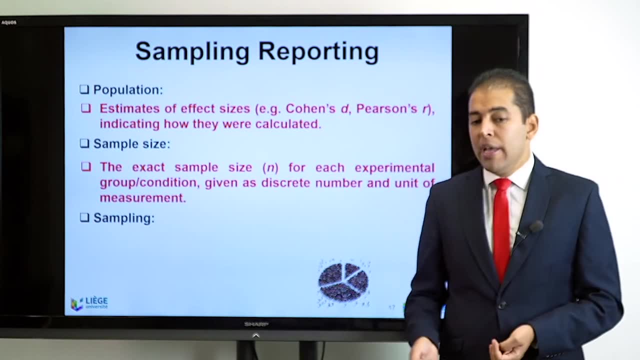 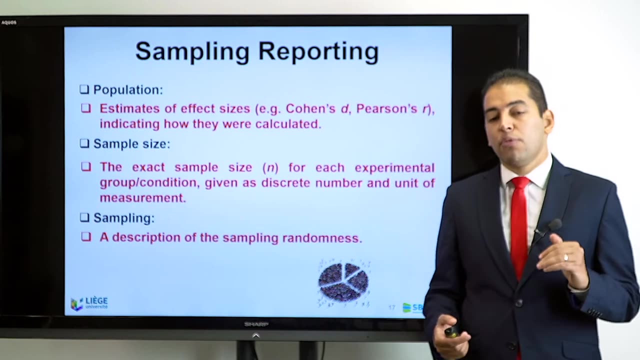 When we talk about sampling size, how to report that you have to have the exact sample size n number for each experimental group and condition given as a discrete number and unit of measurement. And when you are reporting about sampling, describe your sampling randomness. So those are the basic information that any 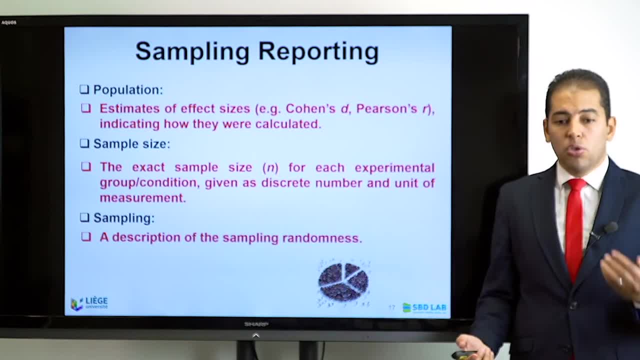 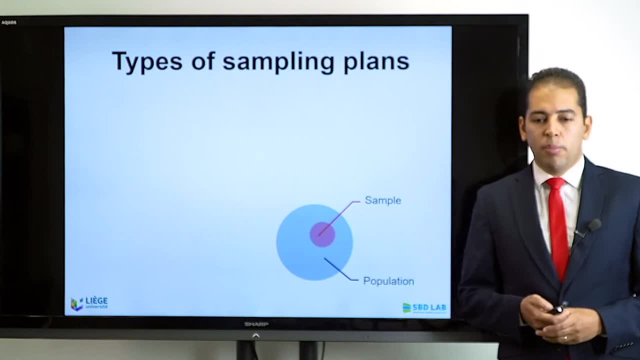 talk about and describe your sampling randomness. So those are the basic information that any description of your sample should include when you report back in a report or in a publication. Now, what are the types of sampling? There is two main types of sampling. One of them, we are not so much. 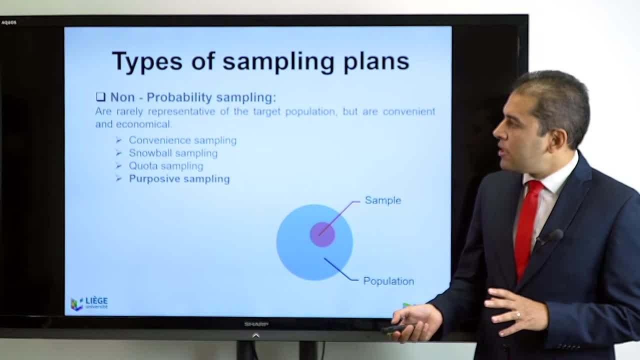 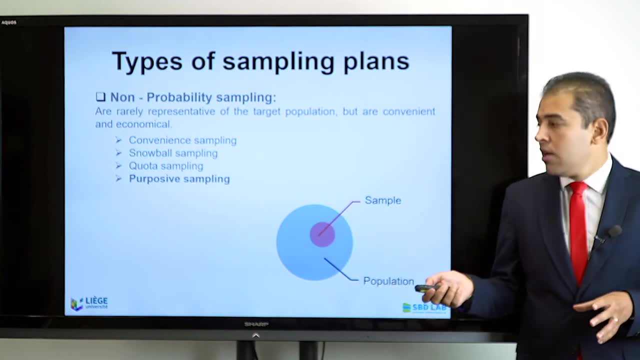 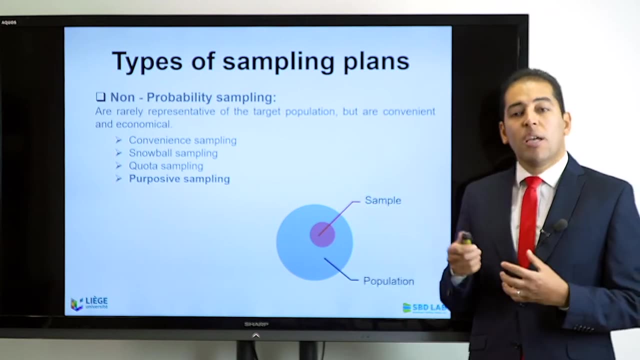 here concerned with, which is the non-probability sampling. The non-probability sampling involves the convenience sampling, snowball sampling, quota sampling and purposive sampling, and it is rarely representative of target population. So therefore, I mentioned those type of sampling in the qualitative research series before, because they are 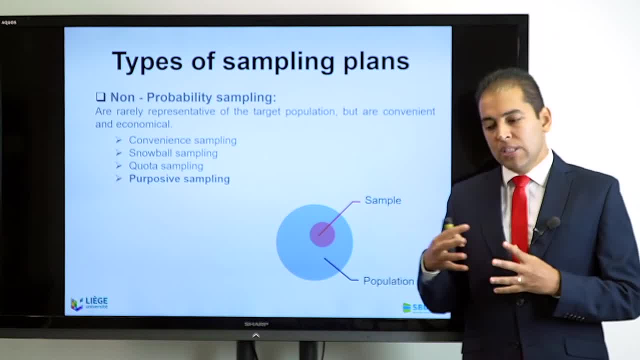 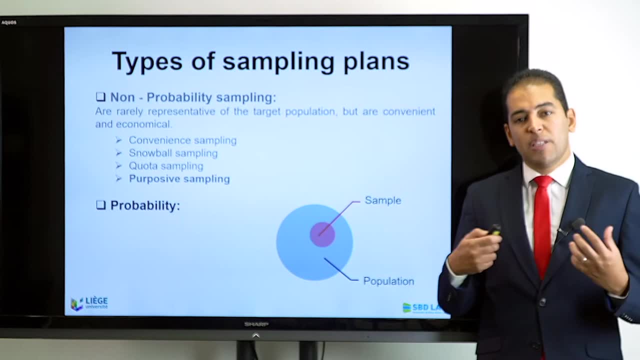 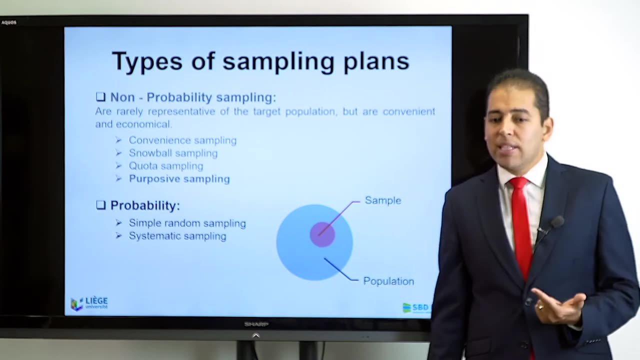 more suitable to be used in the context of qualitative research, While what is the most suitable method or sampling technique in the field of experimental research is the probability sampling, and by probability sampling I mean the simple random sampling, the systematic sampling, the stratified sampling, the 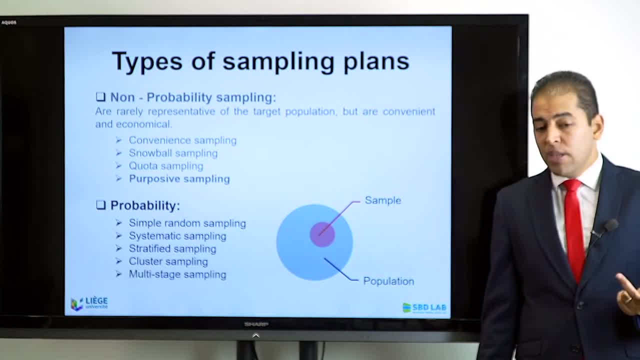 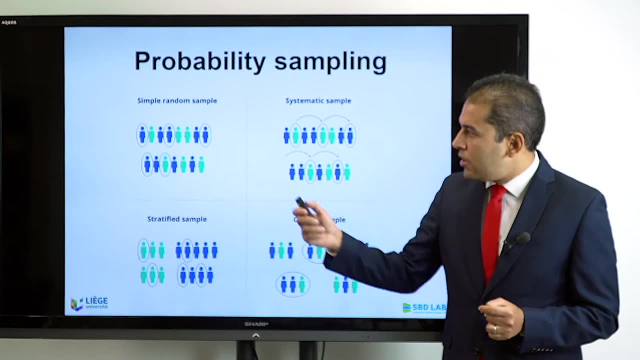 cluster sampling and the multi-stage sampling. So just have a look to give you an idea about probability sampling or the variations of difference sampling You can see here. this is some random sampling. The systematic sampling will have a kind of system that is saying I will select. 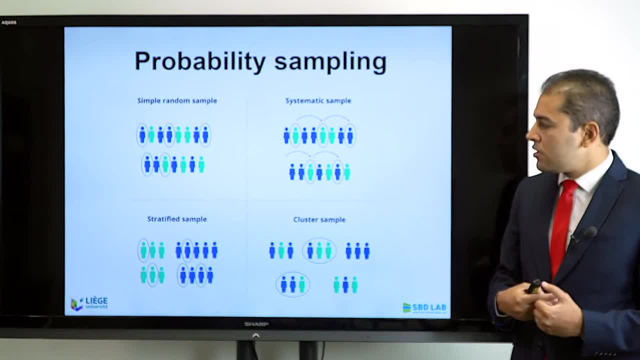 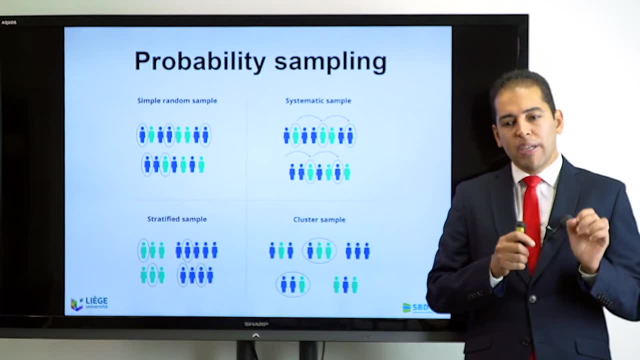 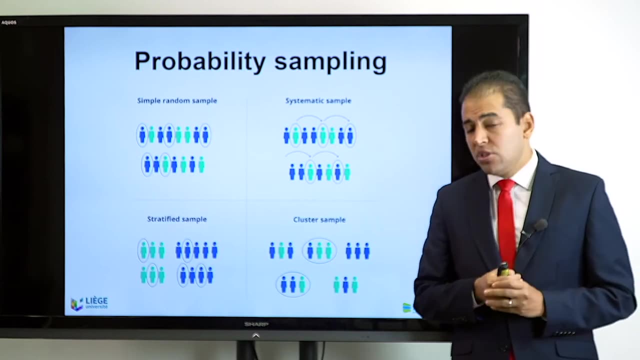 every third, every fifth, for example. subject: Stratified sampling. I try to create stratified groups and represent each of them and I will make sure that every time I'm making sure that I will take a subject based on my gender stratification example- one time a lady, one time a man, so I make sure that I'm having a 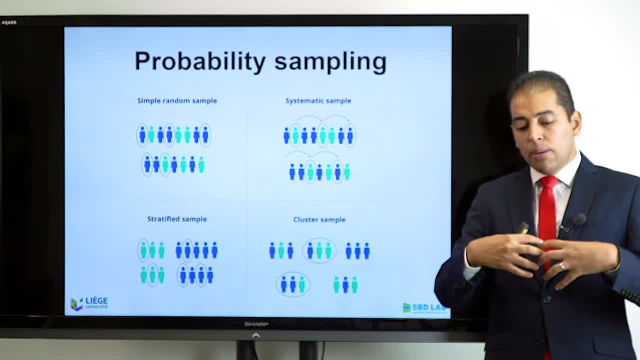 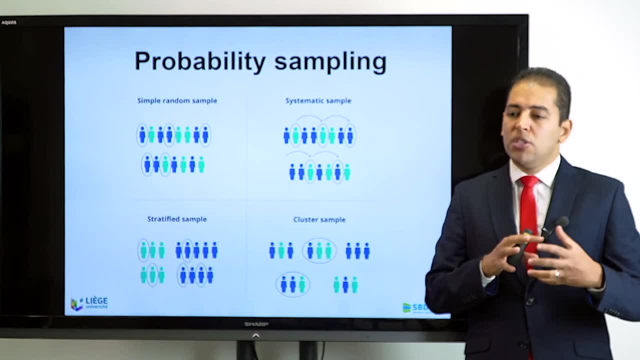 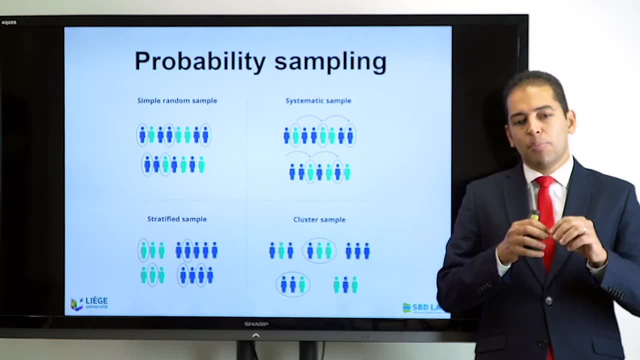 stratified sample and there is also cluster samples, and here I'm talking about groups of subjects that might have common features or conditions or settings and therefore I'm going to select based on the clustering, making sure that I'm representing different clustering, but for sure, for the stratification and for the clustering sampling I need to do an. 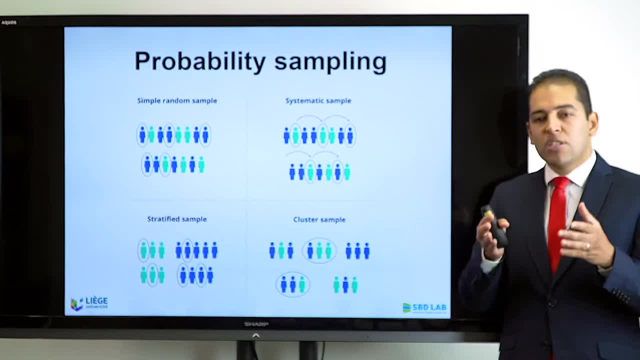 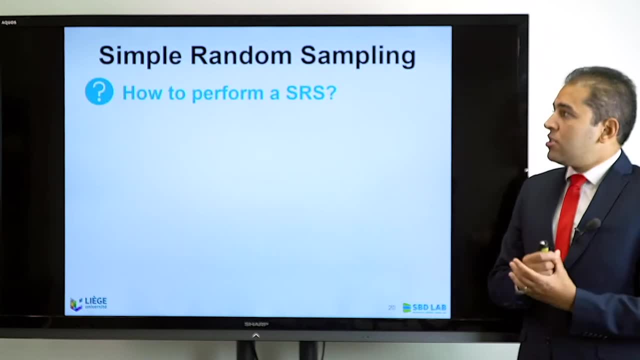 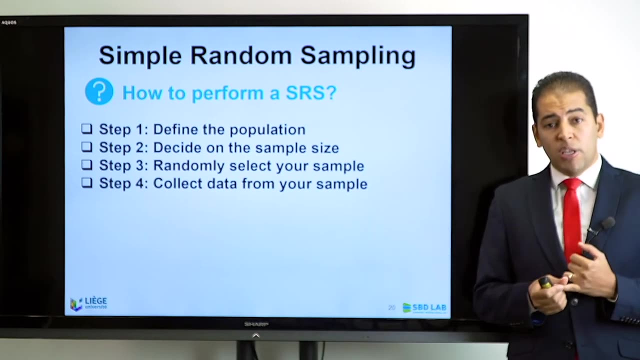 early pre-processing to make sure how I will stratify my overall sample and how I will cluster it. so these are just examples to have an idea. now let's talk about the simple random sampling. how do we perform simple random sampling? first of all, we have to define the population, then we decide the sample size and 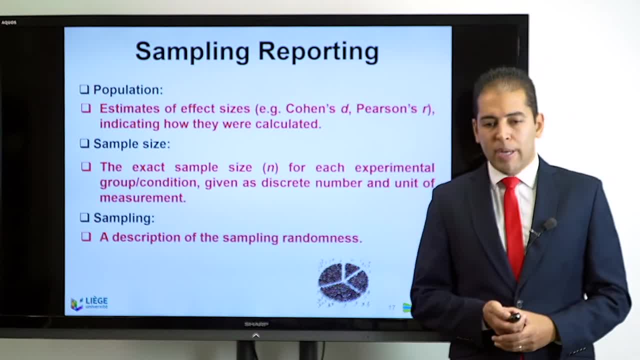 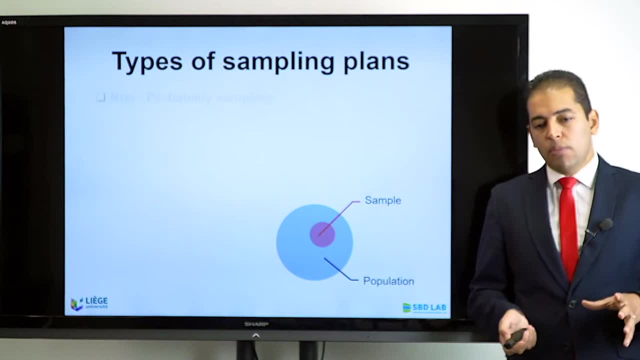 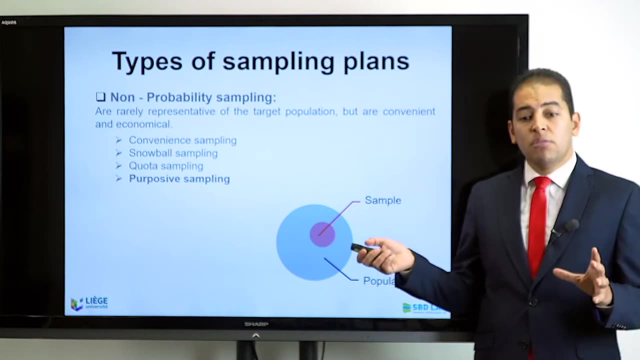 description of your sample should include: when you report back in a report or in a publication. Now, what are the types of sampling? There is two main types of sampling, One of them- we are not so much here concerned with, which is the non-probability sampling. The non-probability sampling involves the 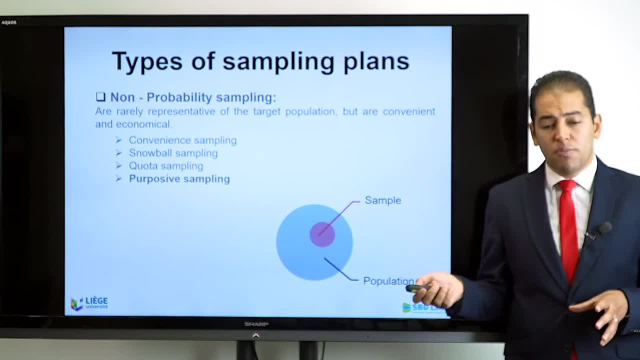 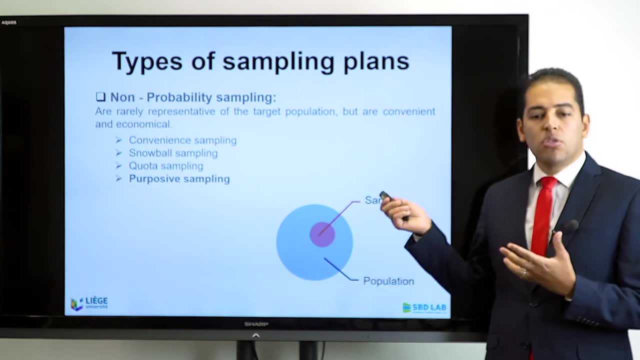 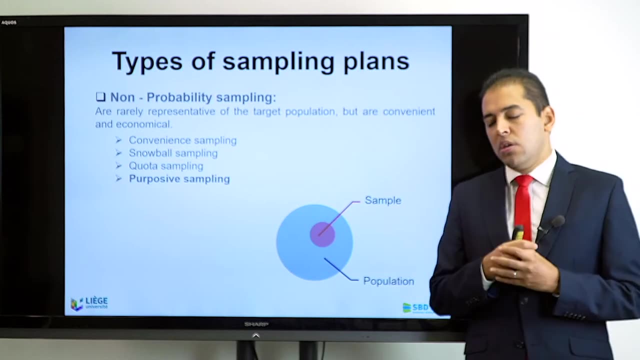 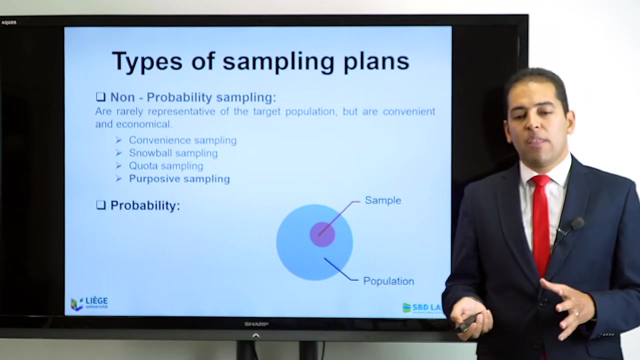 convenience sampling, snowball sampling, quota sampling and purposive sampling- and it is rarely representative of target population. So therefore, I mentioned those type of sampling in the qualitative research series before because they are more suitable to be used in the context of qualitative research, While what is the most suitable method or sampling technique in the 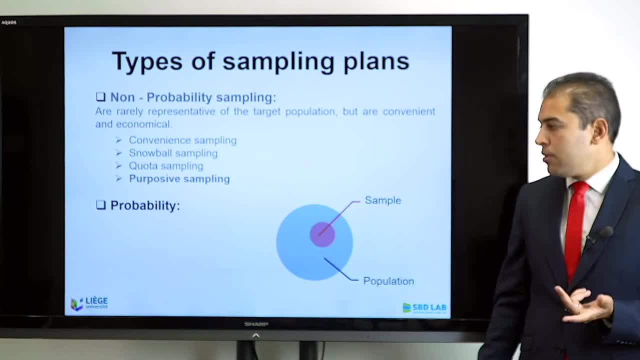 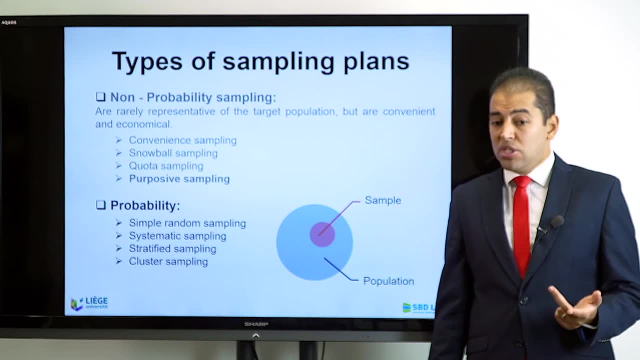 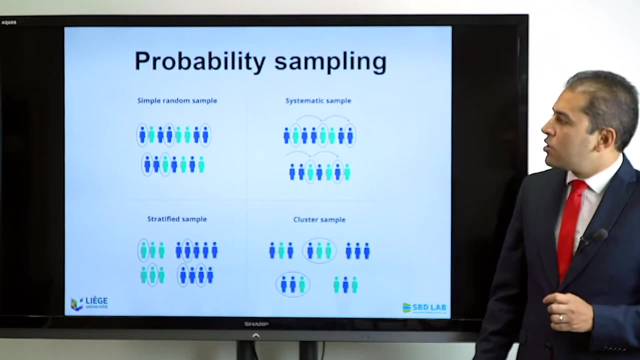 field of experimental research is the probability sampling, and by probability sampling I mean the simple random sampling, the systematic sampling, the stratified sampling, the cluster sampling and the multi-stage sampling. So just have a look to give you an idea about probability sampling or the 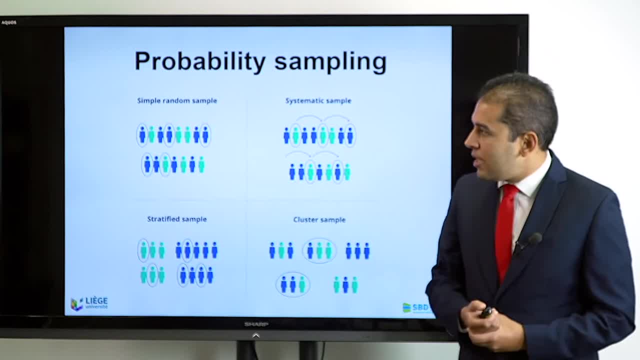 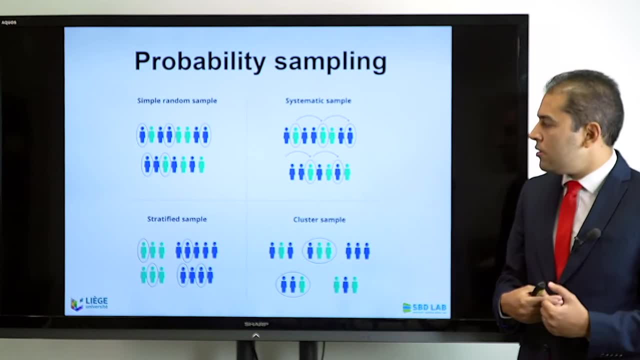 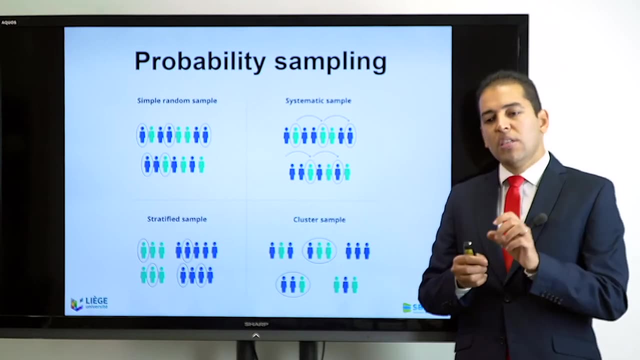 variations of different sampling. You can see here this is random sampling. The systematic sampling will have a kind of system saying I will select every third or every fifth, for example. subject: Stratified sampling. I tried to create stratified groups and represent each of them and I will make sure that every time I'm making sure. 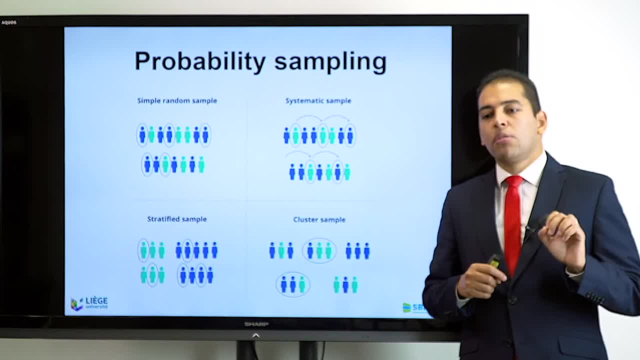 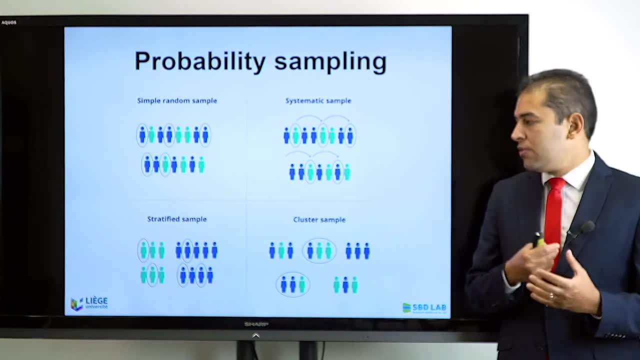 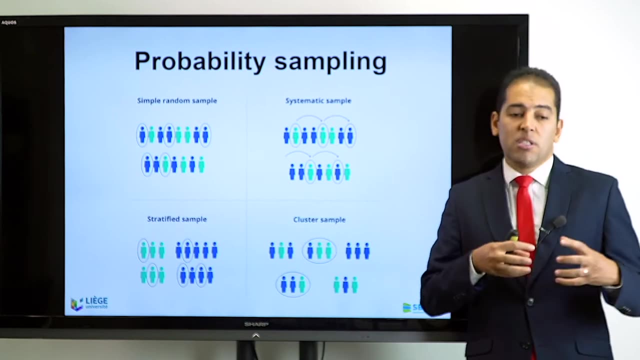 sure that I will take a subject based on my gender stratification- for example, one time a lady, one time a man- so I make sure that I am having a stratified sample and there is also cluster sample samples, and here I'm talking about groups of subjects that might have common features or conditions, or 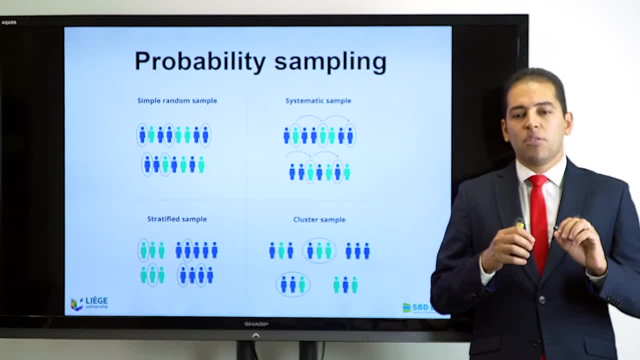 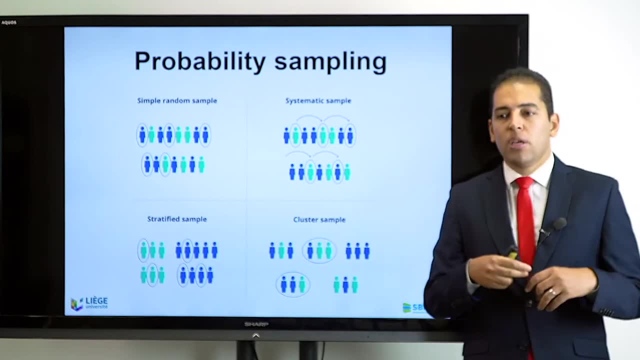 settings and therefore I'm doing, I'm going to select based on the clustering, making sure that I'm representing different clustering, but for sure for the stratification and for the clustering sampling I need to do at early pre-processing to make sure how I will stratify my overall sample and how. 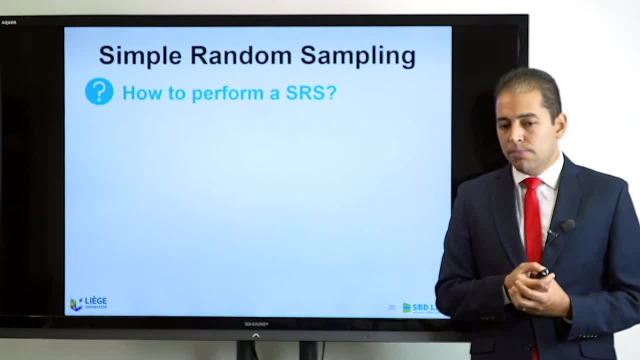 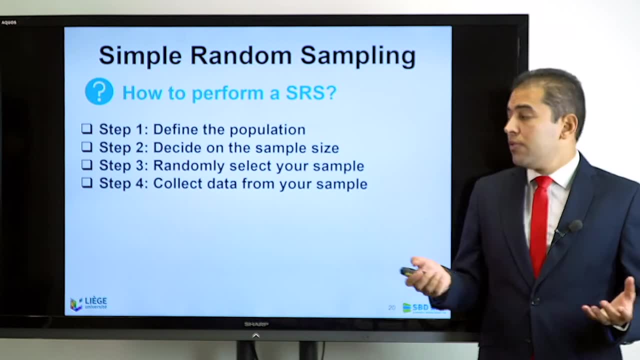 I will cluster it. so these are just examples to have an idea. now let's talk about the simple random sampling. how do we perform simple random sampling? first of all, we have to define the population, then we decide the sample size and finally, and so do, we start to randomly select the 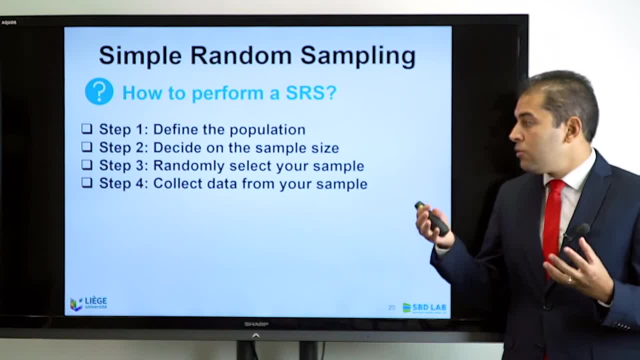 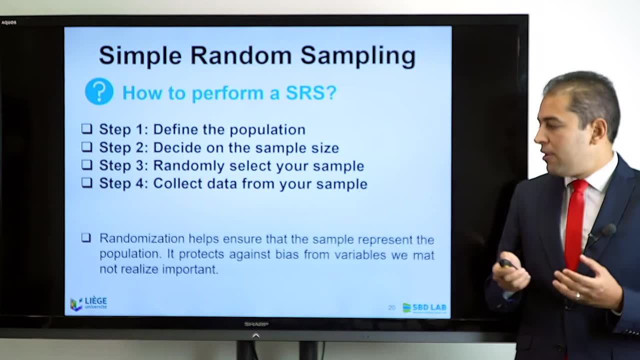 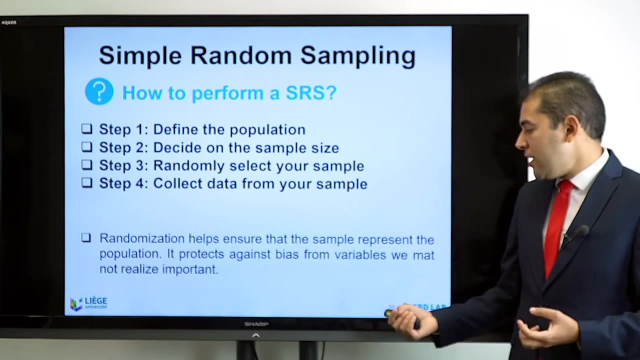 finally, and certainly, we start to randomly select the sample and we, after that, can finally start with step 4, which is the collecting of the data from my sample. so you have to keep into account that randomization helps ensuring that the sample represents the population and it protects against bias from variables. we 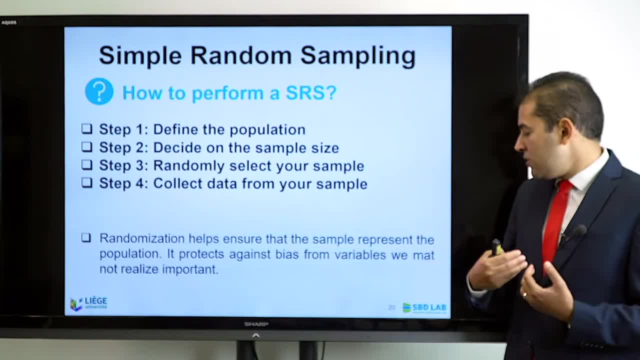 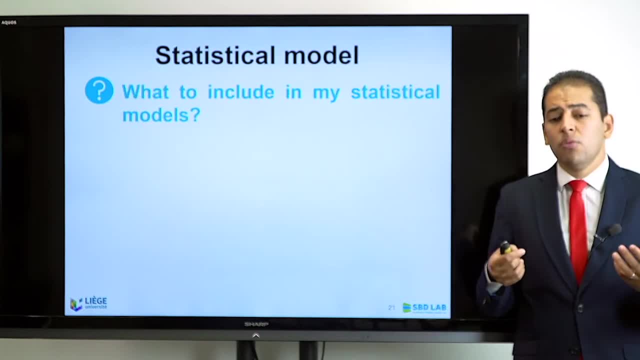 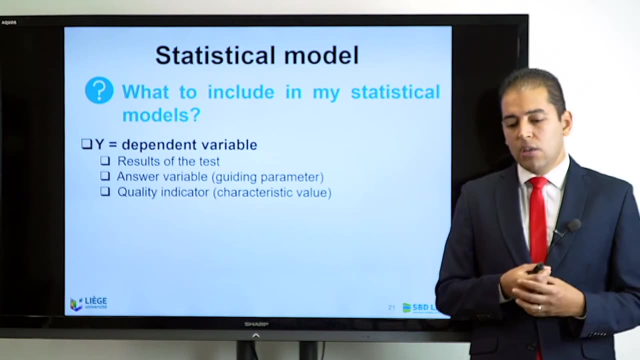 might not realize important or we might not think that they are important. so here it comes, the importance of randomization or random sampling. now, what, what, what to include in my statistical models when I am starting my statistical analysis for my experiments? first of all, you have to include the independent variable. so the independent 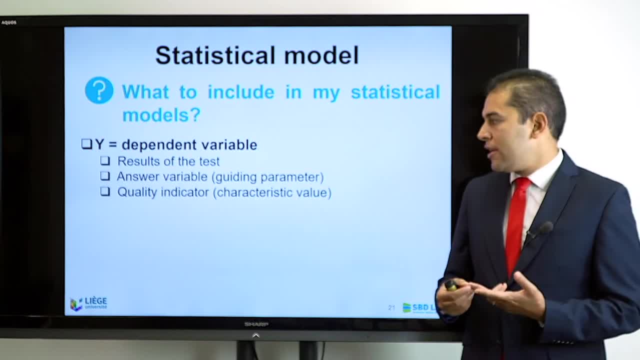 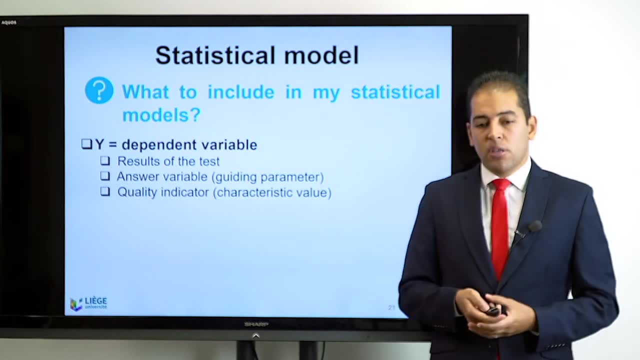 variable will look at the results of the test. it represents the answer variable or the guiding parameter of your work and it is a quality indicator, that characteristic value for your work. the second aspect that I have included in my statistical model when I'm starting to think about how to design my experiment: 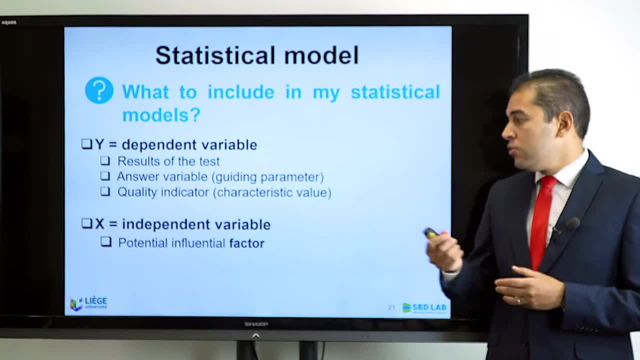 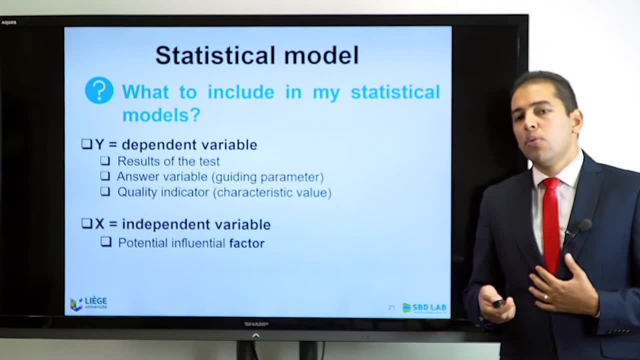 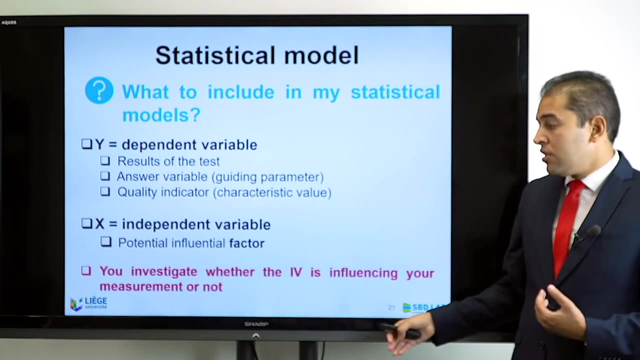 and how to design my statistical framework. I have to define my independent variable, which is, in this sense, the potential influential factor, and always when you are reporting this information in a paper or in a report, you have to investigate whether the independent variable is influencing your measurement or not, and in this sense it can be one variable or multiple values. 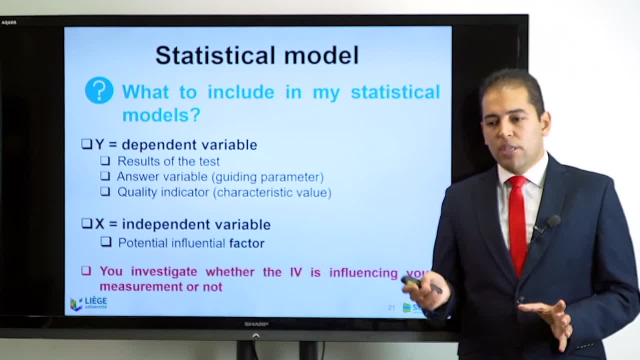 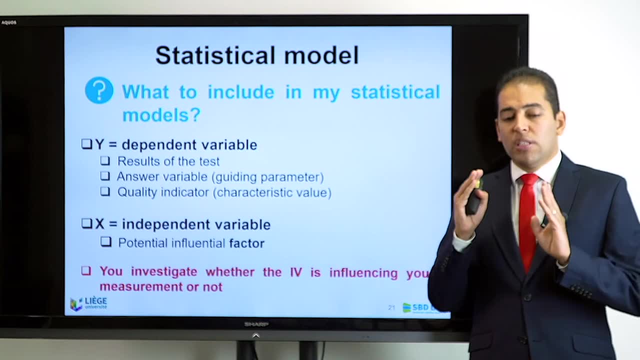 now, if you know about this basic information. I talked about sampling and I talked about the basic statistical models. that has independent variable or it has a dependent variable. you can have several of them, but so far let's start with the most simple. then I have to move to the next step, which is the sampling. 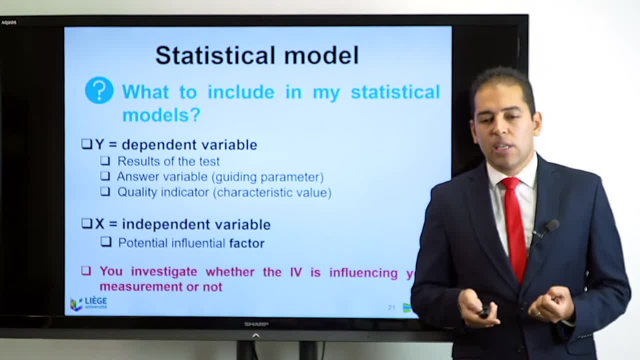 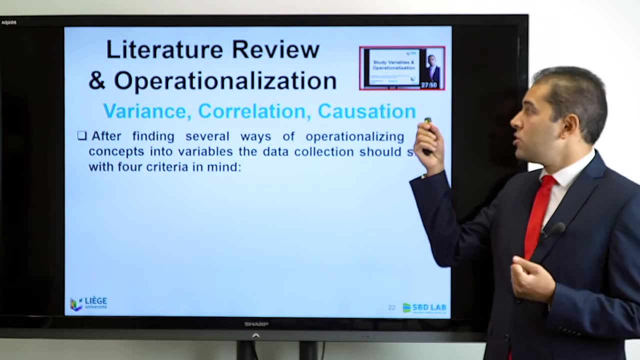 so let's move to the next step: how to start, how to start the story of statistical analysis? well, statistical analysis start with the literature review and the operationalization, and I strongly advise you to watch the video on study variables and operationalization that was prepared previously, because this video will help you to understand exactly how to. 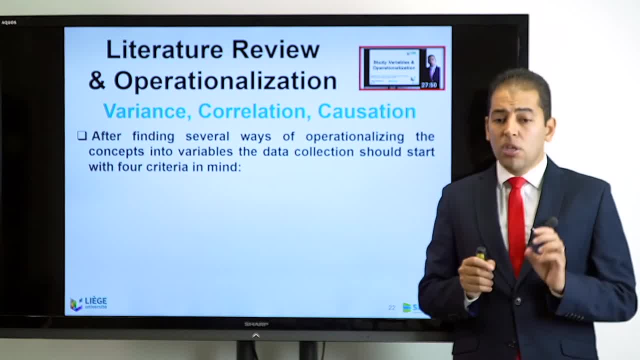 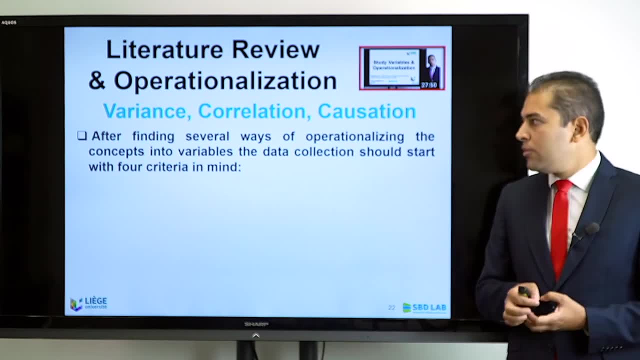 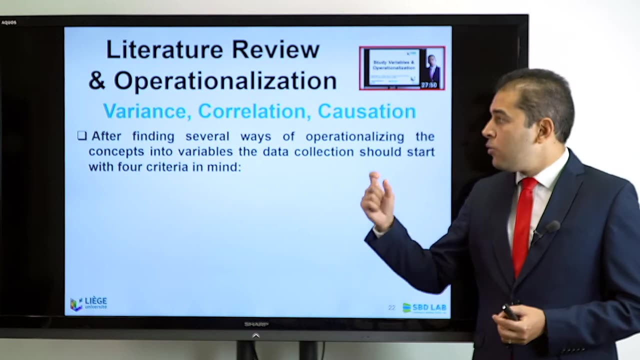 operationalize and select the variables of your study and once this is done, you can go with the next step. actually, when we do statistic and analysis, we are trying through our experiment to trace any variance as an influence of introducing a treatment we are looking to establish. we never know, maybe yes, maybe no. a correlation can be positive, it can be. 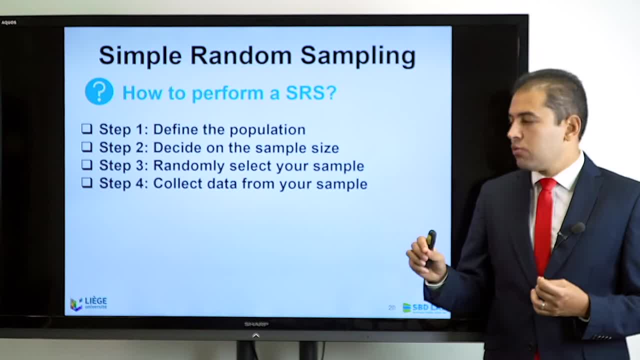 sampling G I and G f and the binary and Tableau of 1 to T is the most modern sample and we after that can finally start with step 4, which is the collecting of the data from my sample. So you have to keep into account that. 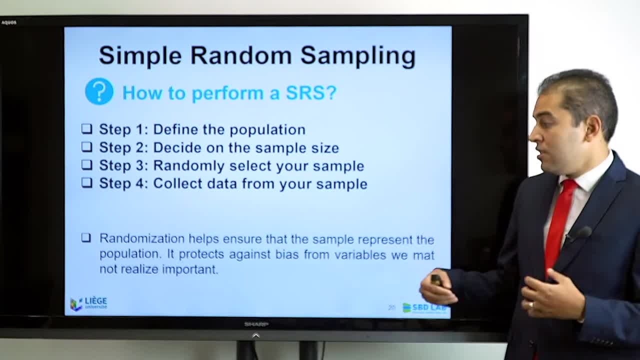 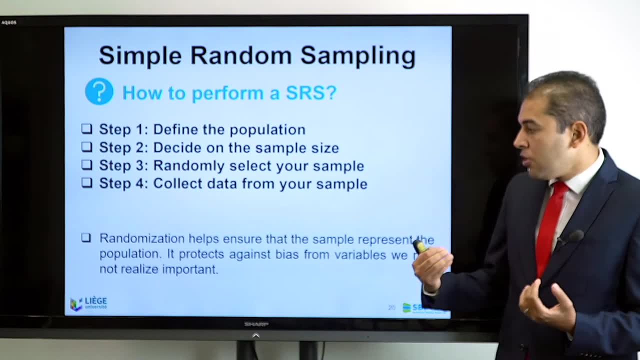 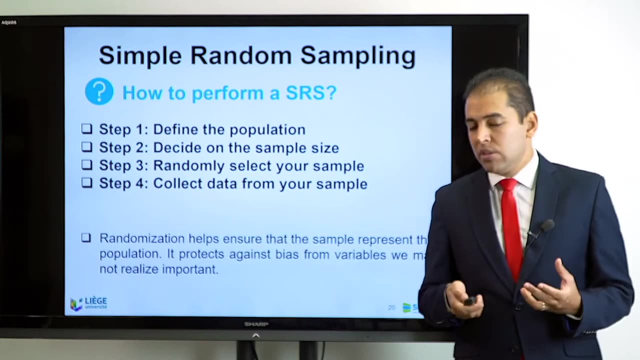 randomization helps ensuring that the sample represents the population and it protects against bias from variables we might not realize important or we might not think that they are important. So here it comes, the importance of randomization or random sampling. Now what to include in my 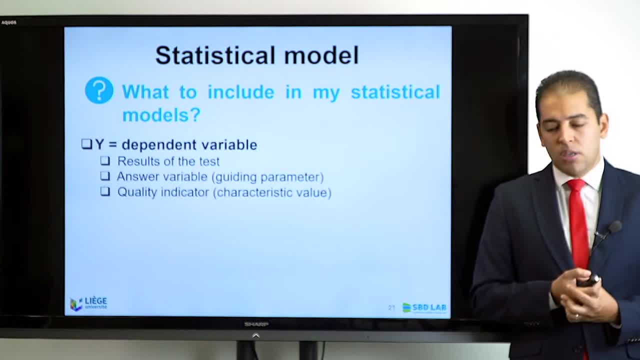 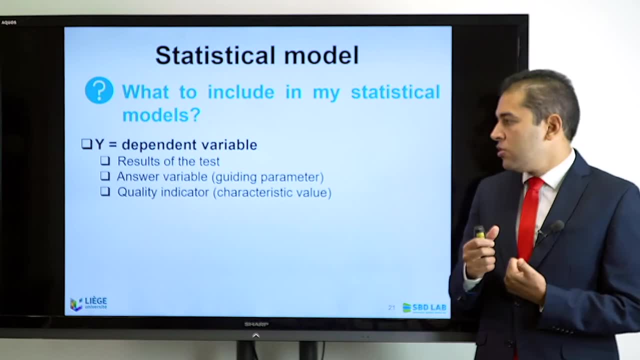 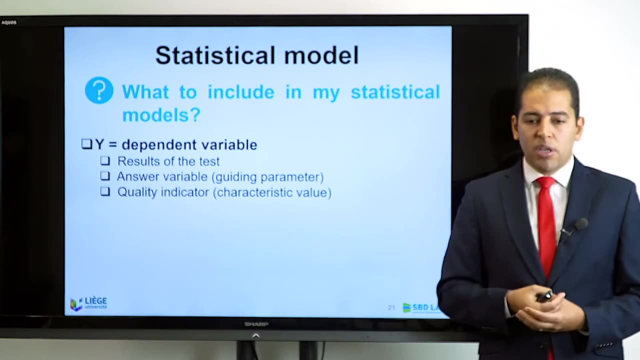 statistical models when I am starting my statistical analysis for my experiment. First of all you have to include the independent variable. So the independent variable will look at the results of the test. It represents the answer variable or the guiding parameter of your work, and it is a quality. 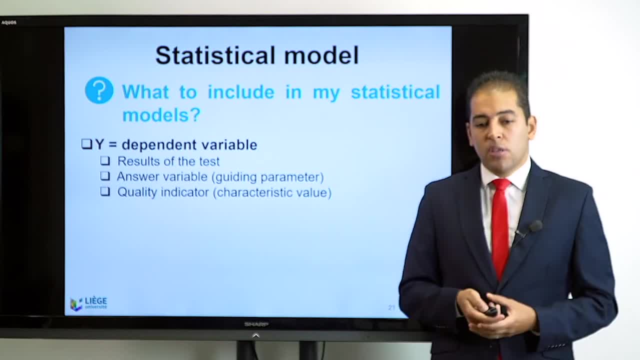 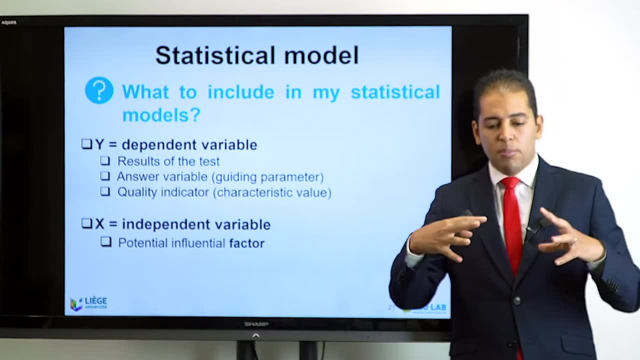 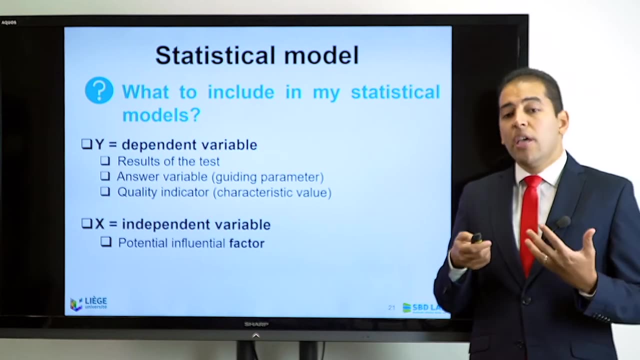 indicator with a characteristic value for your work. The second aspect that I have included in my statistical model: when I'm starting to think about how to design my experiment and how to design my statistical framework, I have to define my independent variable, which is, in this sense, the potential influential factor. and always when you 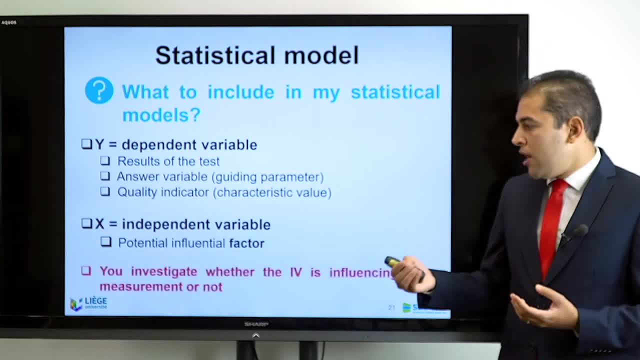 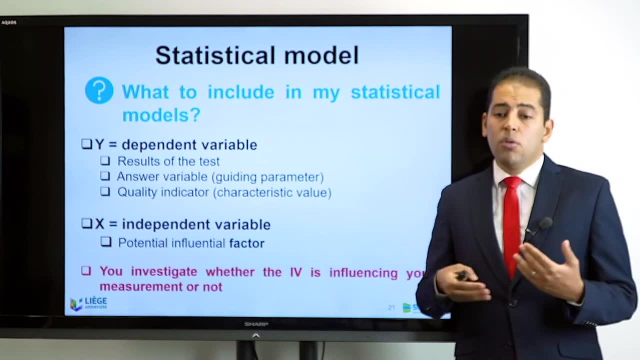 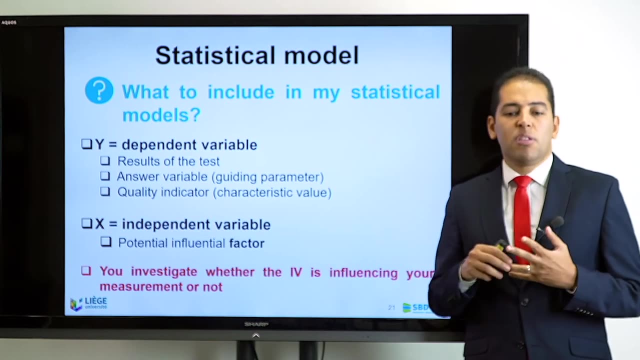 are reporting this information in a paper or in a report, you have to investigate whether the independent variable is influencing your measurement or not, and in this sense, it can be one variable or multiple values. Now, if you know about this basic information- I talked about sampling and I talked about the basic statistical models- that has independent 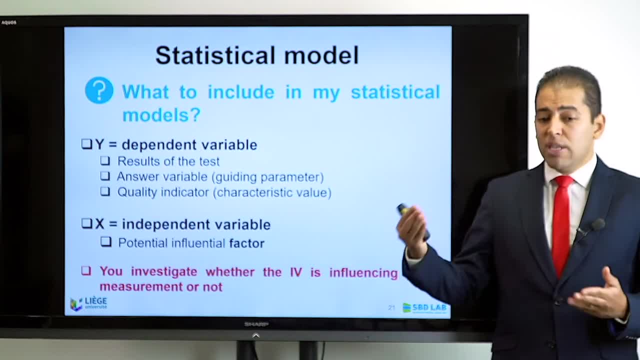 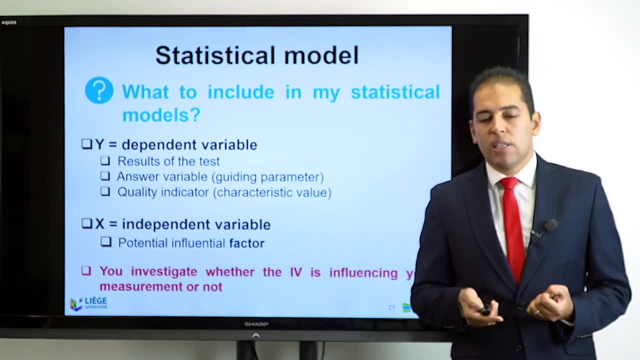 variable or it has a dependent variable. You can have several of them, but so far let's start with the most simple. Then I have to move to the next step: How to start, How to start the story of statistical analysis? Well, statistical analysis starts with the literature review and operationalization, and I 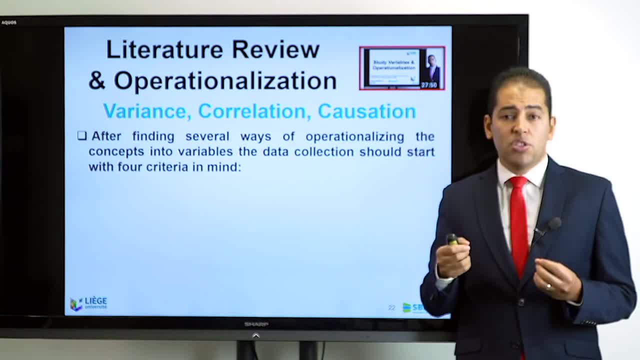 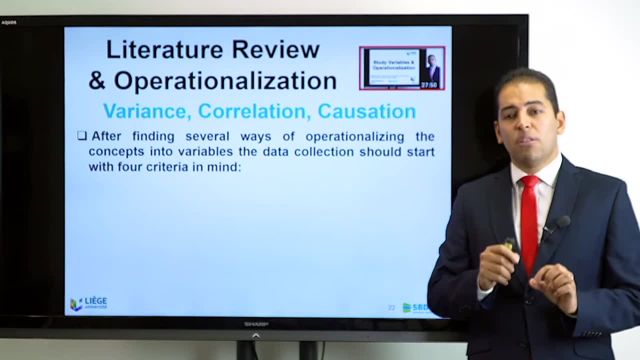 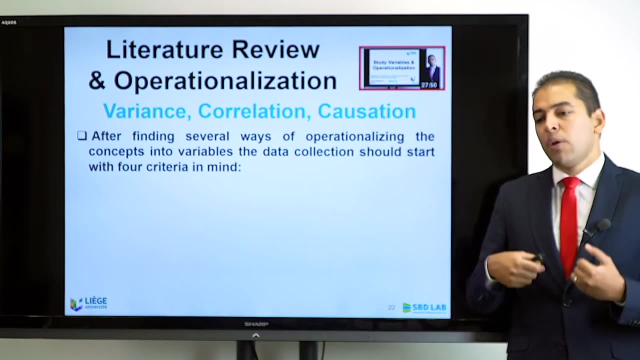 strongly advise you to watch the video on study variables and operationalization that was prepared previously, because this video will help you to understand exactly how to operate and how to operationalize and select the variables of your study, and once this is done, you can go with the next step. Actually, when we do statistical analysis, 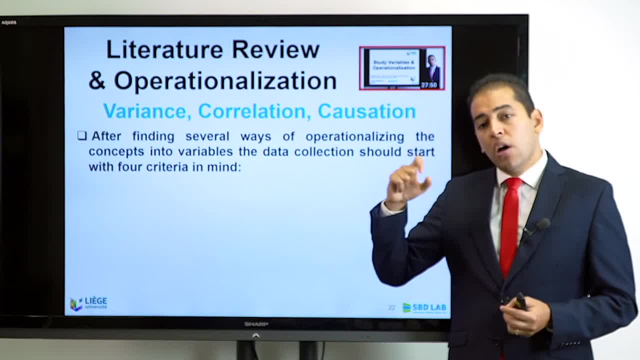 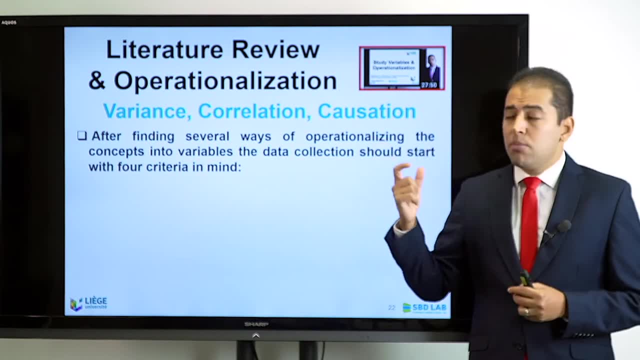 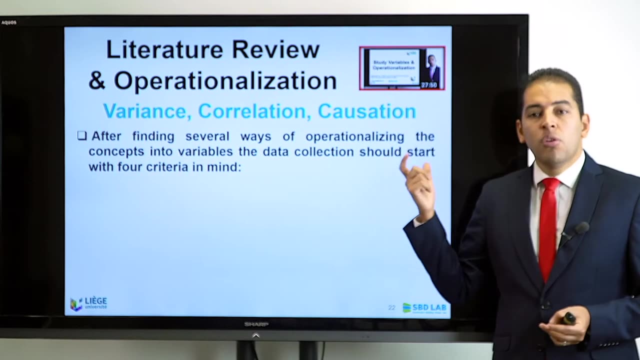 we are trying, through our experiment, to trace any variance as an influence of introducing a treatment We are looking to establish. we never know, maybe yes, maybe no, a correlation can be positive, it can be negative, maybe there is no correlation and, if possible, we are trying to establish a causation. It doesn't work. so 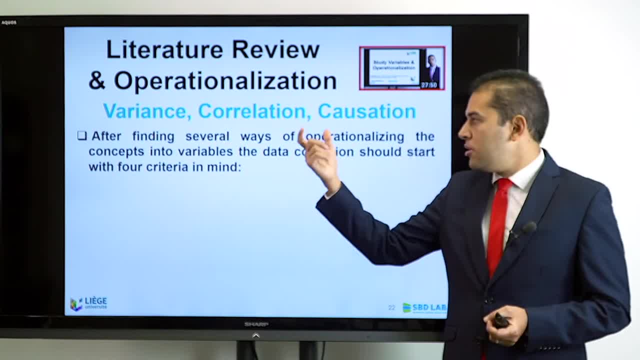 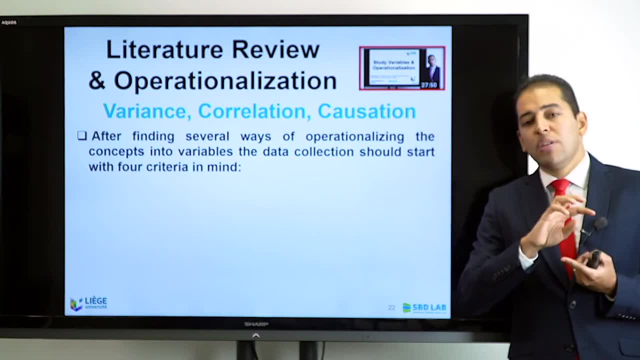 easy, like I'm saying every time. sometimes it stops with variance, maybe it stops with correlation, but that's what we are seeking when we do statistics. We are looking at variance as an as a consequence of introducing an intervention or a treatment, and if this variance is well documented, we try to 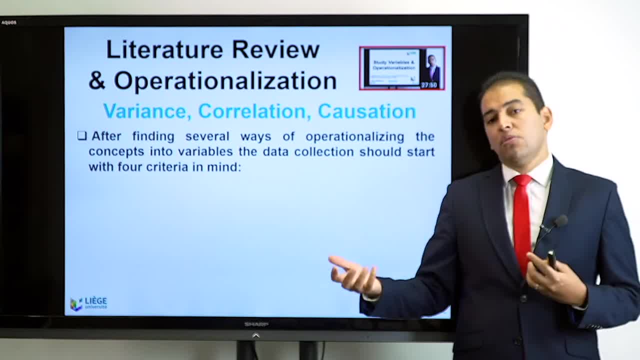 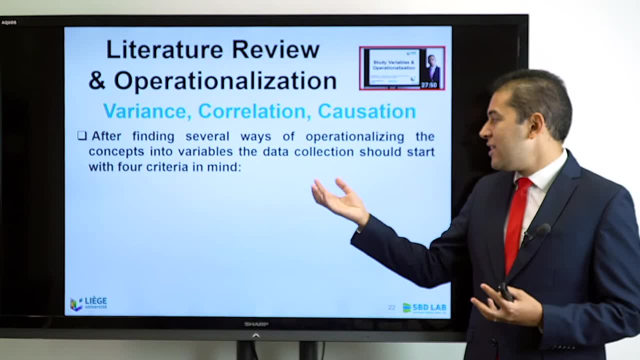 check if this variant is correlated. and if it's correlated, we try to check if there is a causality behind it or not. So, after finding several ways of operationalizing the concept into variables of your research, the data collection should start with four criteria in mind. 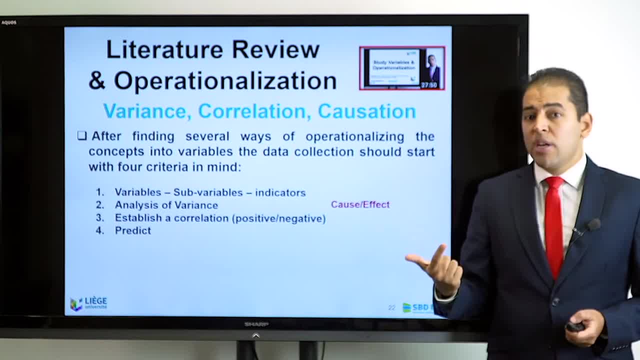 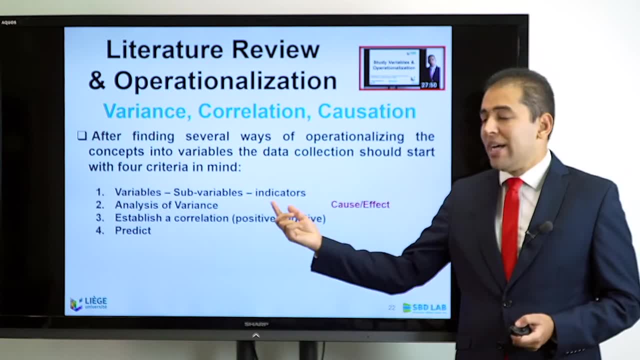 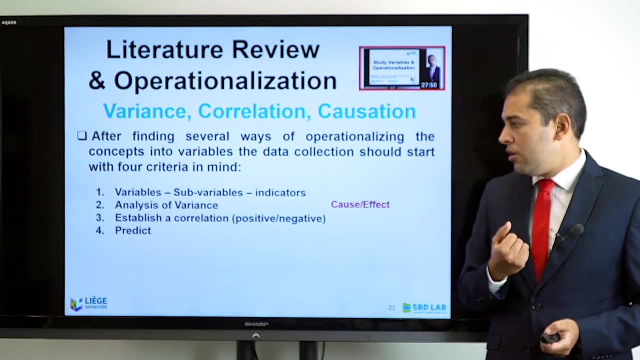 You have to look at your variables. what are the sub variables that you are investigating and what are the indicators that you will use to measure and quantify each variable? You have to have analysis of variance for the influence of introducing your independent variable on the dependent variable. You have to 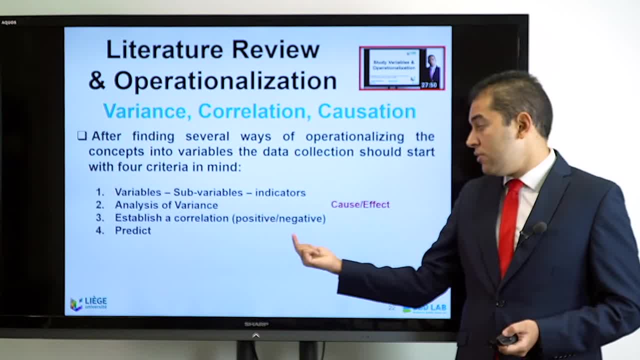 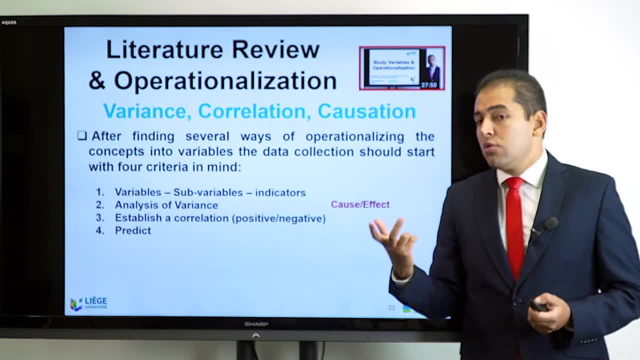 look at establishing a correlation if possible, whether it's positive or negative. but you have to be very attentive to that. You cannot establish a correlation without proving that there is variance. so once there is no variance proved, you cannot move to step number three. and if step 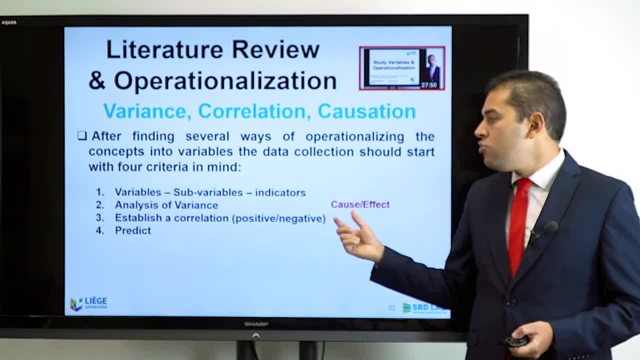 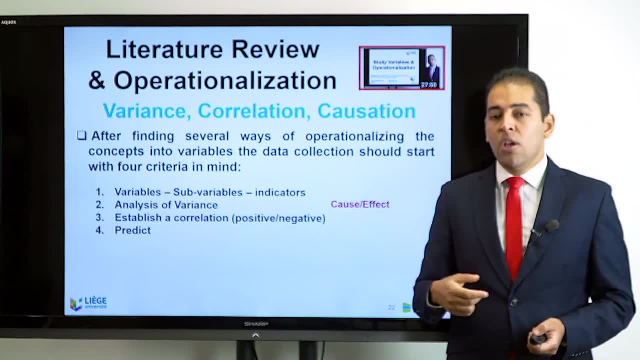 number three is established and you have a correlation, you might be able to investigate causality, the cause effect and finally, you can predict, which is something very powerful we look at when we do research. However, the prediction part is always considered in the modeling side, which is the research. 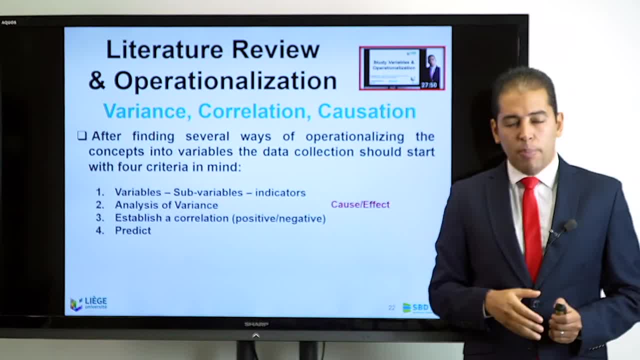 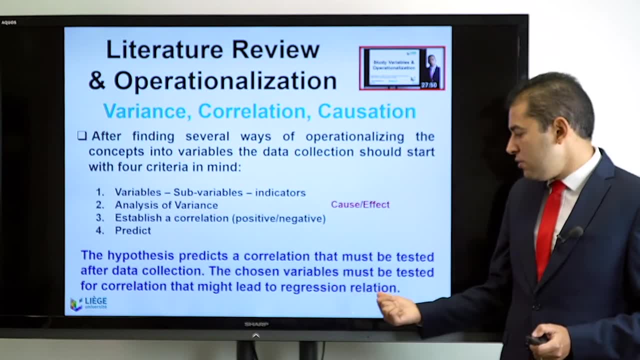 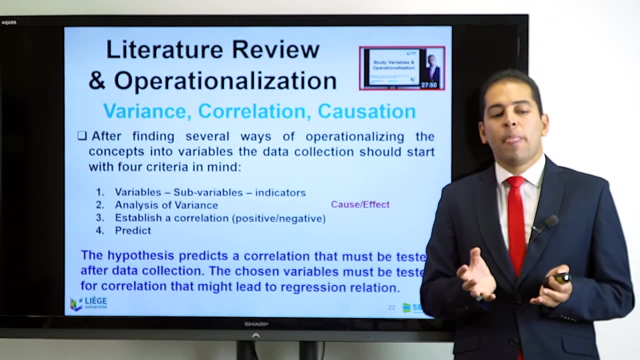 methodology for that I will have a playlist upon in the future. Now, the hypothesis predicts a correlation that must be tested after data collection and the chosen variables must be tested for correlation that might lead to regression relation. So this is the overall beginning point when I start to design my experiment, and in parallel, 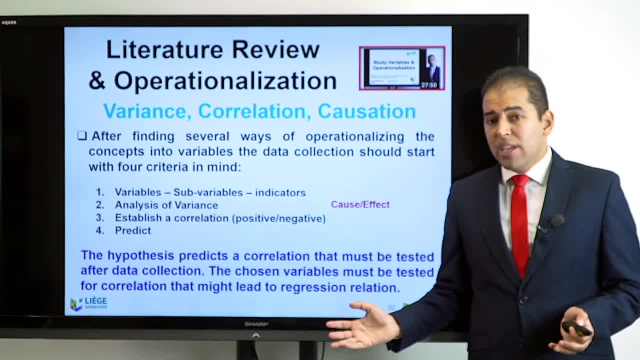 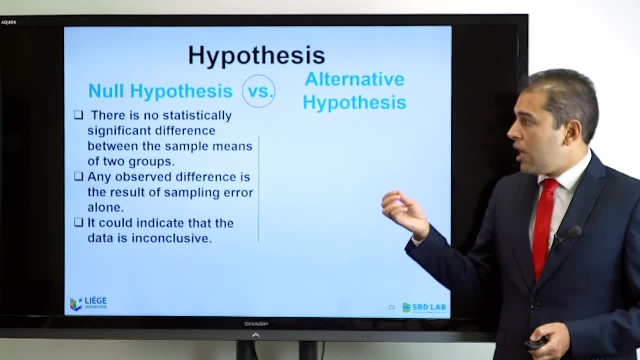 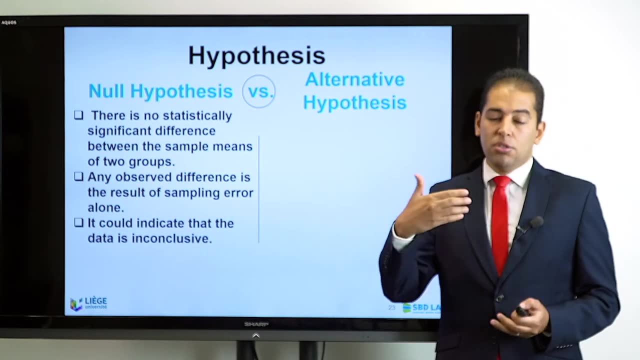 design my statistical framework. Now, talking about hypothesis, I need to be aware about the null hypothesis versus the alternative hypothesis. What is the null hypothesis? The null hypothesis: in fact, there is no statistical significant difference between the sample means of two groups. So I introduced my 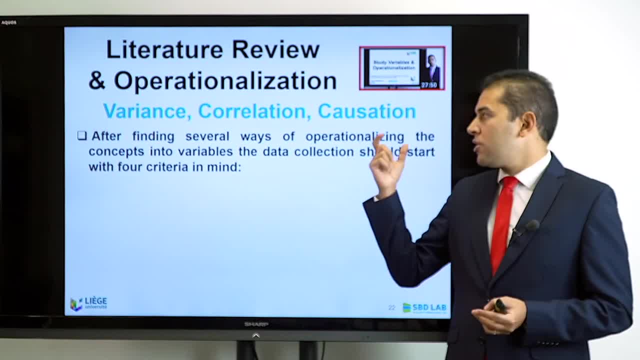 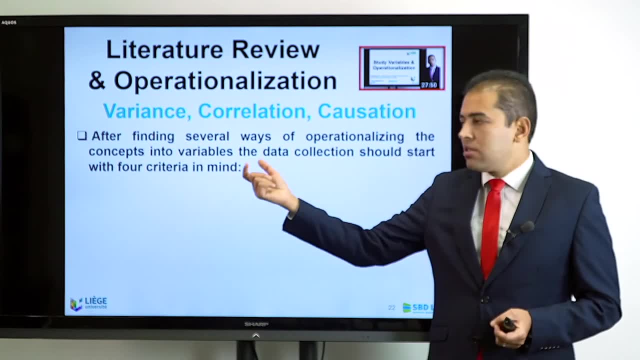 negative. maybe there is no correlation and, if possible, we are trying to establish a causation. it doesn't work so easy, like I'm saying every time, sometimes it stops with variance, maybe it stops with correlation, but that's what we are seeking when we do statistics: we are looking at variance as an, as a 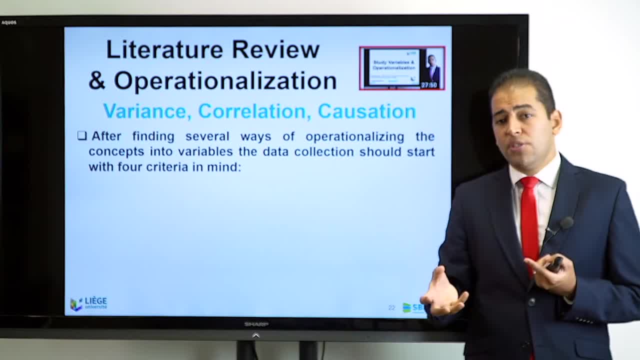 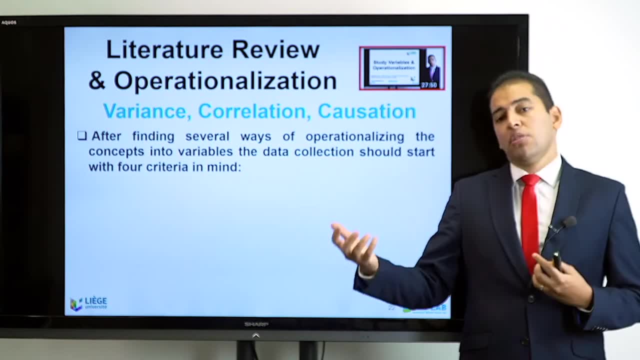 consequence of introducing an intervention or a treatment, and if this variance is well documented, we try to check if this variant is correlated. and if it's correlated, we try to check if there is a causality behind it or not. so, after finding several ways of operationalizing the concept into variables of your 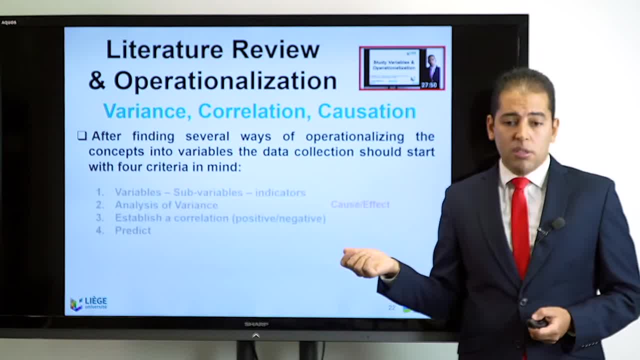 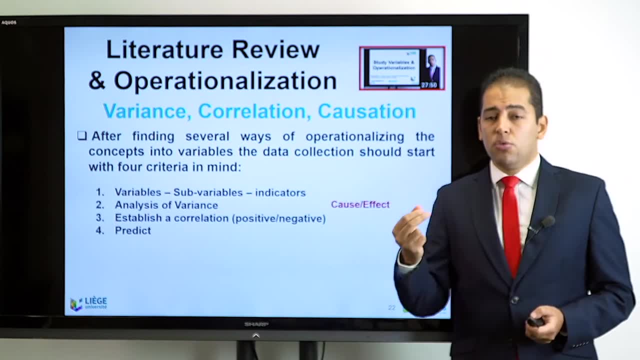 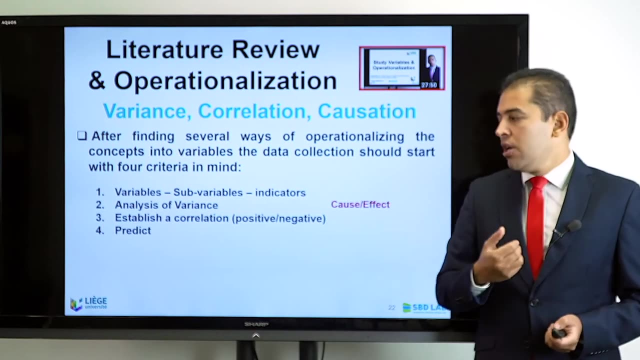 research, the data collection, should start with four criteria in mind. you have to look at your variables. what are the sub variables that you are investigating and what are the indicators that you will use to measure and quantify each variable? you have to have an analysis of variance for the influence of introducing your independent variable on the dependent. 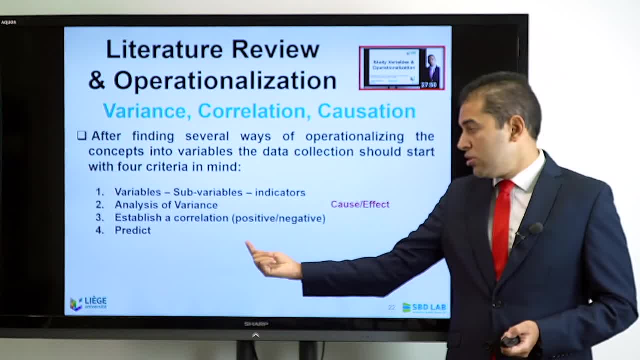 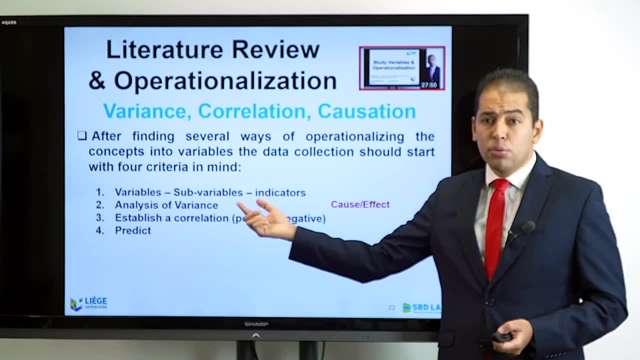 variable, you have to look at establishing a correlation, if possible, whether it's positive or negative, but at it you have to be very attentive to that. you cannot establish a correlation without proving that there is variance. so once there is no variance proved, you cannot move to step number three. and if 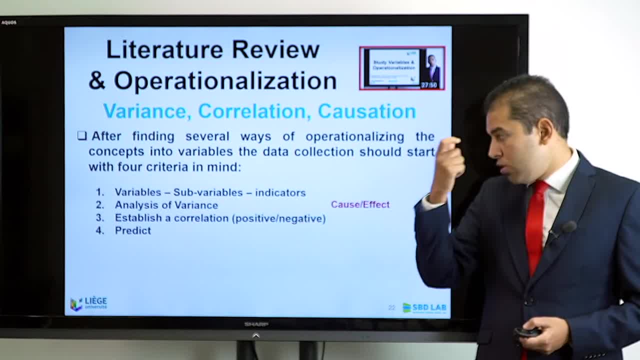 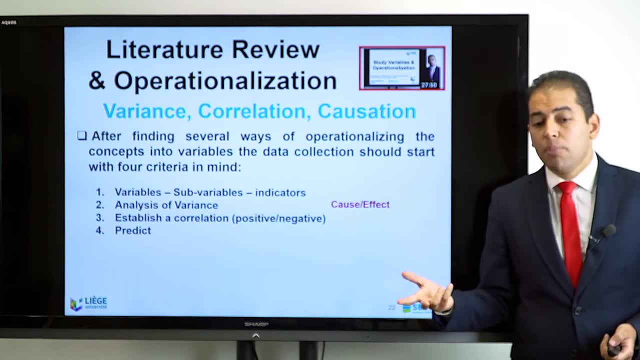 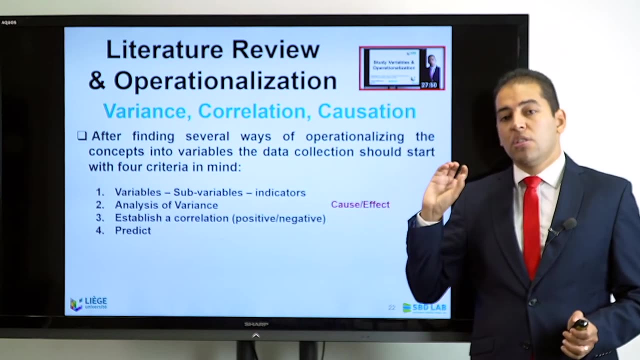 step number three is established and you have a correlation. you might be able to investigate causality, the cause-effect, and finally you can predict, which is something very powerful we look at when we do research. However, the prediction part is always considered in the modeling side, which is the research methodology. for that I will have a 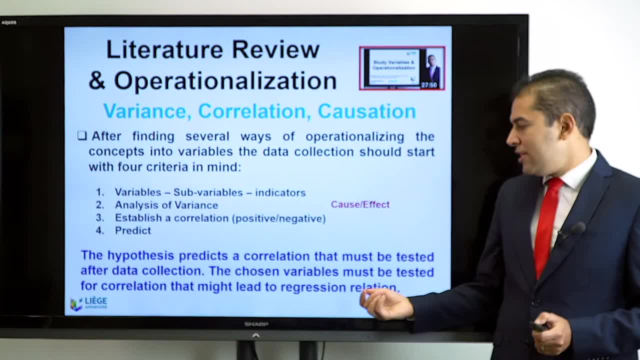 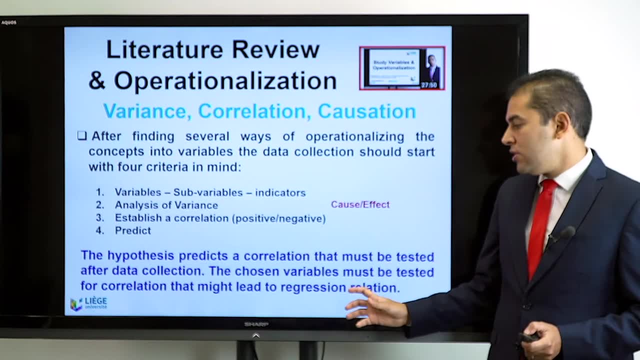 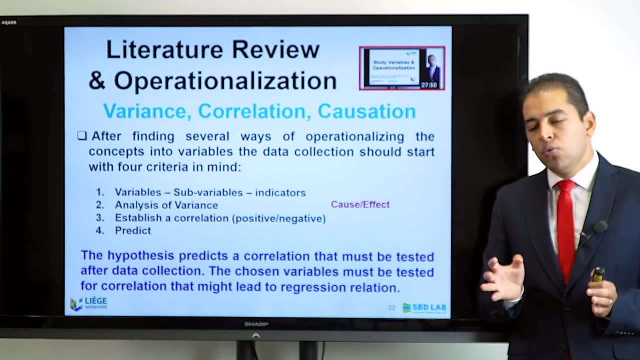 playlist upon in the future. Now, the hypothesis predicts a correlation that must be tested after data collection, and the chosen variables must be tested for correlation that might lead to regression relation. So this is the overall beginning point when I start to design my experiment, and in parallel, 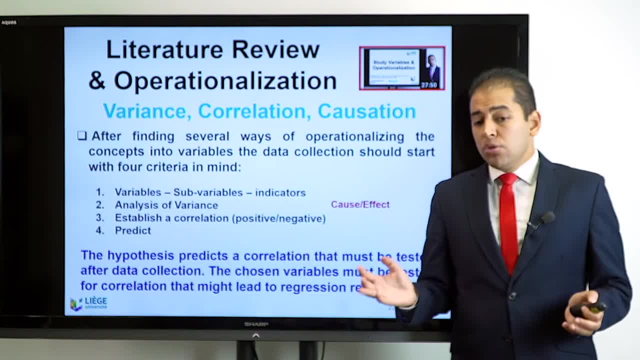 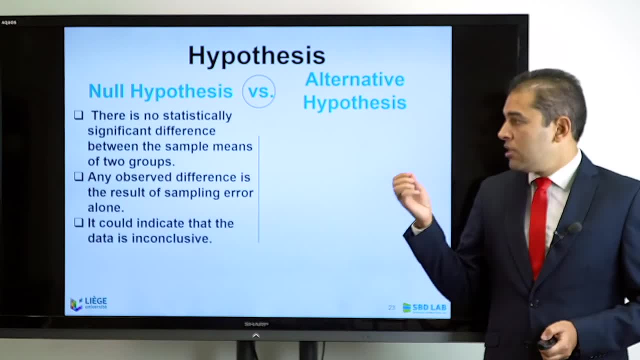 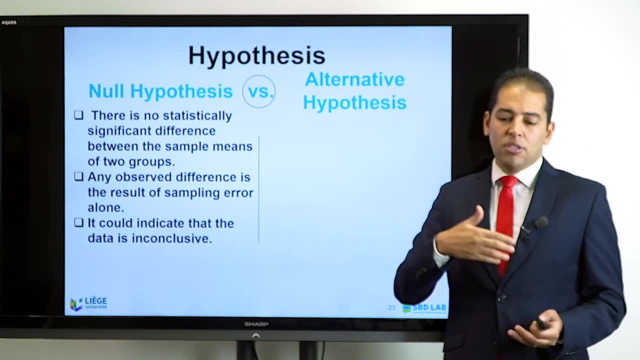 design my statistical framework. Now, talking about hypothesis, I need to be aware about the null hypothesis versus the alternative hypothesis. What is the null hypothesis? The null hypothesis: in fact, there is no statistical significant difference between the sample means of two groups. So I introduced my 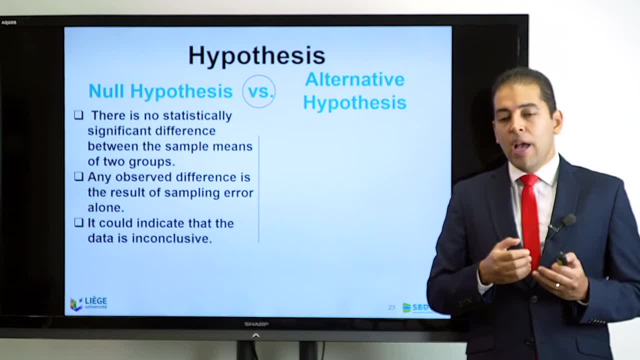 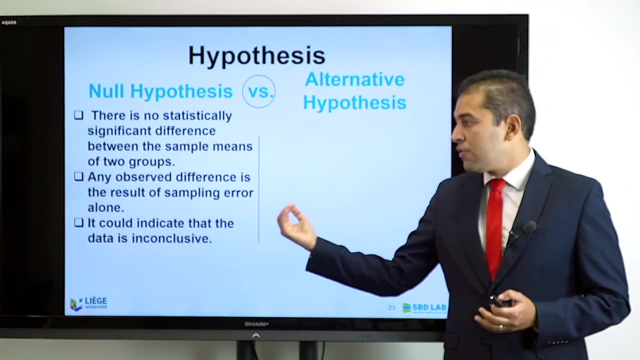 intervention or my treatment to my sample and I found that there is no variance. So here I say there is no difference between the sample, the baseline sample, and alternative or sample number one, which includes the intervention. Any observed difference is the result of sampling error alone in this case. most probably This can be another. 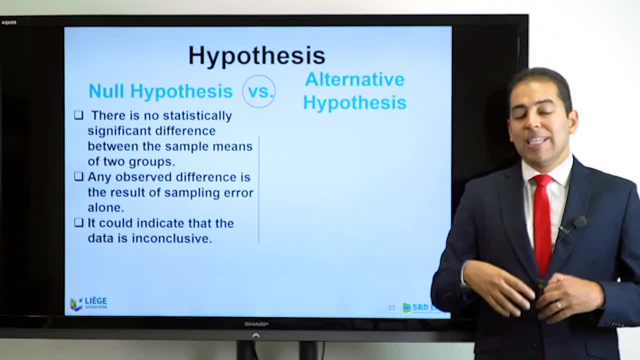 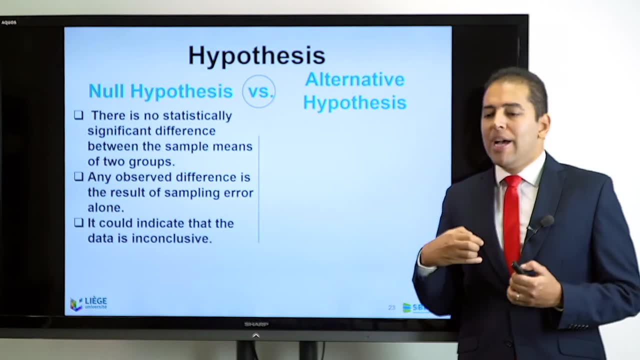 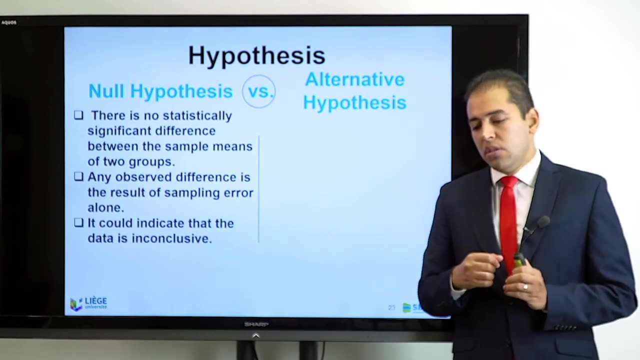 interpretation or it could be indicating that the data is inconclusive. Those are the three options. if I cannot detect variance, when I do my experiment and I introduce my experiment, My intervention, I cannot find a variance between the base case condition without intervention and the alternative condition with intervention. Now, if you 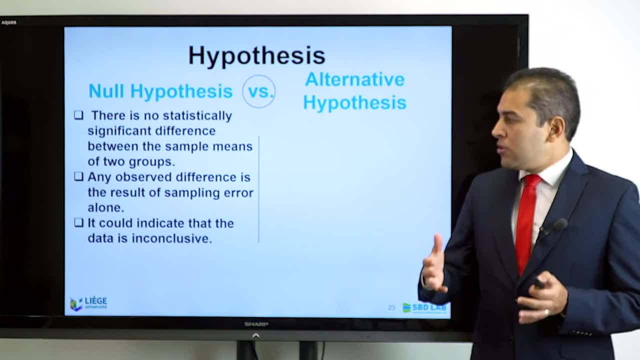 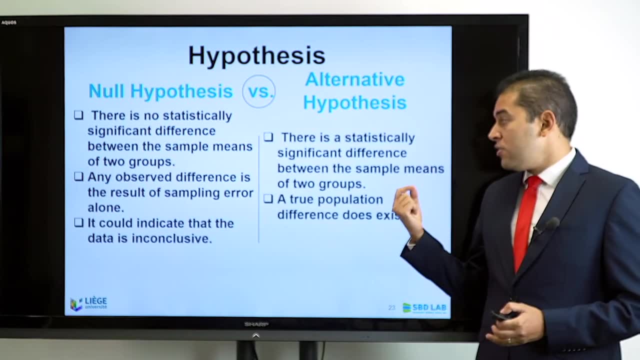 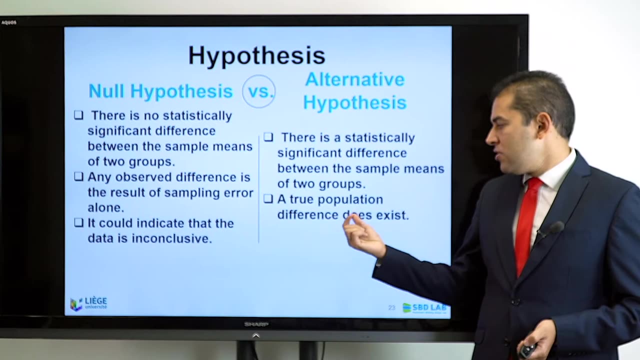 have a positive outcome. in this sense we talk here about the alternative hypothesis. there is a statistical significant difference between the sample means of the two groups. Then we can talk here about alternative hypothesis and in this sense we can say that there is a true 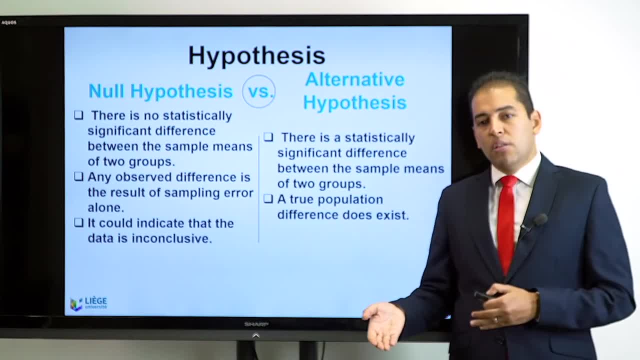 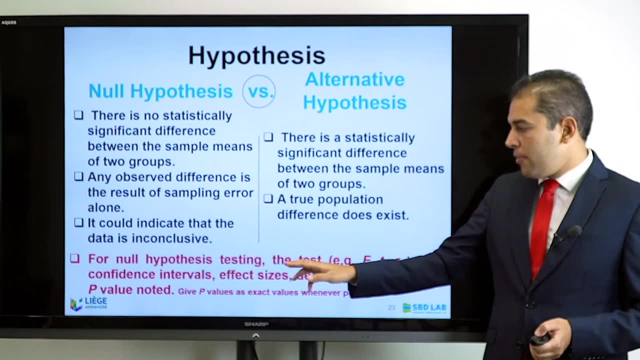 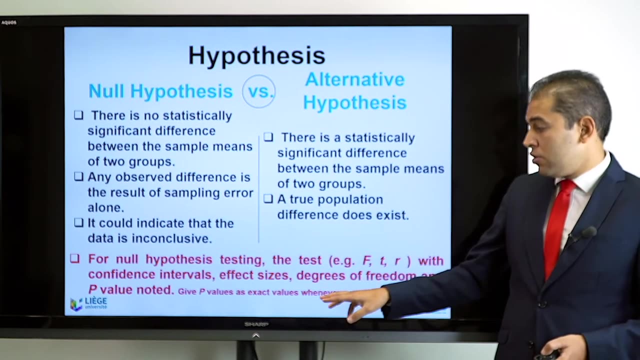 population difference between the intervention population and the no intervention population. And again, when we do reporting, we must talk about our null hypothesis, testing all the type of tests that were conducted, for example the F factor, the T, the R factor, with confidence intervals and the effect of size, the degree of freedom and the P. 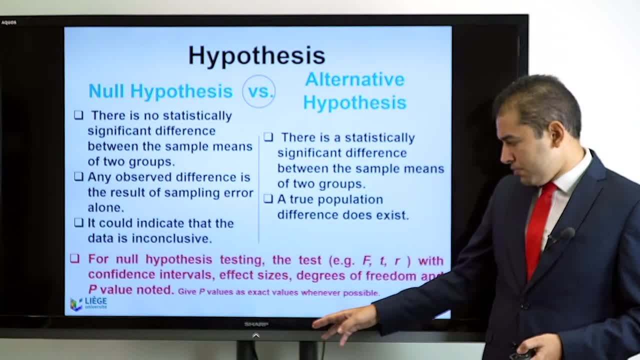 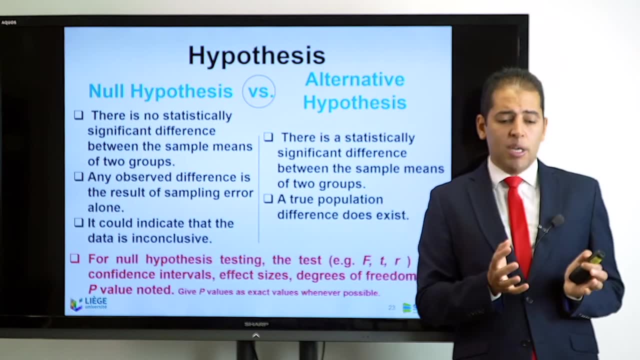 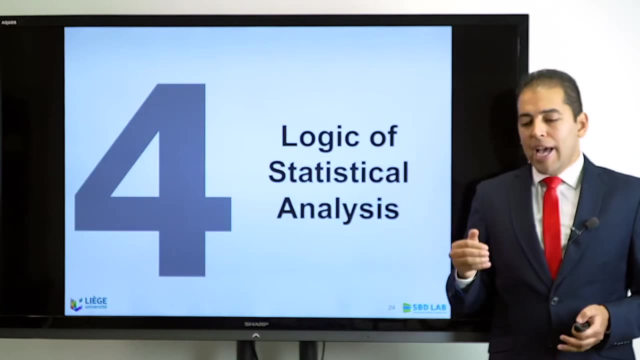 value must be also noted. So, in this sense, P values are, as an exact value, whenever possible, must be communicated. So this is the overall logic before starting designing my statistical framework and before starting my test. Now let's talk about the logic of statistics, and this is a 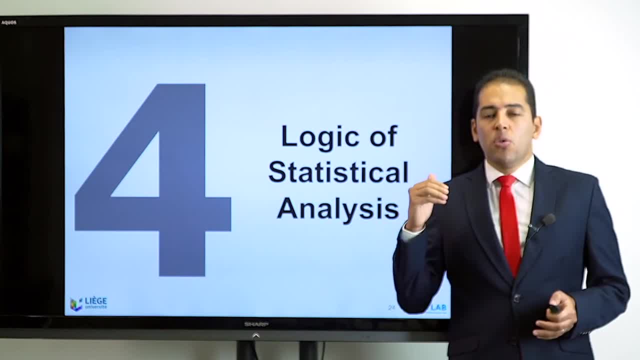 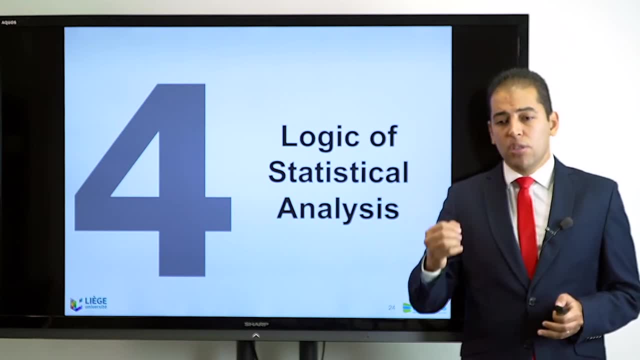 very important part of our presentation today, because many people go into detail with doing testing without understanding the logic, And for me, I care more about the logic of statistic understanding it and I want you to make sure that you are in line, understanding what is the logic behind your statistical testing, Why we 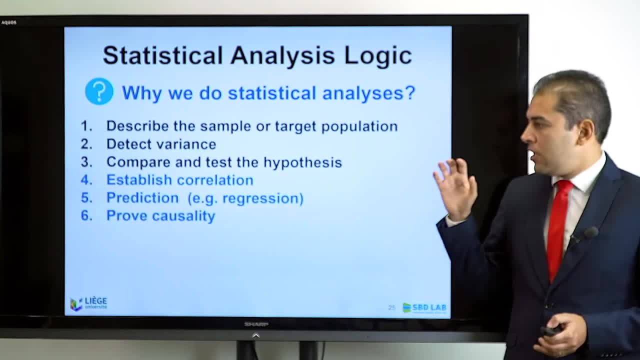 do statistical analysis actually. Keep this into account and I advise you to keep always take note of that why we do statistical analysis. keep this in the account and I advise you to keep always take note of that why we use statistical analysis before and put this in front of you when you start working on statistics. 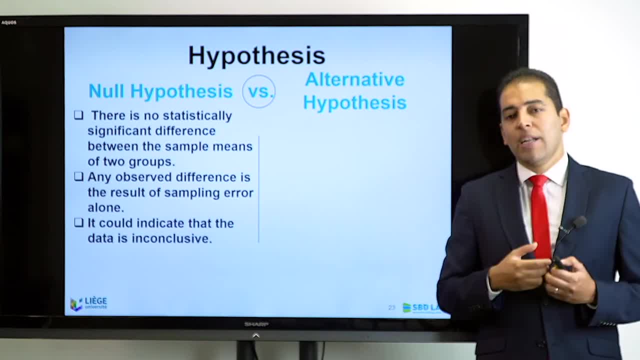 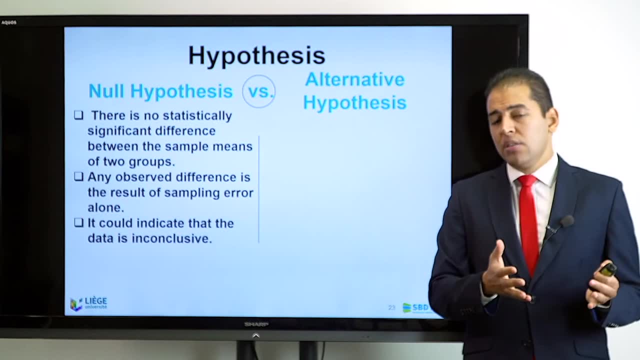 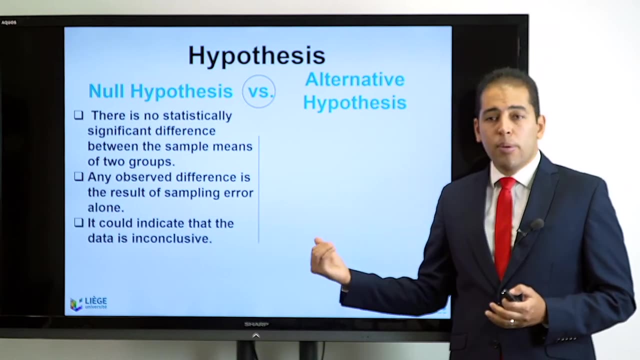 intervention or my treatment to my sample and I found that there is no variance. so here I say there is no difference between the sample, the baseline sample, and alternative or sample number one, which includes the intervention. Any observed difference is the result of sampling error alone. in 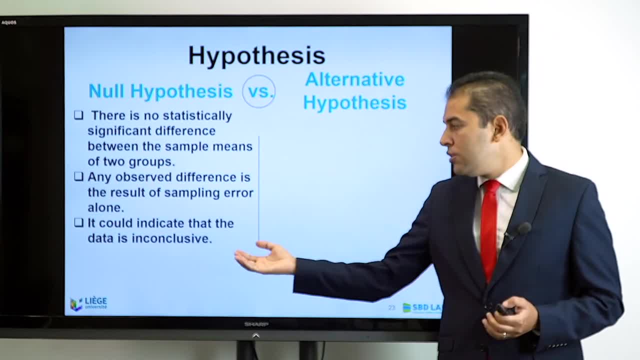 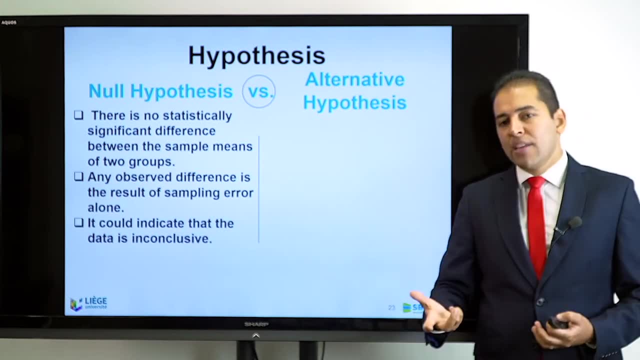 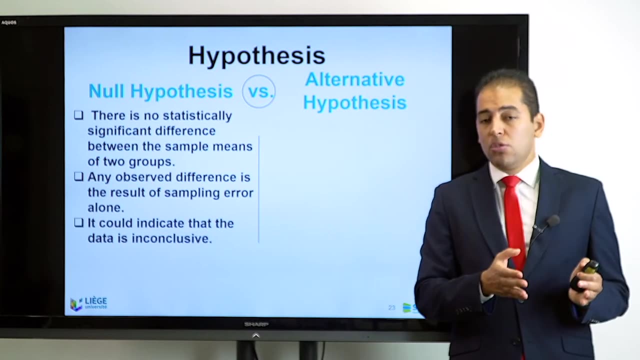 this case. most probably this can be another interpretation or it could be indicating that the data is wrong. In conclusion, those are the three options. if I cannot detect variance, when I do my experiment and I introduce my intervention, I cannot find a variance between the base case condition without intervention and the alternative. 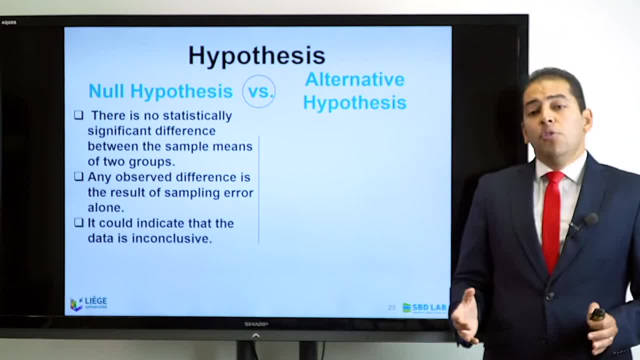 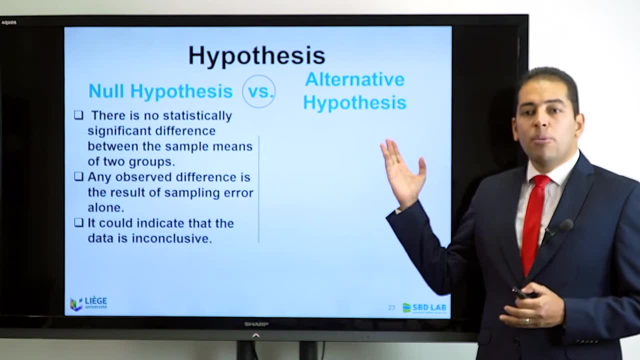 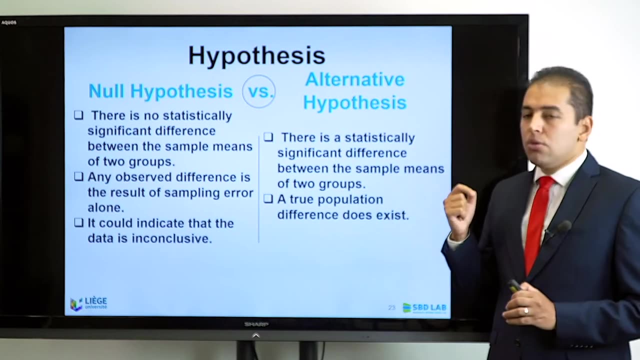 condition with intervention. Now, if you have a positive outcome. in this sense we talk here about the alternative hypothesis- there is a statistical significant difference between the null hypothesis and the alternative hypothesis, So we can say that there is a true population difference between the sample means of the two groups. then we can talk here about alternative. 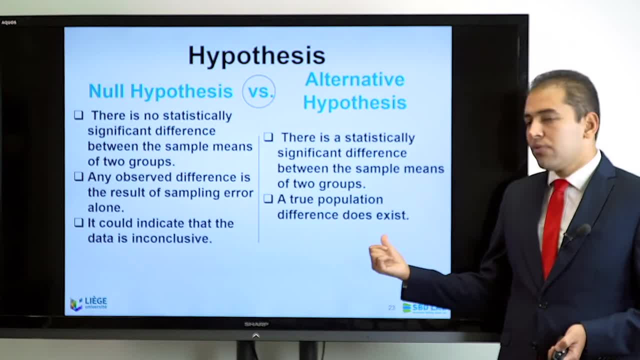 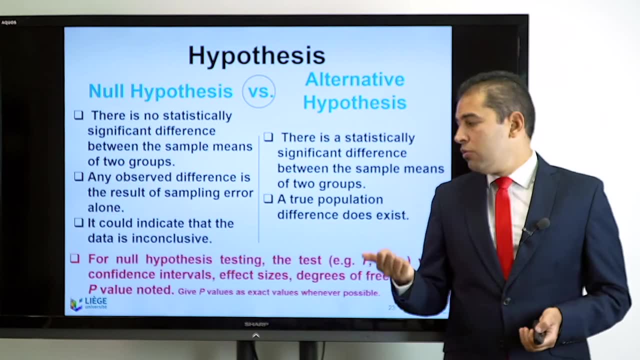 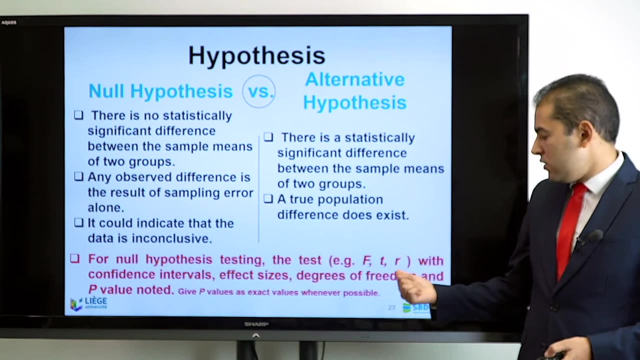 hypothesis and in this sense we can say that there is a true population difference that exists between the intervention population and the no intervention population. and again, when we do reporting, we must talk about our null hypothesis, testing all the type of tests that were conducted, for example the F factor, the T, the R factor, with confidence intervals and the effect of 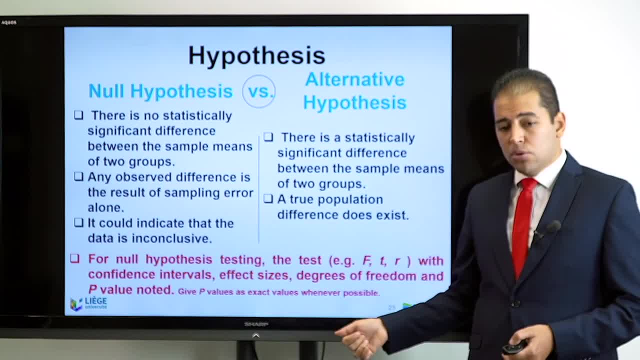 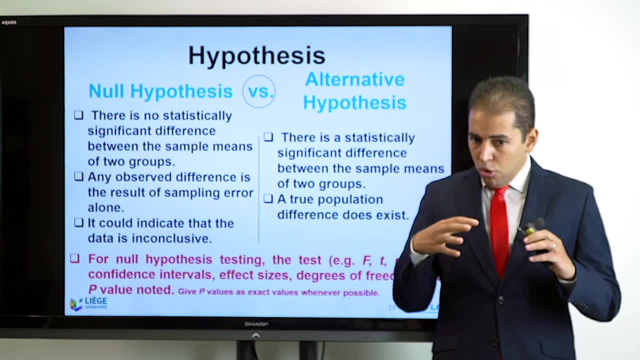 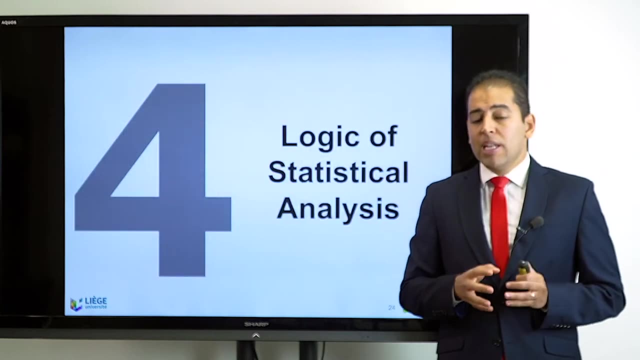 size, the degree of freedom and the p-value must be also noted. So, in this sense, p-values are, as an exact value, whenever possible must be communicated. So this is the overall logic before starting designing my statistic statistical framework and before starting my testing. Now let's 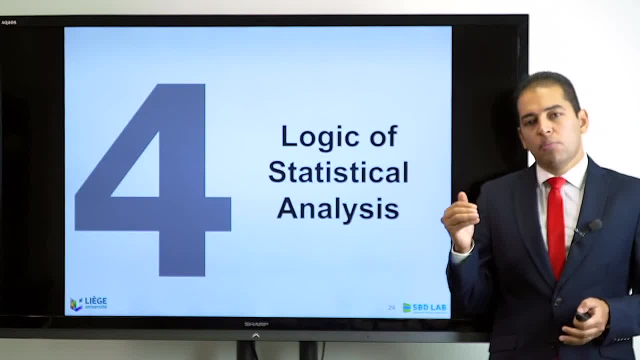 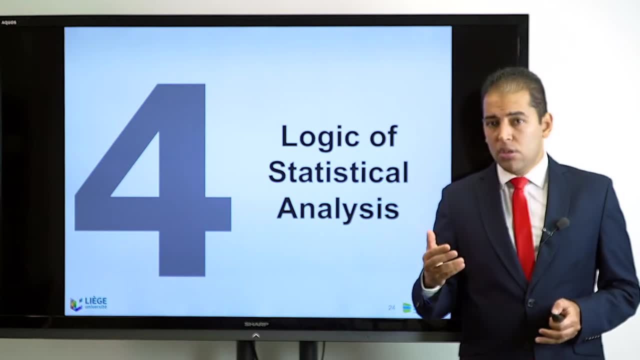 talk about the logic of statistics, and this is a very important part of our presentation today, because many people go into detail with doing testing without understanding the logic, and for me, I care more about the logic of statistic, understanding it, and I want to make sure that you are online. 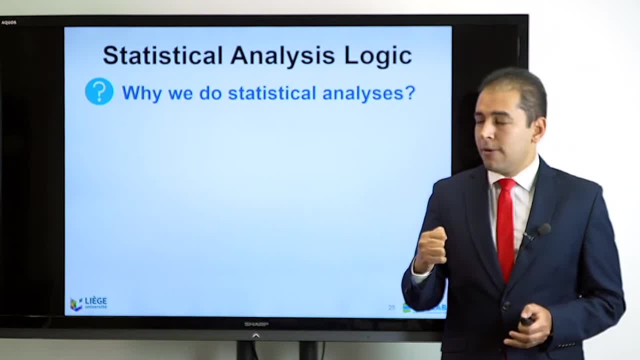 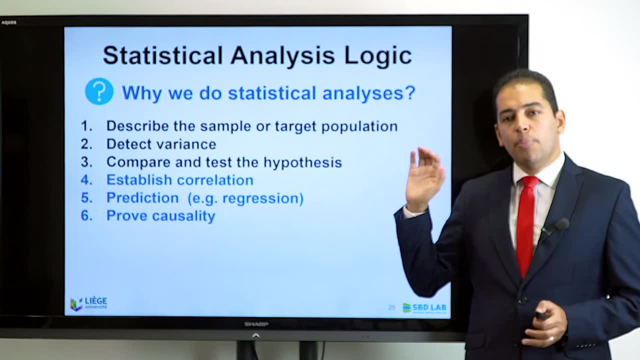 understanding what is the logic behind it. Let's talk about the logic behind it and how we can use it to improve your statistical testing. Why we do statistical analysis actually. keep this into account and I advise you to keep always take note and put this in. 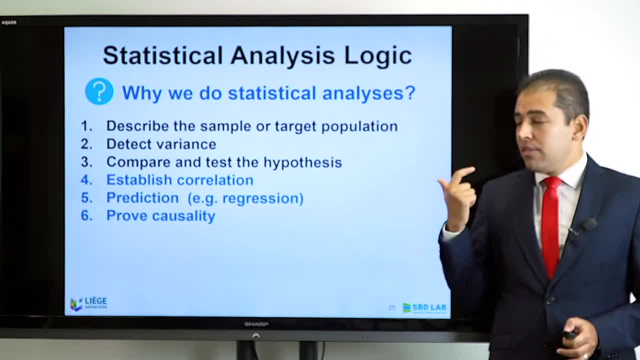 front of you when you start working on statistic. First of all, we look at describing the sample sample or the target population. Number two, we are looking to detect variance. This variance will come mainly from an intervention that we'll introduce. Then we would like to compare and test a hypothesis and if 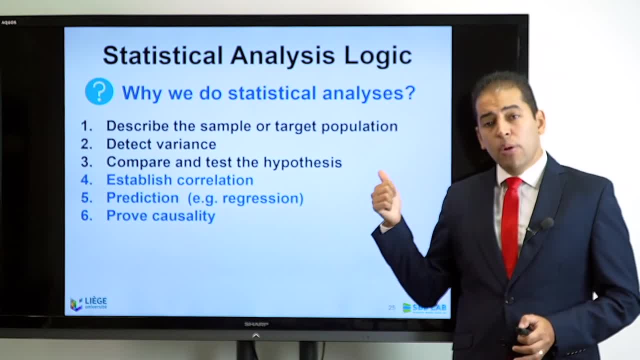 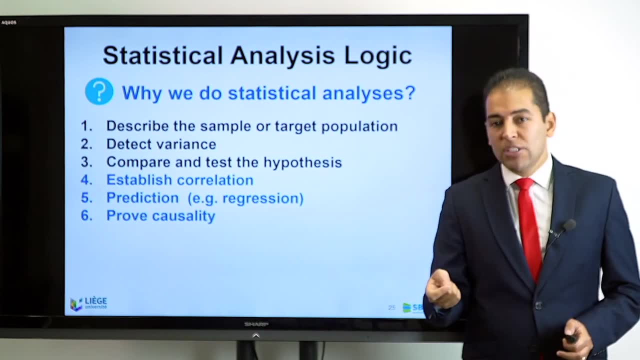 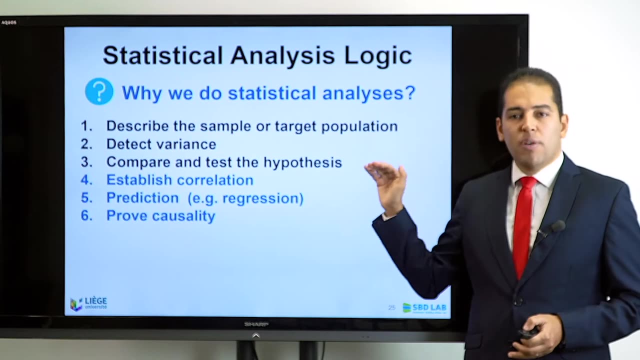 First of all, we look at describing the sample or the target population. Number two, we are looking to detect variance. This variance will come mainly from an intervention that we'll introduce. Then we would like to compare and test a hypothesis and if we have a positive variance or there's a significant variance, 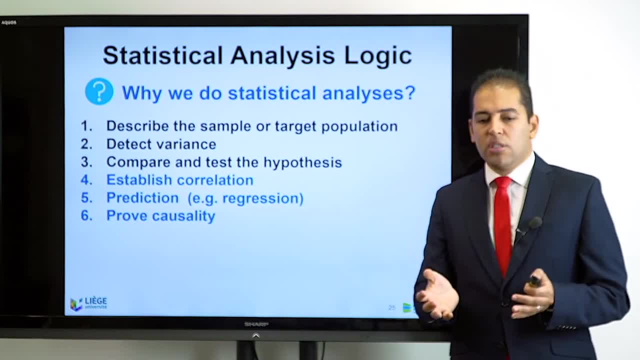 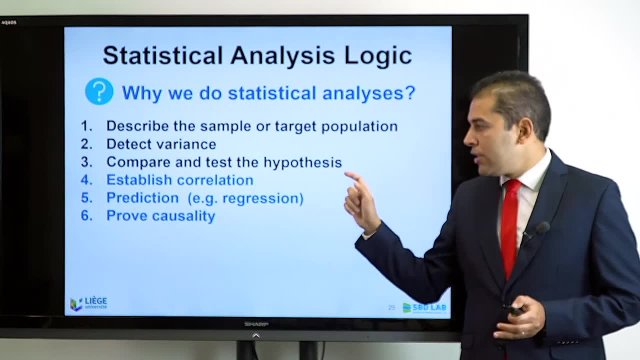 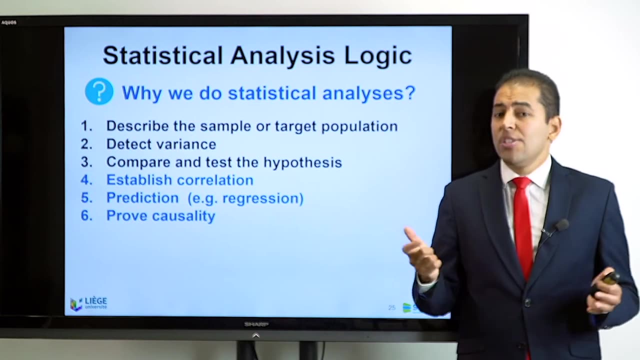 between our intervention to the subjects and the baseline condition of the subject. then we can start to look at establishing a correlation and we can look at the capacity of predicting, through regression for example, and finally we can prove causality. So actually that's all about statistics and that's what we look at. 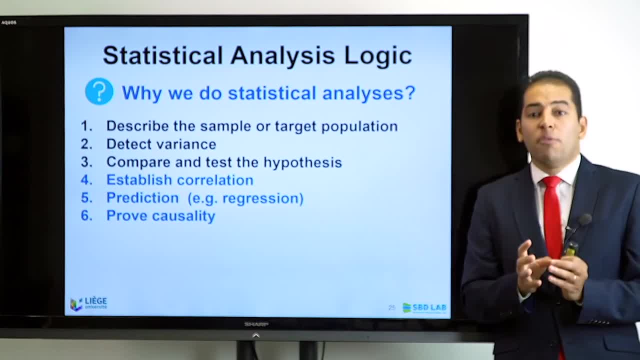 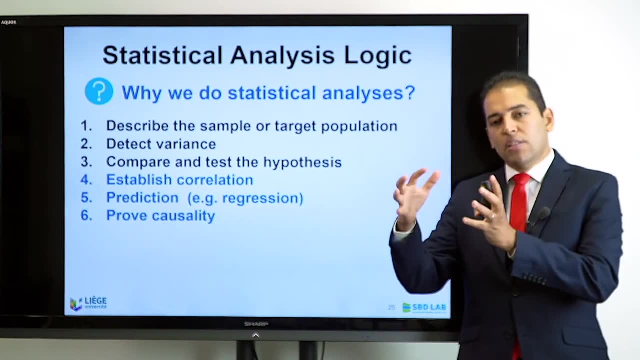 We start with first describing our statistical samples. For sure we are talking here about a comparative approach. I will have always statistical data for a sample without the intervention and a statistical information with intervention, and I start to go step by step checking variance. 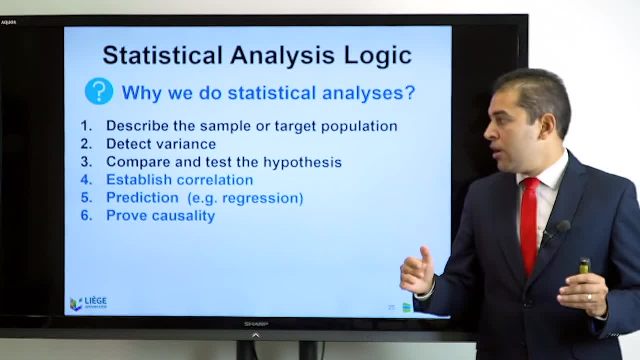 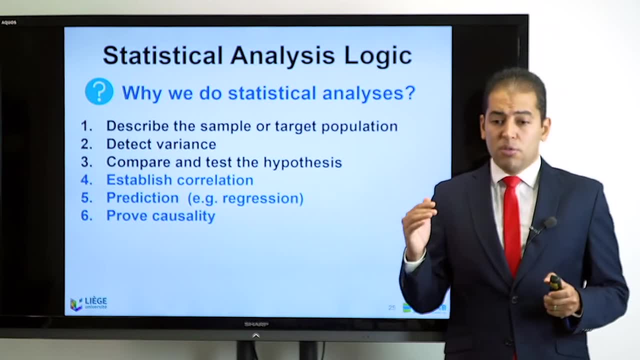 If it's significant, if it's remarkable, I move to the next step, which is establishing a correlation. If it's negative or positive correlation, I can go to the next, which is causality and prediction. So it's very important to keep in this account. 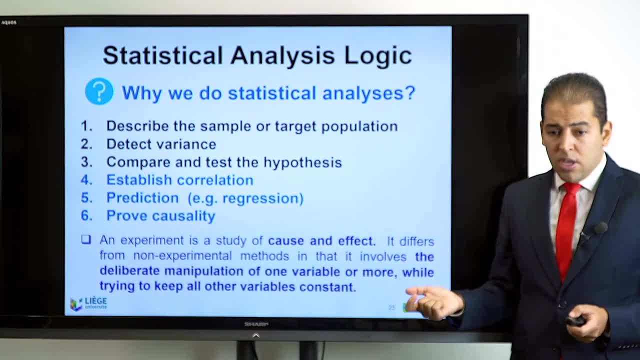 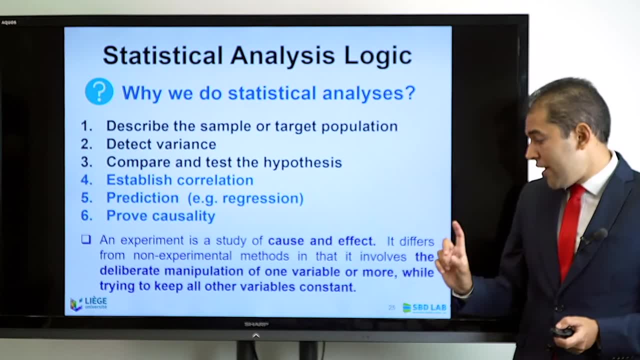 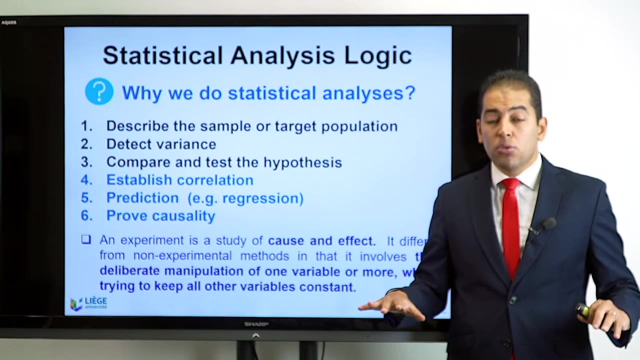 And, in general, an experiment is a study of cause and effect. So it differs from non-experimental method in that it involves the deliberate manipulation of one variable or more, while trying to keep all other variables constant, And here is the importance of control or noise reduction. 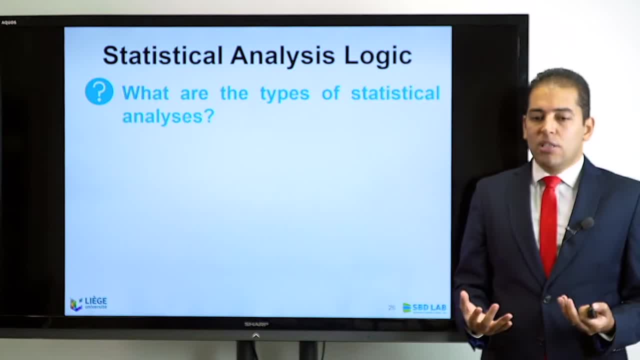 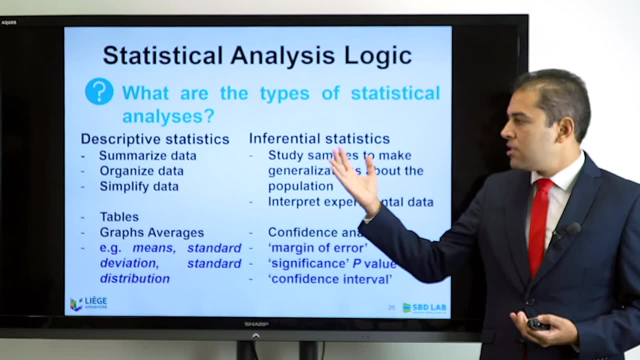 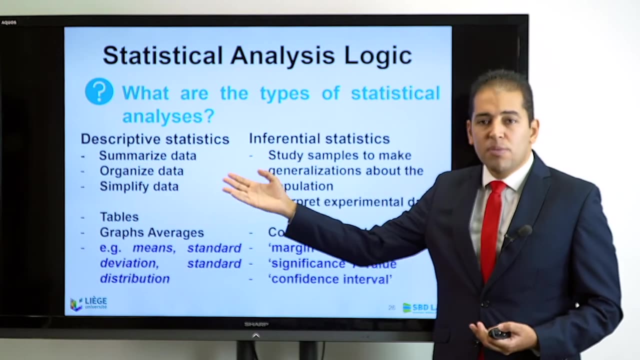 Now, what are the types of statistical analysis that we conduct in general? Well, we do normally two types of statistical analysis: Descriptive statistical analysis and inferential statistics. We call the inferential also parametric and we call the descriptive non-parametric. 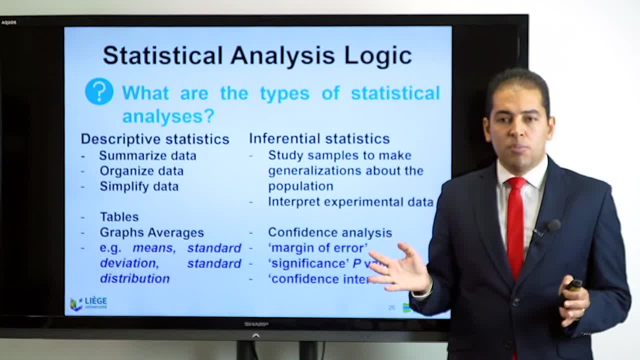 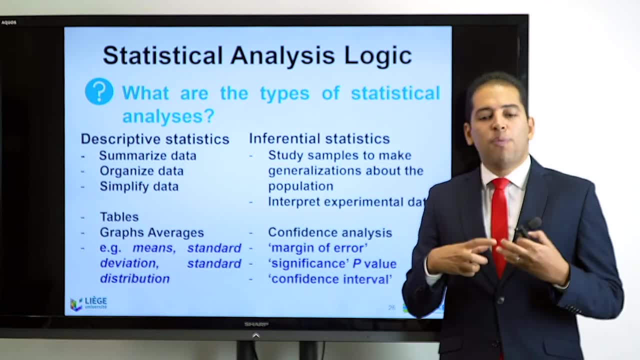 So these are different namings. But what is a descriptive parametric, A statistical or non-parametric statistic? It's simply summarizing the data, organizing the data, simplifying the data We present- tables, graphs, averages- means standard deviation. 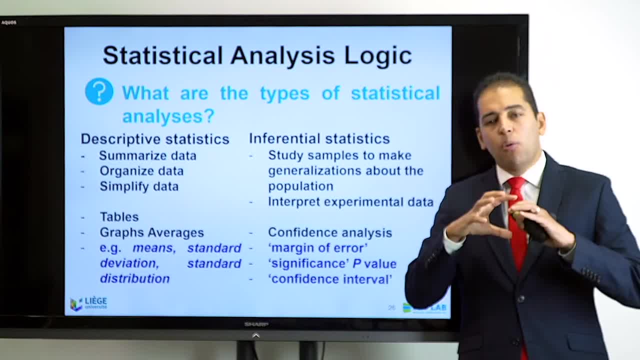 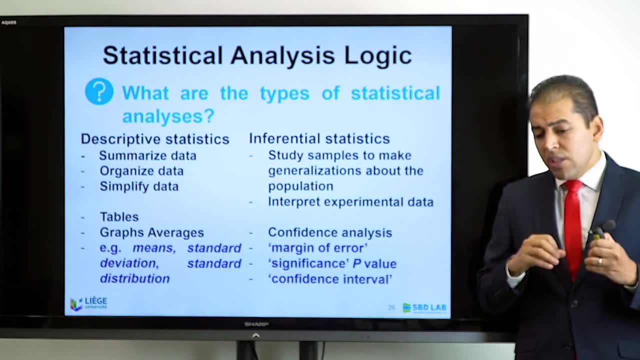 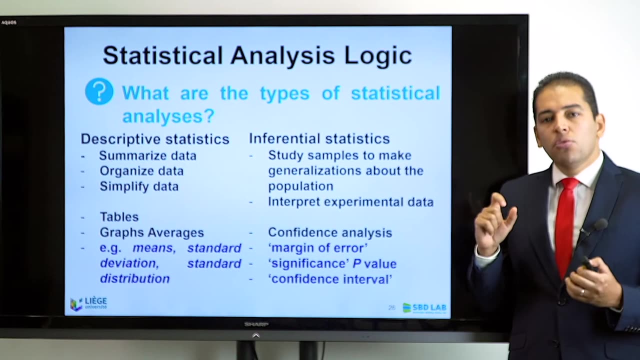 standard distribution. So we are just trying to characterize our sample or our information And that's it, without any analysis or any further treatment. that goes beyond the description. However, when I talk about inferential statistics or parametric statistics here I'm trying to compare samples. 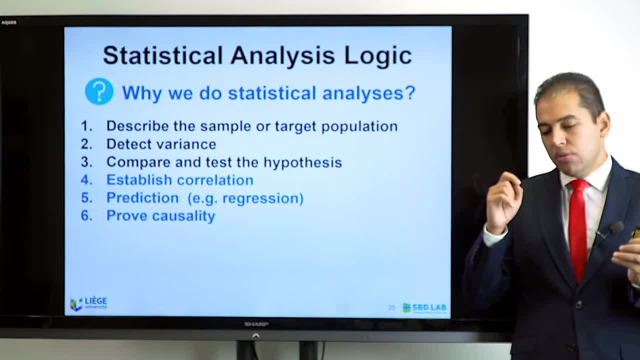 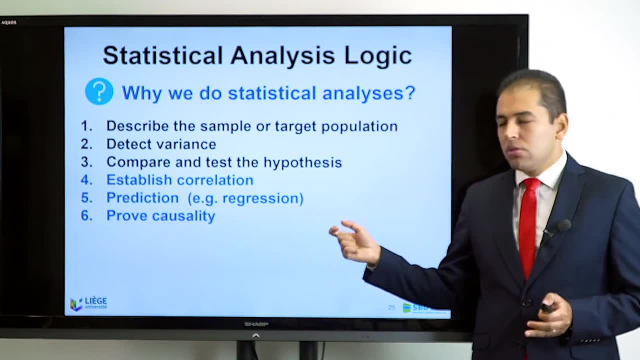 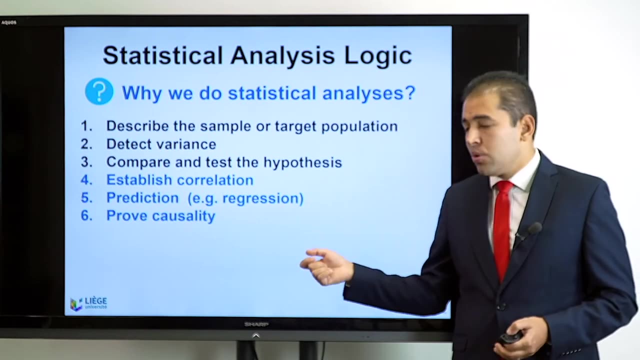 there is variance, or there is a significant variance, between our intervention to the subjects and the baseline condition of the subject, then we can start to look at establishing a correlation and we can look at the capacity of predicting, through regression for example, and finally we can prove causality. So actually, that's all about statistic and that's what we 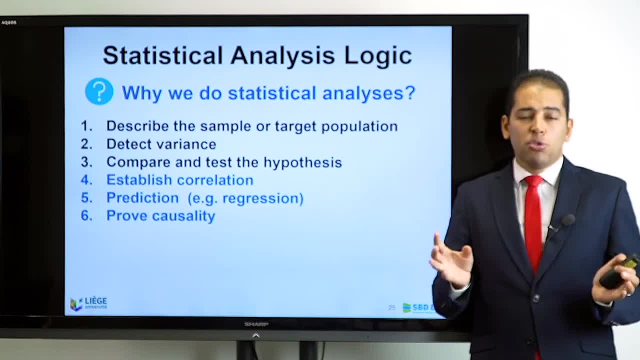 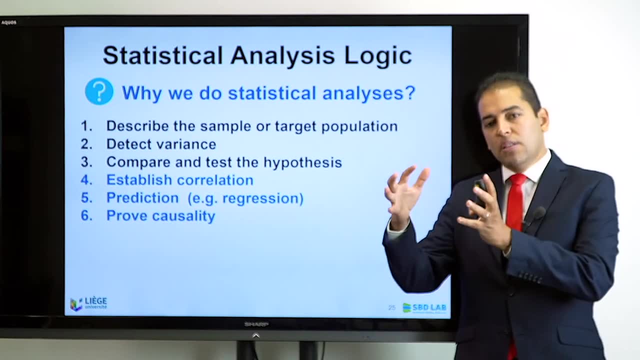 look at. We start with first describing our statistical samples. For sure we are talking here about a comparative approach. I will have statistical data for a sample without the intervention and a statistic information for with intervention, and I start to go step by step Checking. 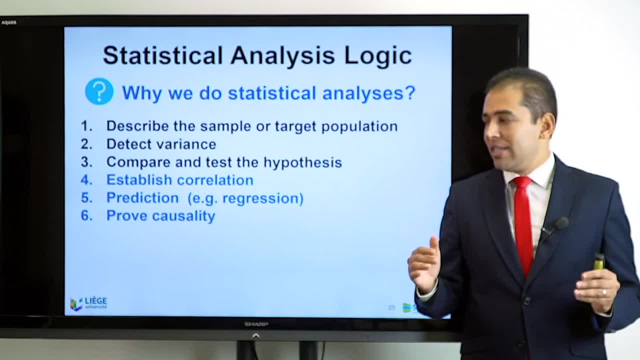 variance. if it's significant, if it's remarkable, I move to the next step, which is establishing a correlation. If it's negative or positive correlation, I can go to the next, which is causality and prediction. So it's very important to keep in this account and, in general, an experiment is a study of cause and 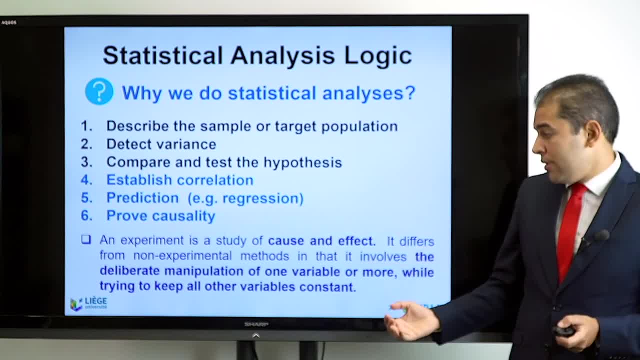 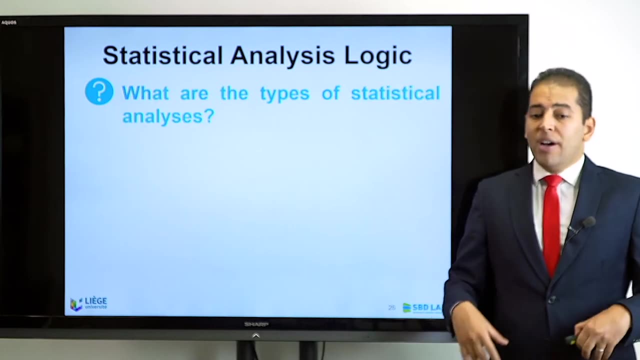 effect. So it differs from non-experimental method in that it involves the deliberate manipulation of one variable or more, while trying to keep all other variable constant, and here is the important of control or noise reduction. now, what are the types of statistical analysis that we conduct in general? well, 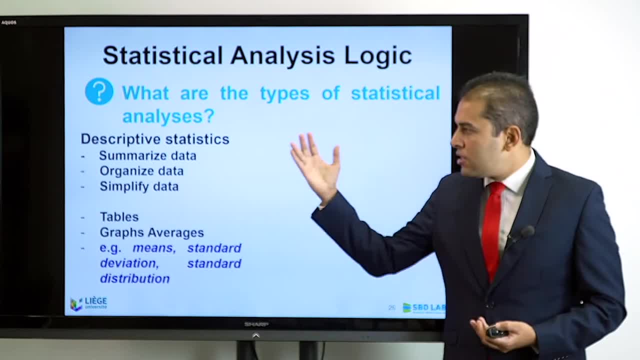 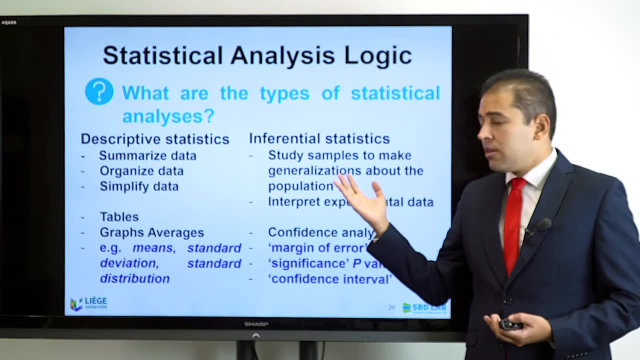 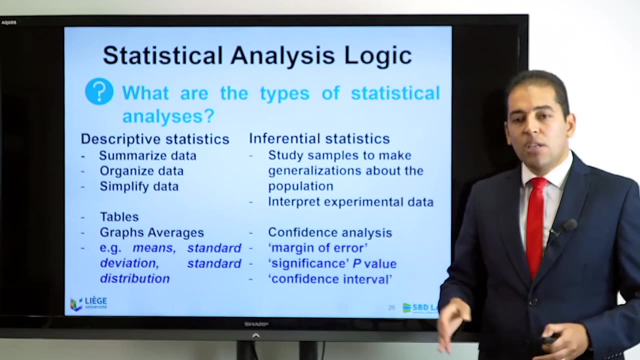 we do normally two types of statistical analysis: descriptive statistical analysis and inferential statistics. we call the inferential also parametric and we call the descriptive non-parametric. so these are different namings. but what is a descriptive statistic or non-parametric statistic? it's simply. 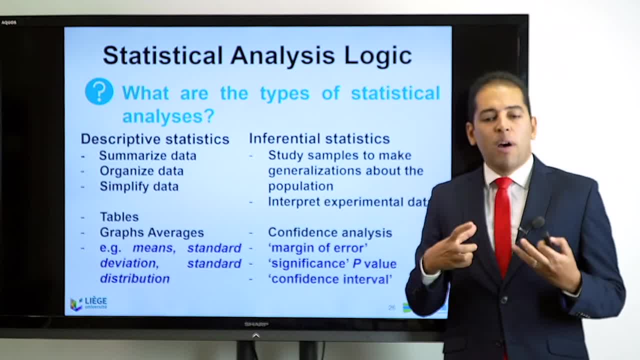 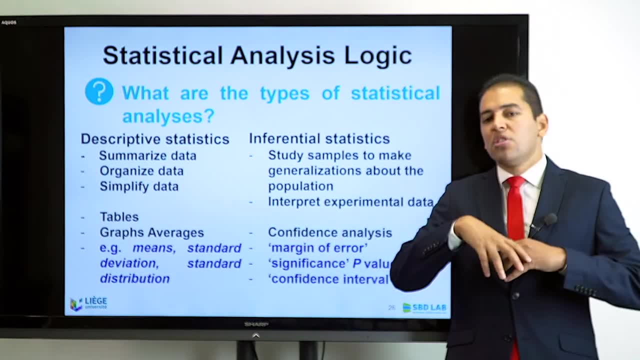 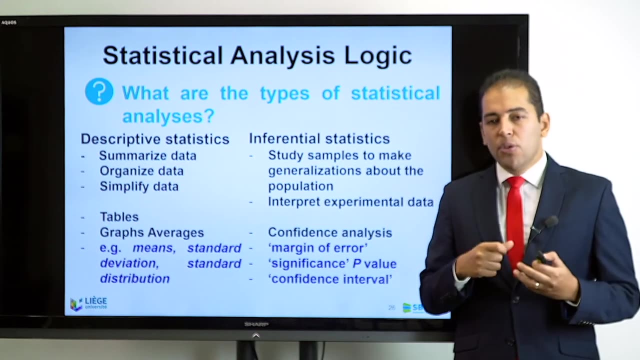 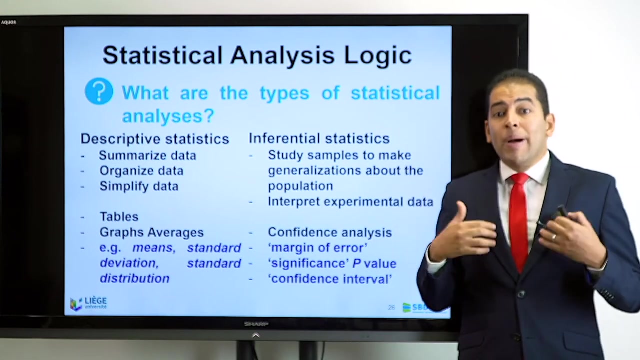 summarizing the data, organizing the data, simplifying the data we present- tables, graphs, averages- means standard deviation, standard distribution. so we are just trying to characterize our sample or our information and that's it, without any analysis or any further treatment. that goes beyond the description. however, when I talk about inferential statistic or parametric statistics here, 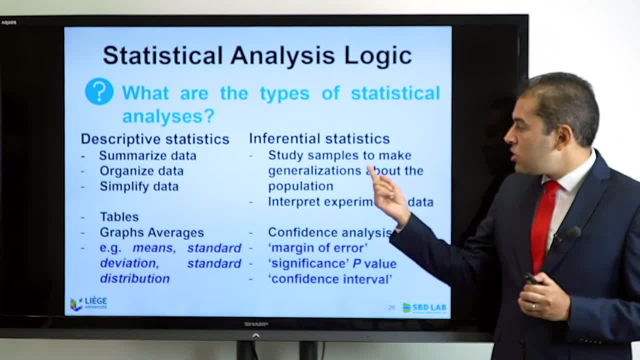 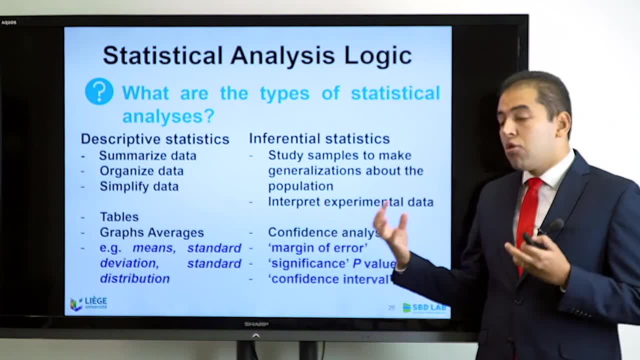 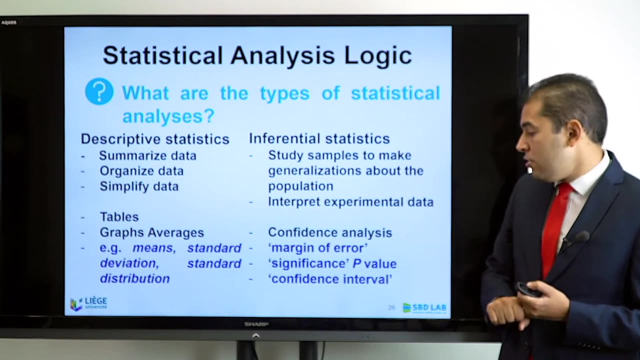 I'm trying to compare samples and I start to study samples to make generalization about the population or interpret the experimental data. look at the confidence of my analysis, and here I can look at the margin of error, the significance, the p-value, the confidence interval and so on. so it's very 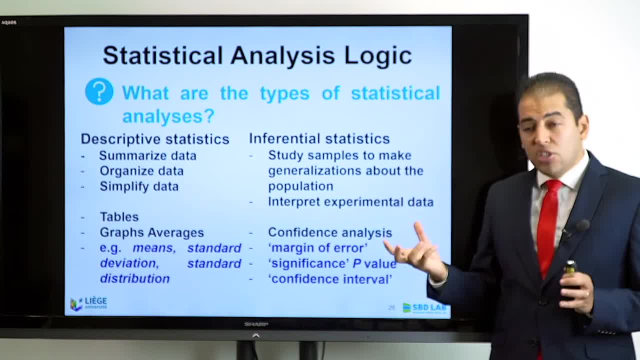 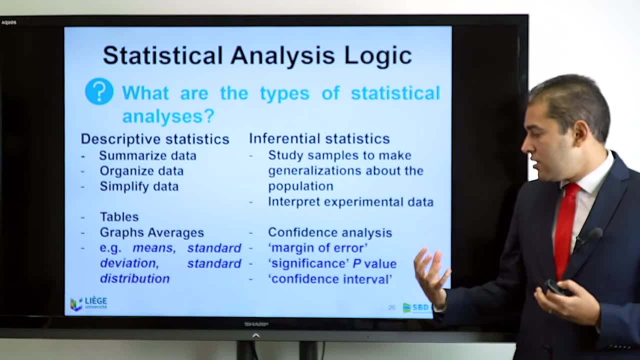 and I try to study samples to make generalization about the population or interpret the experimental data. look at the confidence of my analysis, and here I can look at the margin of error, the significance, the p-value, the confidence interval and so on. 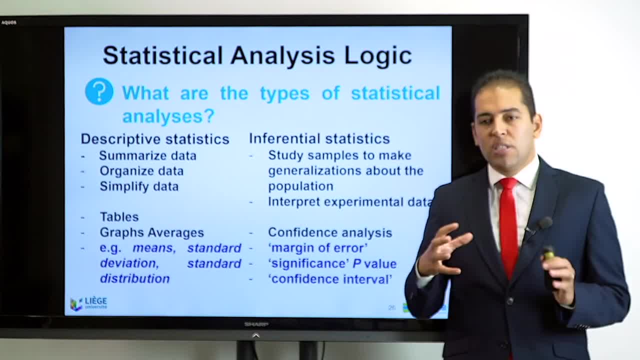 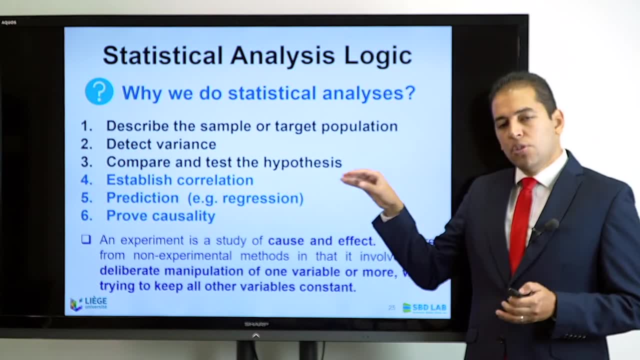 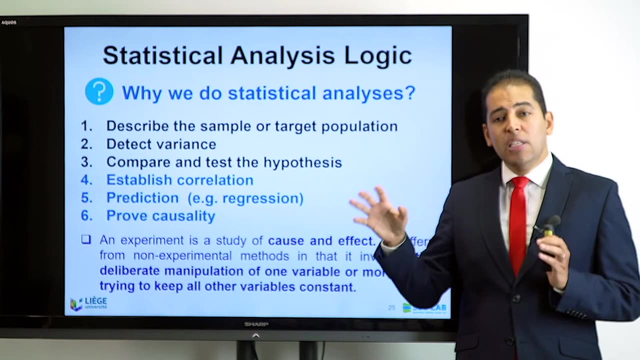 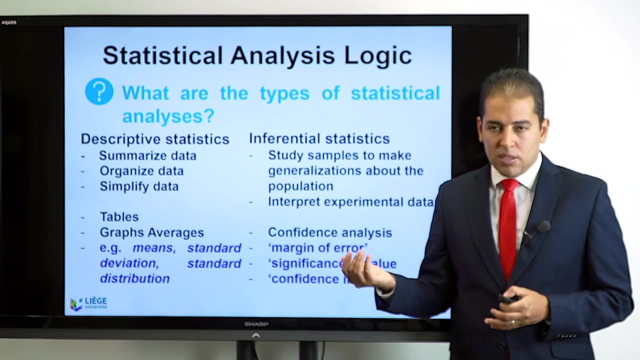 So it's very important to look at those two types of statistical analysis And, as I mentioned before, if you want to go beyond comparing- comparing your different samples- that has an intervention and no intervention- then you must leave the descriptive statistic and go into the inferential statistics and do parametric statistics. 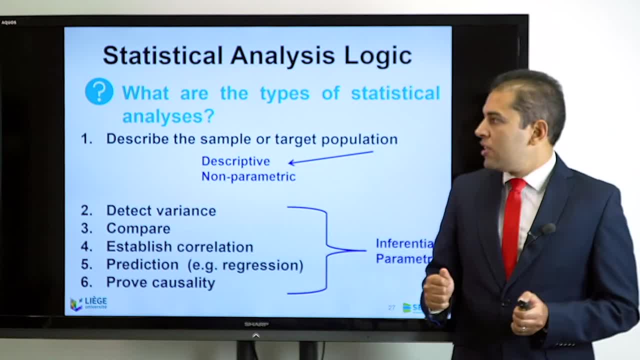 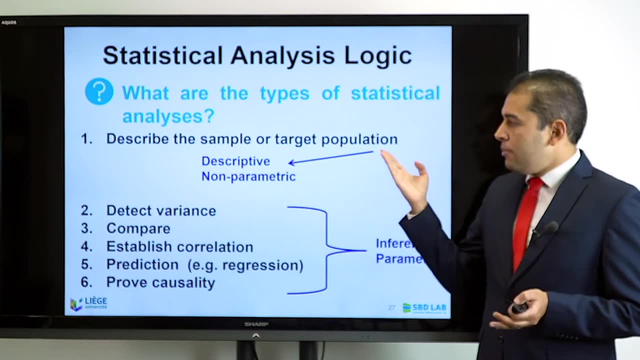 So, as you can see, I'm repeating, or allow me to reiterate. what are the types of statistics? Mainly, we can say we have a group of types of statistics that describe the sample or the target population. We call them descriptive or non-parametric. 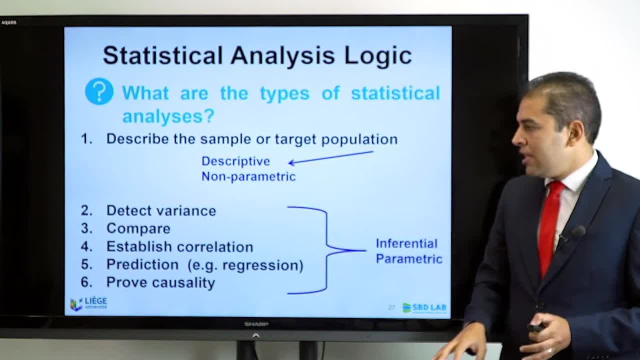 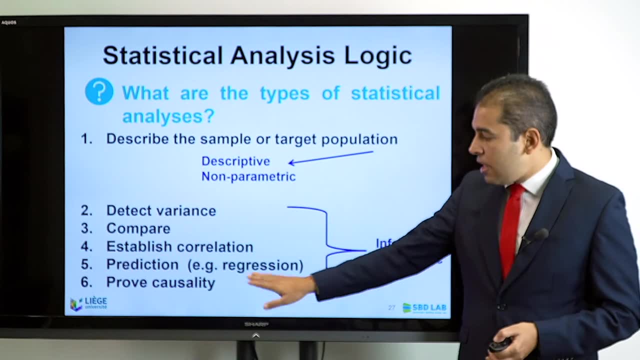 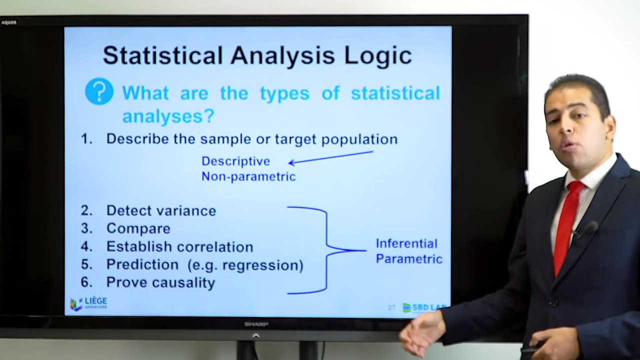 And the second type of statistics. they are looking to detect variance, the covariance, for example the ANOVA test and so on, compare different samples, establish correlation, predict and prove causality, And in this sense we call it inferential or parametric statistics. 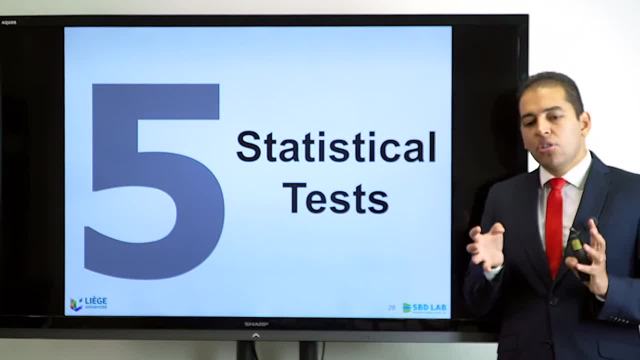 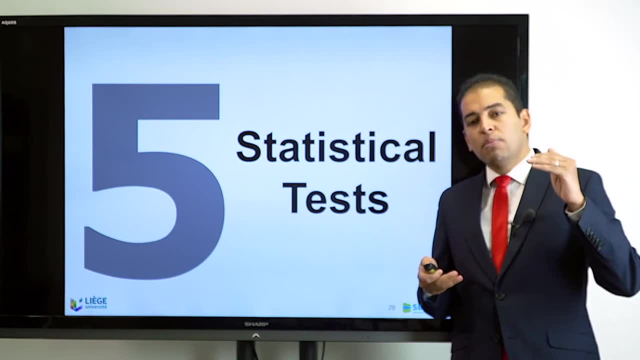 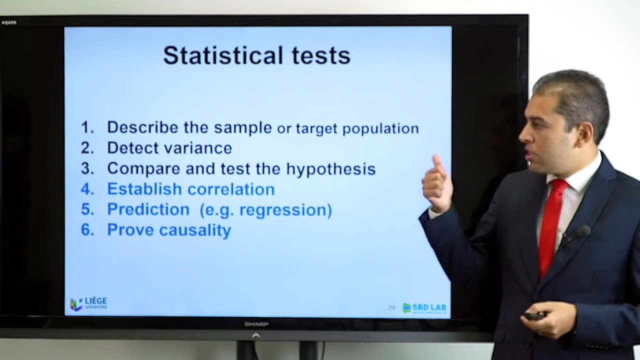 Now let's talk about the main major statistical tests. In this I'm almost reaching the end, but I will go through six main tests and the famous approaches to conduct statistical tests that are based on this coming framework Description: detection of variance, comparison and testing hypothesis. 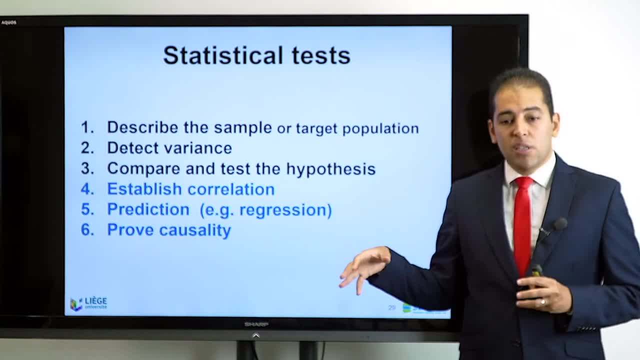 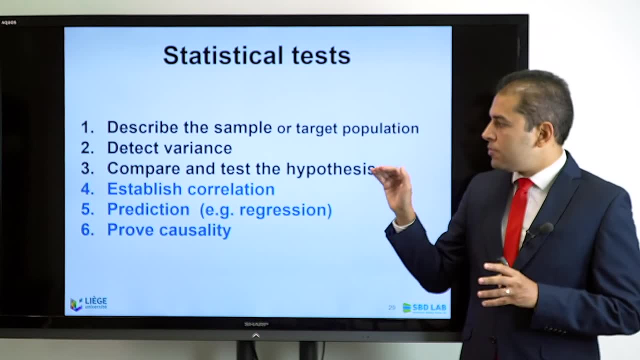 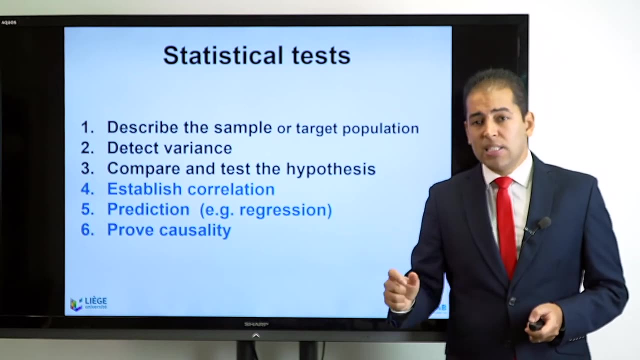 establishing correlation, prediction and proving causality, What I'm going to do in the following presentation. I will follow this number and, for each number of those types of statistical analysis that we conduct, I will share with you the most common tests that are done. 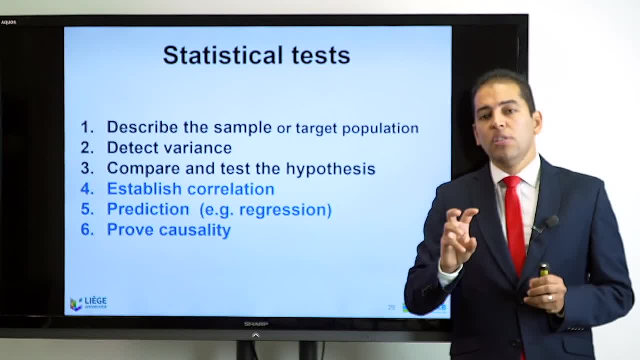 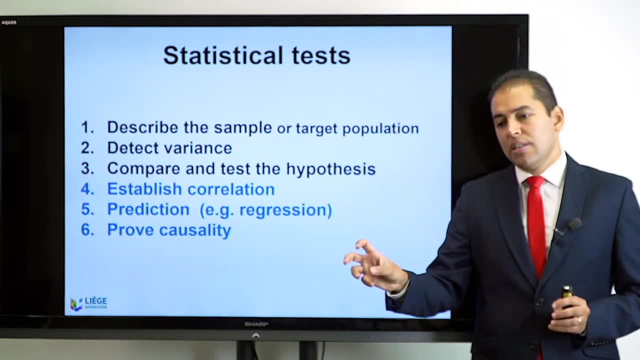 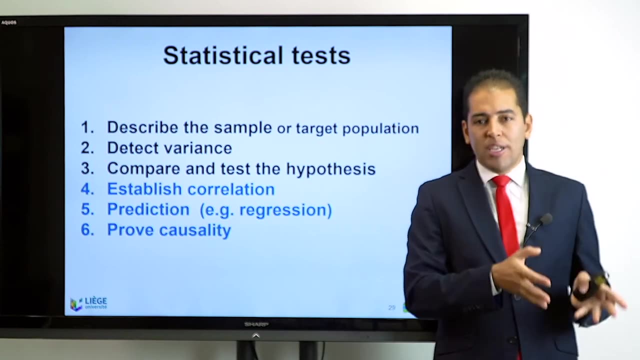 so that when you have an idea and you get lost in all these different statistical tests, you can go back and question yourself and ask: actually this statistical test is meant, for which purpose and why I'm doing it? And then you can go back and make sure that you are using the right test. 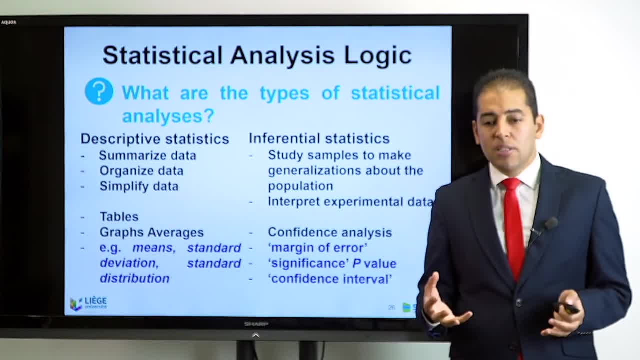 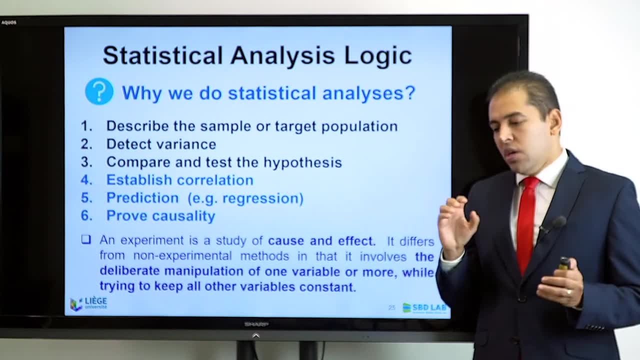 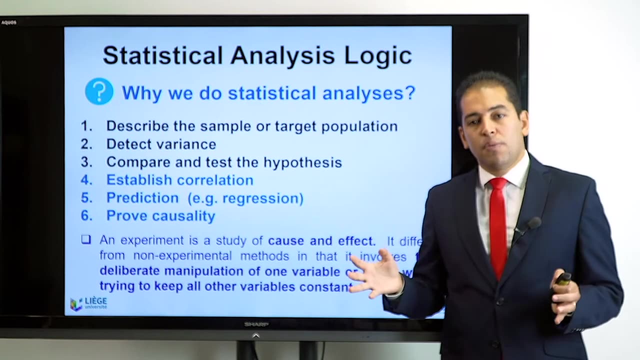 important to look at those two types of statistical analysis and, as I mentioned before, if you want to go beyond comparing your different samples- that has an intervention and no intervention- then you must leave the descriptive statistic and go into the infrared inferential statistics and do parametric. 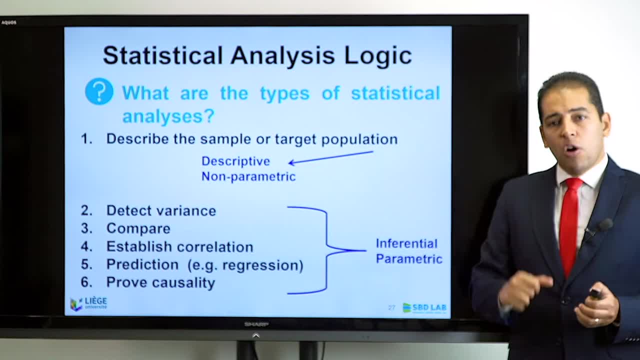 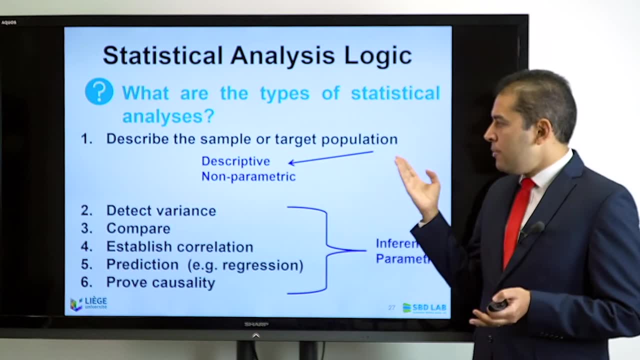 statistics. so, as you can see, I'm repeating, or allow me to reiterate what are the types of statistics? mainly we can say we have a group of types of statistic, that's that describe the sample, sample Y, the masscalm that is defined, number and times y, times y, times k, times the amount of outgoing rate. it's not cooking down by就是ป. 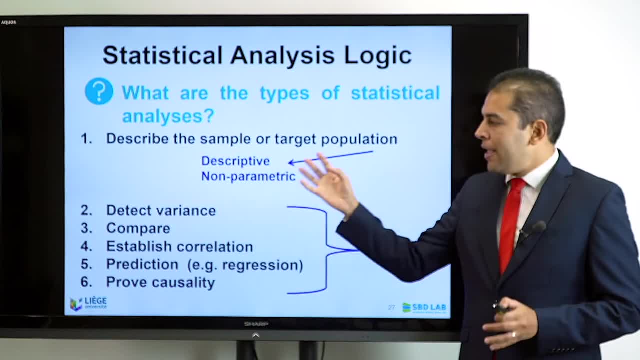 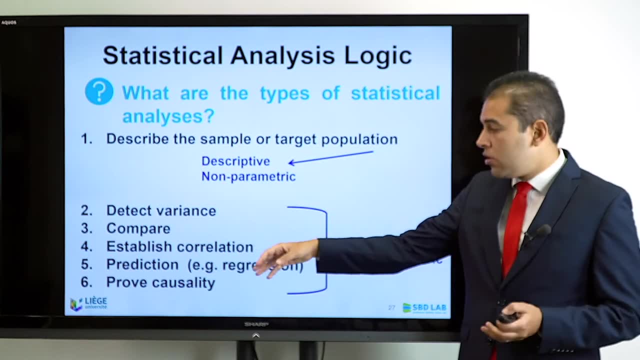 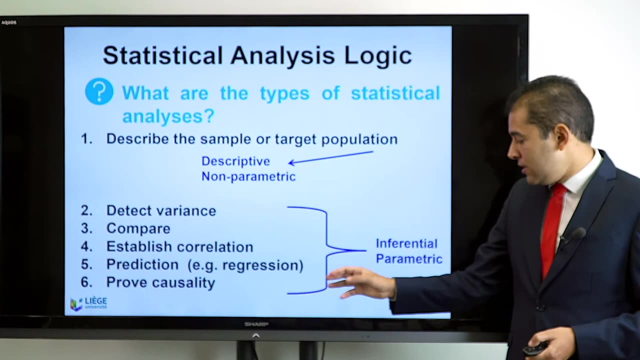 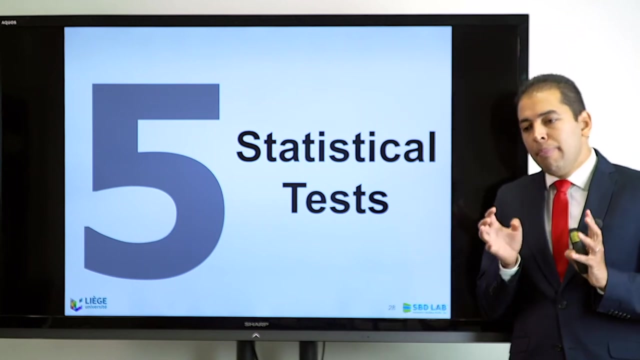 or the target population. we call them descriptive or non-parametric. and the second type of statistics. they are looking to detect variance, the covariance- for example the anova test and so on- compare different samples, establish correlation, predict and prove causality, and in this sense we call it inferential or parametric statistics. now let's talk about the main major statistical text. 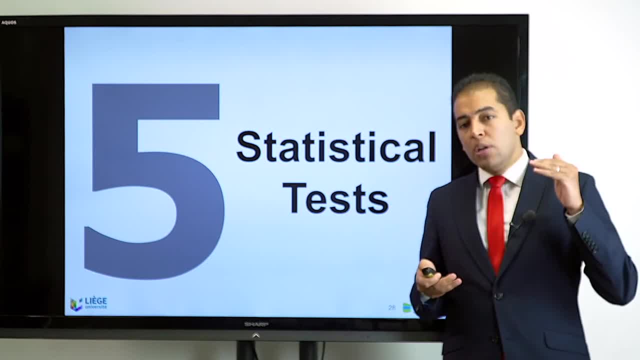 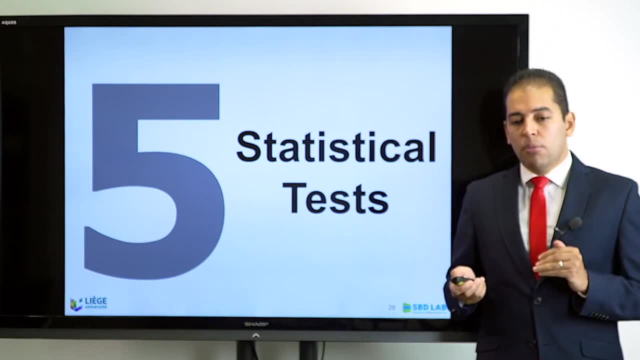 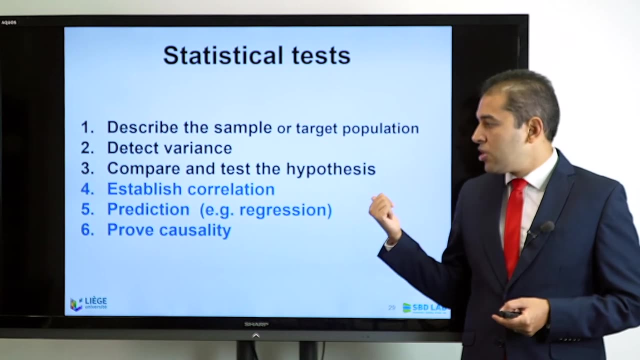 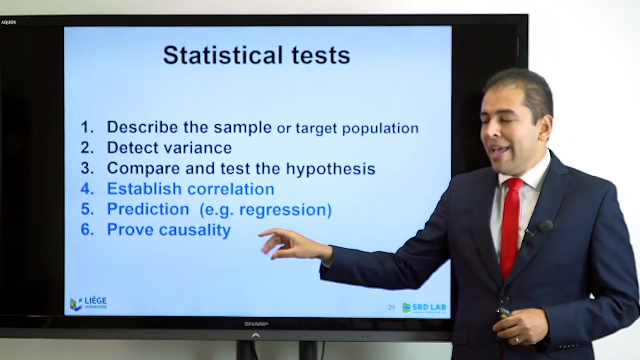 tests. in this i'm almost reaching the end, but i will go through six main famous approaches to conduct statistical text that are based on this coming framework description: detection of variance, comparison and testing hypothesis, establishing correlation, prediction and proving causality. what i'm going to do in the following presentation. i will follow this number and, for each number of 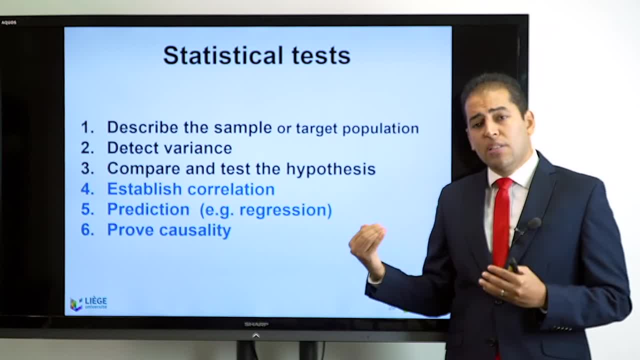 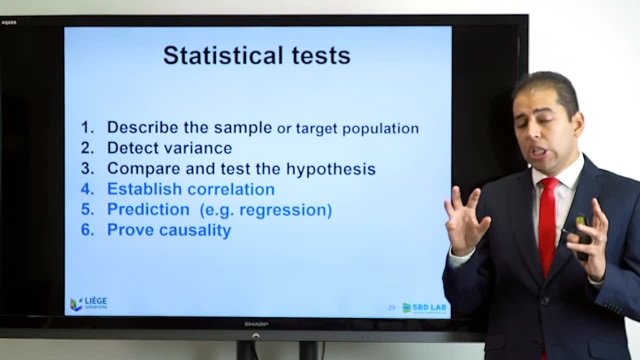 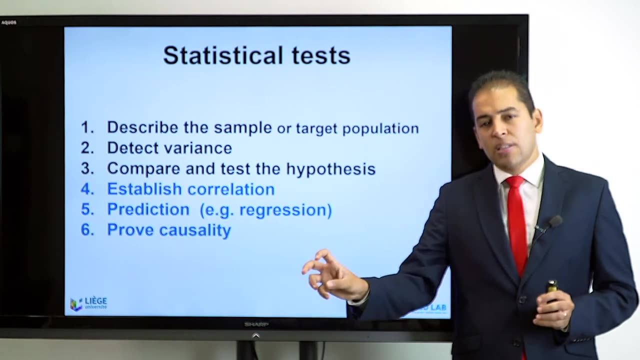 those types of statistical analysis that we conduct. i will share with you the most common tests that are done so that when you have an idea and you get lost in all these different statistical tests, yeah, you can go back and question yourself and ask: actually this, does this statistical test is meant? for which purpose? 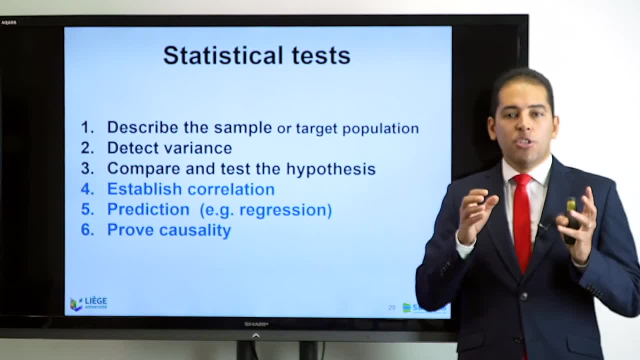 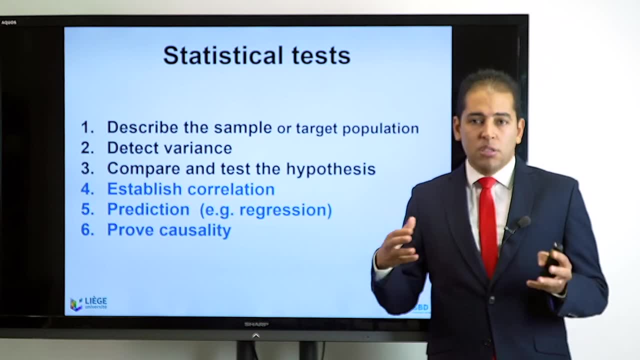 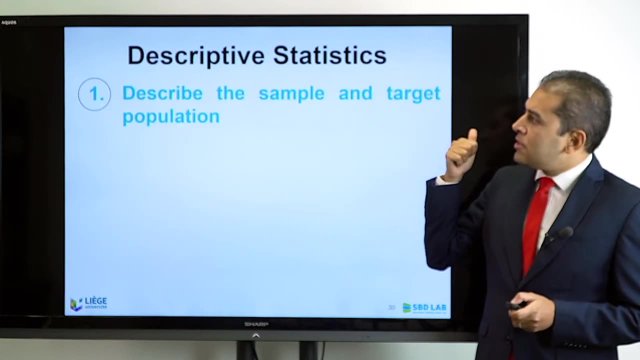 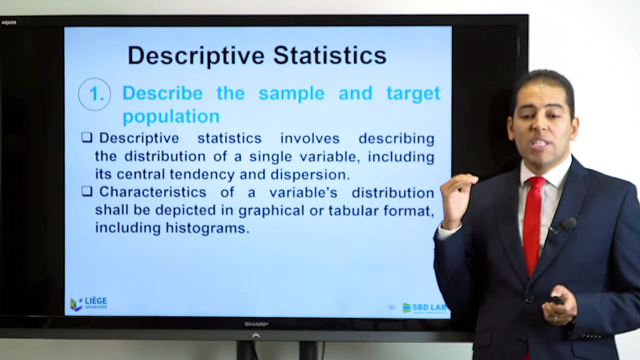 and why i'm doing it, and then you can go back and make sure that you are using the right test for proving the right statistical, let's say, intervention. so first of all, number one, the description part, descriptive statistic. it describes the sample and target population. what is that? descriptive statistic involves describing the distribution. 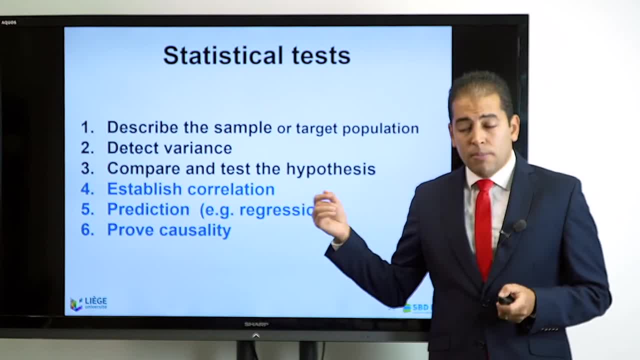 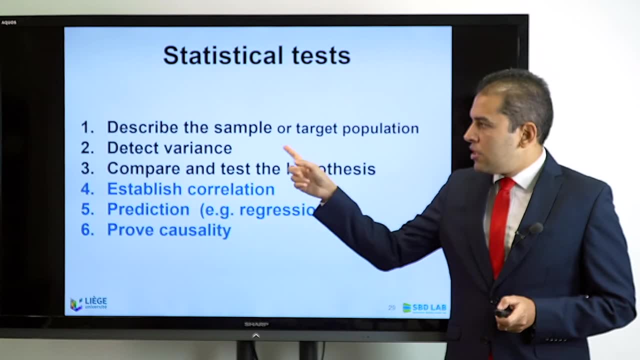 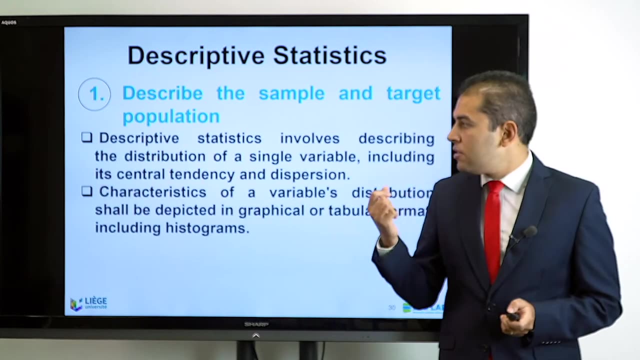 for proving the right statistical, let's say, intervention. So first of all, number one, the description part, Descriptive statistic. It describes the sample and target population. What is that? Descriptive statistic involves describing the distribution of a single variable. 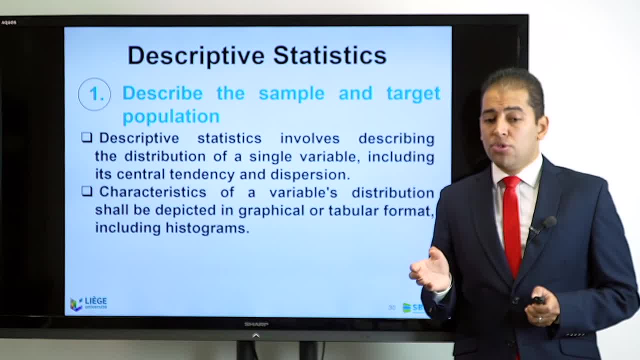 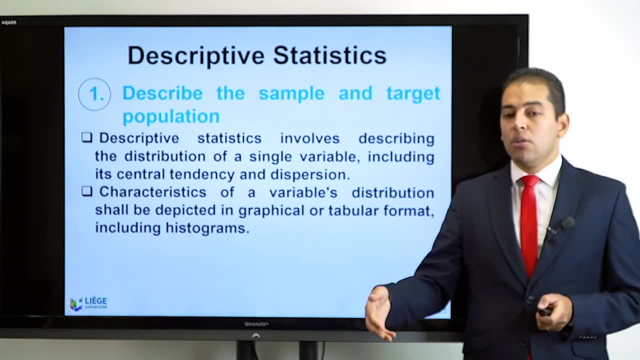 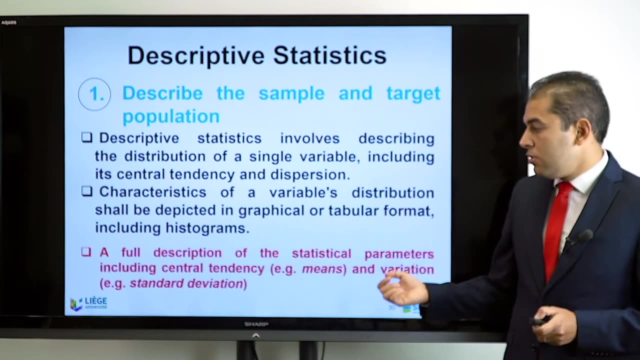 including its central tendency and dispersion, and the characteristic of variable's distribution, shall be depicted in graphical or tabular format, including histograms, And always when you report about it, you need to describe fully your statistical parameters, including the central tendencies, like the means and the variation and the standard deviation. 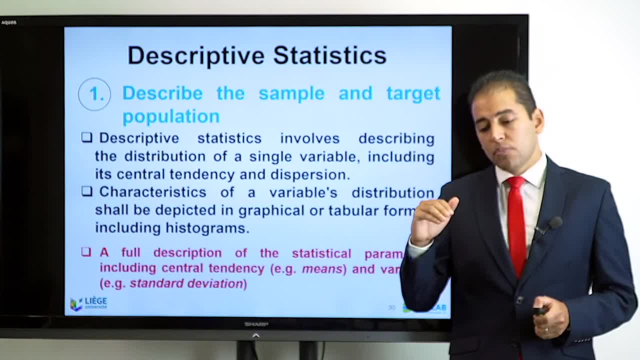 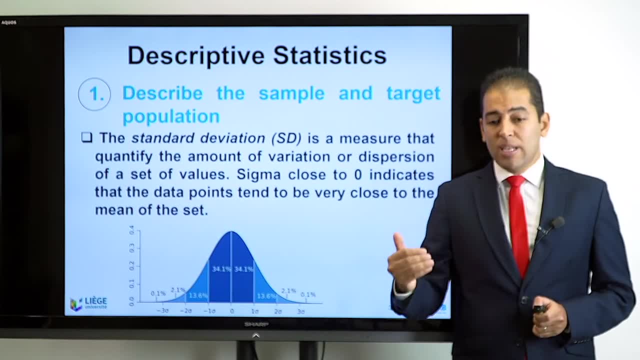 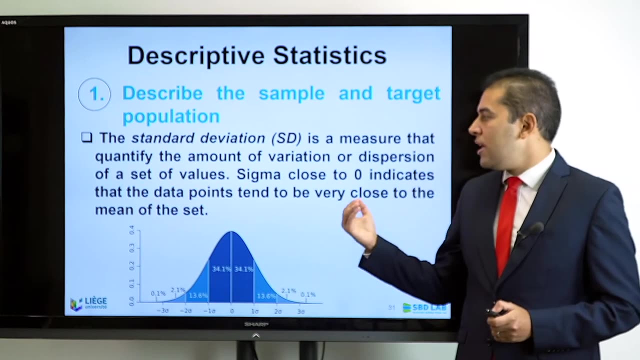 So this is one of the kind of methods to describe your samples, And one of the very famous ways to describe your sample is the standard deviation method, or test, which is a measure that quantifies the amount of variation or dispersion of a set of values. 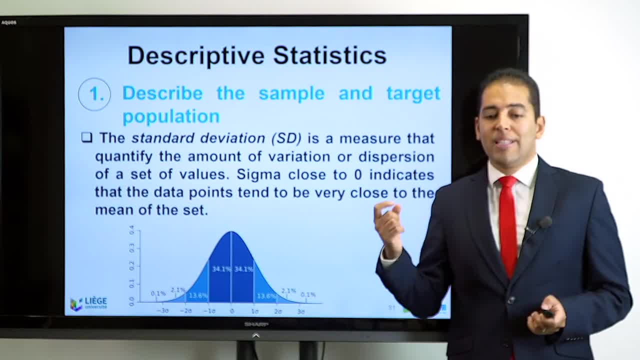 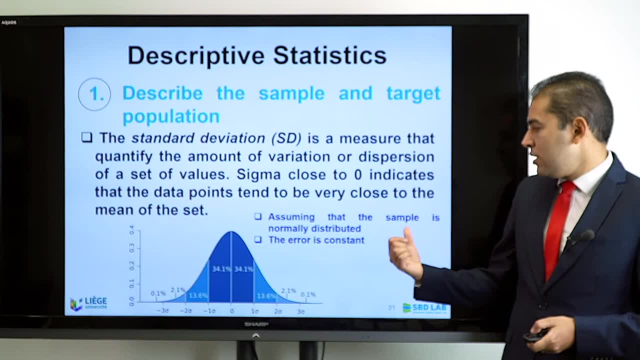 And in this sense we use a sigma close to zero, indicating that the data points tend to be very close to the means of a set. So here, as you can see, we are assuming that the sample is normally distributed and we have a constant error. 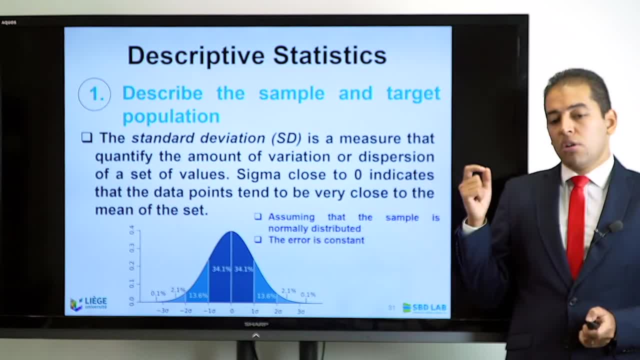 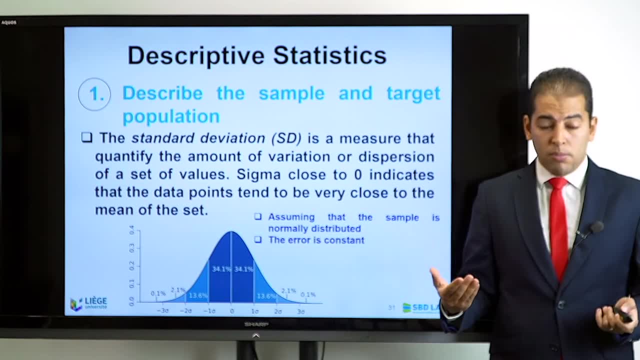 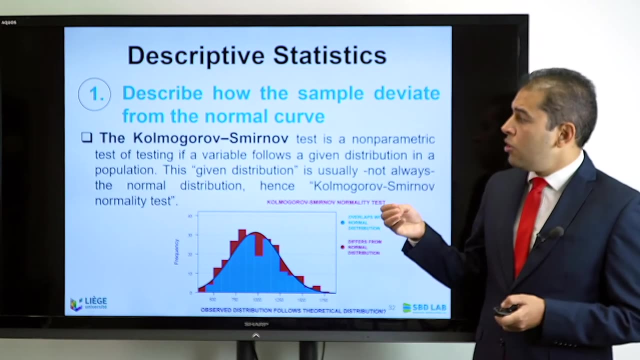 The standard deviation test is one of the most common tests that we use to test the distribution and check if the sample is normally distributed or not. Another very common test that is used to describe a sample is called the Kolmogorov-Smirnov test. 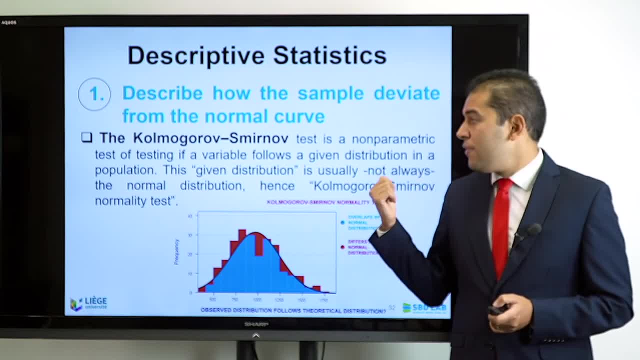 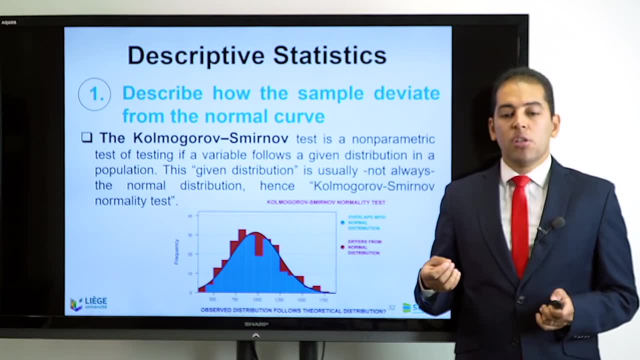 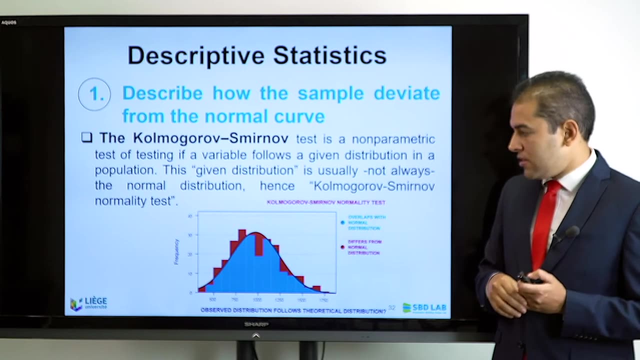 It is a non-parametric test of testing if a variable follows a given distribution in a population, And this given distribution is usually not always the normal distribution. hence the Kolmogorov-Smirnov normality test. And here I can visualize it, and I can through juxtaposition: 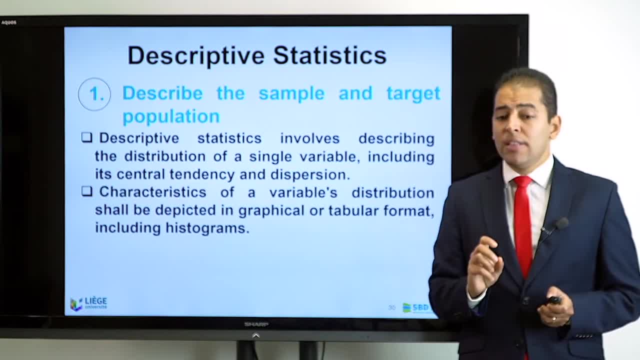 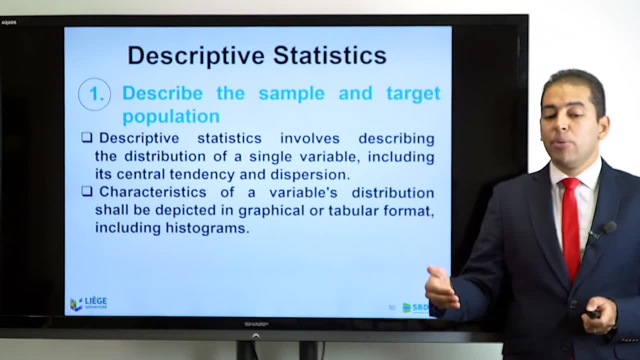 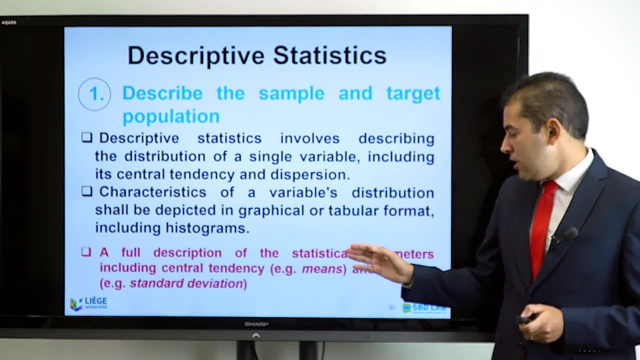 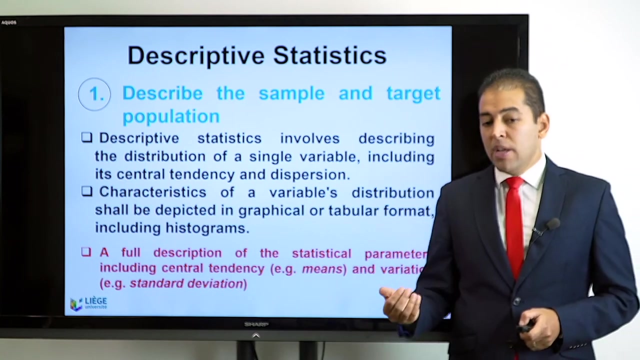 of a single variable, including its central tendency and dispersion, and the characteristic of variables distribution, shall be depicted in graphical or tabular format, including histograms. and always when you report about it, you need to describe fully your statistical parameters, including the central tendencies, like the means and the variation and the standard deviation. so this is one of the 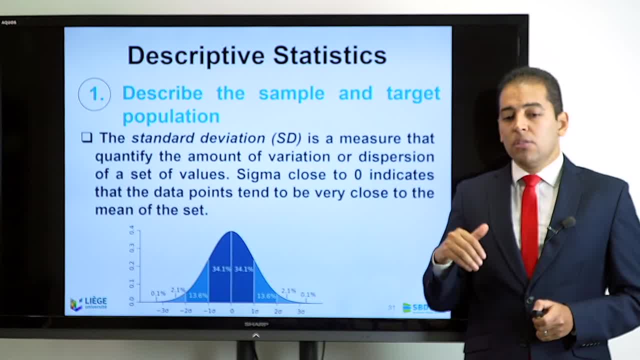 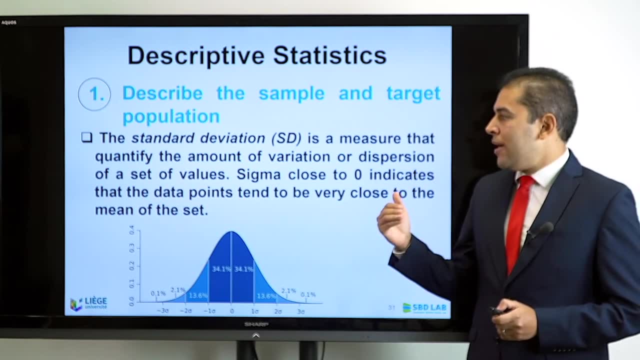 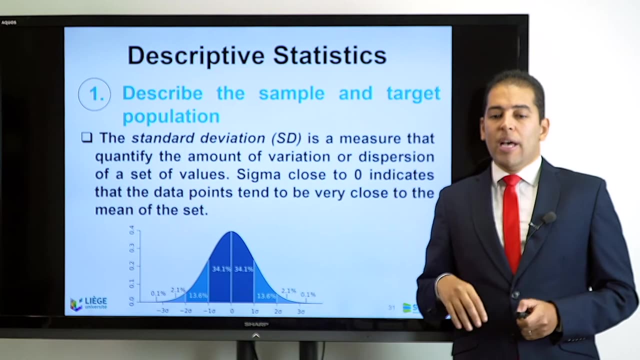 kind of methods to describe your samples, and one of the very famous ways to describe your sample is the standard deviation method or test, which is a measure that quantify the amount of variation or dispersion of a set of values, and in this sense we use a sigma close to zero, indicating that the data points tend to be very 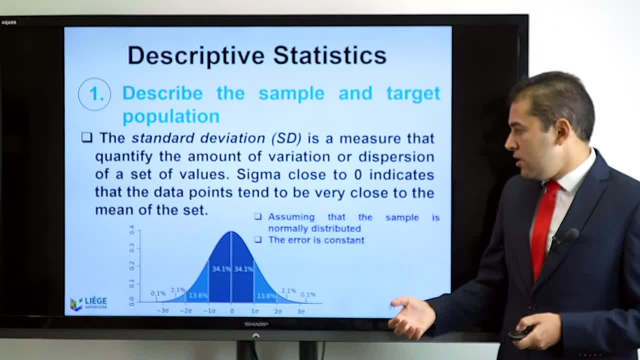 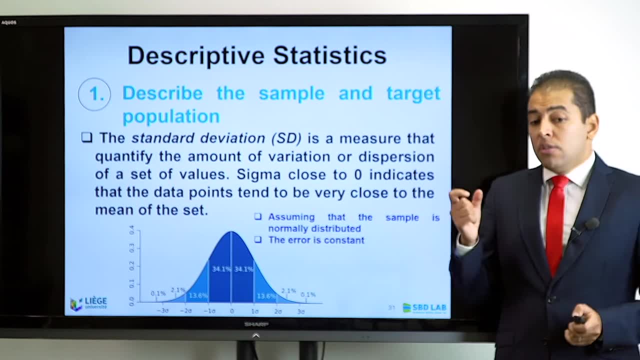 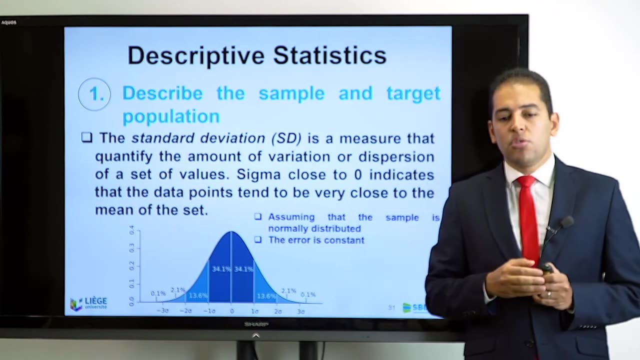 close to the means of a set. So here, as you can see, we have assumed, we are assuming that the sample is normally distributed and we have a constant error. The standard deviation test is one of the most common tests that we use to test the distribution and check if this sample is normally distributed or not. 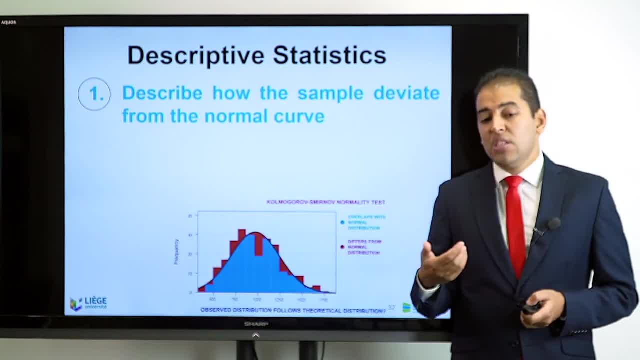 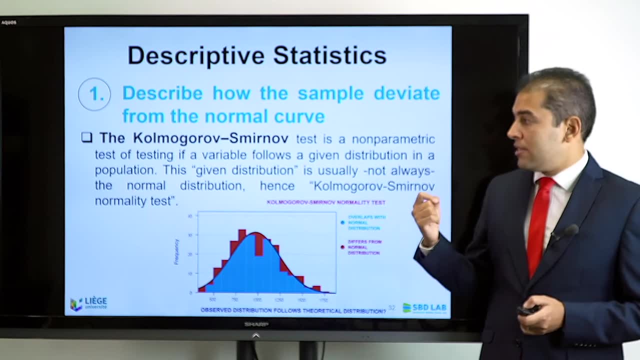 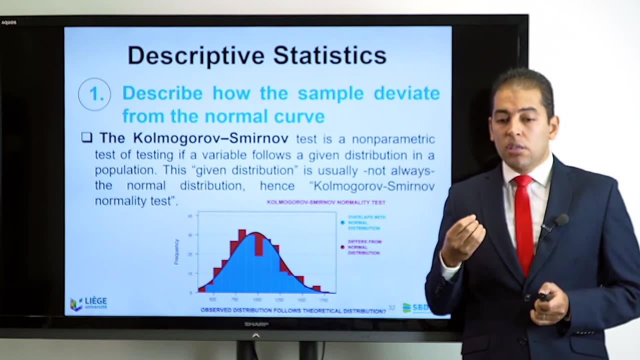 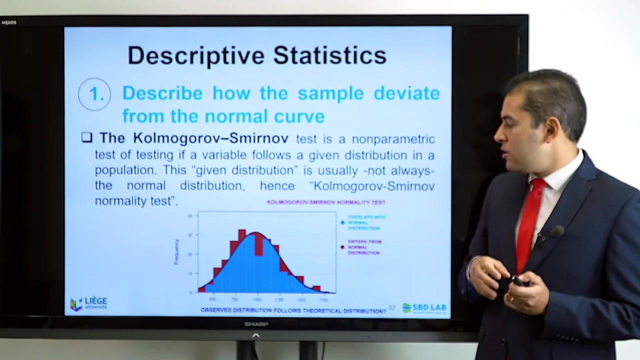 Another very common test that is used to describe a sample is called the Kolmogorov-Smirnov test. It is a non-parametric test of testing if a variable follows a given distribution in a population and this given distribution is usually not- not always- the normal distribution, hence the Kolmogorov-Smirnov normality. 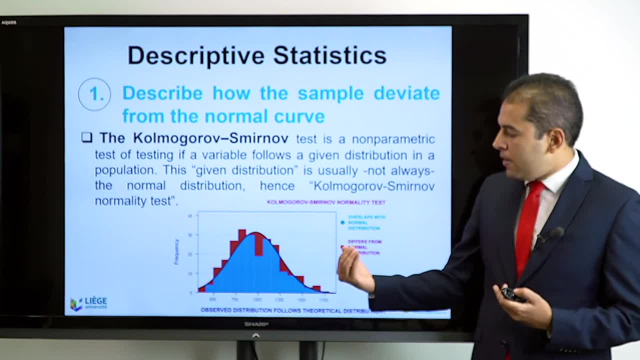 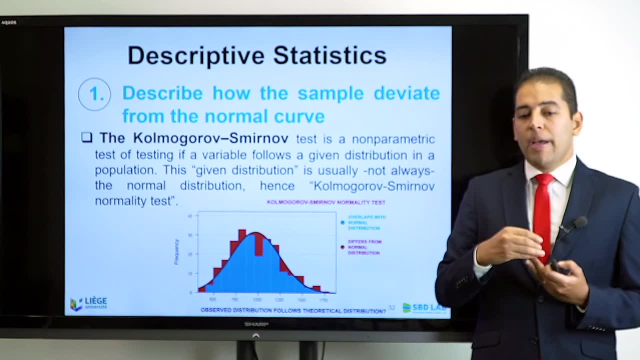 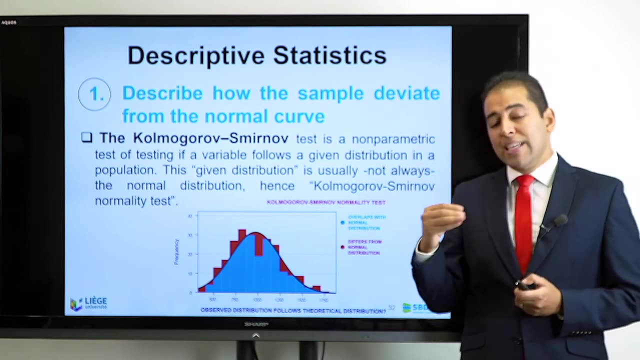 test, And here I can visualize it and I can through juxtaposition characterize how far is my sample normally distributed or not, and if there is variance or between a standard distribution or not. So this is the second test that can be conducted in the field of describing the 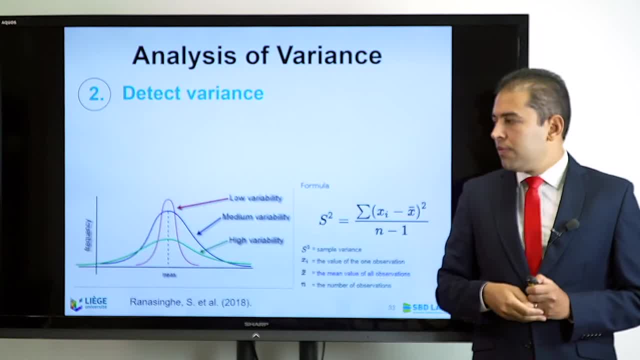 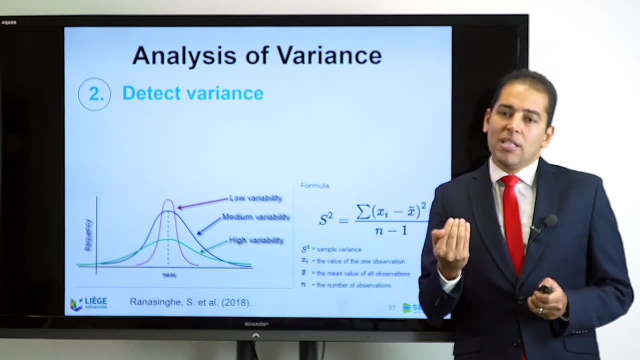 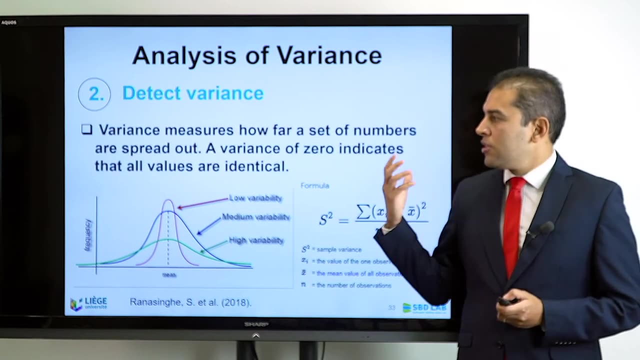 statistics. Now, moving to the second type of statistical analysis that I conduct, the statistical analysis that is seeking to detect variance. and in this sense, if I'm detecting variance, most probably, I have introduced, in this sense, a treatment And the most common way to do that. what? 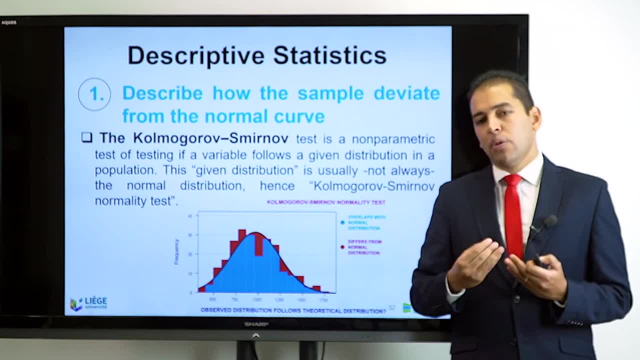 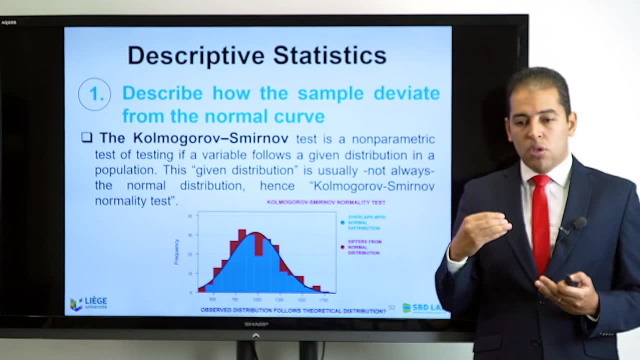 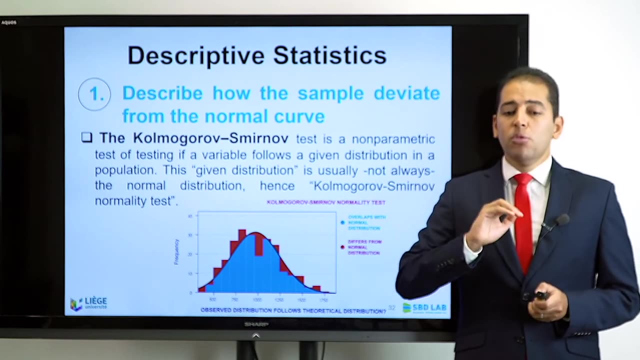 characterize how far is my sample normally distributed And if there is variance between a standard distribution or not. So this is the second test that can be conducted in the field of describing the statistics. Now, moving to the second type of statistical analysis that I conduct, 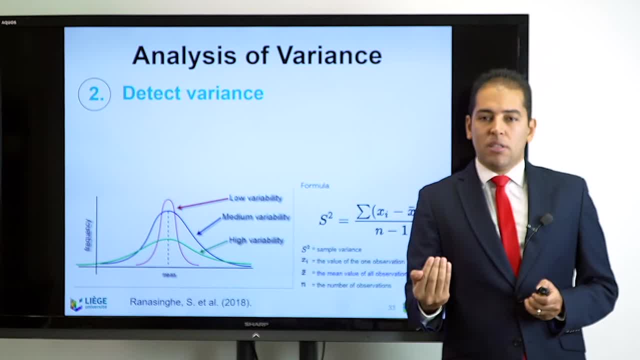 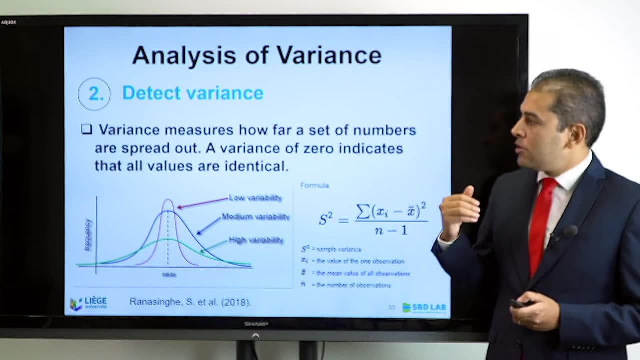 the statistical analysis that is seeking to detect variance. And in this sense, if I'm detecting variance, most probably I have introduced in this sense a treatment And the most common way to do that. what is variance? Variance measures how far a set of numbers are spread out. 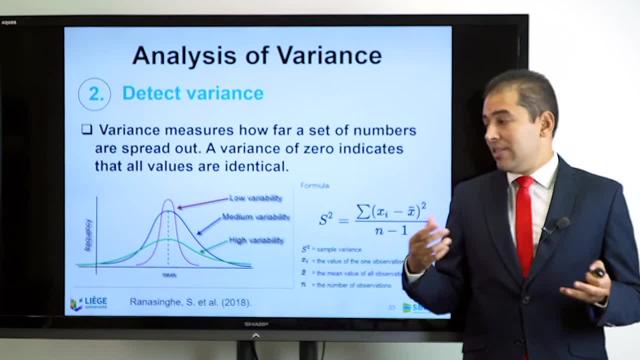 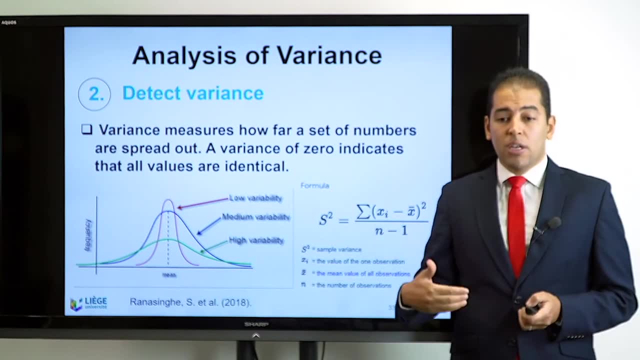 So a variance of zero indicates that all values are identical, And here we look at high variability, medium variability, low variability And based on this formula we can go detect the variance between two groups of samples And if this variance is significant. 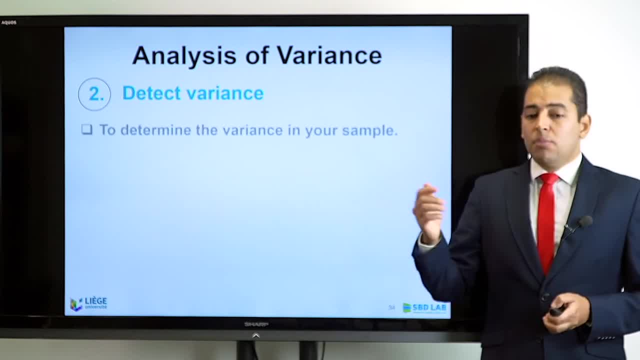 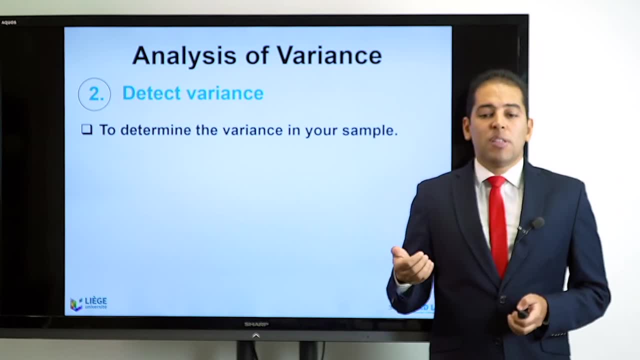 then we can go proceed with the next step. But let me rebuild on what I'm talking here. rebuild on the detection of variance. The aim of detection of variance is to determine the variance of your sample. And what are the most common tests that are done in this field? 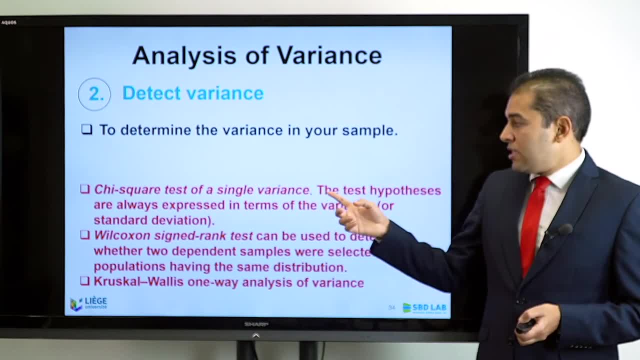 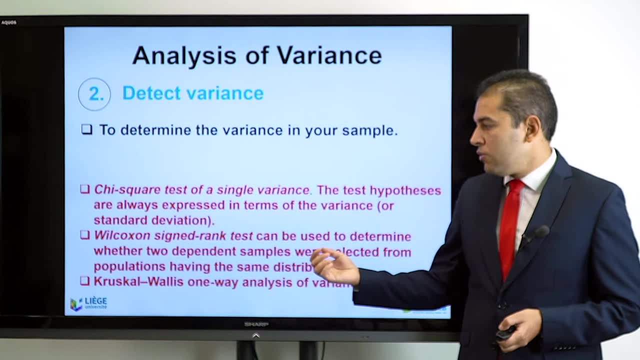 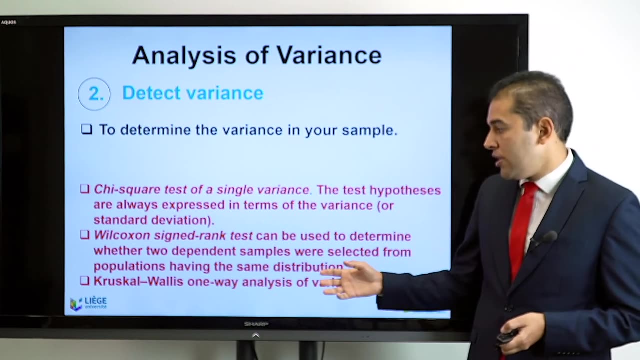 The QI2 test of single variance. This is the test hypothesis that must be always expressed in terms of variance or standard deviation. We have the Wilcoxon signed rank test that can be used to determine whether two independent variables were selected from populations having the same distribution. 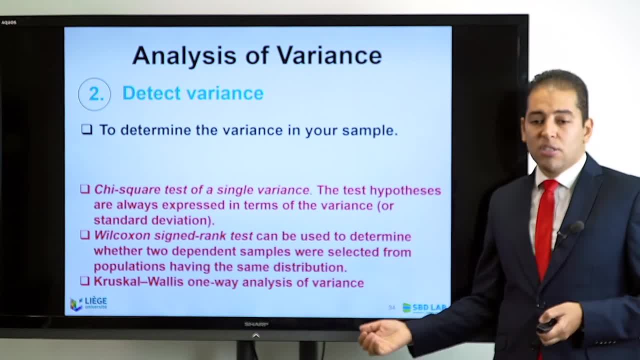 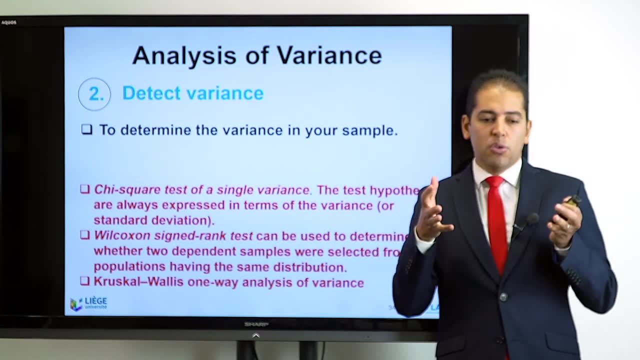 And the Krugskall-Wallis one-way analysis of variance. Those are the most common tests that are used to check the variance And in this sense, you know that you have in your experimental setting a subject with intervention, a subject without intervention. 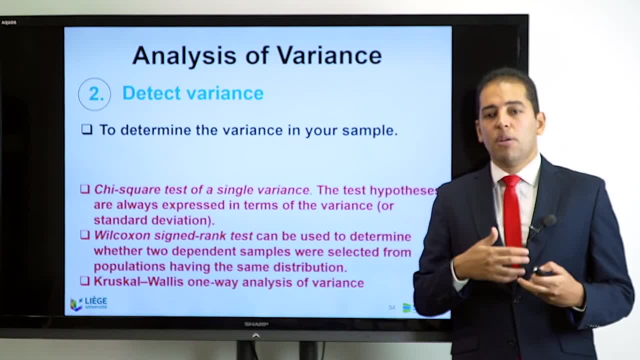 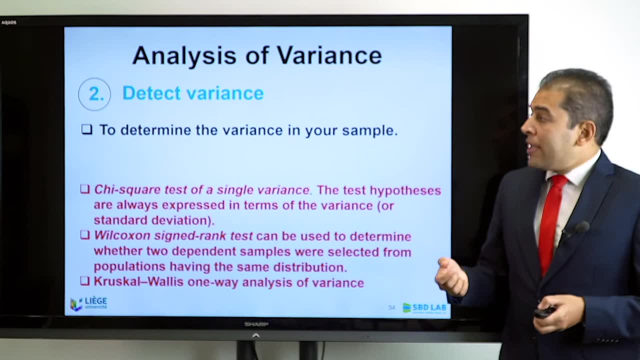 And then you conduct these tests on the results, after repeating them, after having the different randomization effects, And then you start to prove your variance. Also, following up on the detection of variance, you can look at the ANOVA test. So here we look at it's a statistical method. 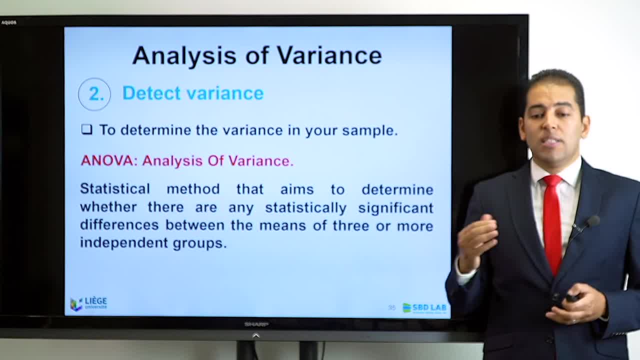 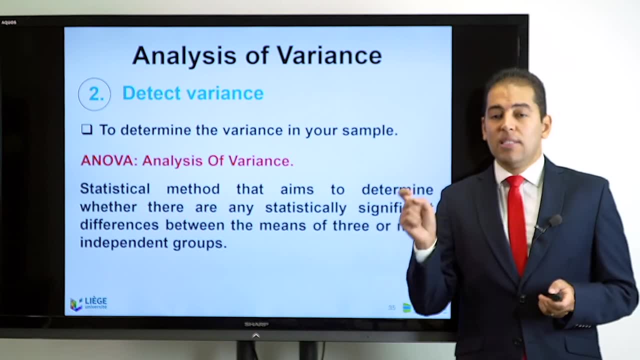 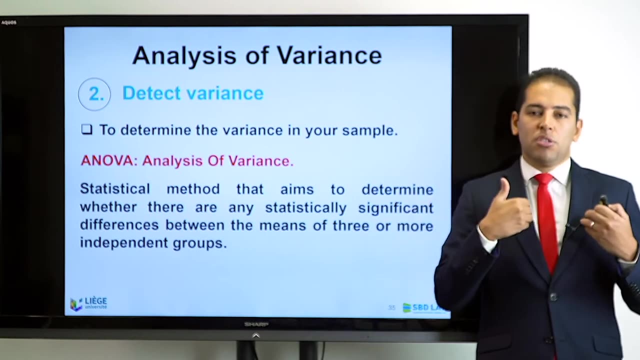 that aims to determine whether there are any statistical significant difference between the means of three or more independent groups. And it's a very famous test And again, it is the key to proceed with your statistical testing. If you cannot prove variance, then you cannot prove that your treatment or your intervention. 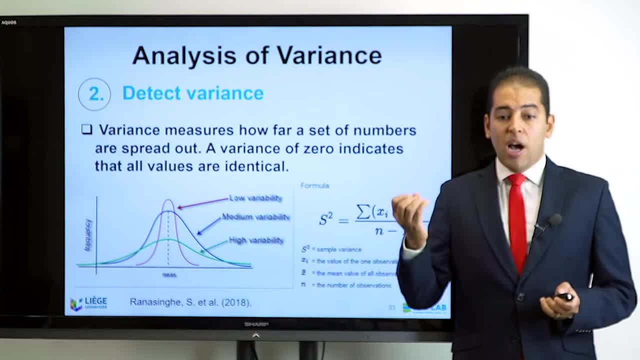 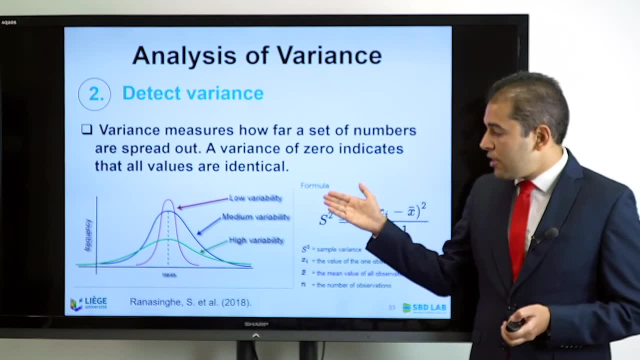 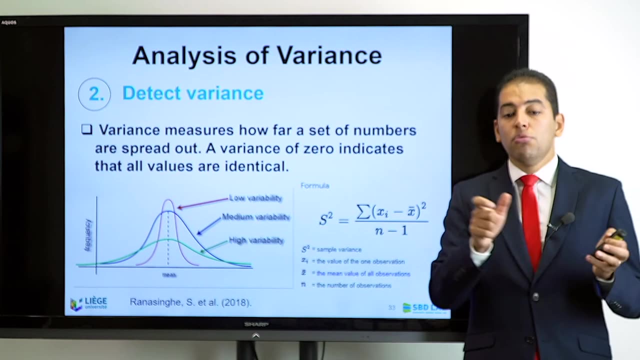 is variance. Variance measures how far a set of numbers are spread out. So a variance of zero indicates that all values are identical. and here we look at high variability, medium variability, low variability and based on this formula we can go detect the variance between two groups of samples and if this variance 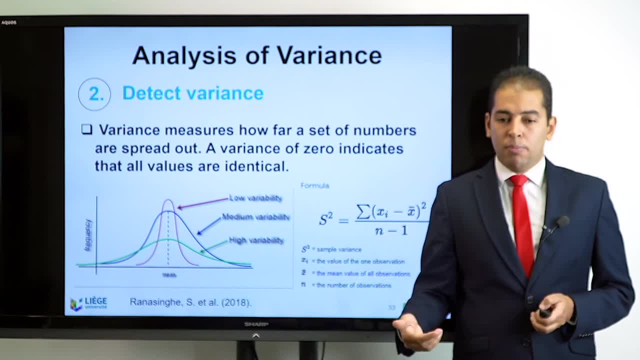 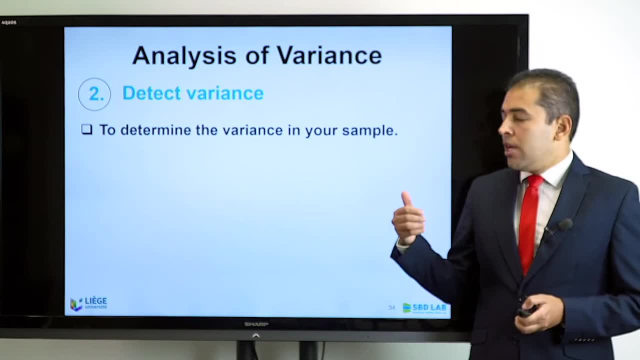 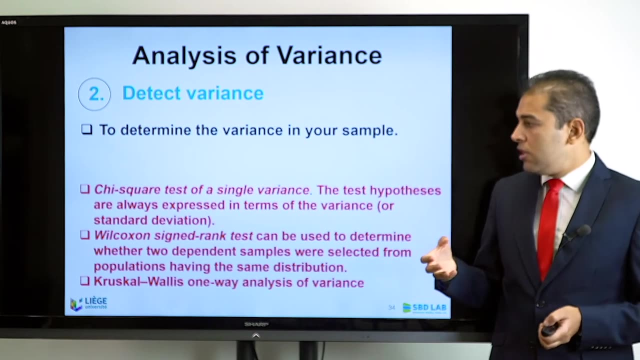 is significant, then we can go proceed with the next step. But let me build on what I'm talking here. rebuild on the detection of variance. The aim of detection of variance is to determine the variance of your sample. And what are the most common tests that are done in this field? The qui-square test of single. 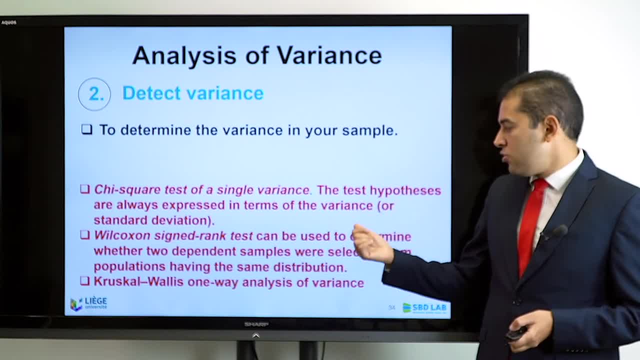 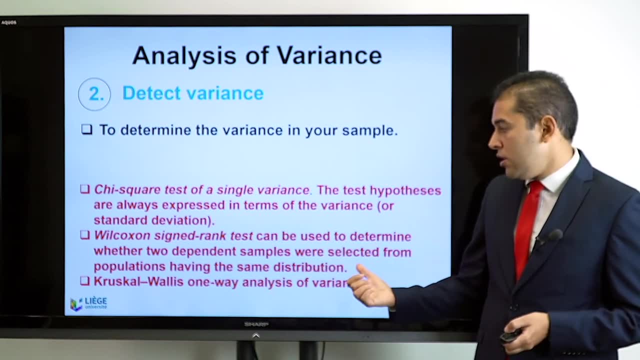 variance. This is the test hypothesis that must be always expressed in term of variance or standard deviation. We have the Wilcoxon signed rank test that can be used to determine whether two independent variables were selected from populations having the same distribution, and the Krugskall-Wallis one-way 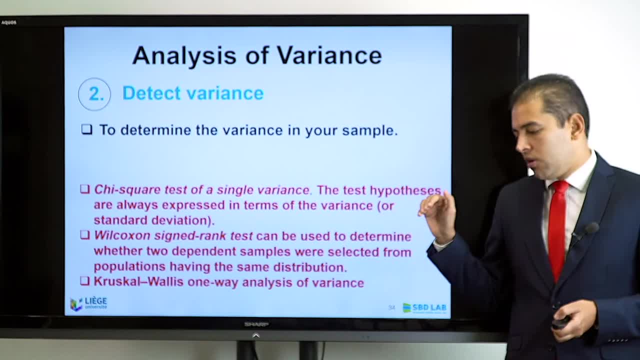 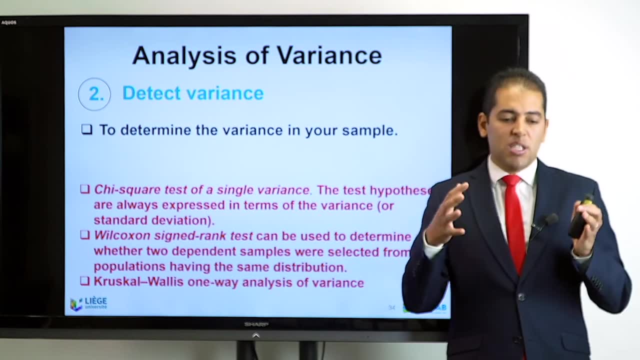 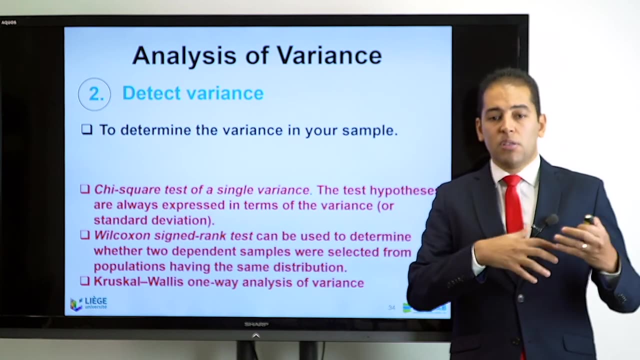 analysis of variance. Those are the most common tests that are used to check the variance and in this sense, you know that you have in your experimental setting a subject with intervention, a subject without intervention, and then you conduct these tests on the results, after repeating them, after having the 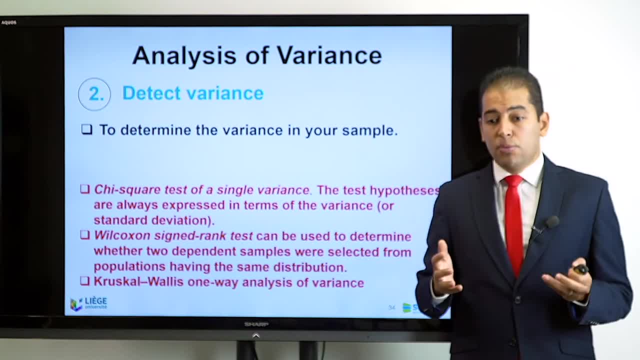 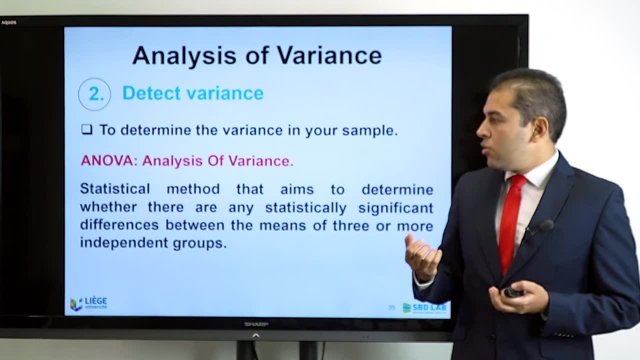 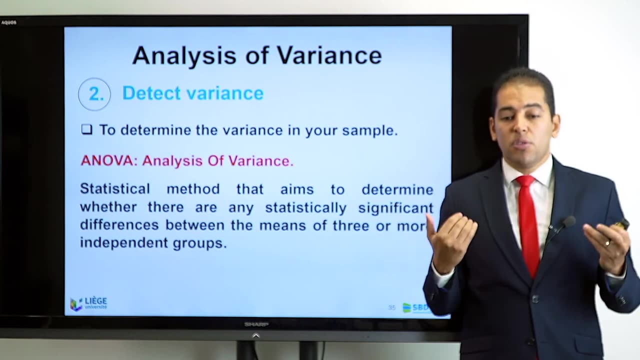 different randomization effects and then you start to prove your variance. Also, following up on the detection of variance, you can look at the ANOVA test. So here we look at that. it's a statistical method that aims to determine whether there are any statistical significant difference between the means. 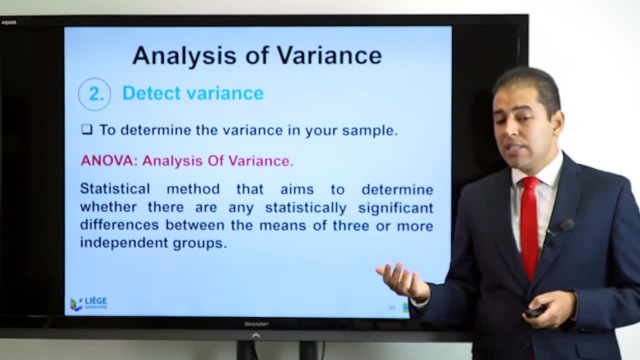 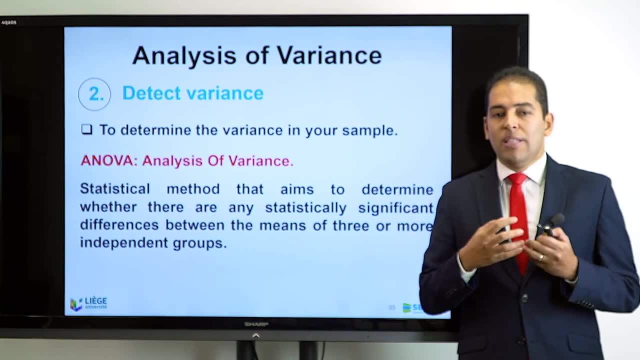 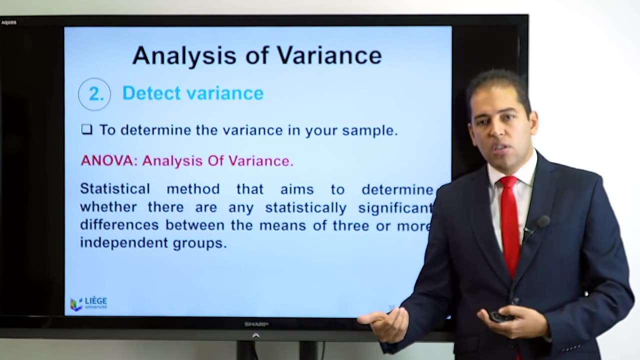 of three or more independent groups and it's a very famous test. and again, it is the key to proceed with your statistical testing. If you cannot prove variance, then you cannot prove that your treatment or your intervention has a significant effect on the results, Or whether they are improvement or getting worse, negative or positive. So 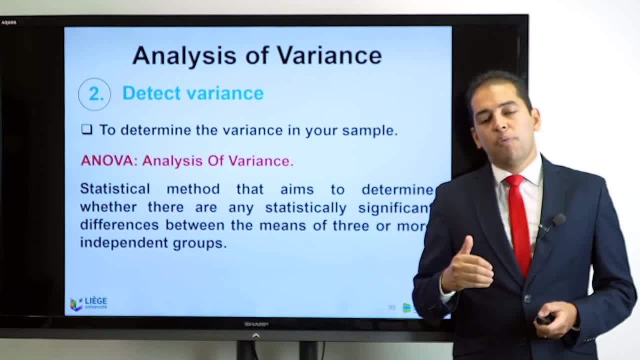 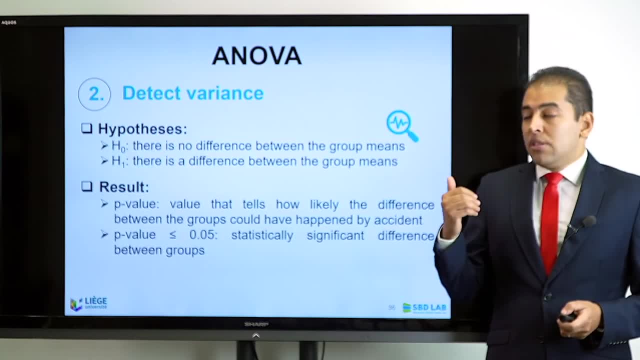 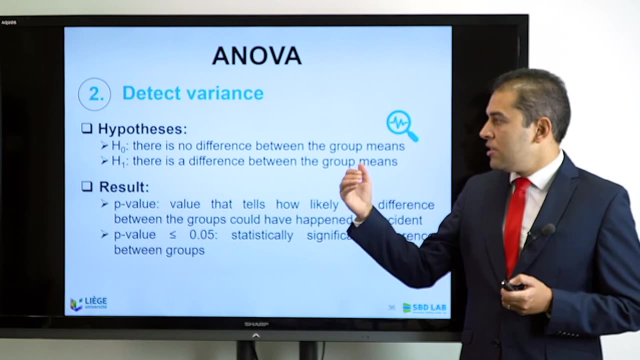 also, the ANOVA test is the second type of statistical analysis we do after the description. Still, I am talking about the detection of variance, the ANOVA test. simply, I will have always two hypotheses: The hypothesis zero, which is there is no difference between the group means and the H1 or the 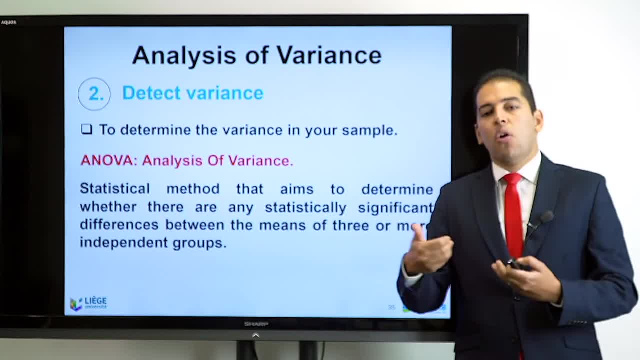 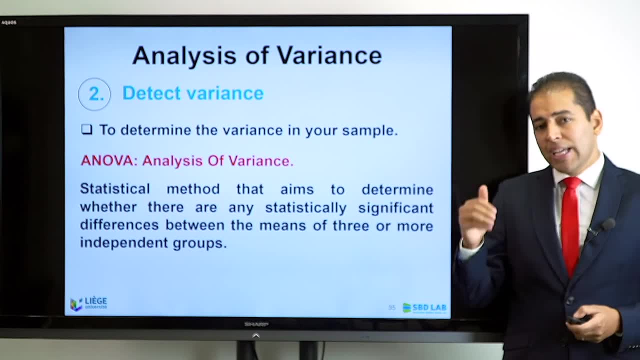 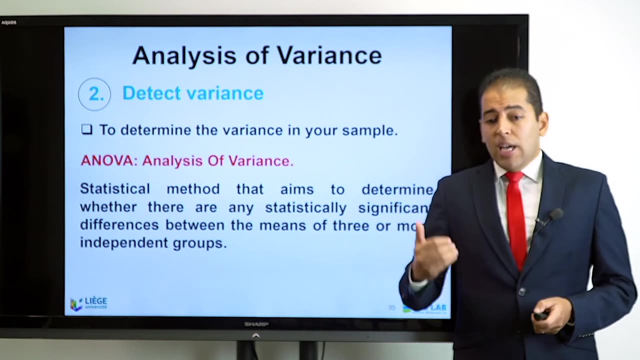 has a significant effect on the results or whether they are improvement or getting worse, Negative or positive. So also the ANOVA test is the second type of statistical analysis we do after the description. Still, I am talking about the detection of variance. 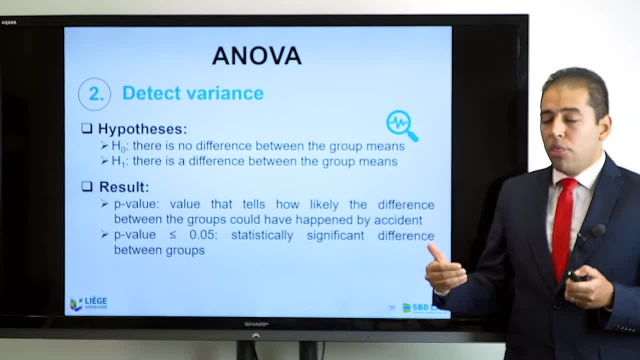 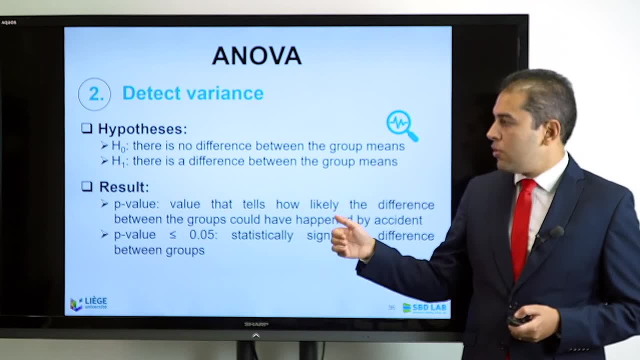 the ANOVA test. Simply, I will have always two hypotheses: The hypothesis zero, which is there is no difference between the group means, And the H1, or the hypothesis one. there is a difference between the group means And in this sense I can use the p-value. 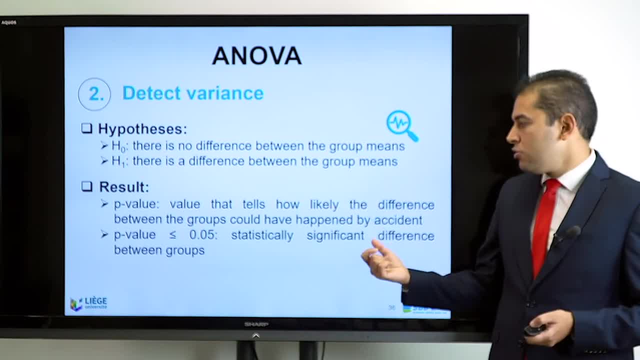 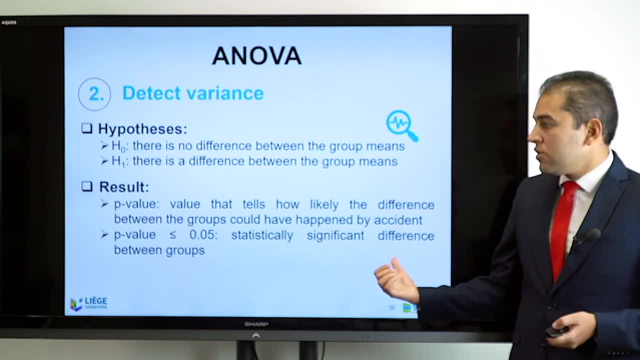 which tells me how much variance there is and how likely the difference between groups should have happened by accident, And if it's less than 0.5,, statistically significant difference between groups is proved. So this is the second approach when I do variance. 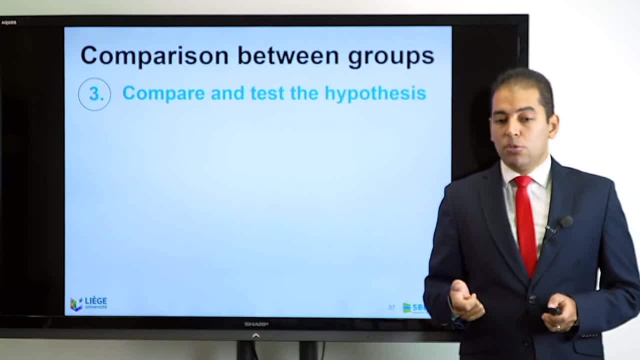 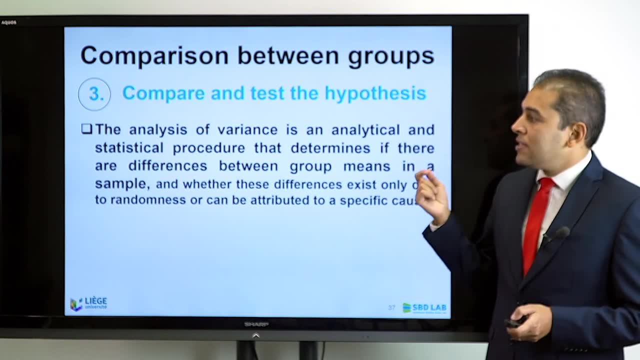 Now I will move to the third approach when I start to compare between groups, And this is called the comparing and testing, the hypothesis approach. And here we are looking at the analysis of variance as an analytical and statistical procedure to determine if there are differences between groups. 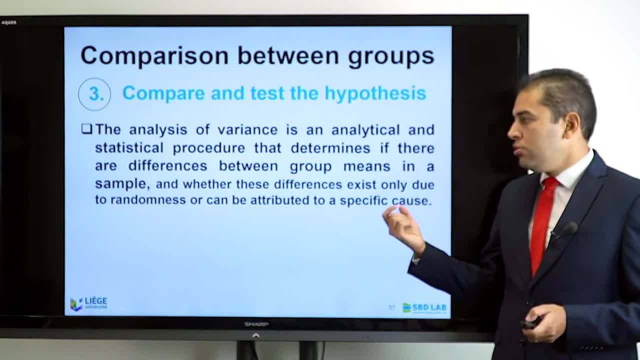 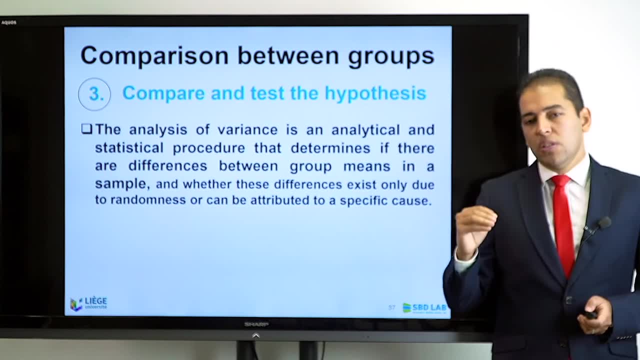 means in a sample, and whether these differences exist only due to randomness or can be attributed to a specific cause. Here the level of complexity and certainty- the certainty- is getting higher, because I am looking also to causation. And what are the most common tests. 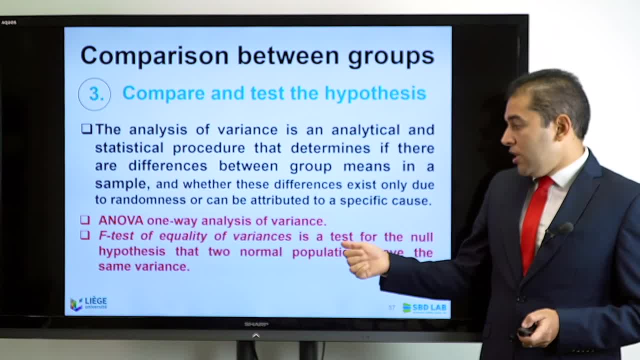 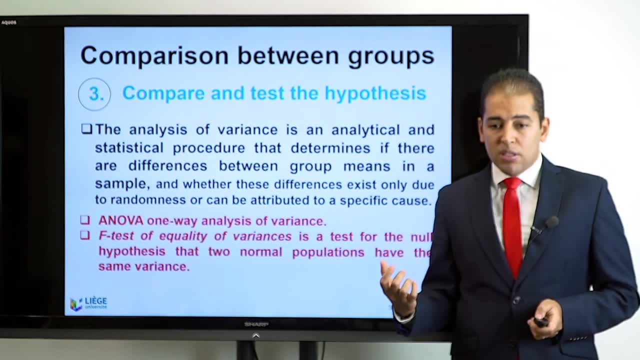 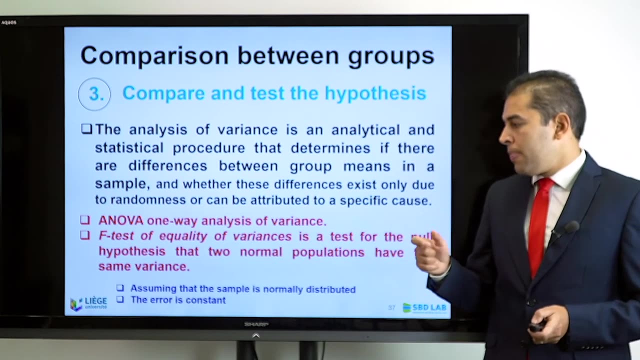 The one-way and the two-way ANOVA. The F-test of equality of variance is also used to test the null hypothesis that two normal populations have the same variance. So this is important when I start to look at comparison and refute or confirm or deny a hypothesis. 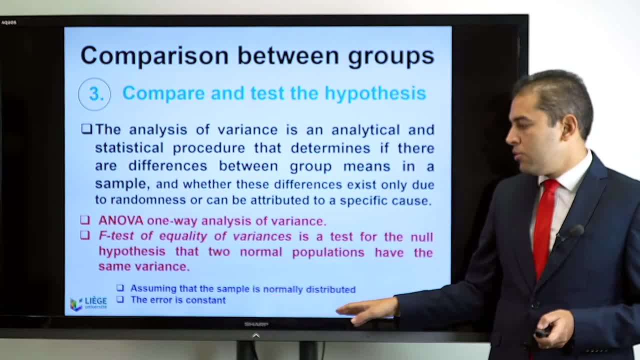 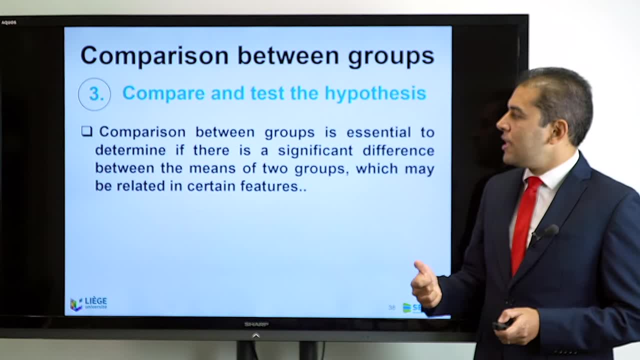 So always we are assuming here that the sample is normally distributed and that the error is constant, because if it's not, we have different type of testings. Now comparing, also the testing Comparison between groups is essential to determine if there is a significant difference. 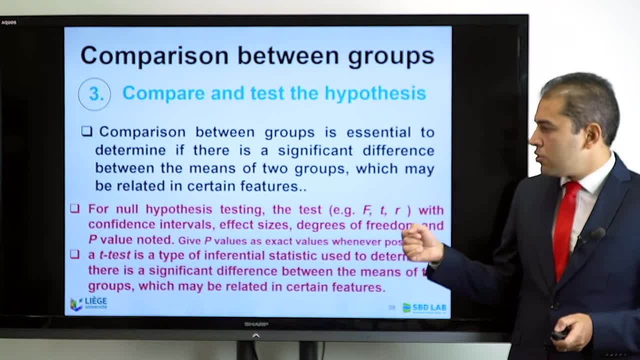 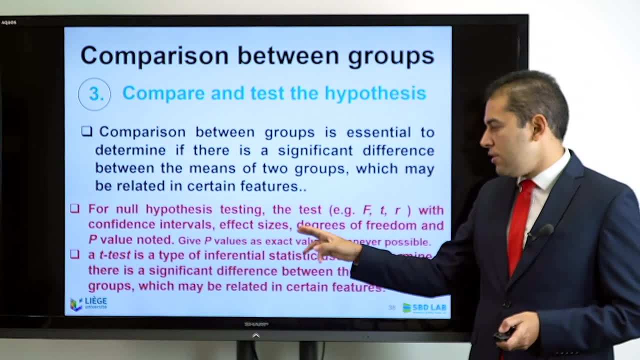 But the other type of test that can be used in this approach is the null hypothesis we mentioned. We can have the F and the T and the R test With confidence intervals, effect size, degrees of freedom and p-value noted, And we can have also the T test. 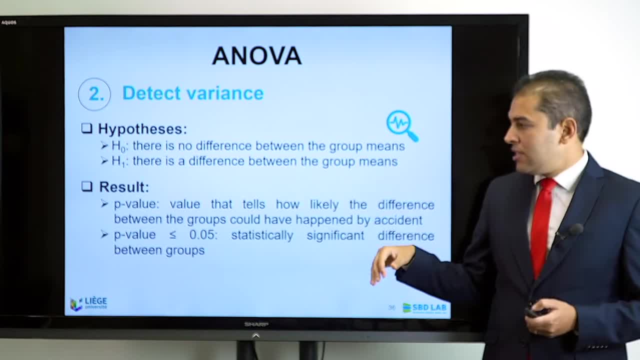 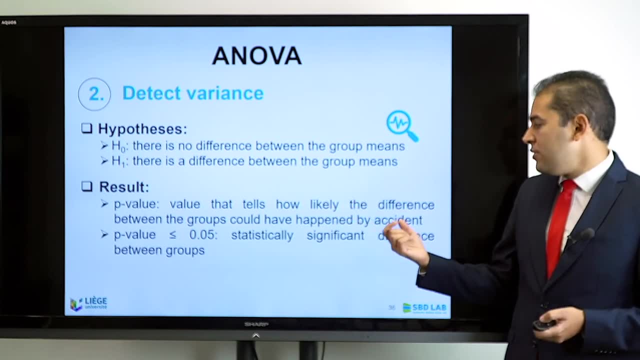 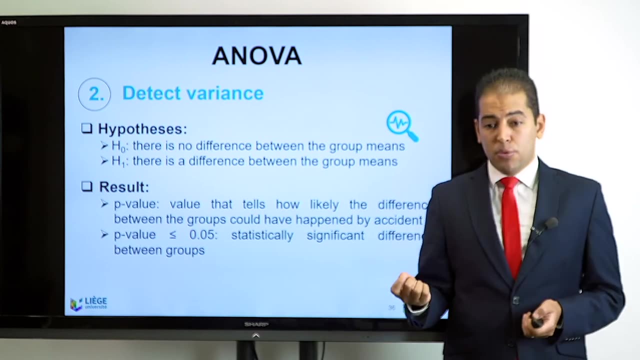 hypothesis one, there is a difference between the group means- and in this sense I can use the p-value, which is which tell me how likely the difference between groups should have happened by accident, and if it's less than 0.5, statistically significant difference between groups is proved. So this is the 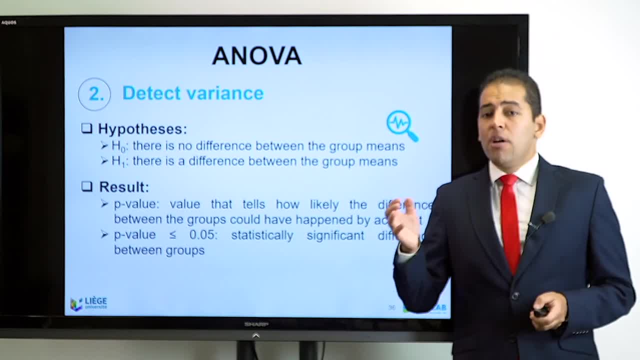 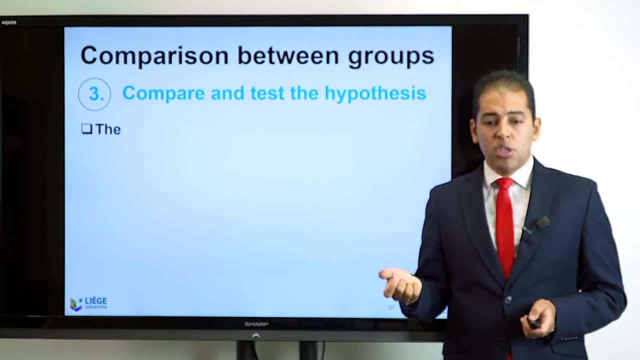 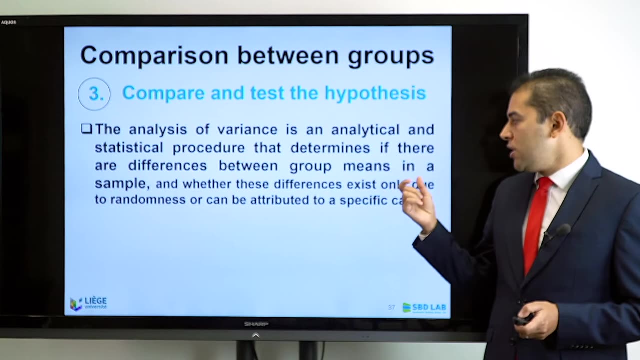 second approach, when I do variance. Now I will move to the third approach, when I start to compare between groups, and this is called the comparing and testing, the hypothesis approach. and here we are looking at the analysis of variance as an analytical and statistical procedure To determine if there are differences between group means in a sample and 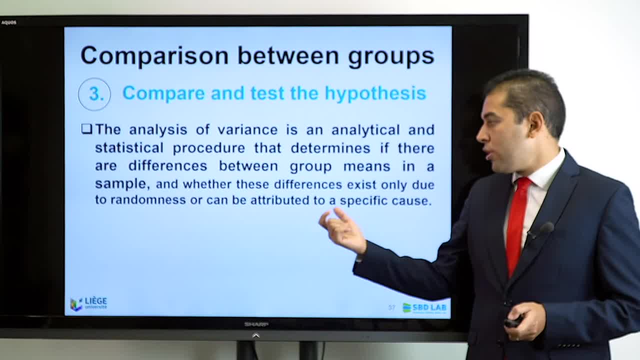 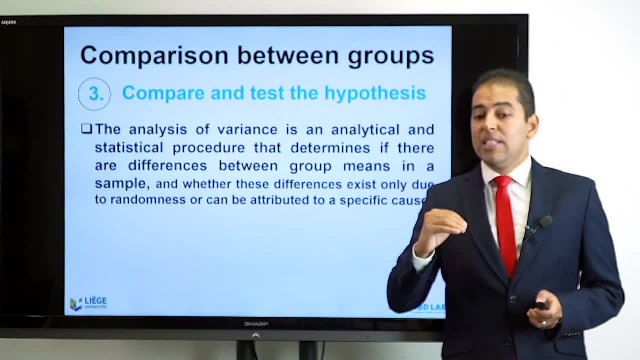 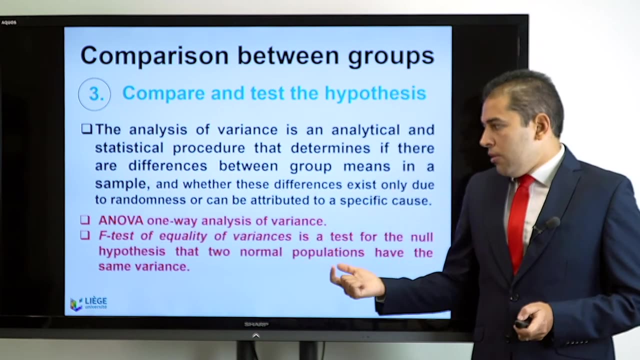 whether these differences exist only due to randomness or can be attributed to a specific cause. Here the level of complexity and certainty- the certainty is getting higher because I'm looking also to causation. And what are the most common tests? The one-way and the two-way ANOVA, The F-test of equality of 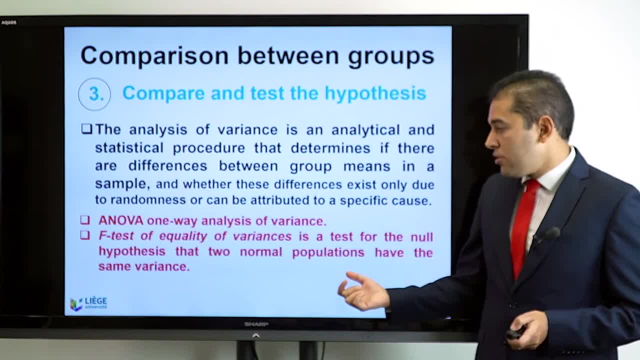 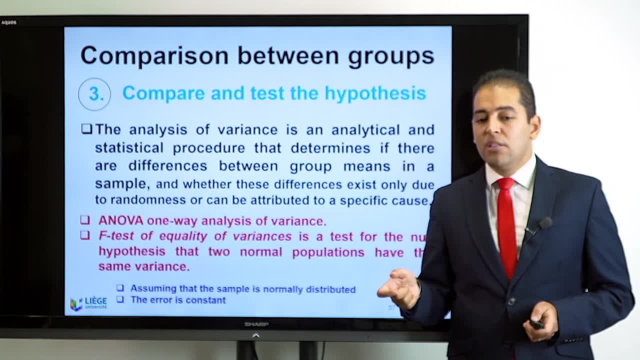 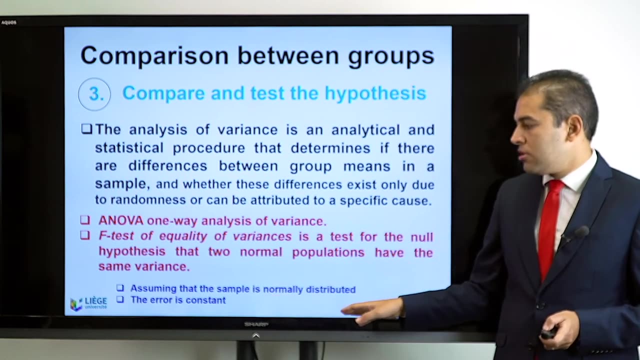 variance is also used to test the null hypothesis that two normal population have the same variance. So this is important when I start to look at comparison and refute or confirm or deny a hypothesis. So always we are assuming here that the sample is normally distributed and that the error is. 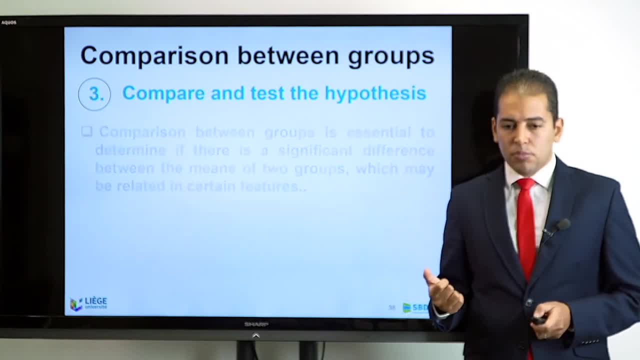 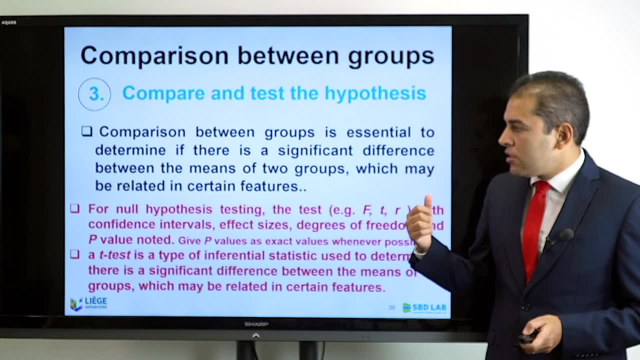 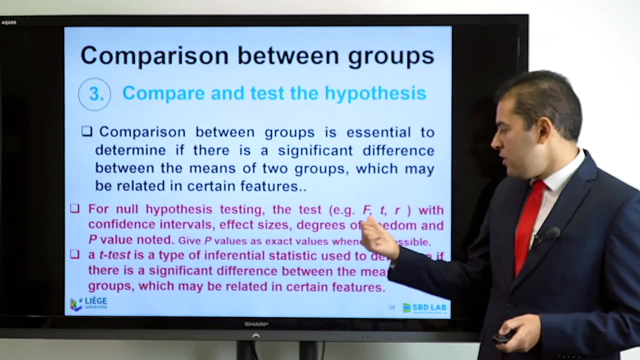 constant, because if it not, we have different type of testings. Now comparing also the testing comparison between groups, is essential to determine if there is a significant difference. but the other type of test that can be used in this approach is the null hypothesis. we we can have the F and the T and R test with confidence intervals, effect size. 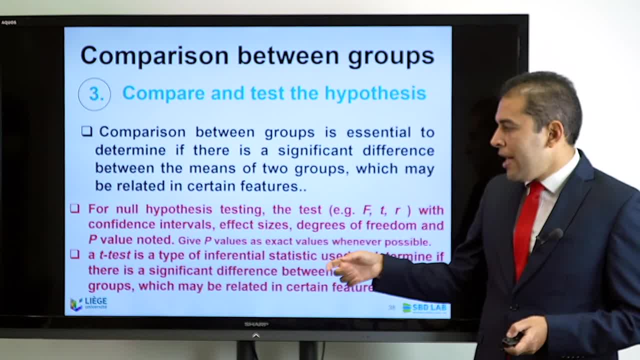 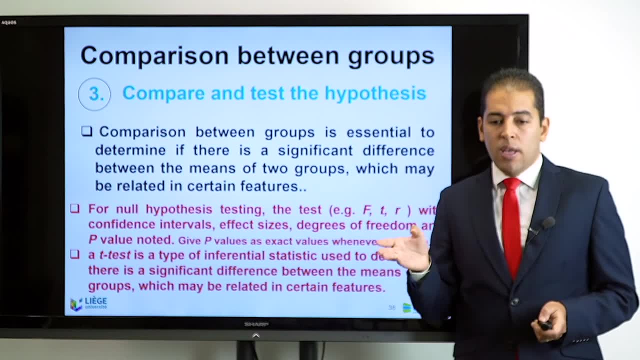 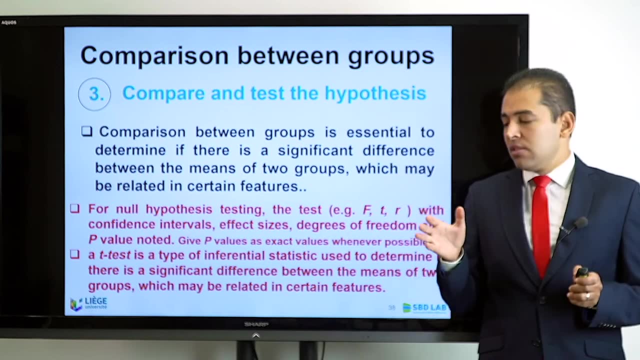 degrees of freedom and p-value noted. and we can have also the T test, which is a type of inferential statistic used to determine if there is a significant difference between the means of two groups which may be related in certain features. so here these are the reported tests that are mostly used to assure. 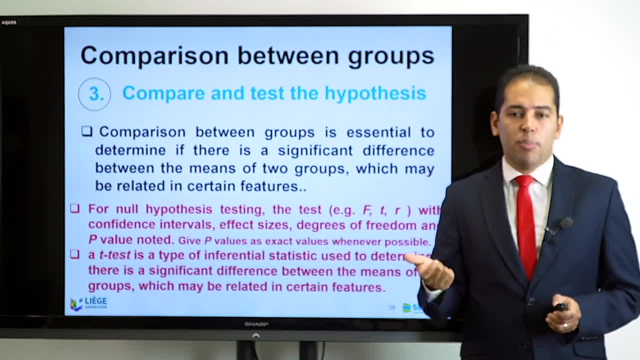 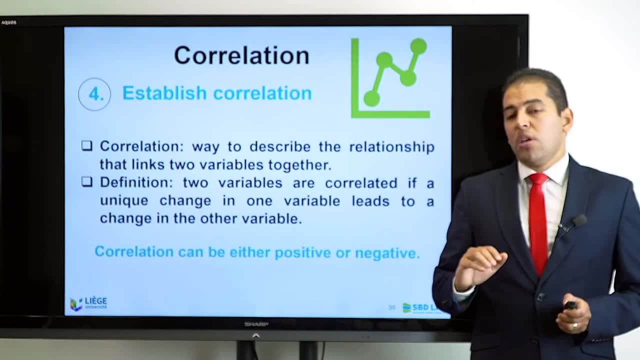 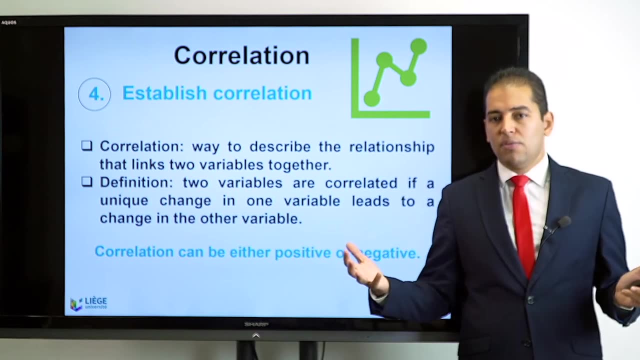 that there is a comparison that was done and that we have a positive or a null, like the hypothesis is null or the hypothesis is positive. now, moving to the fourth type of testing, if I have proved already that there is a variance and I succeeded to make sure that the groups indicate that there are variance, then I 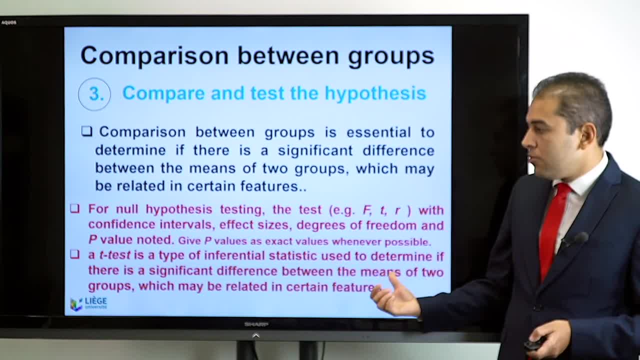 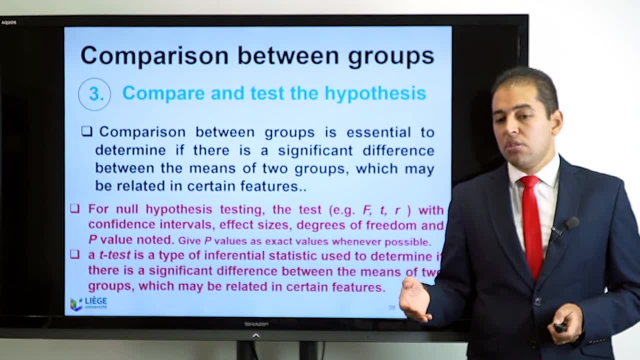 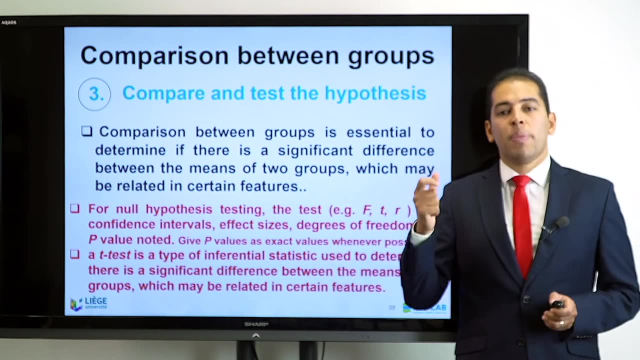 which is a type of inferential statistic used to determine if there is a significant difference between the means of two groups which may be related in certain features. So here these are the reported tests that are mostly used to assure that there is a comparison. that was done. 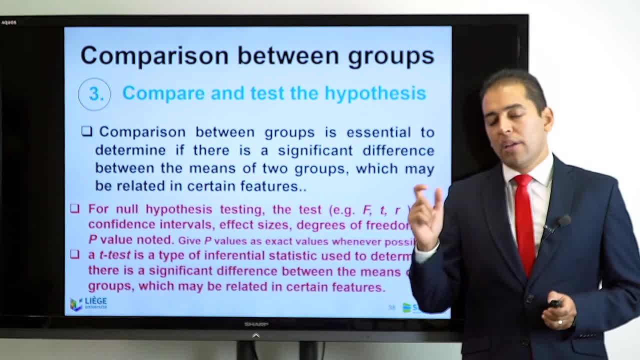 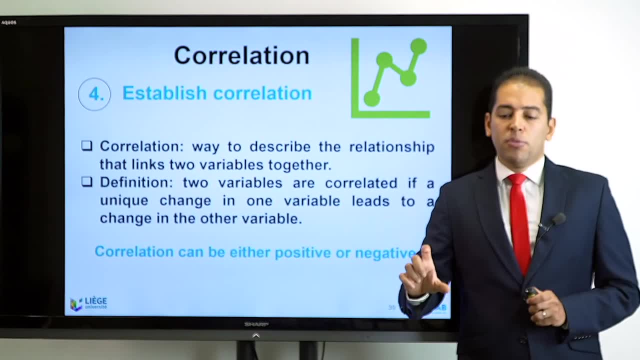 and that we have a positive or a null, like the hypothesis is null or the hypothesis is positive. Now, moving to the fourth type of testing, If I have proved already that there is a variance and I succeeded to make sure that the groups indicate that there are variants, 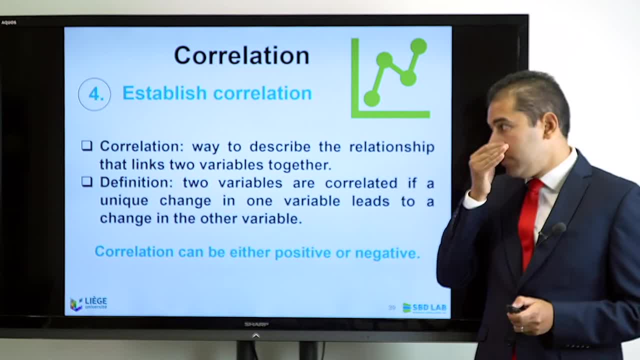 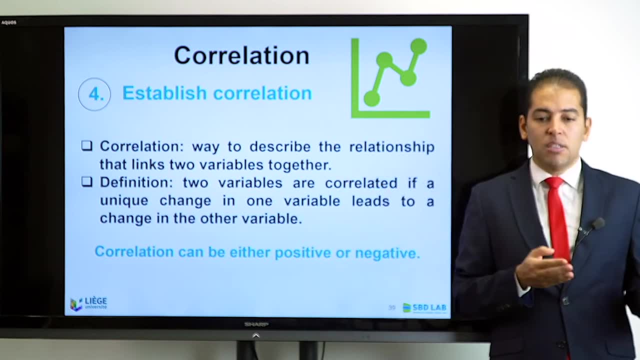 then I can move now to look at establishing correlation. What do I mean by establishing correlation? Well, correlation is a way to describe if there is a relationship that links the two variables that I am investigating And in this sense, the definition is that these two variables are correlated. 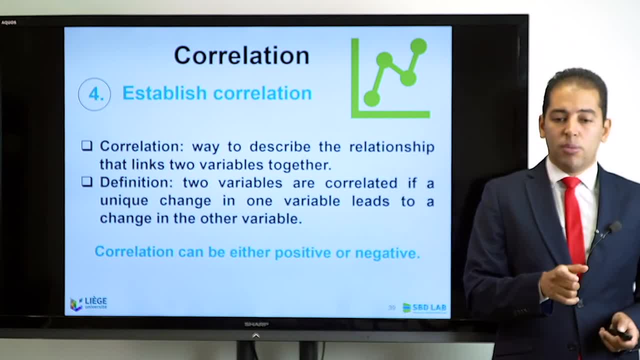 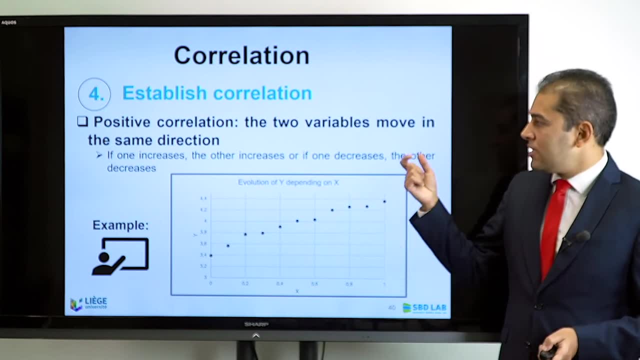 if a unique change in one variable leads to a change in the other variables. So correlation can be either positive or negative And as we look at here in this example, positive correlation- we can say that the two variables move in the same direction. 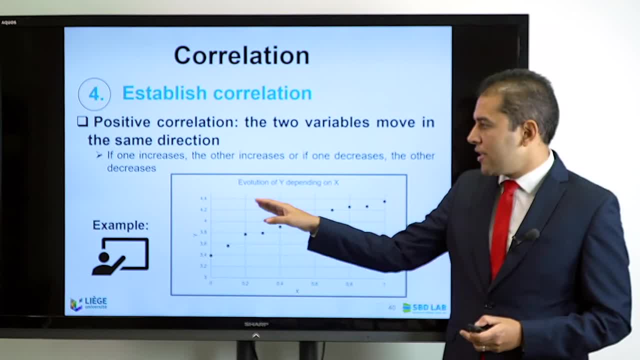 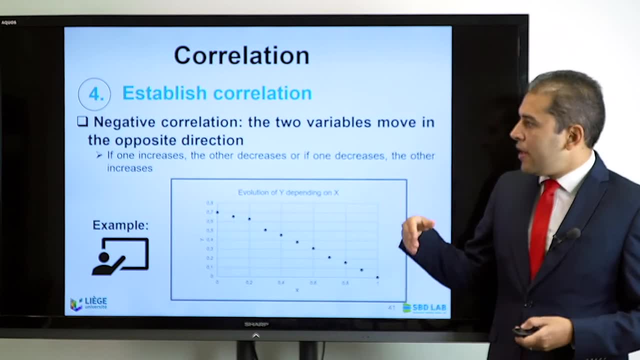 If I increase the x-axis, the y-axis will increase too. If one increases, the other increases, And if one decreases, the other decreases. And if I have a negative correlation, the two variables also move in the opposite direction, as you can see. 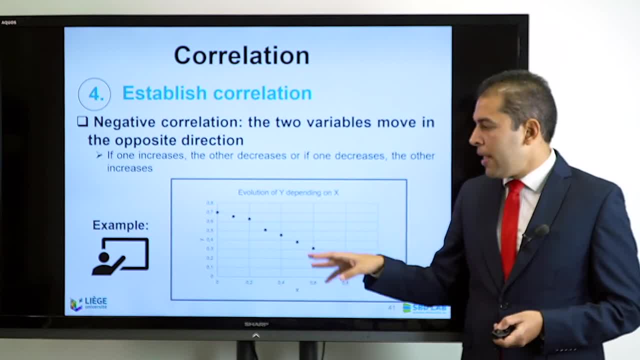 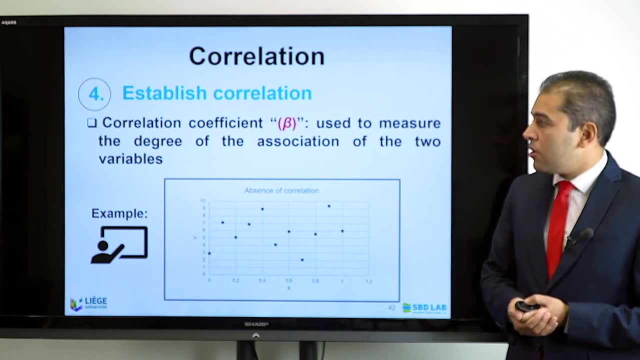 So if one increases, the other increases, If one decreases, the other increases, And this is an example. And for sure, maybe to indicate my correlation, I need to use the beta coefficient, which is used to measure the degree of the association of the two variables. 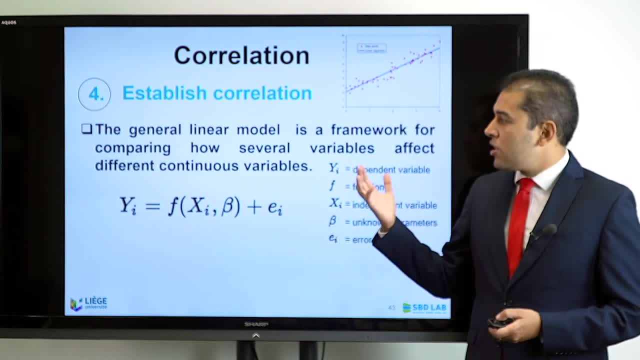 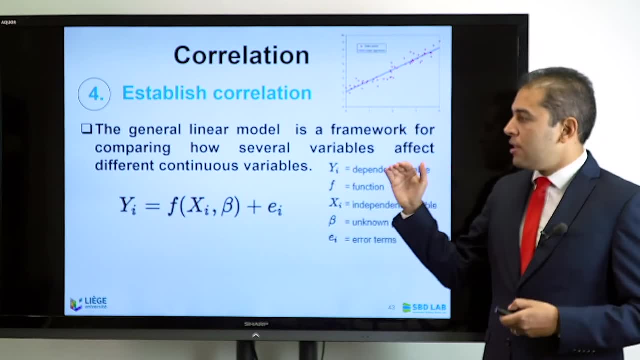 And it's a calculation, So I need to look at this. This is the general in normal. if it's a linear model, then it will be a general model, which is a framework for comparing how several variables affect how many homogeneous variables. 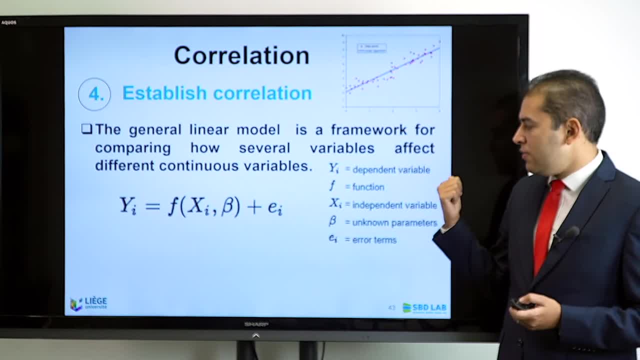 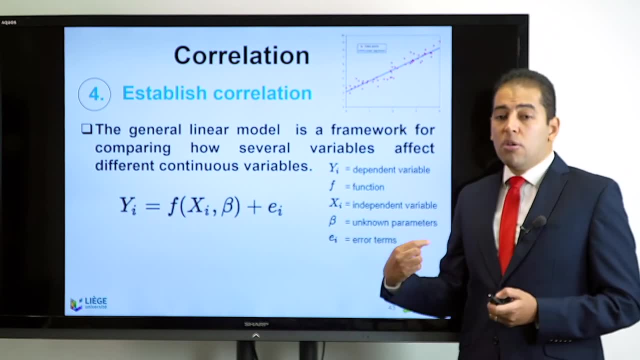 And then I can use this equation where I have the dependent variable and independent variable, Then I have a function f, And then I have the unknown parameter, the beta, And then I can also communicate my error terms, so that I make sure that I'm taking care. 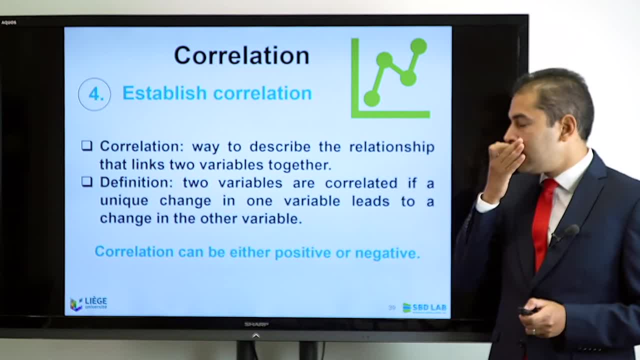 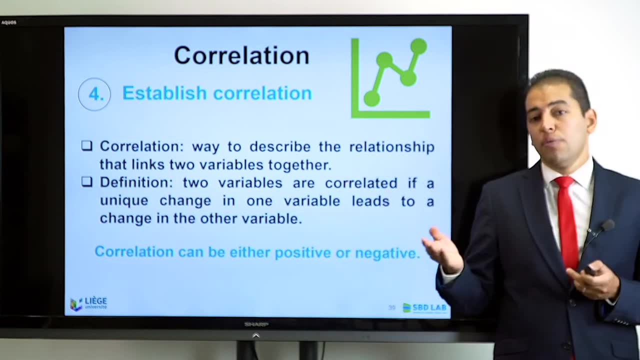 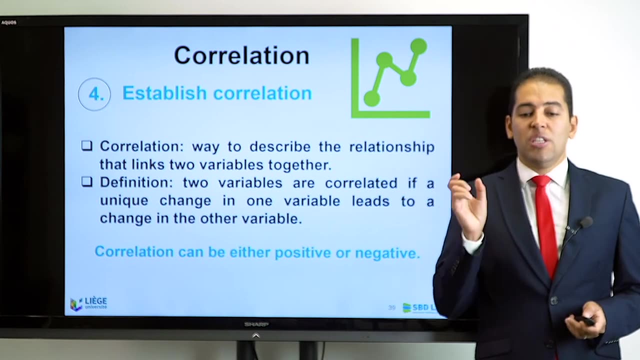 can move now to look at establishing correlation. what do I mean by establishing correlation? well, correlation way is a way to describe if there is a relationship that links the two variables that I am investigating, and in this sense the definition is: two variables are correlated if a unique change in one variable leads to a change in the other. 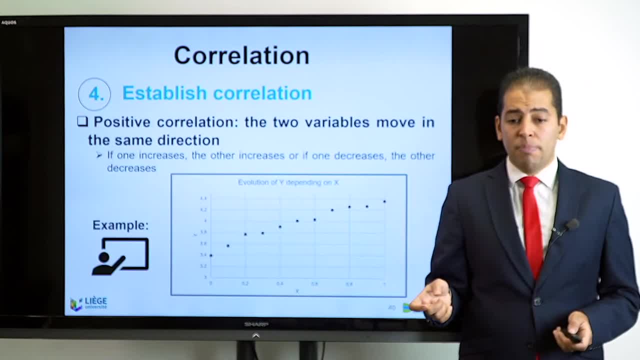 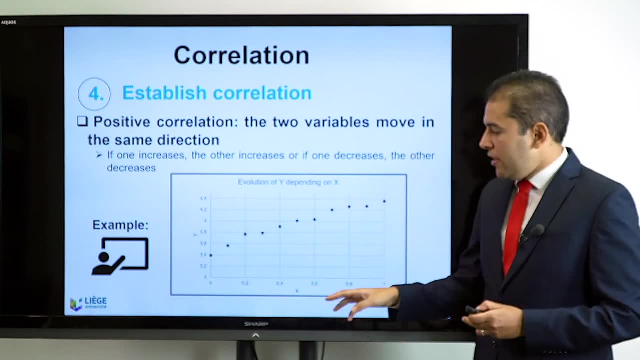 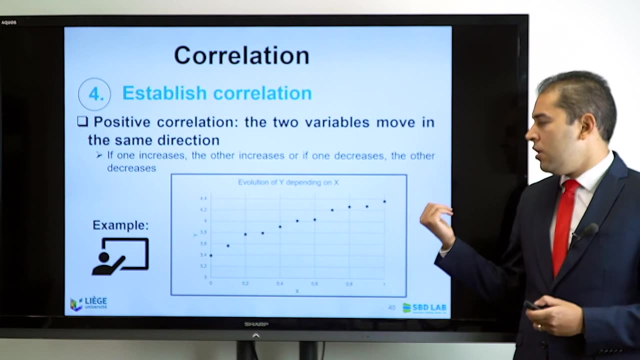 variables. so correlation can be either positive or negative and as we look at here in this example, positive correlation- we can say that the two variables move in the same direction. if I increase the x axis, that Y axis will increase to. if one increase, the other increase and if I want one, decrease the. 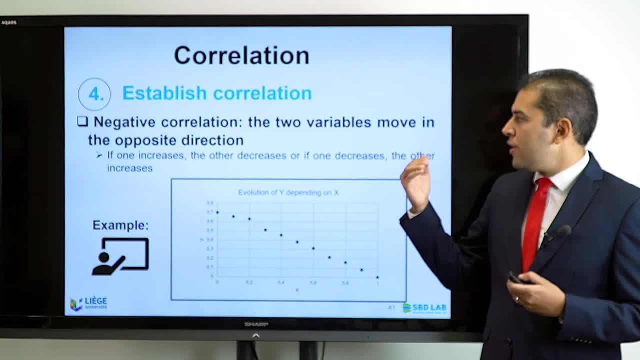 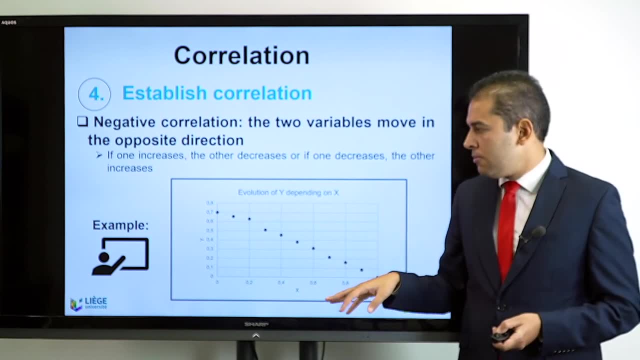 other decreases. and if I have a negative correlation, the two variables also move, but in the opposite direction, as you can see. so if one increase, the other decrease. if one decrease, the other increases. and this is an example. and for sure, maybe to indicate my correlation, I need to use 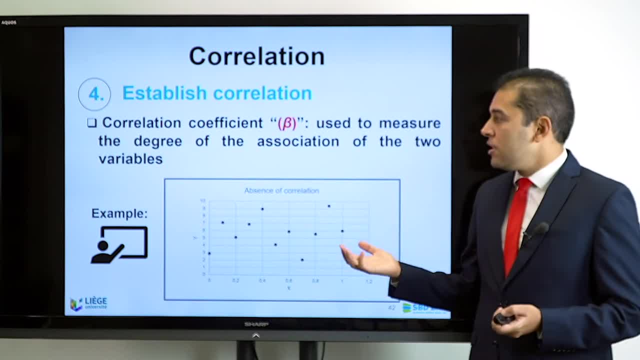 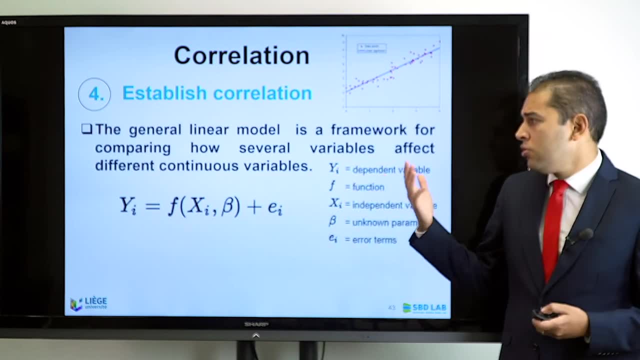 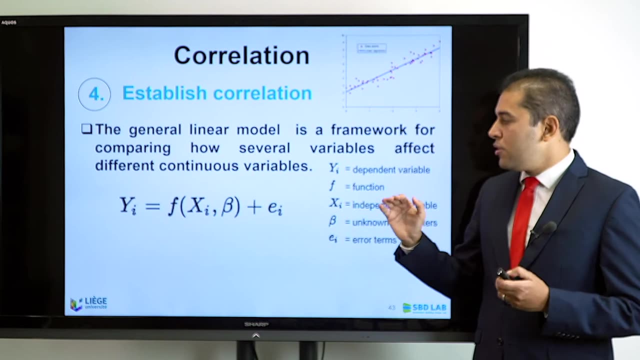 the beta coefficient, which is used to measure the degree of the association of the two variables, and it's a calculation, so I need to look at this. this is the general in normal. if it's a linear model, then it will be a general model which is a framework for comparing how several variables affect different continuous 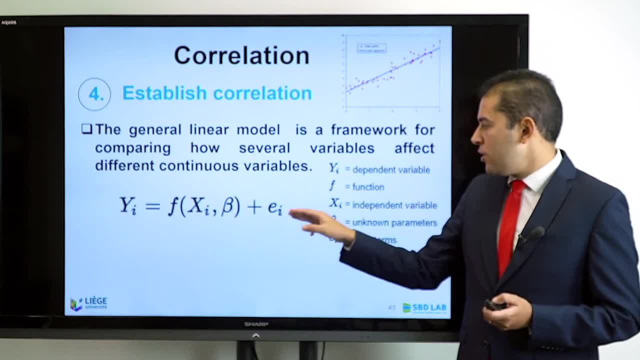 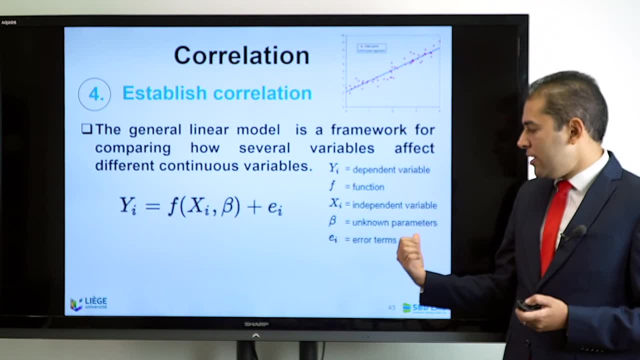 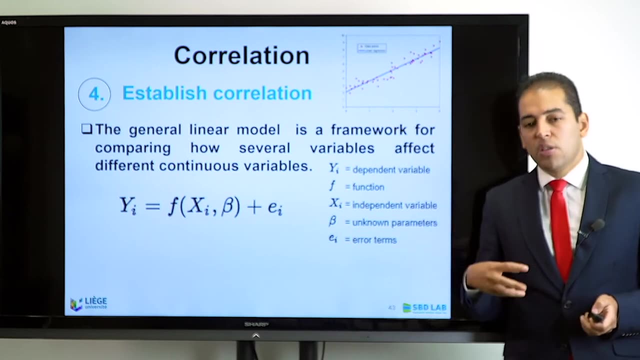 variables, and then I can use this up equation where I have a dependent variable and independent variable, then I have a function F and then I have the unknown parameter, the beta, and then I can also communicate my error terms so that I make sure that I'm taking care of the replication error and any condition. 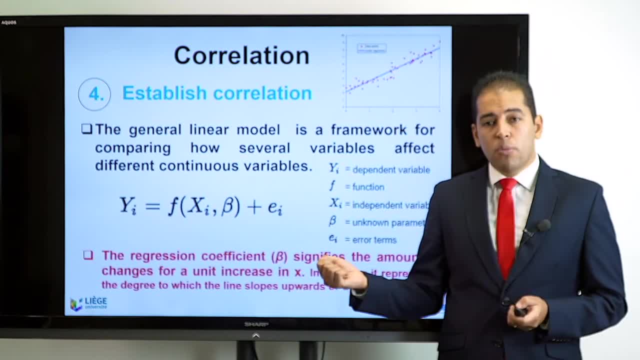 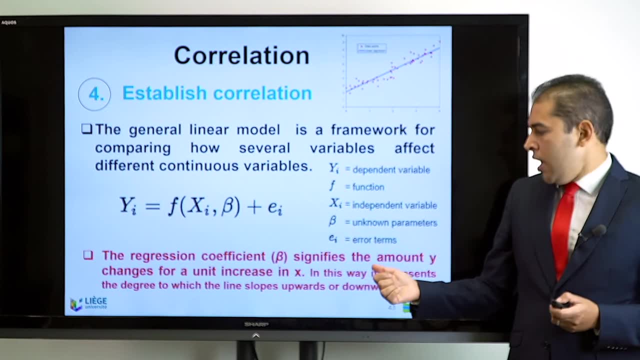 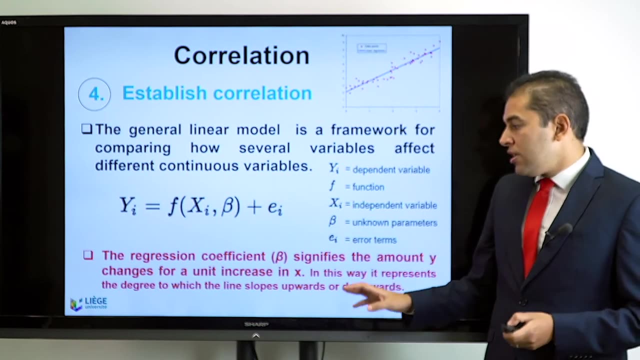 that are in the control condition and when I report this information in any protocol or in any report or any publication, I must have my regression coefficient beta. so it signifies: is the amount Y that changes for a unit increase in X, and in this way it represents the degree of which the line slopes upwards or 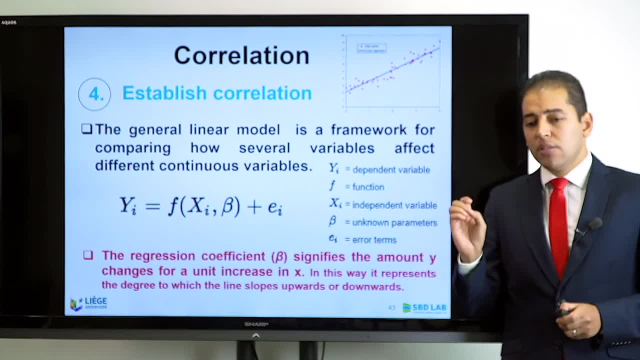 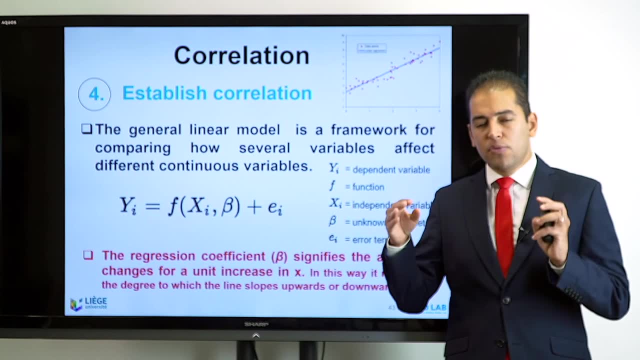 downwards. so here I am having correlation, but just take care that it that it is not a straightforward approach. it doesn't mean that I have I proved covariance in my sample that there is correlation. correlation is a correlation. but it is not a straight forward approach. it doesn't mean that I have I proved covariance in my sample that there is correlation. correlation is a. 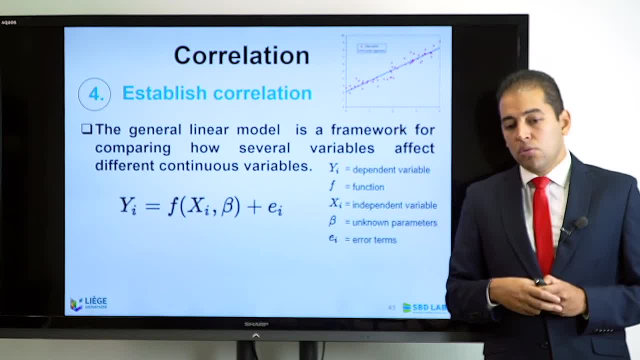 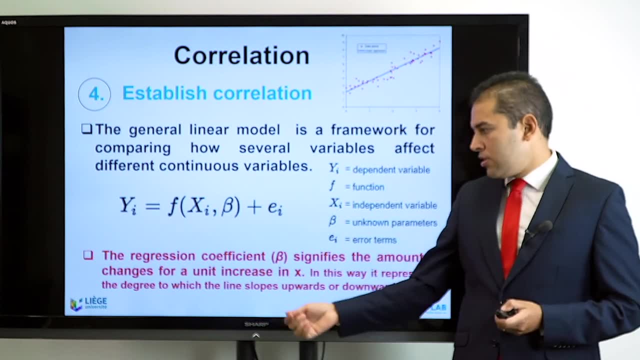 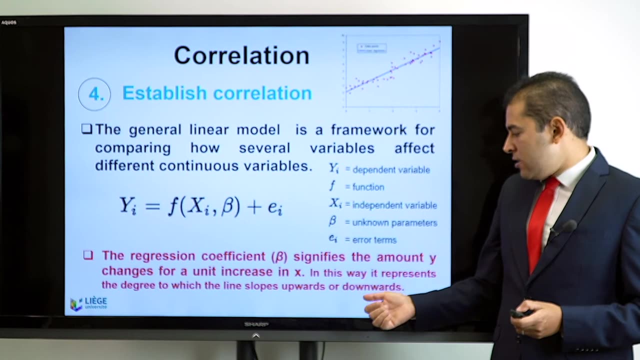 of the replication error and any condition that are in the control condition And when I report this information in any protocol or in any report or any publication, I can use my regression coefficient beta. So it signifies the amount y that changes for a unit increase in x. 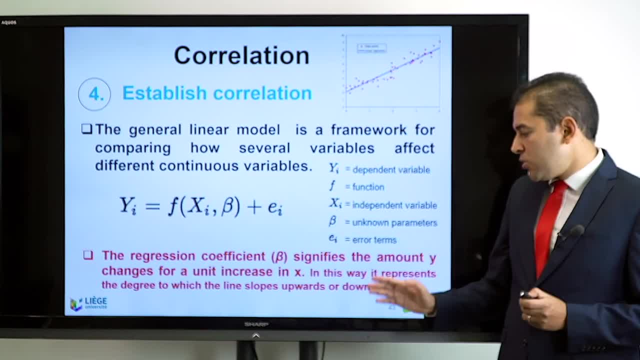 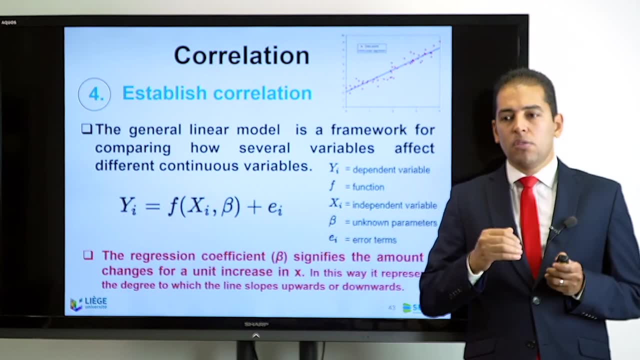 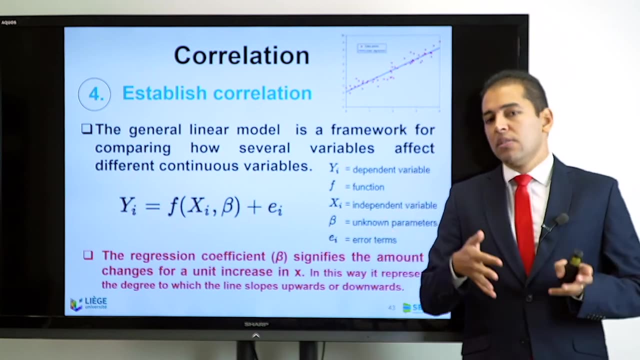 And in this way it represents the degree of which the line slopes upwards or downwards. So here I am having correlation, But just take care that it is not a straightforward approach. It doesn't mean that I proved covariance in my sample, that there is correlation. 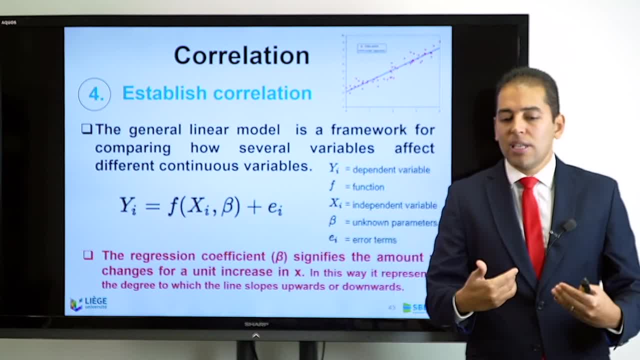 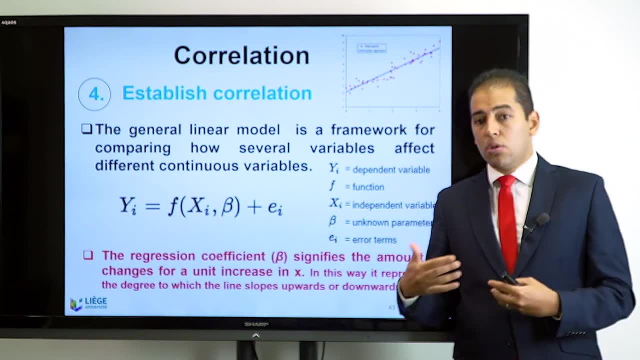 Correlation is. I have to conduct a series of statistical tests and I have to be very rigorous. I have to be very careful to make sure that if there is really a correlation or not, Because it doesn't mean that once I have variance by default that I will have a correlation. 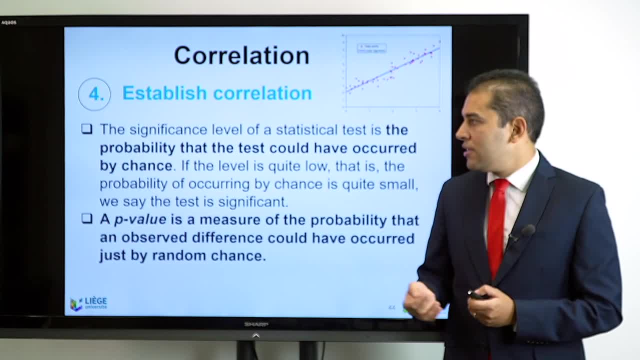 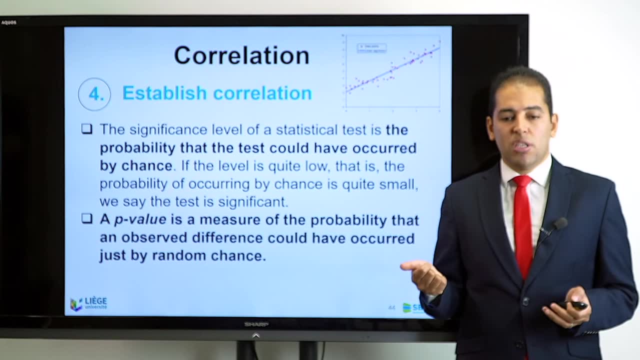 Also, as part of my correlation establishment, I look at the significance of level of statistical test. It is the probability that the test could have occurred by chance. This is important If the level is quite low. that is the probability of occurring by chance. 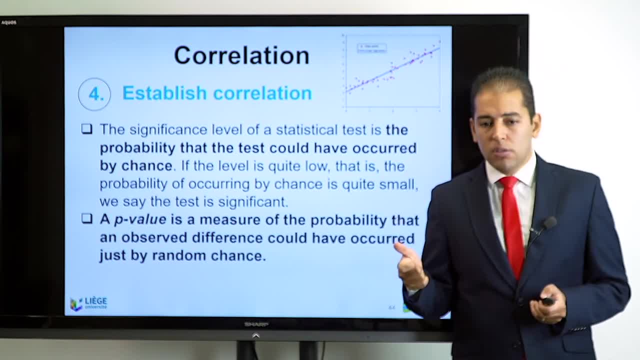 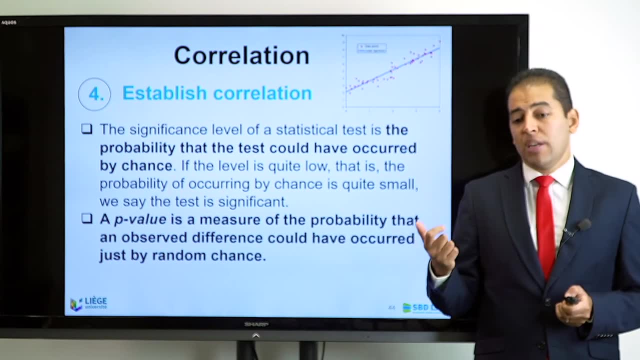 It's quite small, We say the test is significant And a p-value is a measure for the probability that one observed differences could have occurred just by random chance. So therefore we use the p-value And the p-value must be noted in any reporting. 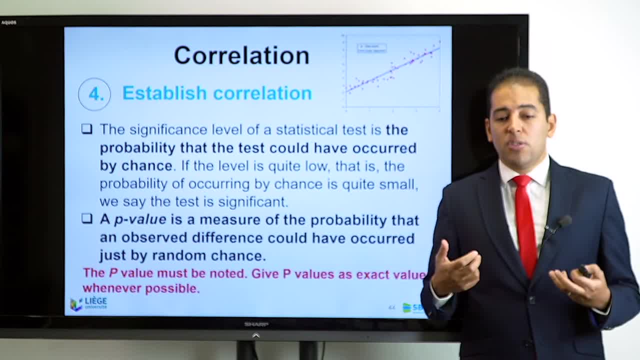 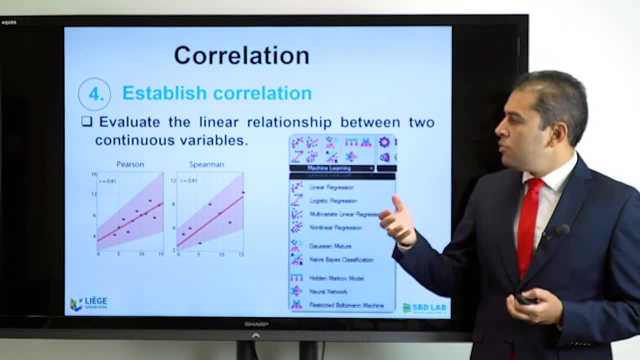 when you are conducting the test And you have to be able to interpret it and position it regarding your relation. Just some brief information about the correlations types. Here we look at linear relations between two continuous variables, But there are different types of correlations. 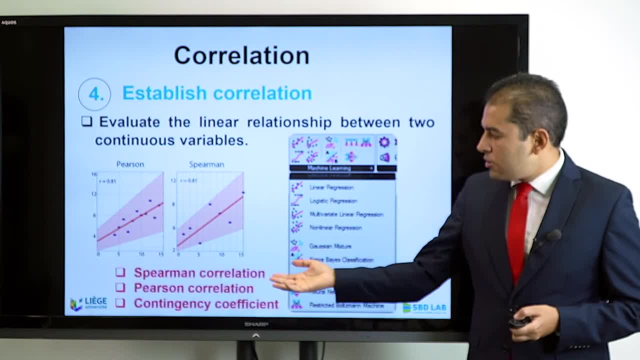 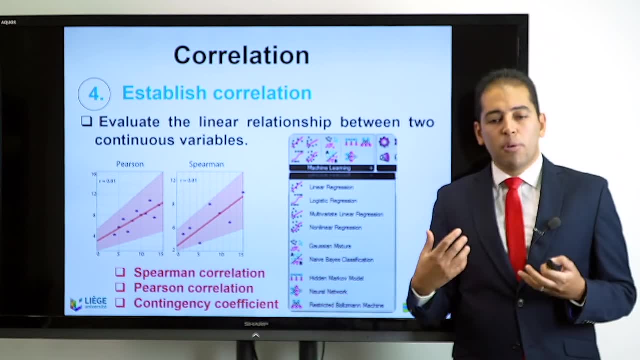 And we can go and move with different approaches. We have the famous Spearman correlation, the Pearson correlation, the contingency coefficient, And they are all types of tests for linear correlation. For non-linear, you have different types of statistical analysis, But this is beyond the presentation today. 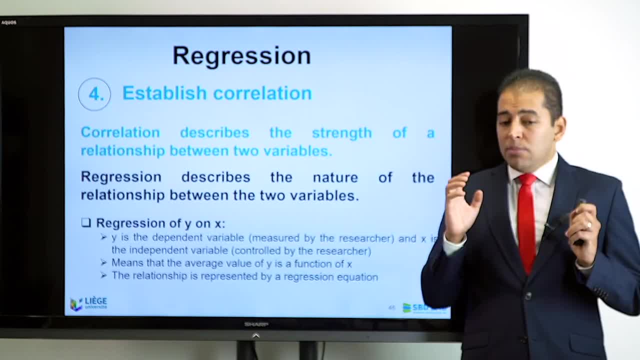 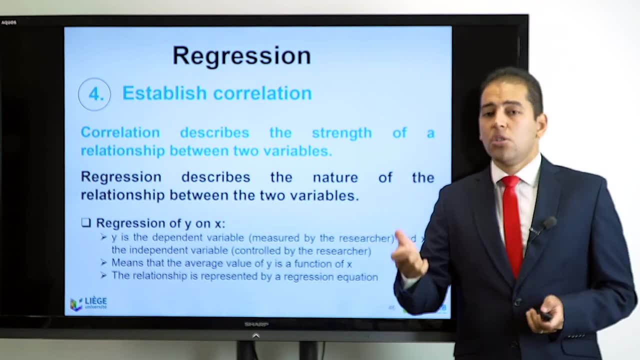 You have to go further in detail. Now I'm still talking about how to establish correlation, And once I prove that there is a correlation, I can go for a regression, And regression will allow me to predict, So I can have a curve, so that I can see what happens. 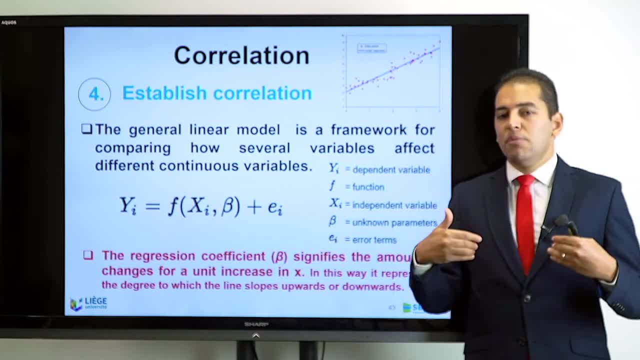 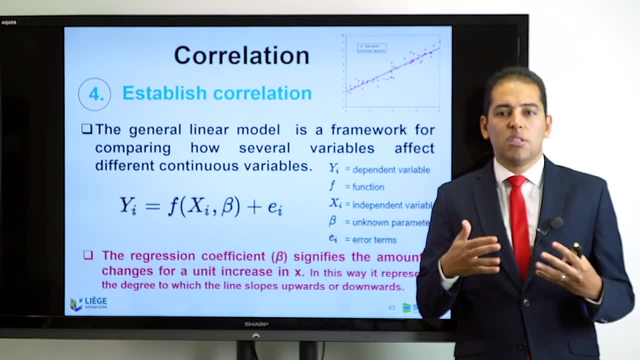 I have to conduct a series of statistical test and I have to be very rigorous. I have to be very careful to make sure that if there is really a correlation or not, because it doesn't mean that once I have variance by default that I will have a correlation also as part of my correlation. 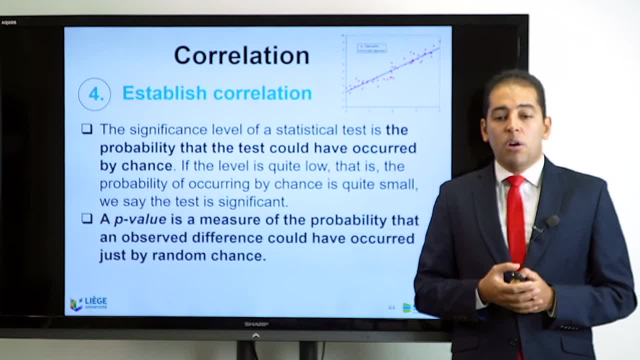 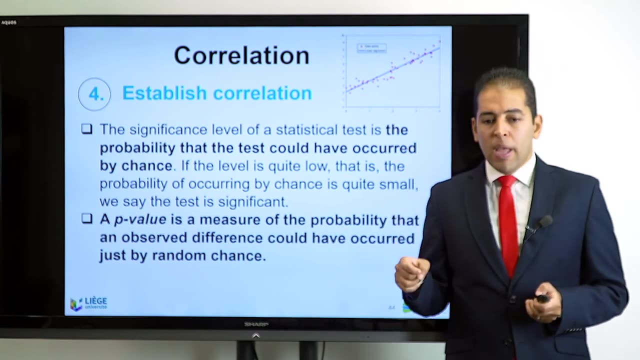 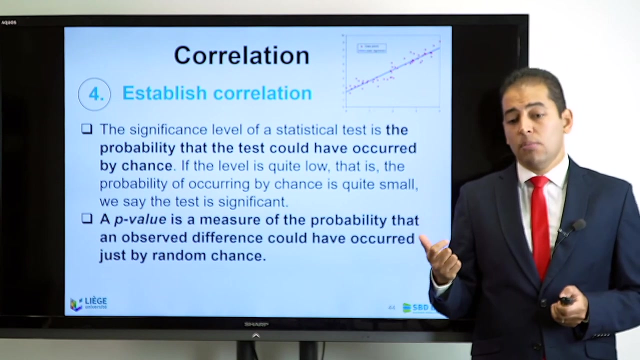 establishment. I look at the significance of level, of statistical level test. it is the probability that the test could have occurred by chance. this is important if, If the level is quite low, that is, the probability of occurring by chance is quite small, We say the test is significant and a p-value is a measure for the probability that one observed differences could have occurred just by random chance. 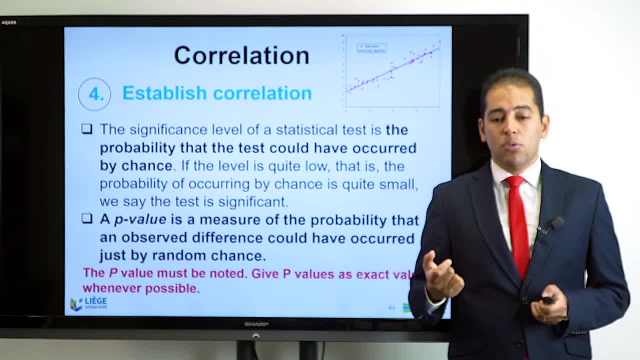 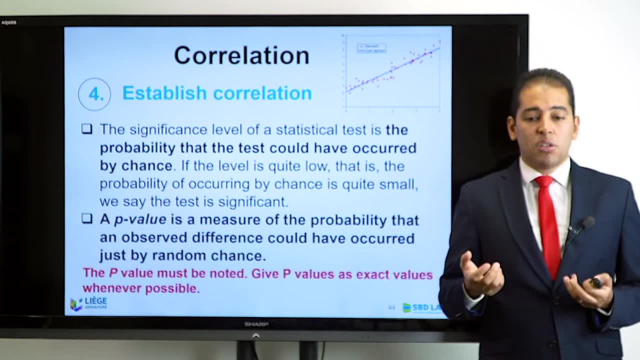 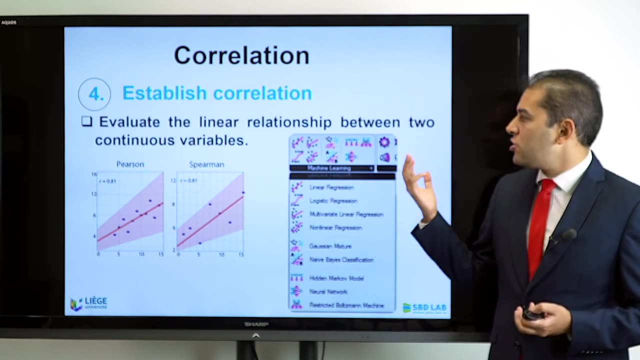 So therefore, we use the p-value and the p-value must be noted in any reporting when you are conducting the test, and you have to be able to interpret it and position it regarding your relation. Just some brief information about the correlations types. Here we look at linear relations between two continuous variables, but there are different types of correlations. 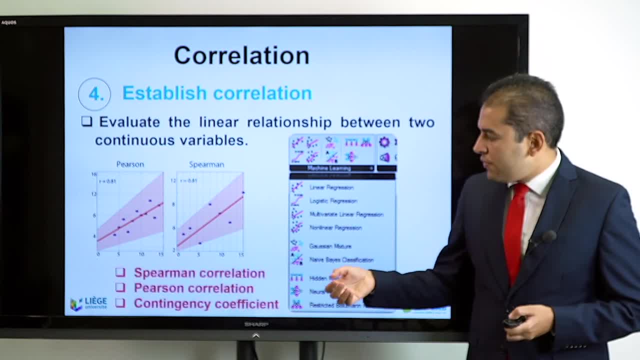 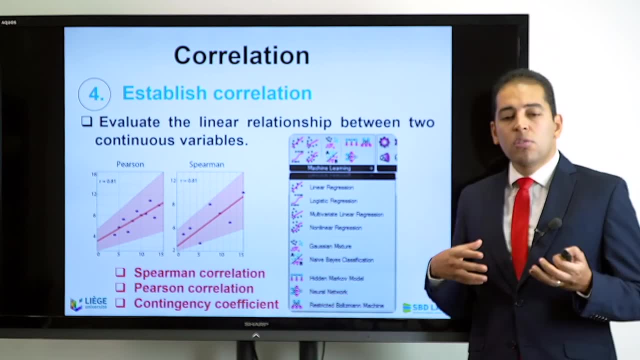 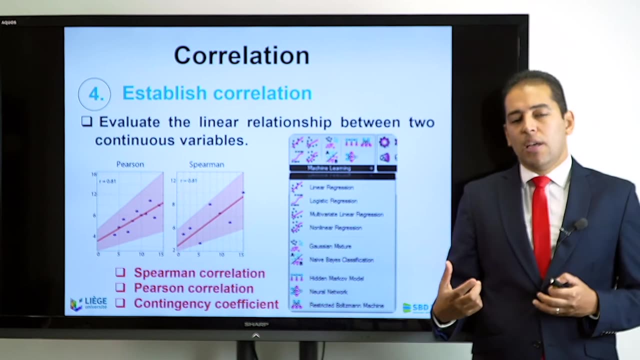 and we can go move with different approaches. We have the famous Spearman correlation, the Pearson correlation, the contingency coefficient and they are all type of tests for linear correlation, For non-linear, you have different types of statistical analysis, but this is. 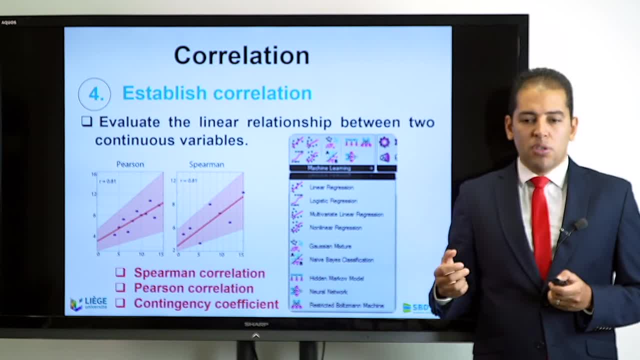 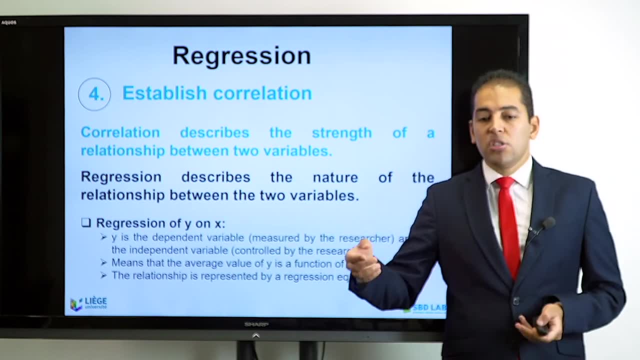 beyond the presentation today, You have to go further in detail. Now I'm still talking about how to establish correlation, and once I prove that there is a correlation, I can go for a regression, and regression will allow me to predict. So I can have a curve so that I can see what happens. 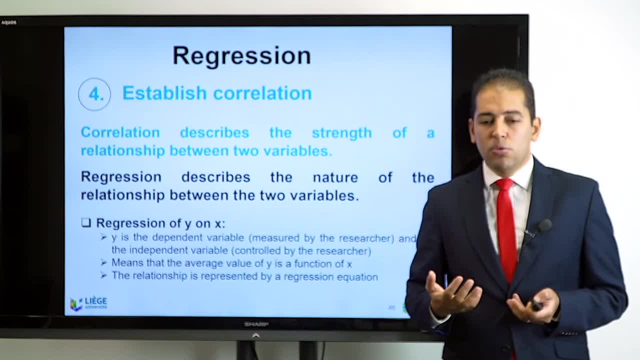 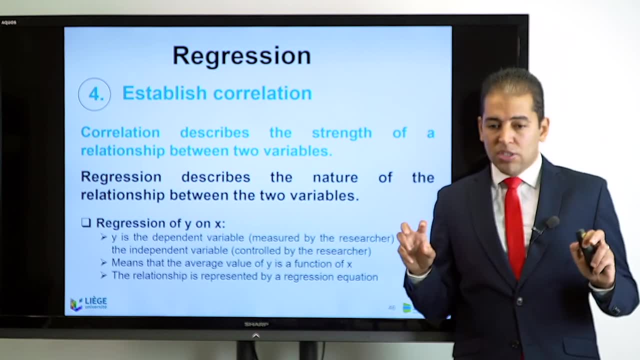 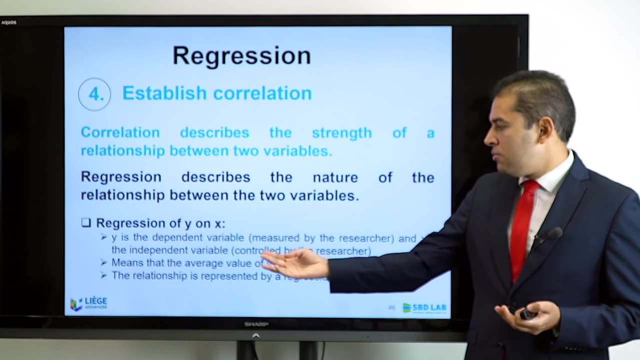 and regression simply describes the nature of the relationship between the two variables and in this sense, regression of a y on a x is simply y is the dependent variable which is measured by the researcher and it is the independent variable- independent variable which is controlled by the researcher and by mean it means. 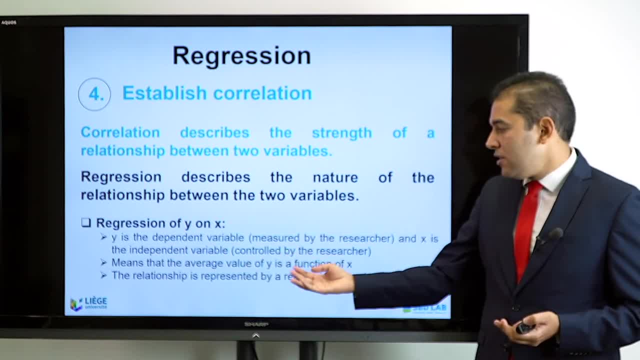 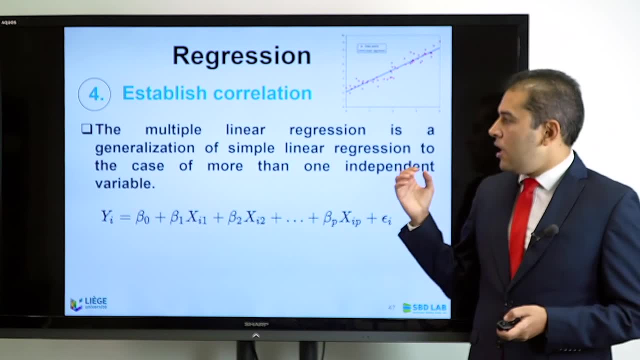 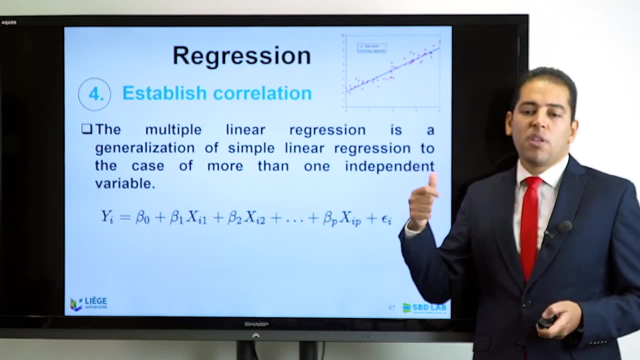 that the average value of y is a function of x and the relationship is represented by a regression equation. as you can see, here is the regression equation. it is the multiple linear here. it allows the multiple linear regression is a generalization of a simple linear regression, so we can have different. 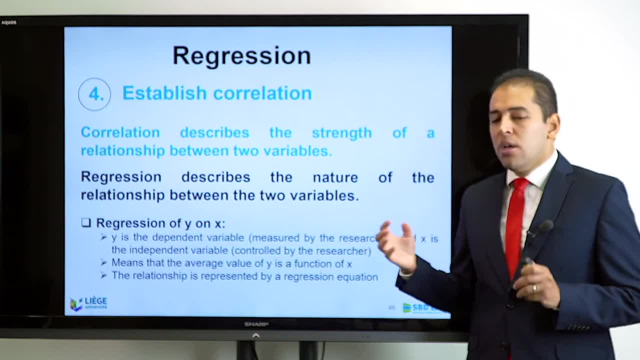 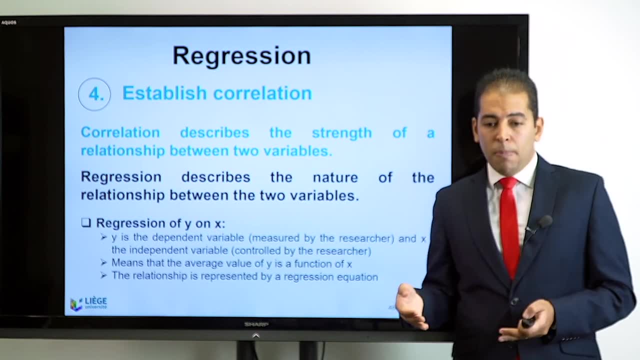 And regression simply describes the nature of the relationship between the two variables And in this sense, regression of a y on an x is simply y is the dependent variable which is measured by the researcher And it is the independent variable which is controlled by the researcher. 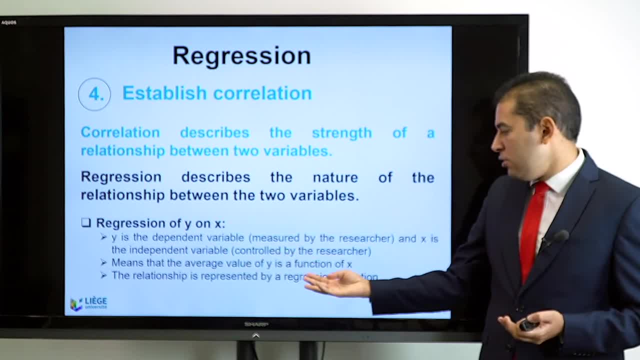 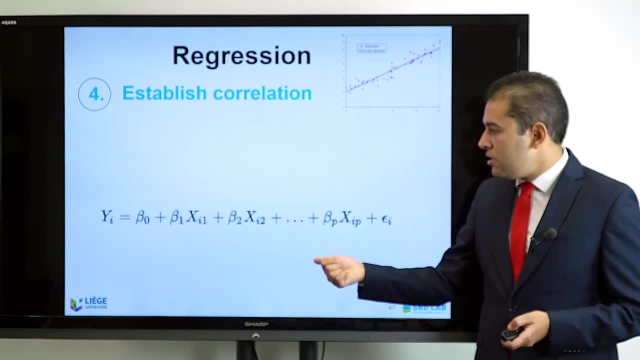 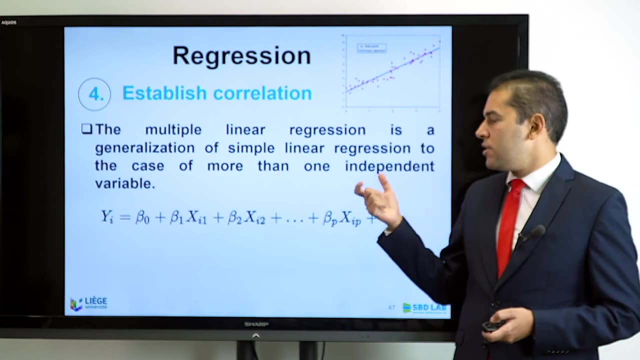 And it means that the average value of y is a function of x And the relationship is represented by a regression equation. As you can see, here is the regression equation. It is the multiple linear. Here it allows the multiple linear. regression is a generalization. 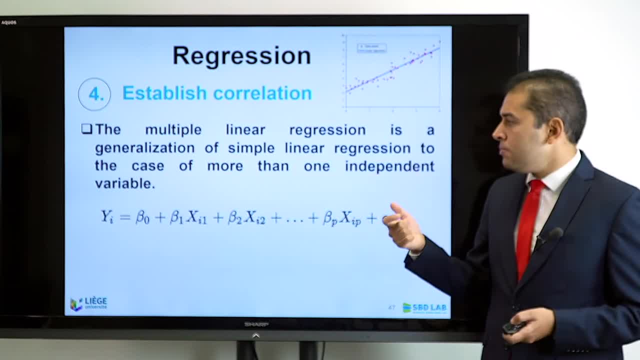 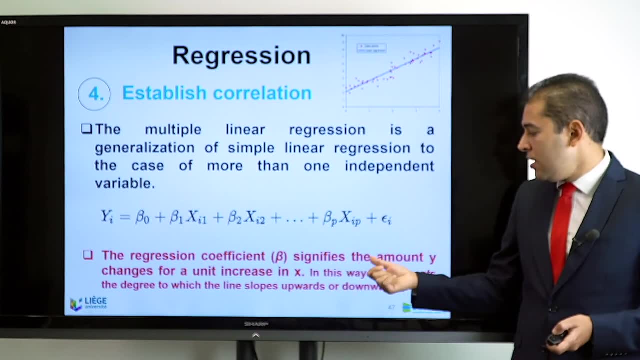 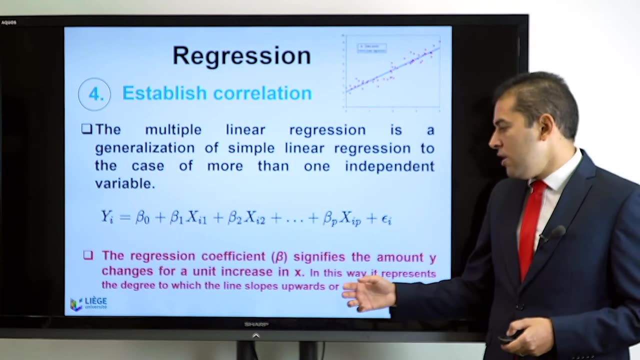 of a simple linear regression. So we can have different types of regressions to the case of more than one independent variable. And here we have to report the regression coefficient, beta. that signifies the amount of y changes for a unit increase in x And it represents the degree. 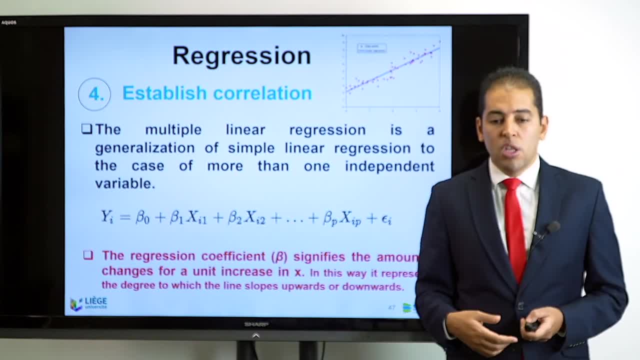 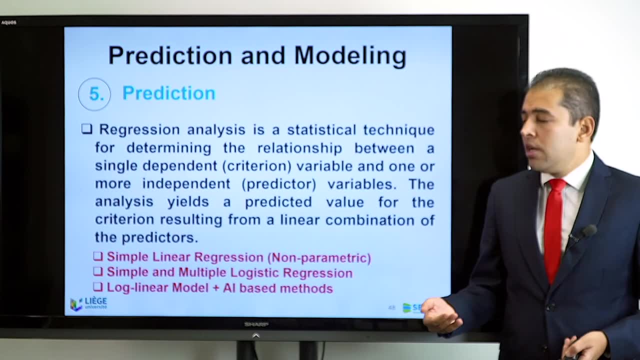 of which the line slopes upwards or downwards. So this is very important to look at. Now, once I have the regression and I am able to establish a correlation, I can go to the prediction part, And here regression analysis is the best way to do it. 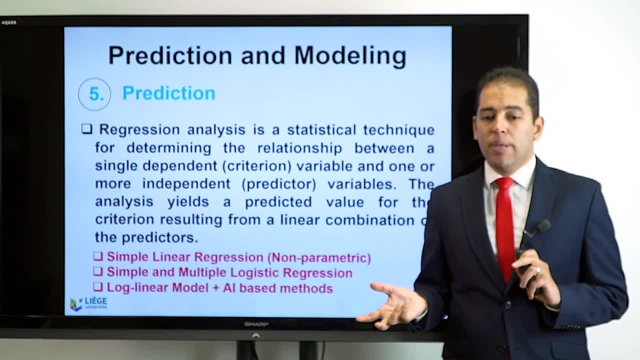 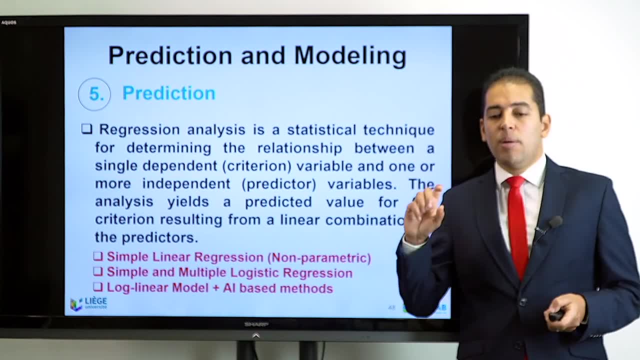 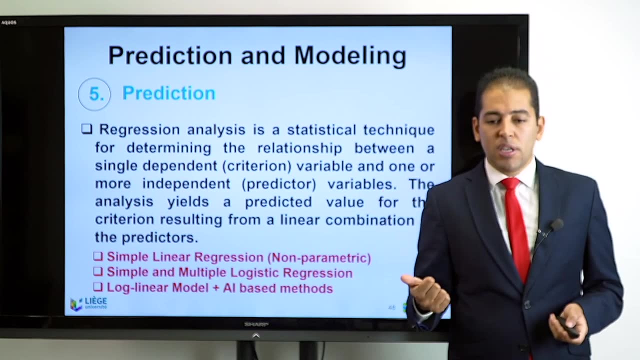 because regression analysis is a statistical technique for determining the relationship between a single dependent criterion or variable and one or more independent predictor variable. And here I can do the criterion resulted from a linear combination of the predictors, And here I can use the simple linear regression. 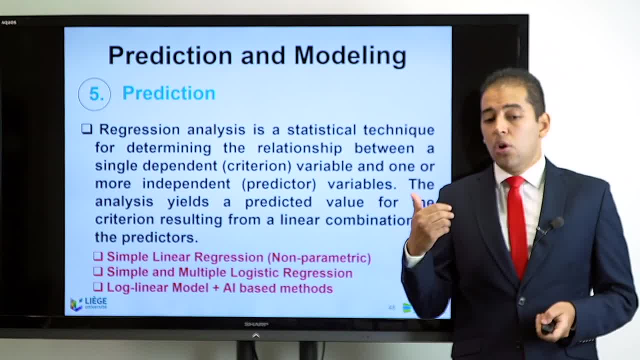 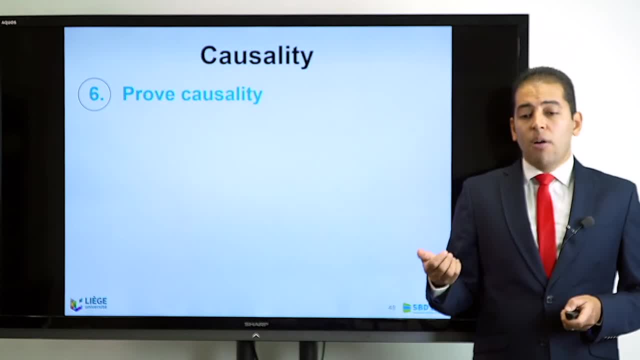 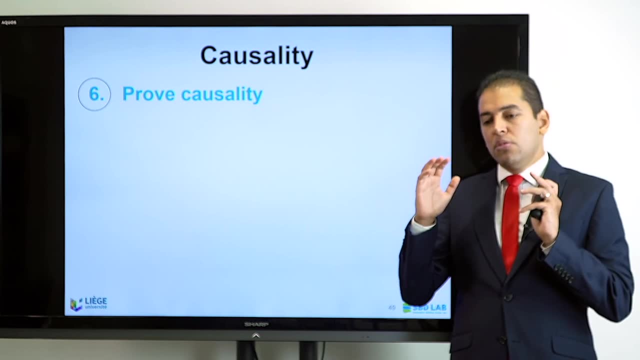 if I am doing non-parametric testing, I can do simple and multiple logistic regression and I can do log, linear models and artificial intelligence based methods that are more complicated and more advanced. Now I am moving to the last part of the types of statistical analysis that you need to be aware about. 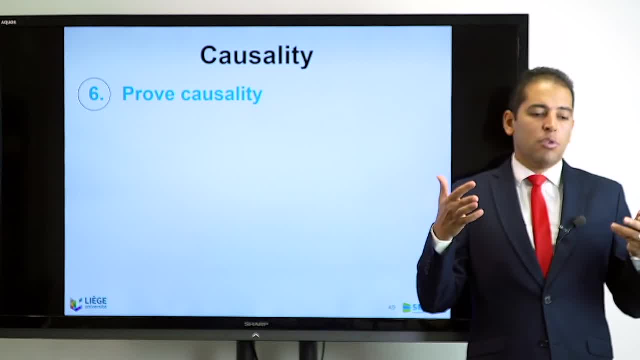 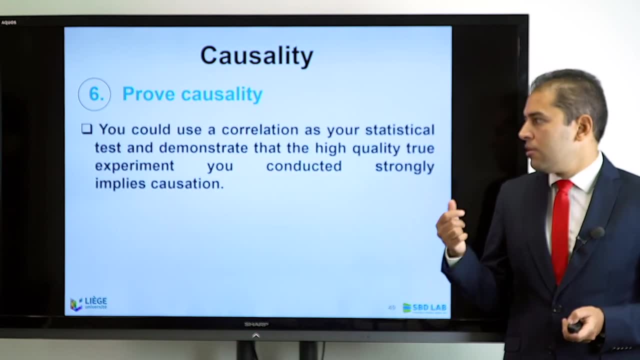 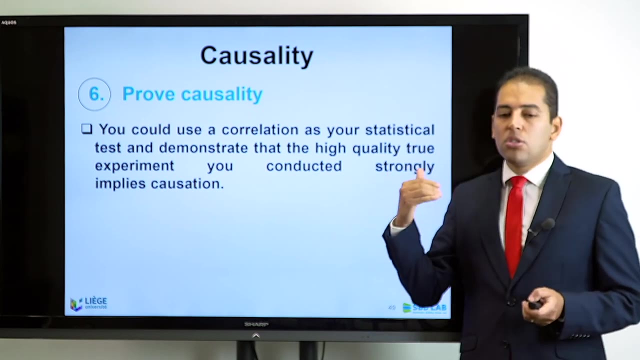 If you described your sample, you proved that there is variance and there is also a correlation. you can look at causality, which is not a straightforward thing. Causality here is very important because you could use a correlation as your statistical test and demonstrate that the high quality 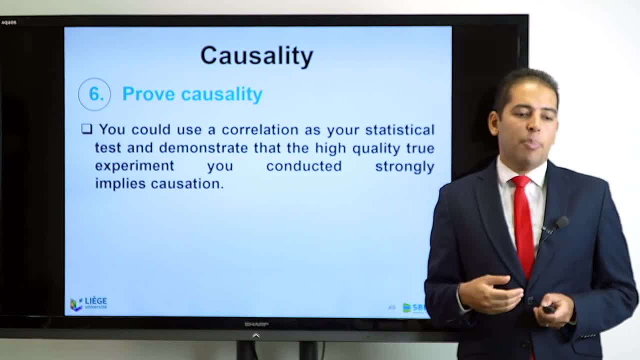 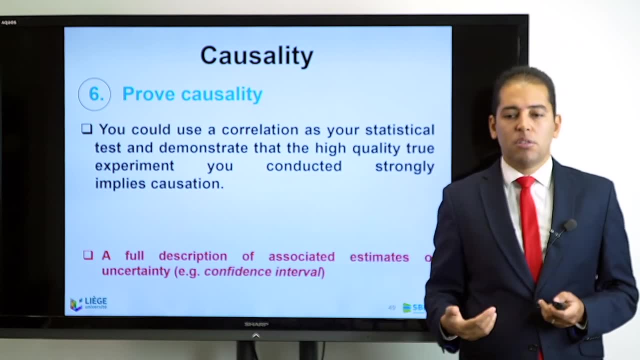 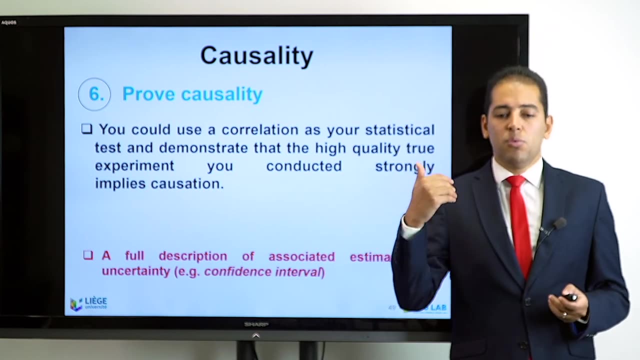 true experiment you conducted strongly implies causation And this is rarely happening because it is very difficult to prove causation. You need a very large sample size. you need to replicate your test. you have to make sure there is randomization. you don't have any biases. 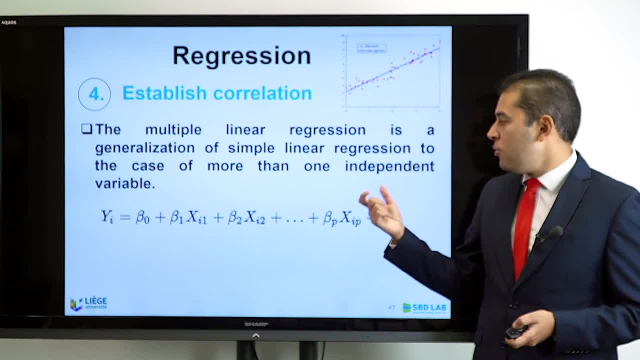 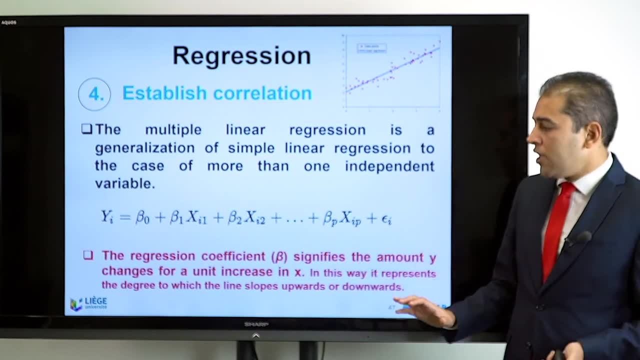 types of regressions to the case of more than one independent variable. and here we have to report the regression coefficient beta. that signifies the amount of y changes for a unit increase in X, and in this way it represents the degree of which the line slopes upwards or downwards. so this is very important. 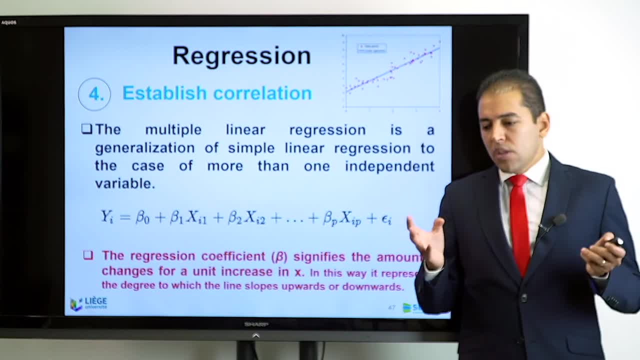 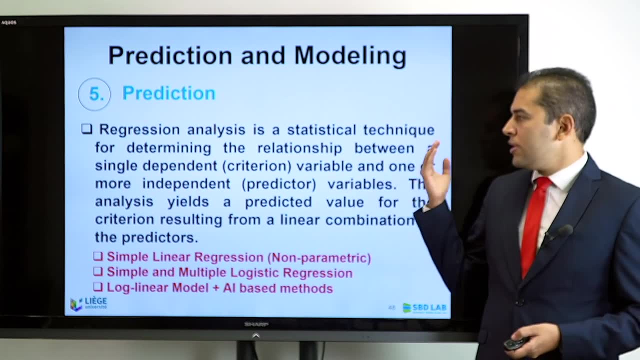 to look at now. once I have the regression and I'm able to establish a correlation, I can go to the prediction part, and here regression analysis is the best way to do it, because a regression analysis is a statistical technique for determining the relationship between a single dependent. 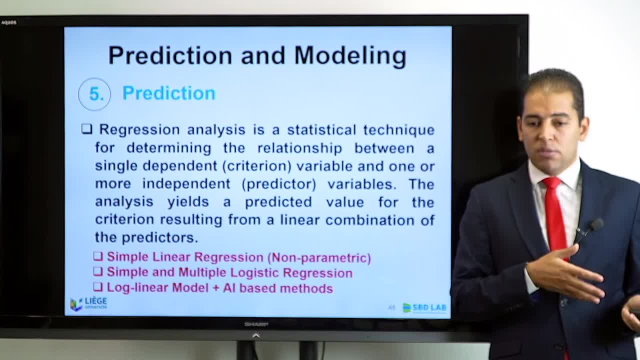 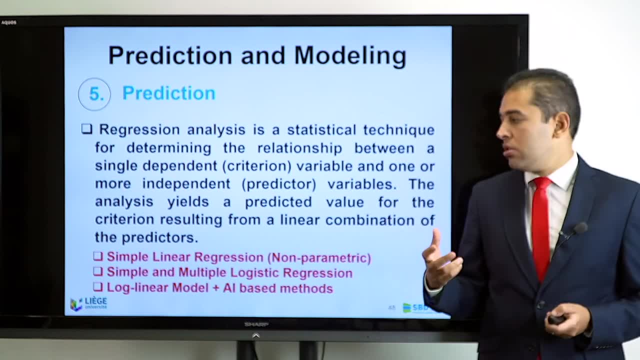 and a single dependent variable, and the regression equation is a statistical technique for determining the relationship between a single dependent criterion or variable and one or more independent predictor variable, and analysis yields a predicted value for the criterion resulted from a linear combination of the predictors, and here I can use the simple linear regression. if 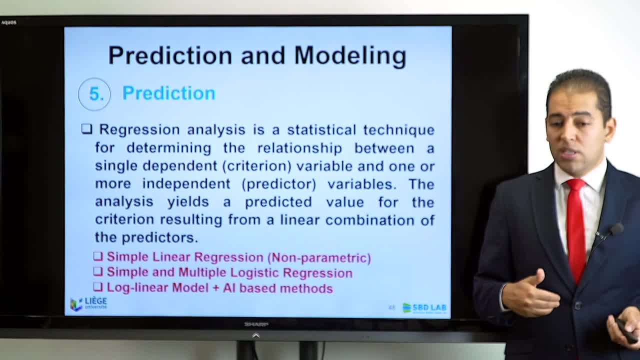 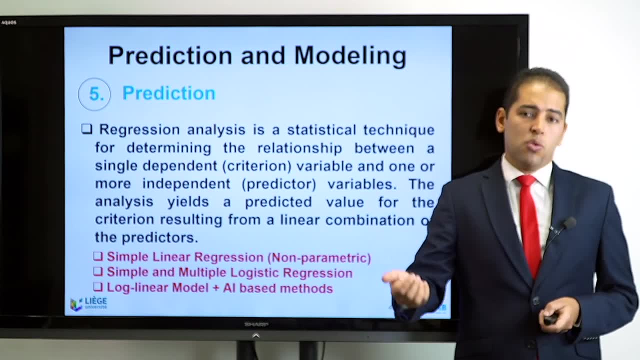 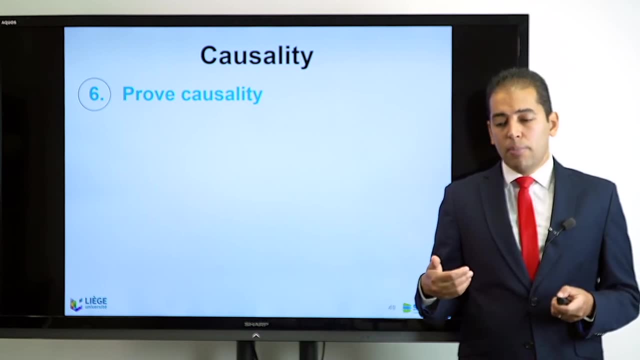 I'm doing nonparametric testing. I can do simple and multiple logistic regression and I can do log linear models and artificial intelligence based methods that are more complicated and more advanced. now I'm moving to the last part of the types of statistical analysis that you need to be aware about if you proved you. 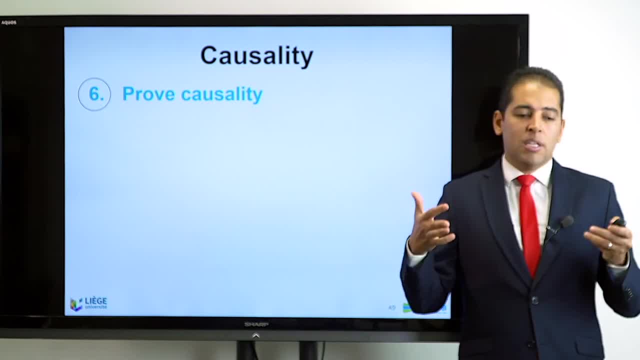 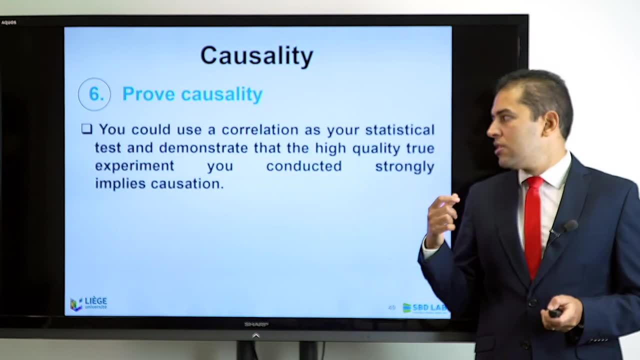 described your sample. you proved that there is variance and now you have also a correlation. you can look at causality, which is not a straightforward thing. causality here is very important because you could use a correlation as your statistical test and demonstrate that the high quality, true experiment you 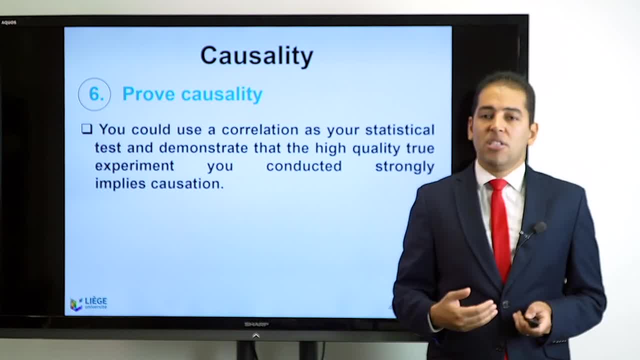 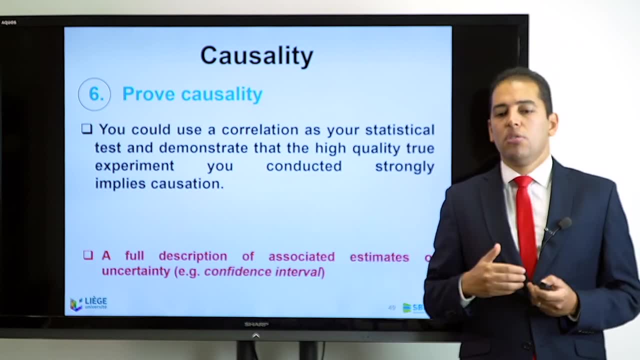 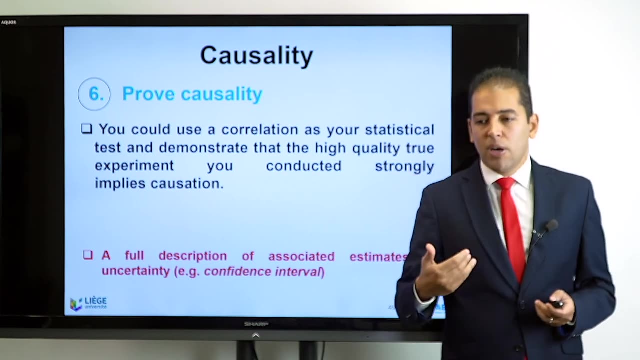 conducted strongly implies causation, and this is rarely happening because it's very difficult to prove causation. you need a very large sample size. you need to replicate your, your, your test. you have to make sure there is randomization. you have to avoid any biases. you have to do blindness. 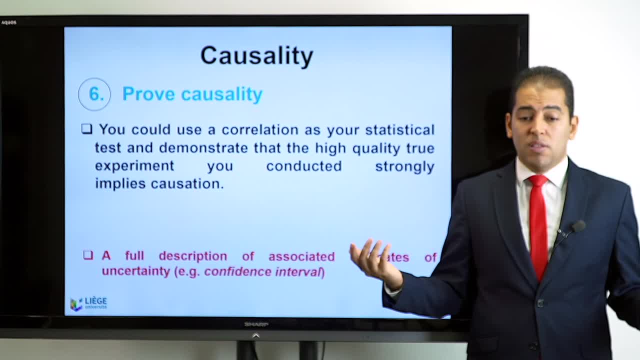 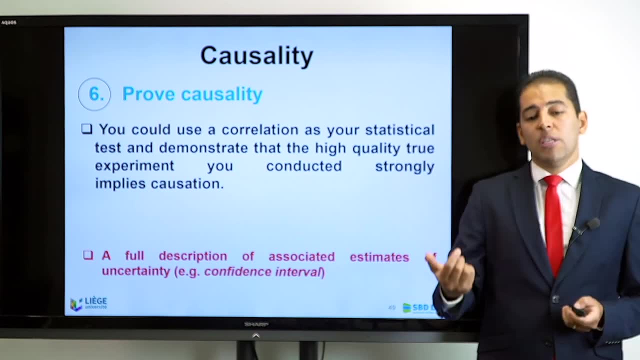 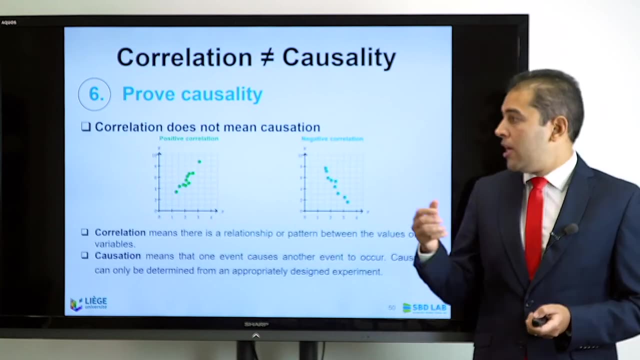 and so on, and if it is positive, then it is there? so a full description of your associated estimations of uncertainty and your confidence intervals. when you are communicating any results that confirm or proves or negates causality needs to be taken into account, and proving causality can have correlation. 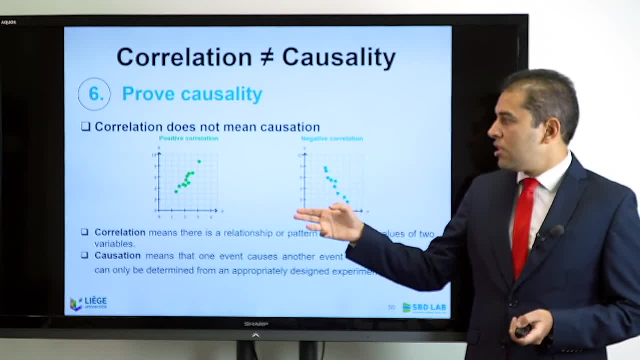 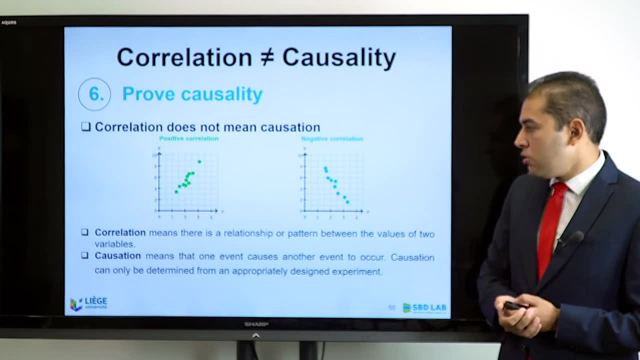 also an important remark here- that correlation doesn't mean that there is a causation, so I can have a positive correlation or a negative correlation, but it doesn't mean that I have a causality. so causation means that one event causes another event to occur, and causation can only be determined from an. 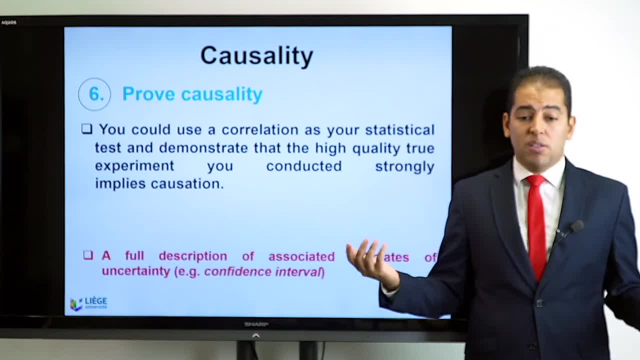 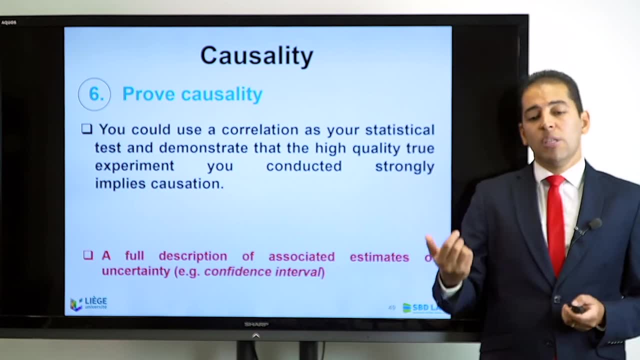 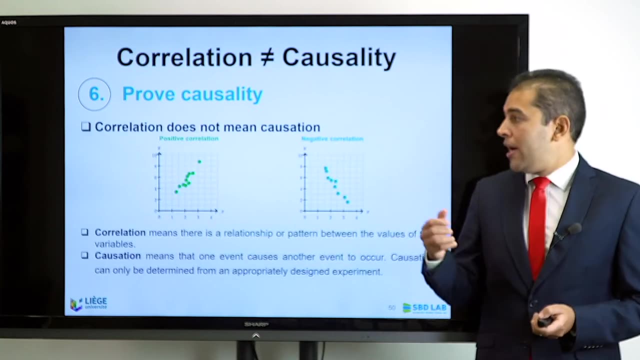 you have to do blindness and so on, and if it is positive, then it is there. So a full description of your associated estimations of uncertainty and your confidence intervals. when you are communicating any results that confirm or proves or negates causality needs to be taken into account. 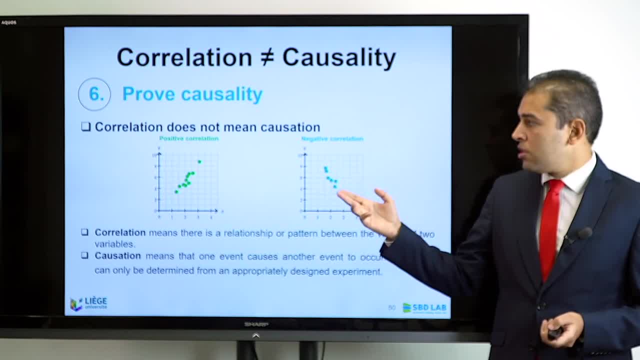 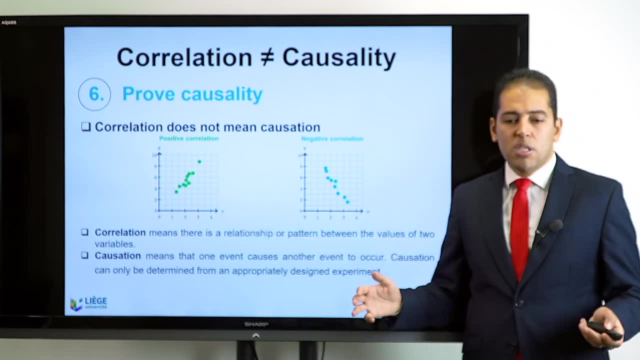 and proving causality can have correlation. also an important remark here: that correlation doesn't mean that there is causation, so I can have a positive correlation or a negative correlation. it doesn't mean that I have causality, so causation means that one event causes another event to occur. 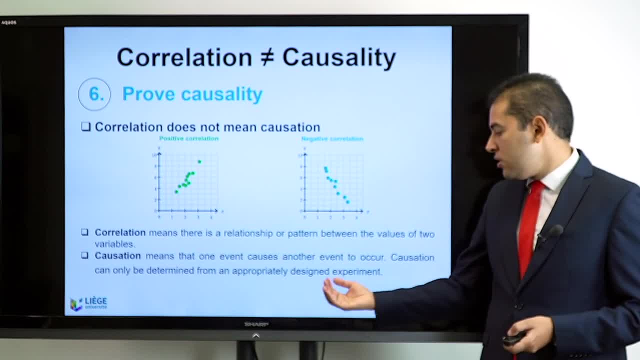 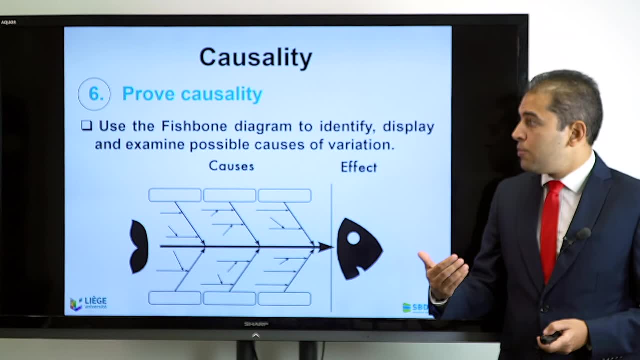 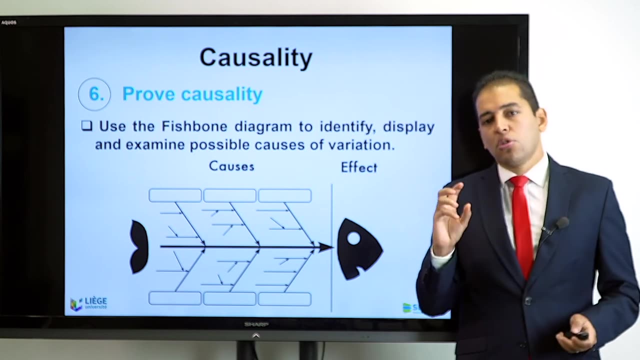 and causation can only be determined from an appropriately designed experiment. the only way and my only advice for you, if you are seeking this causation aspect, that you use the fishbone diagram, because, in most of the time, causation today, phenomena that you are investigating are so complex. 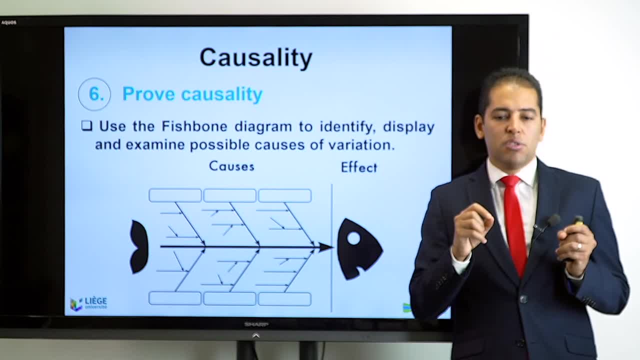 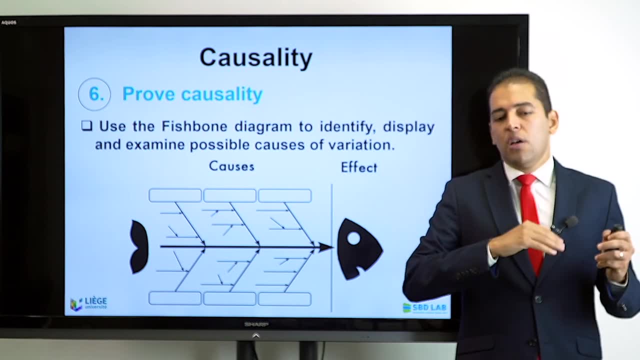 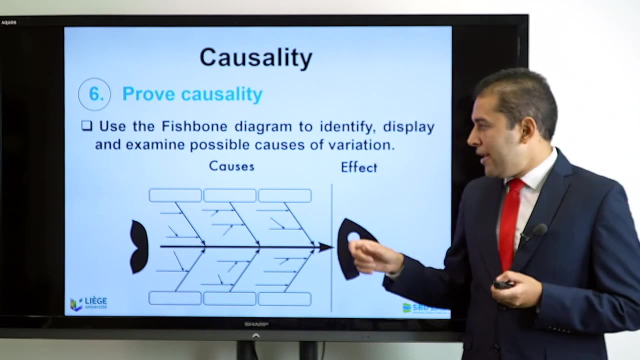 and we have this cocktail effect. so it is very difficult to say that this specific factor has this influence on this phenomena, but most of the time it is a cocktail. it's a series of recurring phenomena that together are working on causing this effect and therefore we use this. 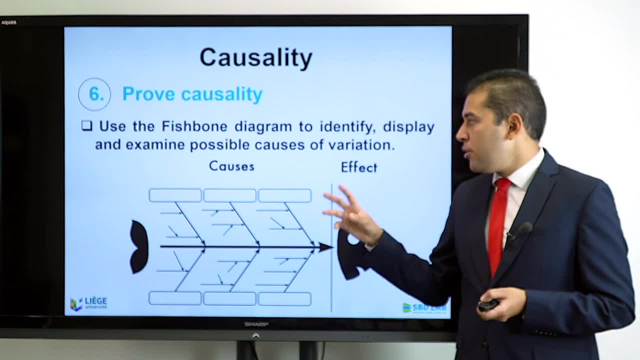 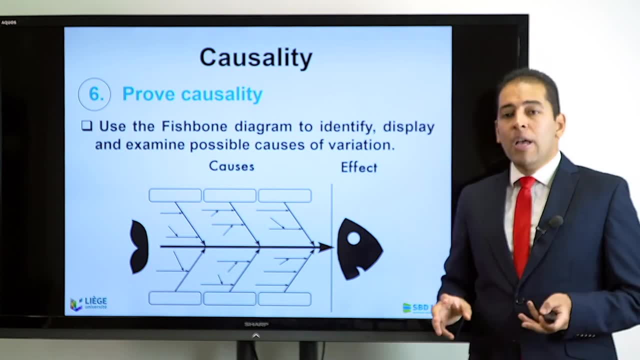 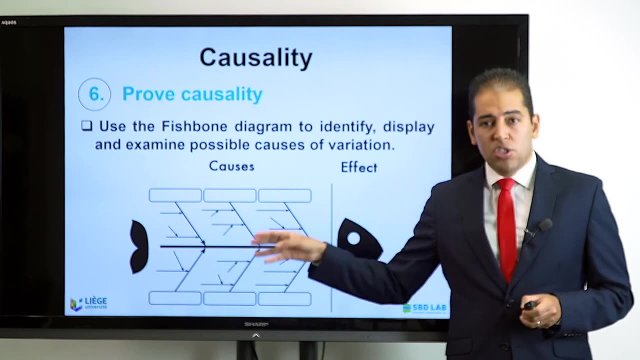 famous fishbone diagram to identify, display and examine possible causes on variance. and once you name your possible causes and you make sure that you control them and neutralize them, all your statistical test has to make sure that this was taken into account and only then you can have a causation. 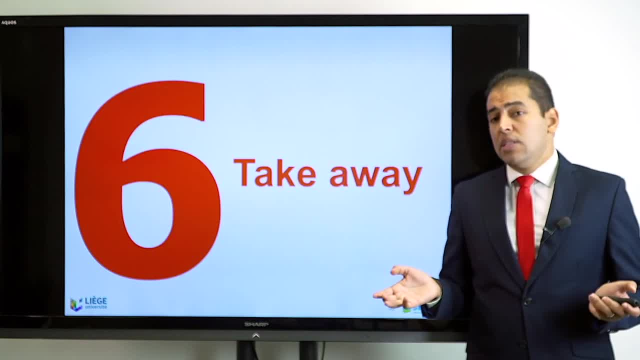 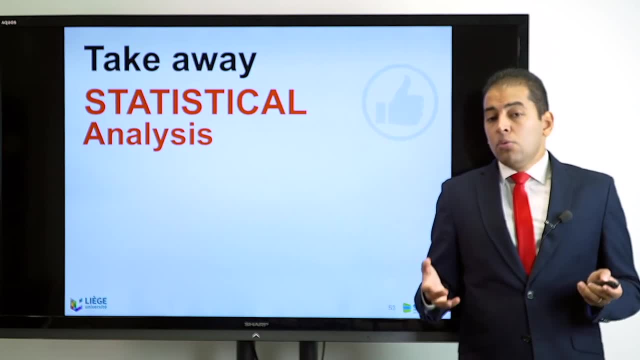 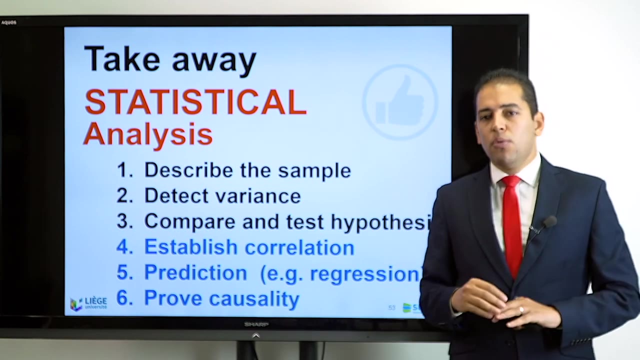 and a positive confirmation, voila. this is the end of today's presentation. some take away messages before you leave. statistical analysis is very important. what do we do with statistical analysis? I want you just to memorize this slide. this is why we do statistical analysis before getting into detail. 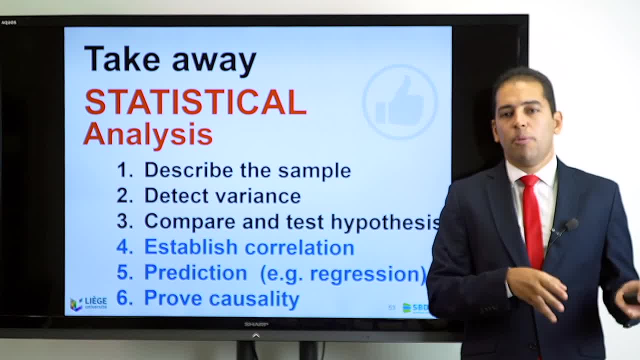 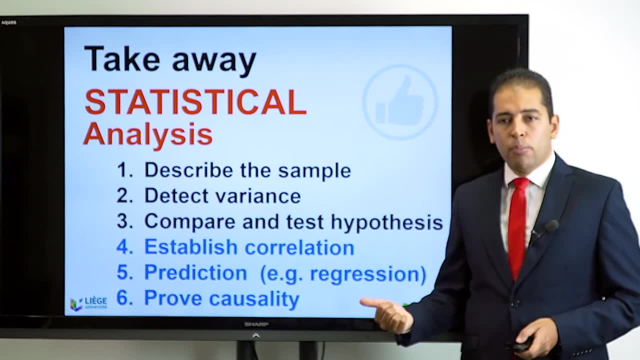 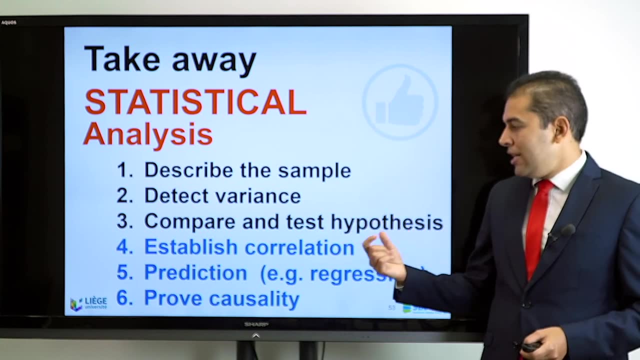 learning software and knowing what type of test to do. you just need to know. why do we do statistical analysis? logically, we do statistical analysis to describe the sample, to detect a variance, to compare two different groups and test our hypothesis, establish a correlation and predict through regression, for example. 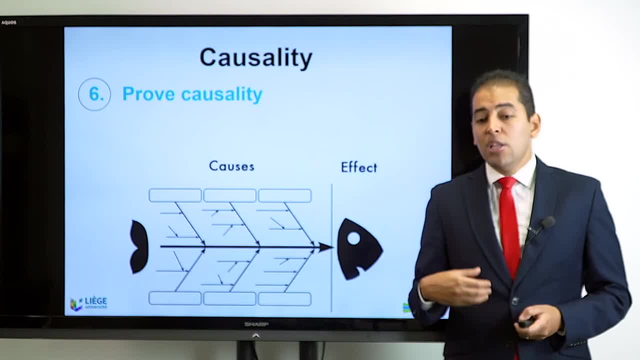 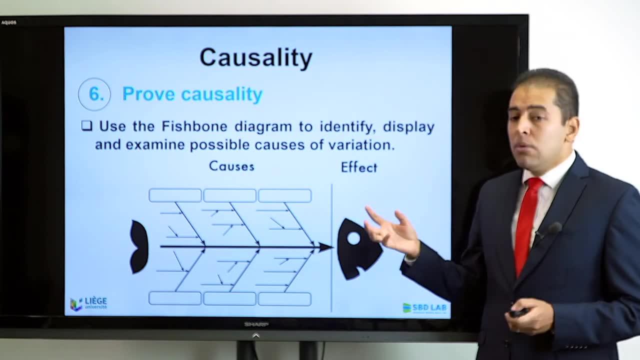 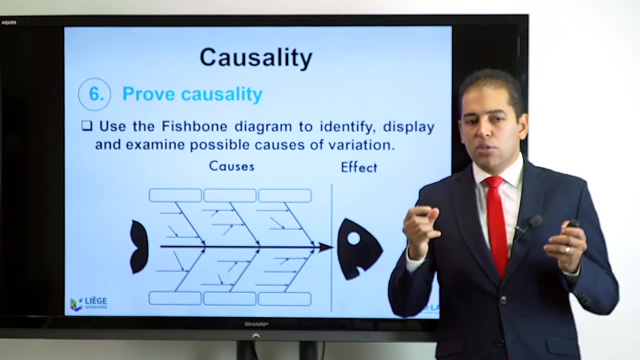 appropriately designed experiment. the only way and my only advice for you, if you are seeking this causation aspect, that you use the fish bone diagram, because in most of the time, causation today, phenomena that we are investigating are so complex and we have this cocktail effect, so it's very difficult to say that this specific 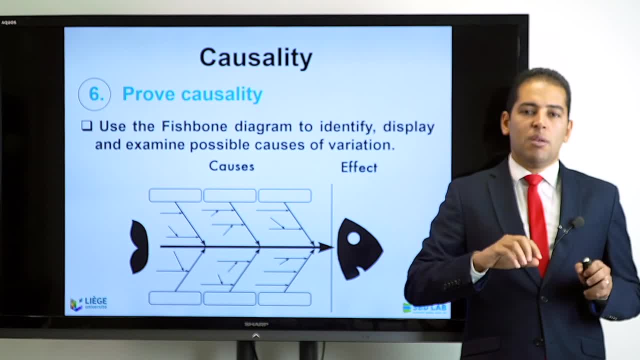 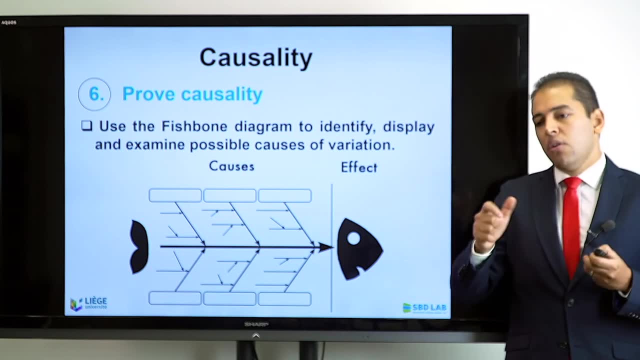 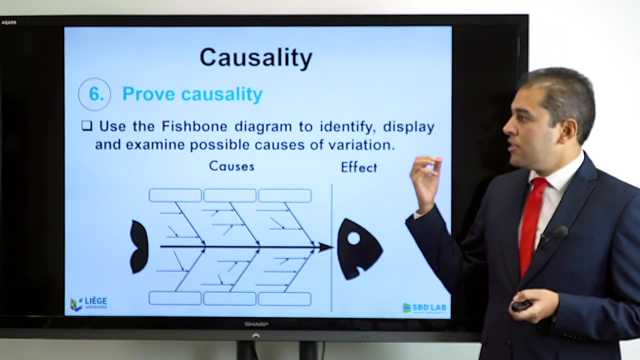 factor has this influence on this phenomena, but most of the time it is a cocktail. it's a series of recurring phenomena that together are working on on causing this effect and therefore we use this famous fish bone diagram to identify, display and examine possible causes. on variance and once you. 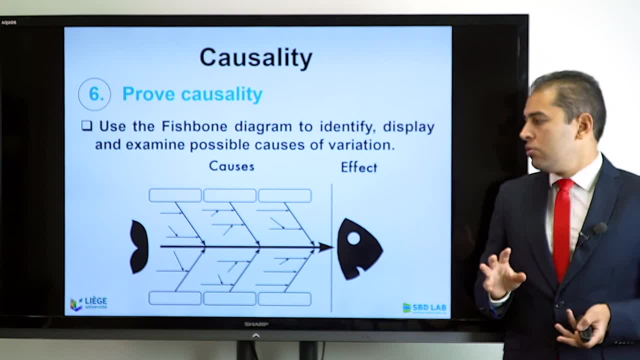 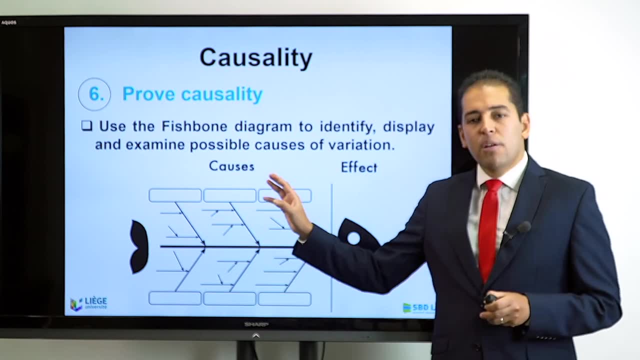 name your possible causes, you will see something that is a good example of a and you make sure that you control them and you neutralize them. all your statistical test has has to make sure that this was taken into account and only then you can have a causation and a confirmation: positive confirmation. 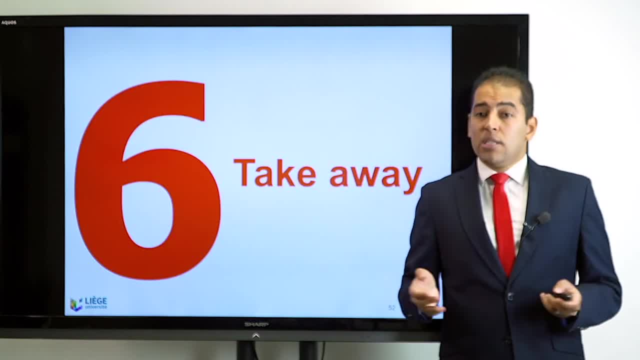 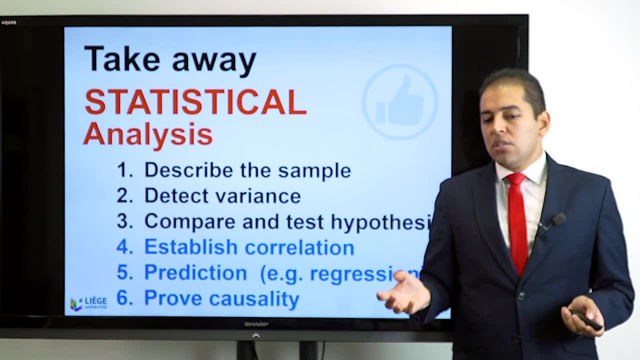 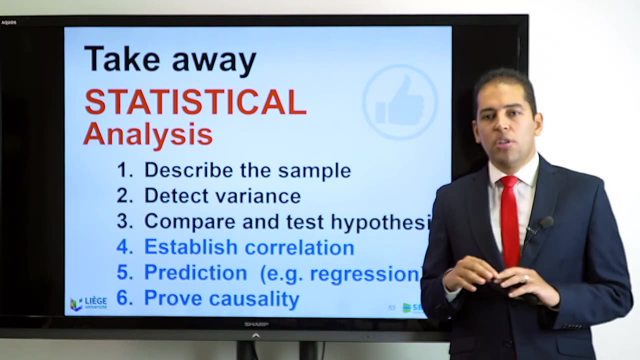 voila. this is the end of today's presentation. some takeaway messages before you leave. statistical analysis very important. what do we do with statistical analysis? I want you just to memorize this slide. this is why we do statistical analysis before in getting into detail, learning software and 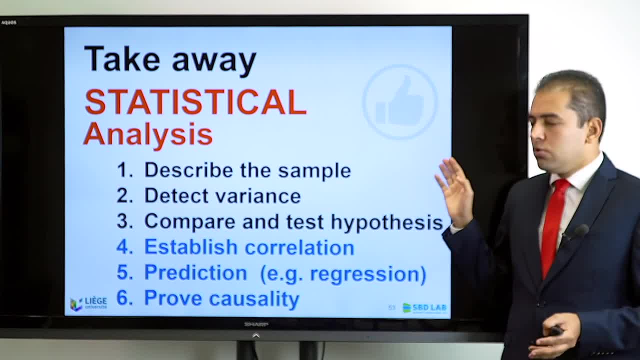 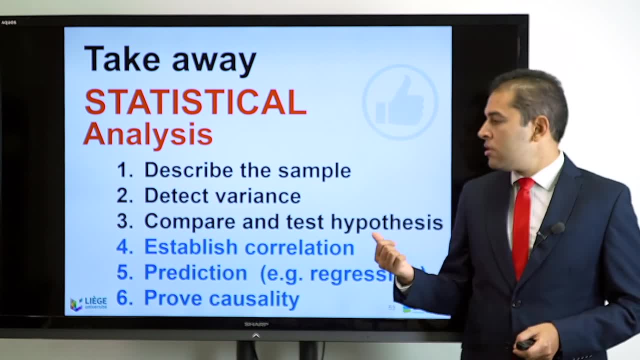 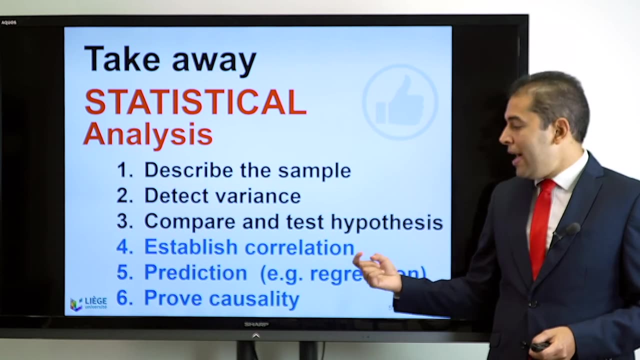 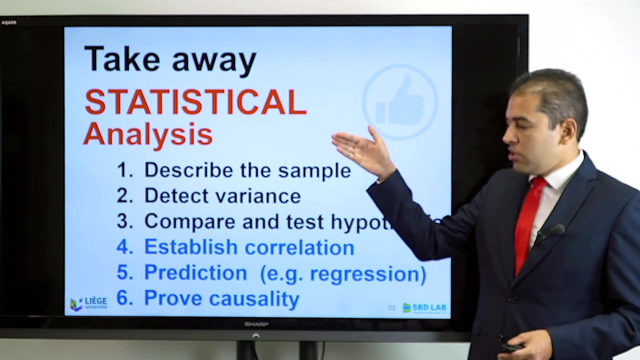 knowing what type of tests to do. you just need to know. why do we do statistical analysis? logical? we do statistical analysis to describe the sample, to detect a variance, to compare two different groups and test our hypothesis, establish a correlation and predict, through regression, for example, and finally prove causality, keep into account. the process is not. 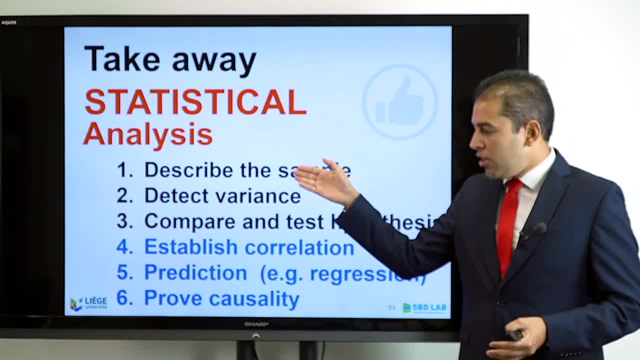 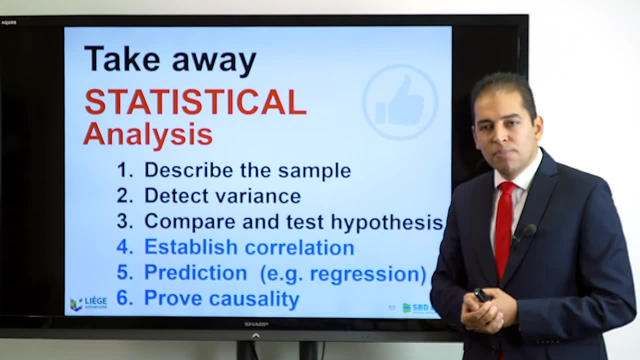 straightforward and not every experiment that you will do will go from 1 to 6. some or most of the test, I can tell you 80% of investigation- they stop after step number 2. we don't detect any variance and then the experiment is dead. and this 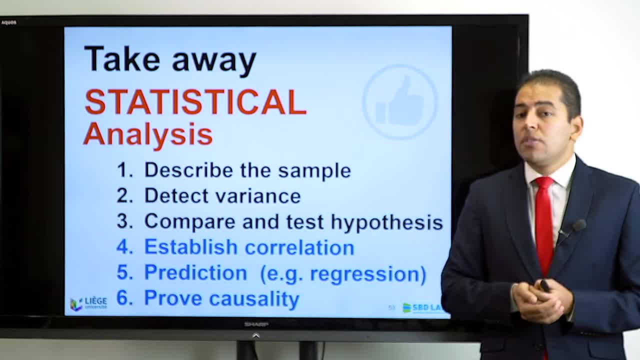 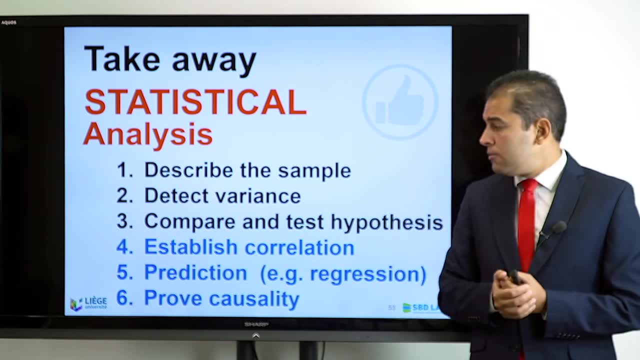 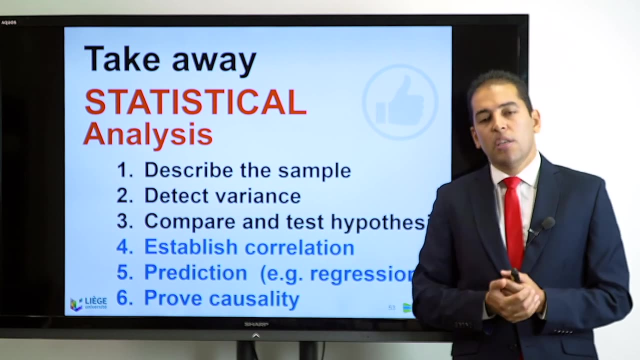 is the, the, unfortunately the null result. but today's scientific word is trying to allow to publish even the null result because we learn from it and if you have a positive variance then you can go to the comparison of the groups and go with prediction and cause, establishing a correlation. 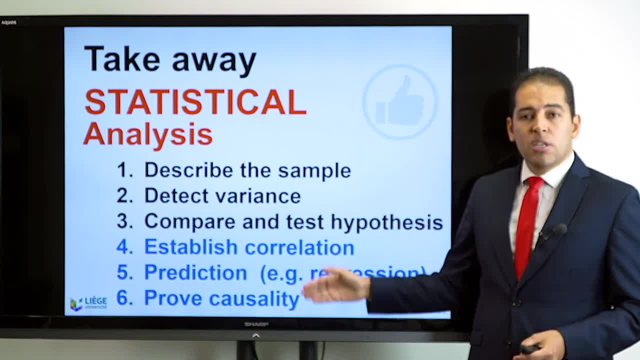 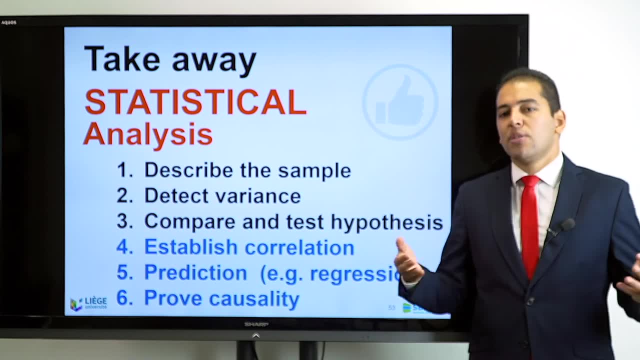 and finally prove causality. keep into account the process is not straight forward and not every experiment that you will do will go from one to six. some or most of the test, I can tell you 80% of investigation- they stop after step number two. we don't detect any variance. 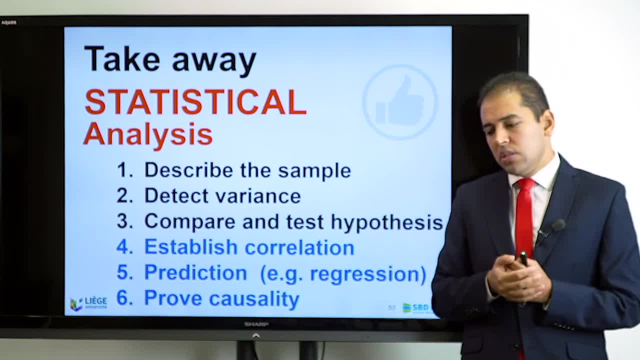 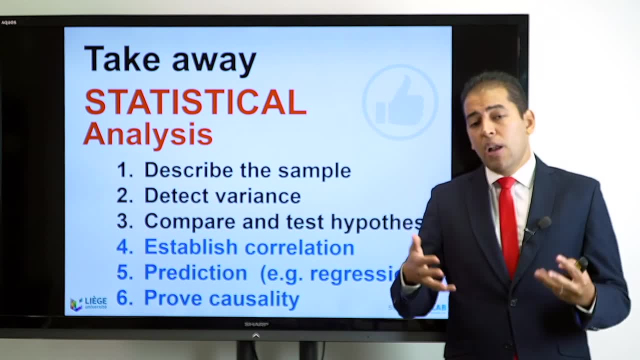 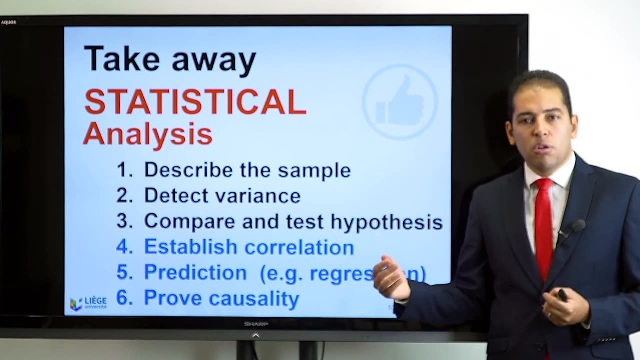 and then the experiment is dead and this is the unfortunately the null result. but today's scientific word is trying to allow to publish even the null result because we learn from it and if you have a positive variance then you can go to the comparison of the groups and go with prediction. 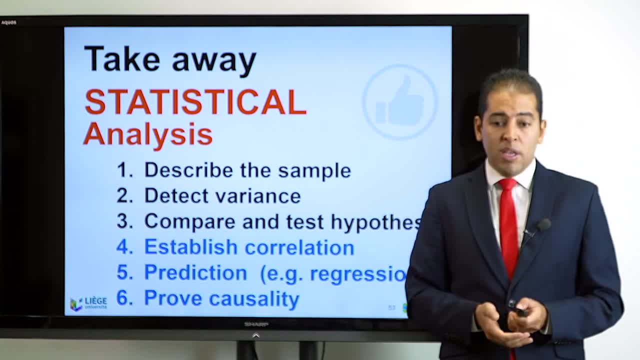 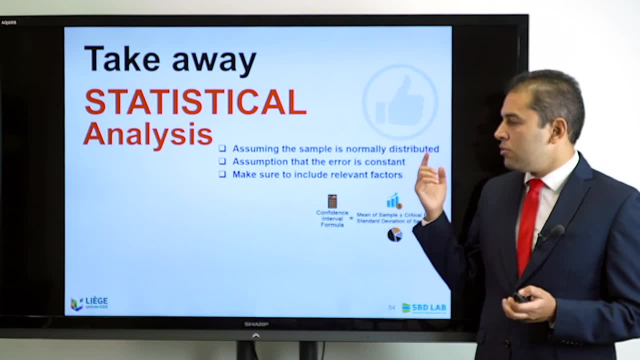 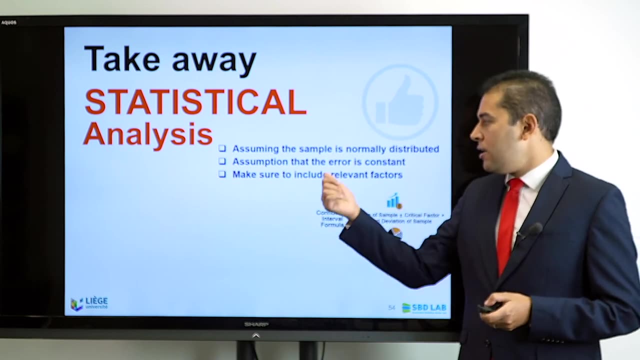 and establishing a correlation before proving causality. the second key take away message of today: you have always to look at the normal distribution. what I talk today about is mainly under the condition that I am assuming that the sample is normally distributed and I am assuming that the error is constant. 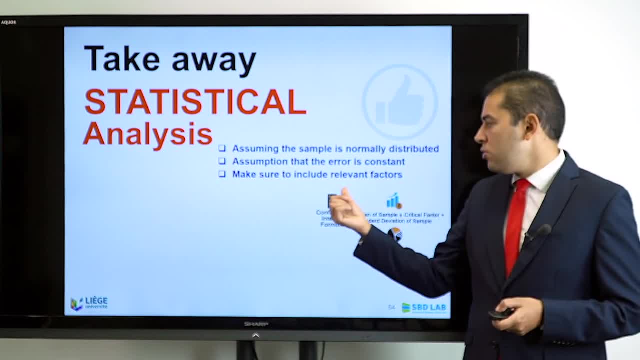 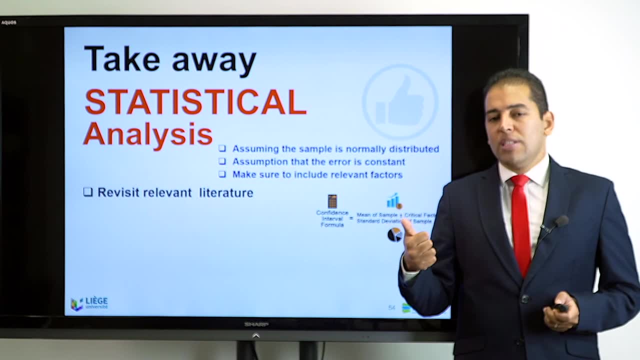 in all your test- and I am here also- you have to make sure to include all relevant factor to control your experiment. number one: revisit when you do statistical analysis or when you are preparing your experiment for statistical analysis. revisit the relevant literature, look of different test and variables. 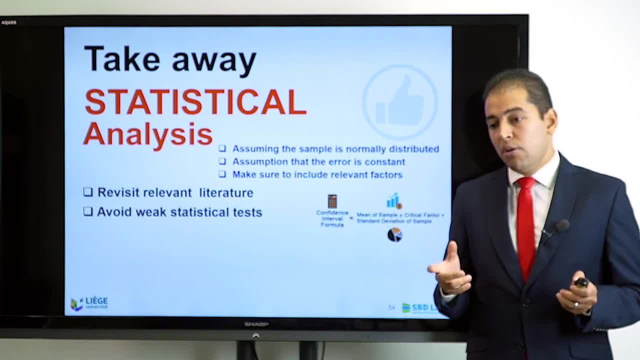 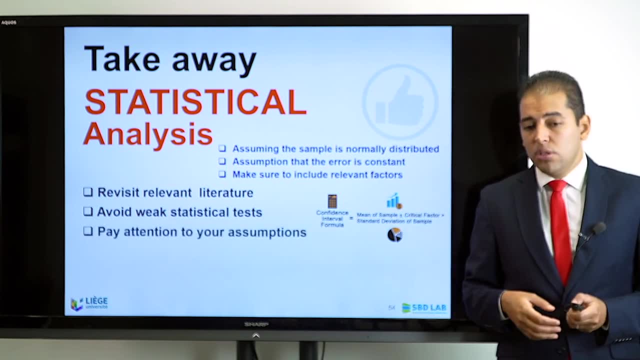 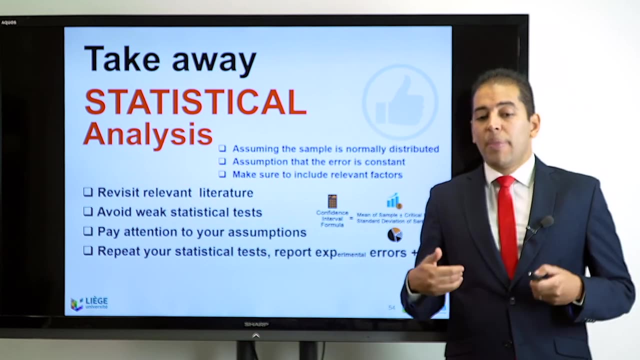 that were done in the field or in the same area of investigation. avoid weak statistical test. any statistical test that is considered as a weak test. try to avoid it. pay attention to your assumptions and reinvestigate them and test them. repeat your statistical test and your report. this is very important. 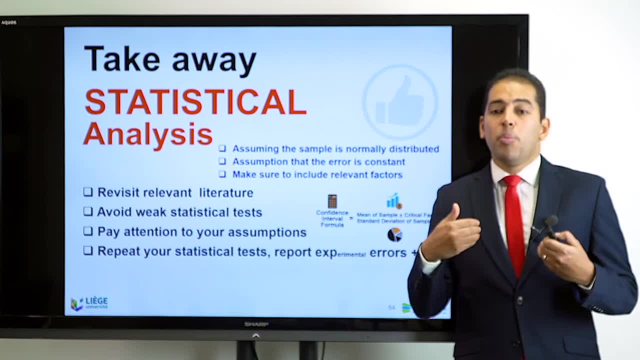 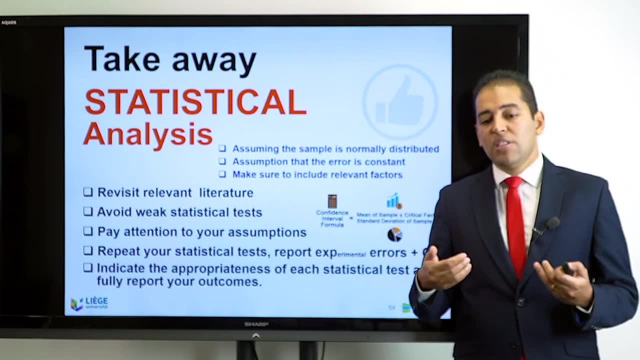 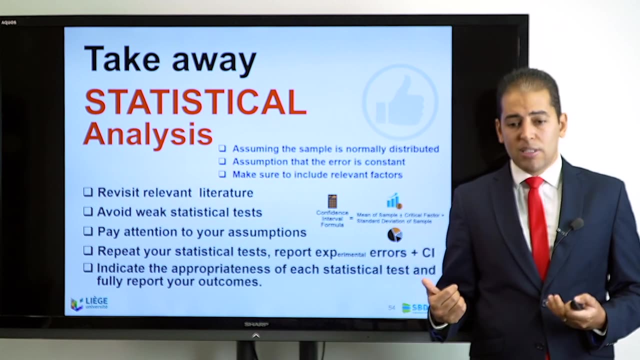 so that you detect the errors and that you detect or report your confidence interval for your experiment. and for sure, you must indicate the evidence of each statistical test and fully report all the outcomes and all the type of test that were conducted when you are doing your test. 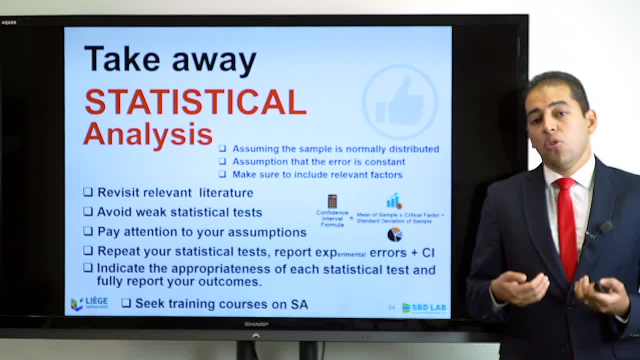 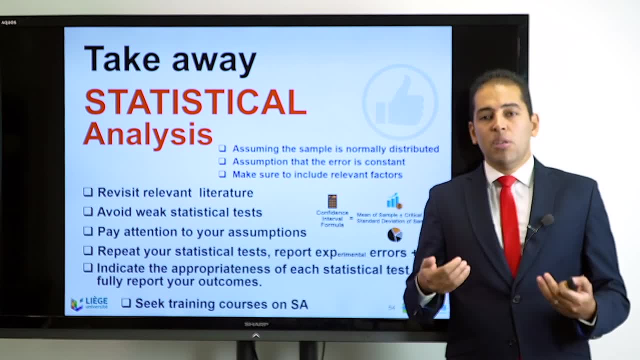 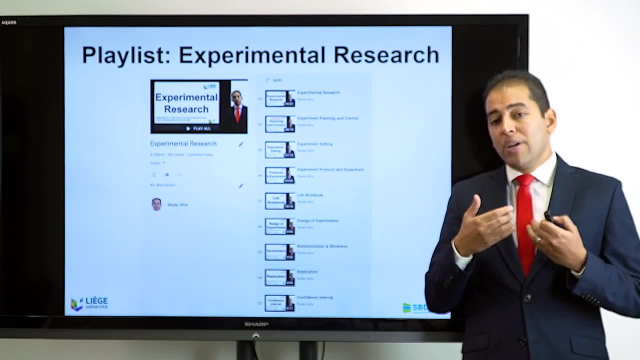 and finally, for sure, I advise you to seek training courses on statistical analysis to better be ready, able to design your experiment, conduct your experiment and analyze the data in a meaningful way and in a straight forward approach. by that I end today's presentation. I advise you to look at the following video: 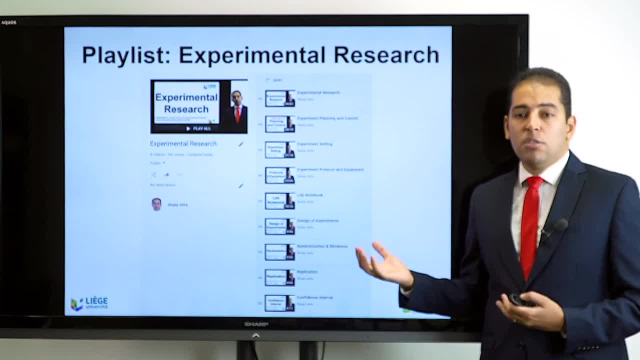 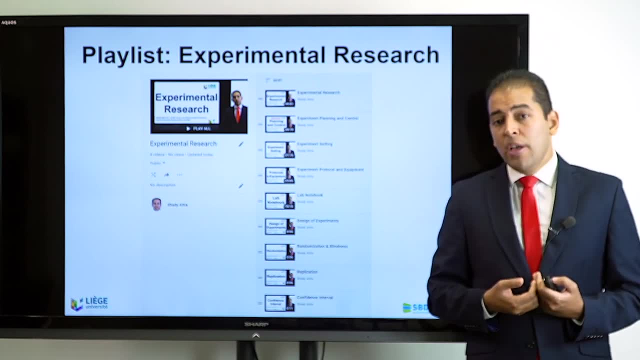 on design of experiments and don't hesitate to share this video with any potential colleague scientist who is looking to learn about statistics and perform experimental research. and finally, I thank you for your attention and I hope you enjoyed this presentation. thank you very much.